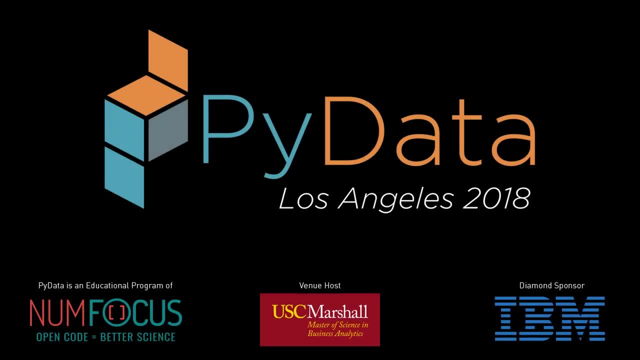 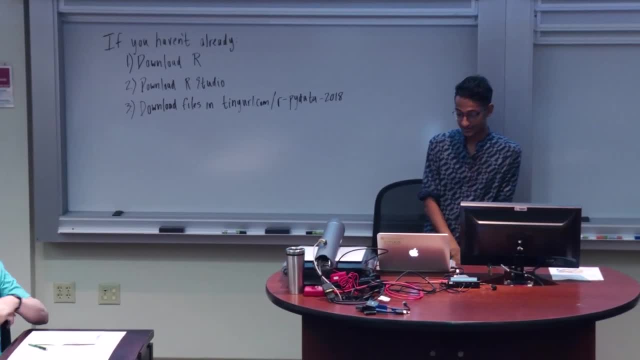 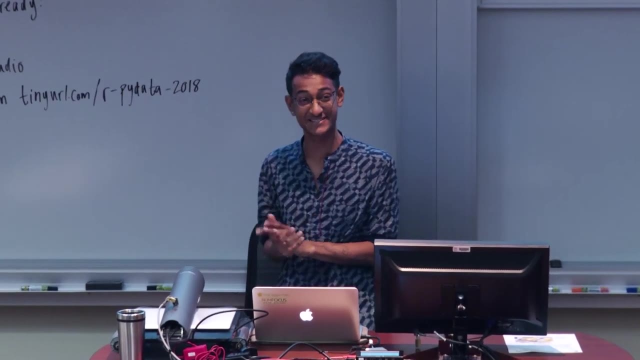 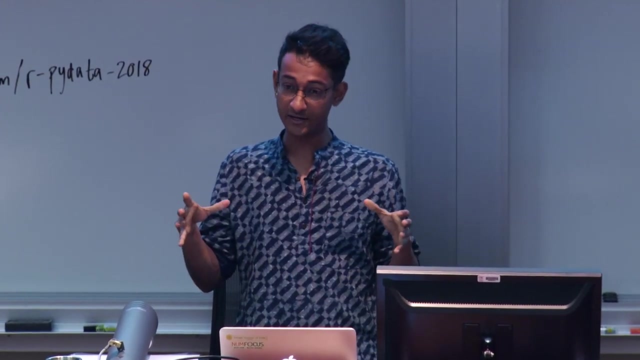 Well, good morning everyone. So my name is Bhargav. Bhargav Srinivasa Desikhan is my full name. You can just call me Gov, because my name is really massive. What we're going to be doing today is text analysis. I will be doing more of a breadth kind of thing than 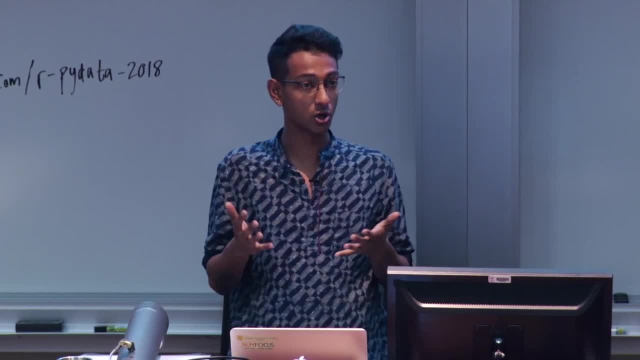 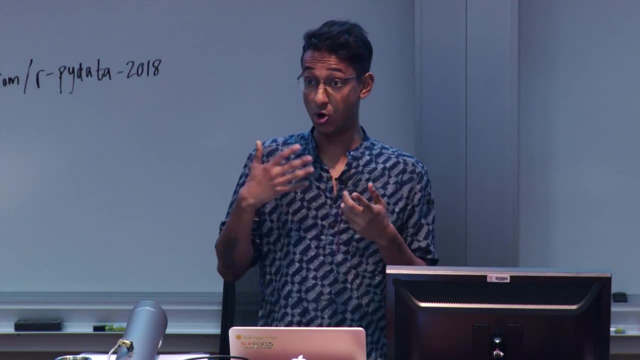 a depth. So I'm going to introduce you all to a really large variety of tools which you can use in the context of Python and text analysis, so that you can all go home or go wherever and then actually do these things on your own, on your own laptops or whatever. 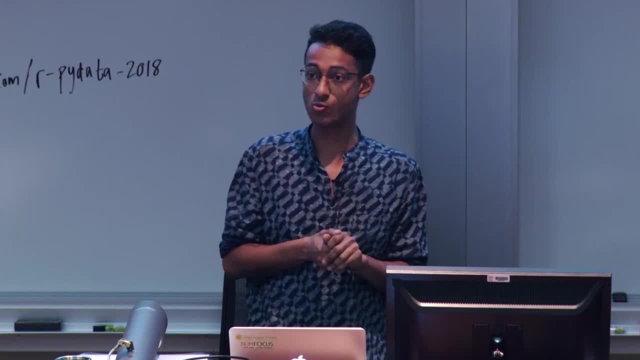 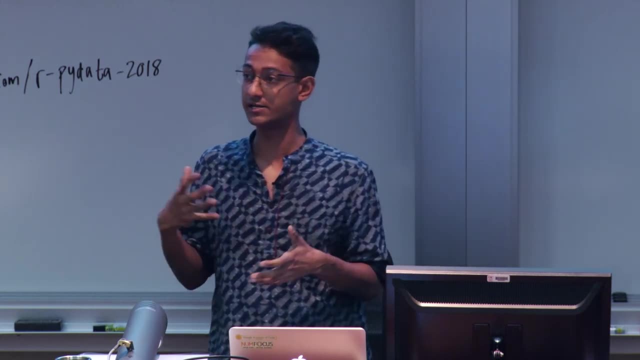 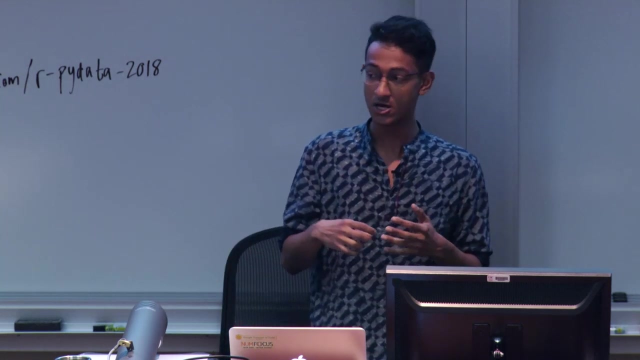 machines you're using. So the idea is to kind of allow everyone to be able to do all of these cool things outside of this tutorial as well and also to understand what kind of tools are available, Because I think what happens especially in data analysis in general, but also in text analysis, is that you're kind of overwhelmed. 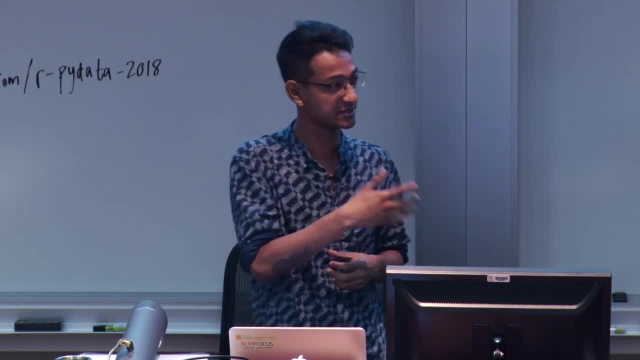 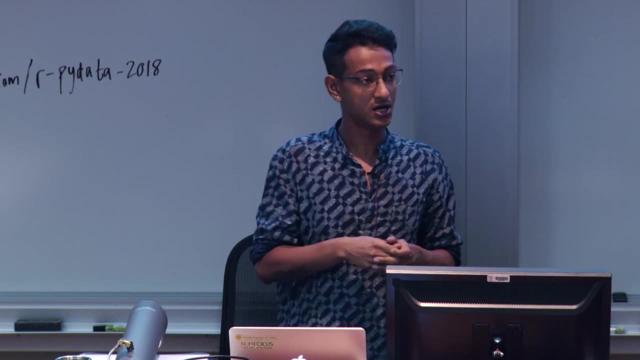 with all the different kinds of tools and you're not sure where to start. what does what exactly, and where do I get data? what's even going on? So I'm going to try and streamline this process for you a little bit, make people aware of the kind of things you can do, and 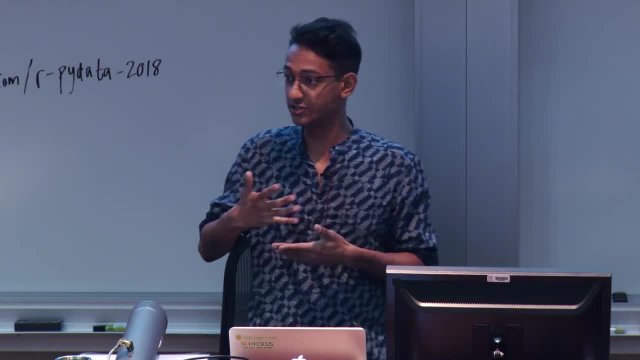 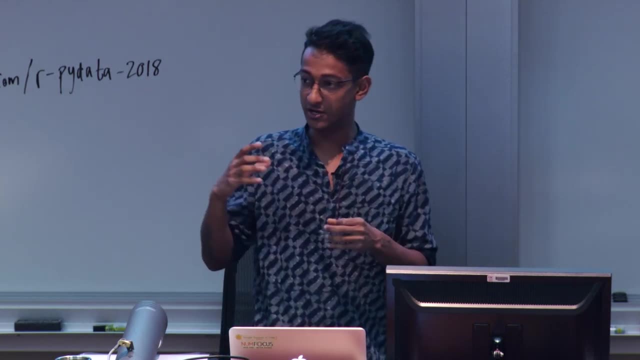 how you're going to go about doing it, And that's going to be the general theme of this tutorial. A few things before we actually get started. How many of you all have installed all the requirements or set up a Jupyter, Anaconda or a virtual environment? 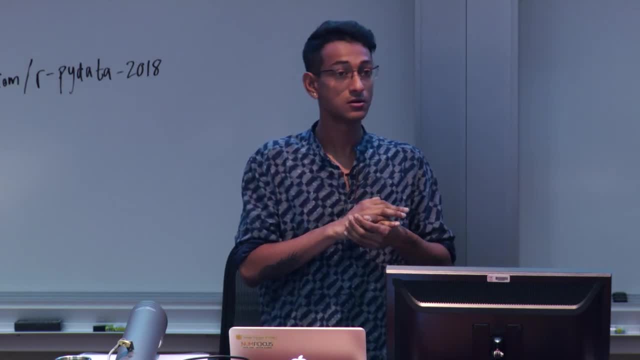 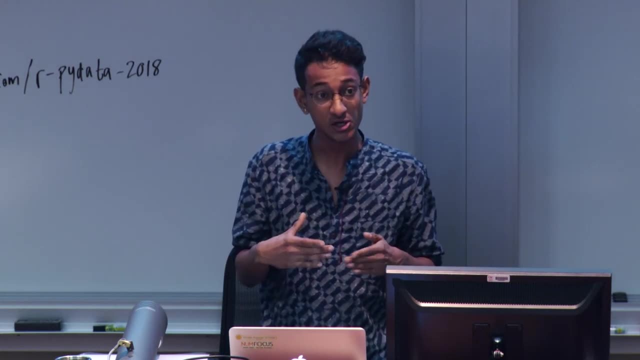 or something. Can I have a hands up briefly for those who have? Okay, that is very cool. So I understand there are some people who might not have this set up And while it would be ideal to have this set up for the purpose of this tutorial, I'm going to be walking. 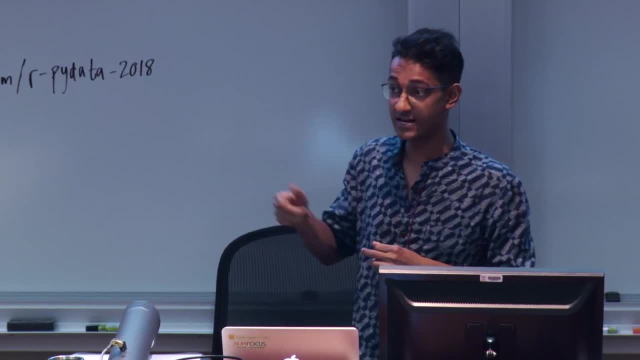 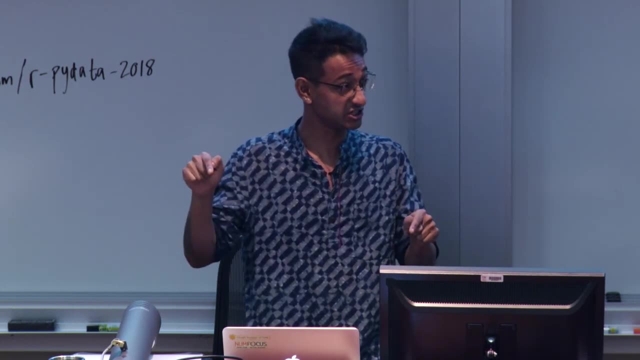 you all through a Jupyter notebook, and we're going to be going through that. But, that being said, there's a lot of information in this tutorial, So the only real thing you all will be doing is pressing shift, enter each Jupyter cell, which is not a lot. I mean there are. 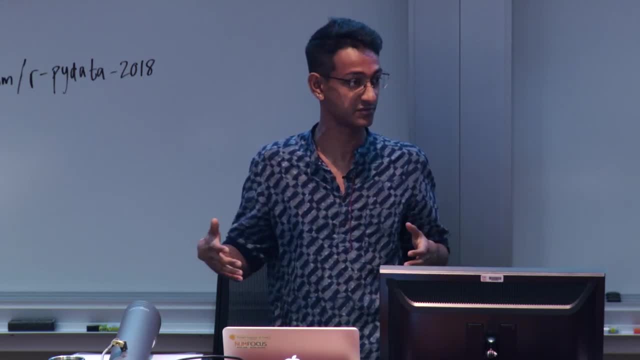 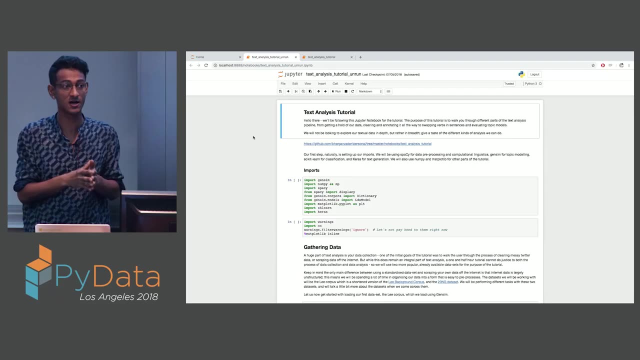 of course, a few things like looking at the contents of a particular list or something which I will also be doing on my own Jupyter notebook, But the point of me saying this is: if you somehow could not have got your entire setup ready, it is okay, It is not. 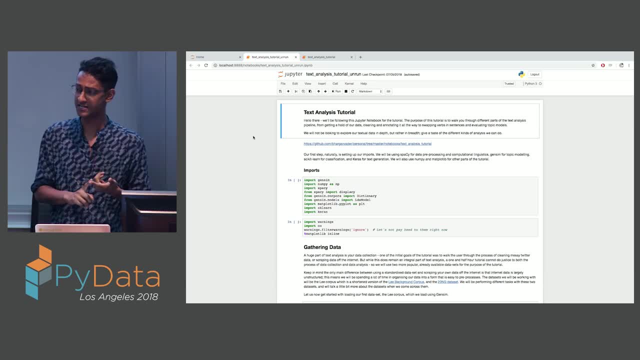 a huge problem. What I would need you to do is you should have also got an email yesterday if you were signed up for the tutorials, with the link to the GitHub repository, which has my code. If you don't, I'm going to just show you this briefly. It's really okay, you can search. 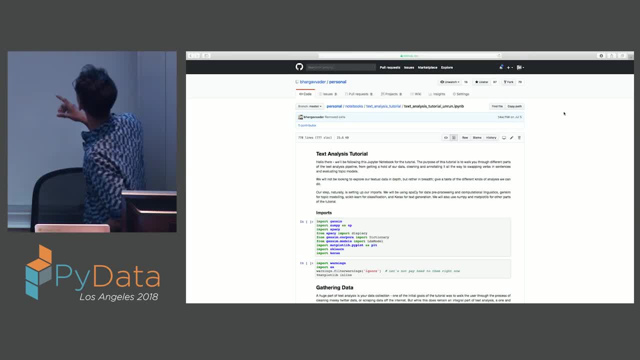 up. I'm just going to write this down if you don't have it. but it's Bhargav Vader, which is my first name, and, like Darth Vader, like V-A-D-E-R after that. So it's Bhargav Vader. 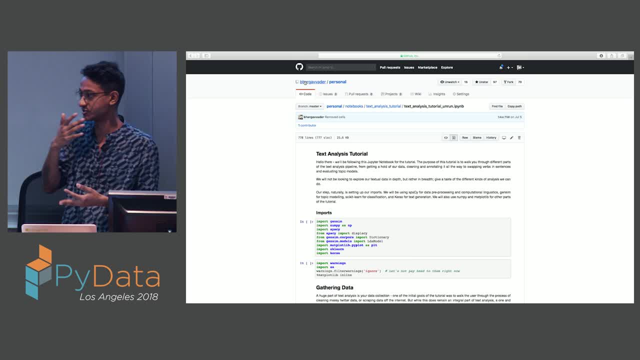 This is my personal GitHub repository and it's slash personal. So if you just go to githubcom, slash Bhargav Vader, slash personal. Yeah, Male Speaker 3. I could do that, definitely. Male Speaker 4. I think I can Hold on. Sorry, Apparently okay. hold on, I'm not sure how to make zoom. 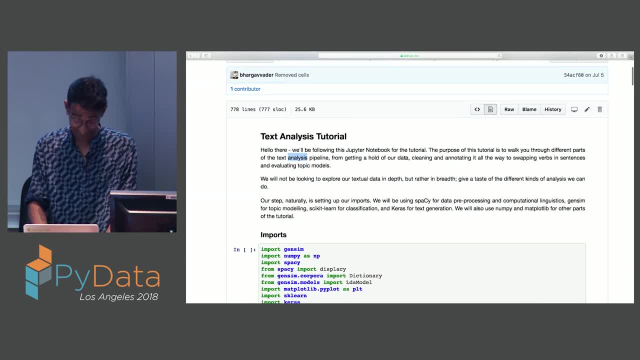 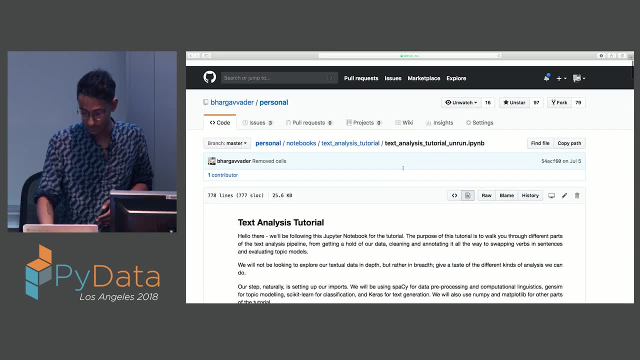 in on using. oh there we go Cool. Oh yeah, sure, Hold on. I'm just going to try that again. Oh neat, Okay, So, yeah, okay, So please. yeah, you're also more than welcome to keep. 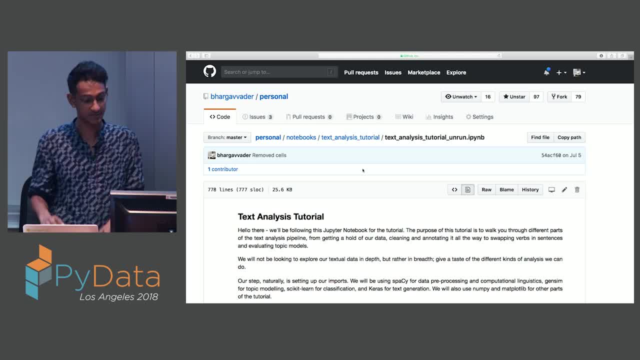 stopping me. if you have any problems with regard to the HoloLens, I'm just going to keep going. Male Speaker 5. Okay, So I'm going to try to find some more problems with regard to the how it's being done or, if I'm not seeing something clearly, Basically to find this tutorial. 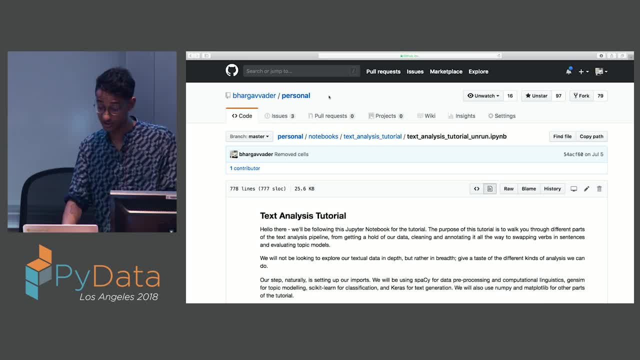 you'd want to go to githubcom slash Bhargav Vader, slash personal, slash notebooks over here. I actually sent this link over yesterday. In case you do not have this link, let's just take a second, if you do not have all of this set up, to go over here and find this. So you'd 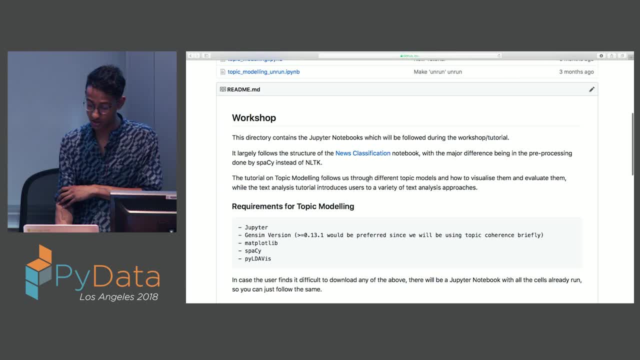 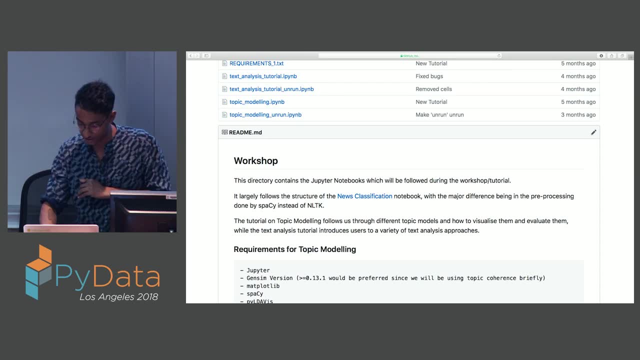 want to go to text analysis tutorial and in the read me I talk about what you would all be needing. It's not going to take me long. I'm not going to go all the way down, so I'm gonna spend around five minutes to just kind of find this particular. 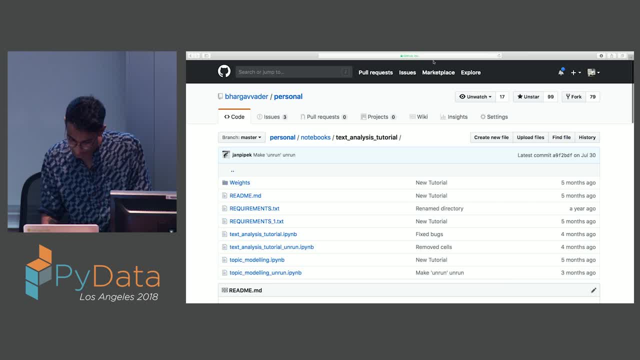 page. if there any problems in finding this page, please put your hand up and I'll get you to find it. so again, it's githubcom: slash cargo waiter, slash personal, then notebooks and text analysis tutorial. so ideally, if you do have, if you would have got this and downloaded and had like your environment. 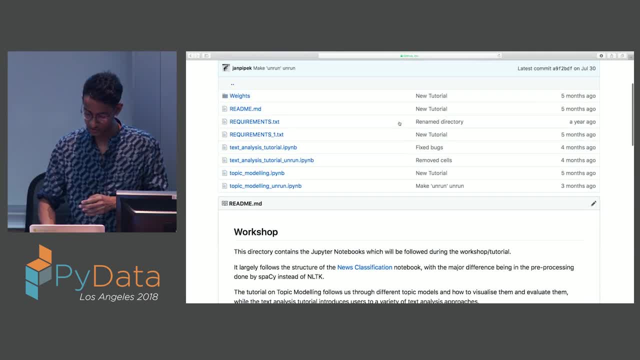 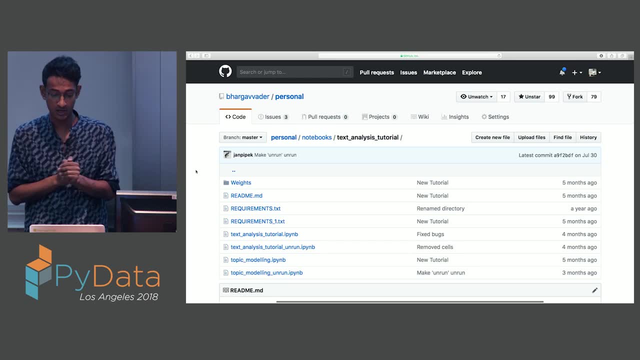 set up. that would be really, really great. I've also given instructions on how to do this. it's basically setting up a virtual environment and downloading, using pip or whatever you would like to use, from the requirements file and then running the Jupyter notebook, if anyway, again, if anyone needs any help with. 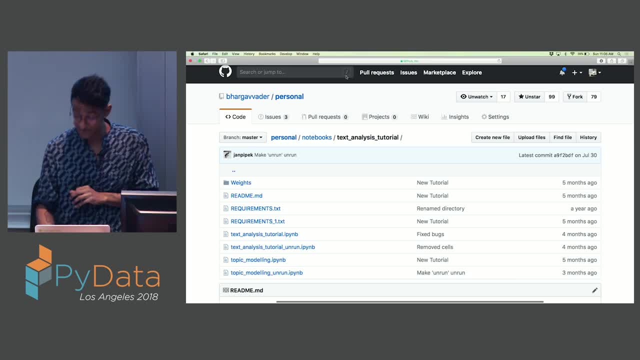 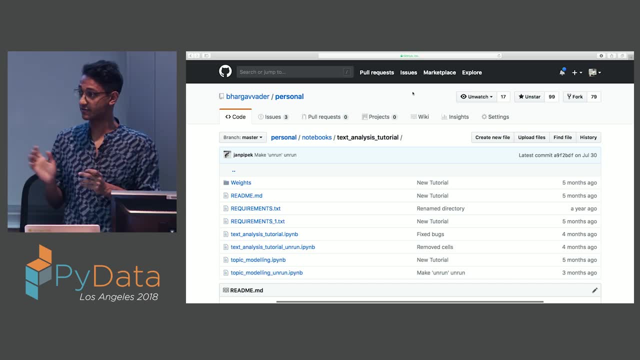 regard to this, I'm over here, I'm just going to give. so it's 1105. I'm waiting till 1110 to kind of get people over here. so I'll just give five minutes for everyone to find this. so let's see if I could close out for a second. 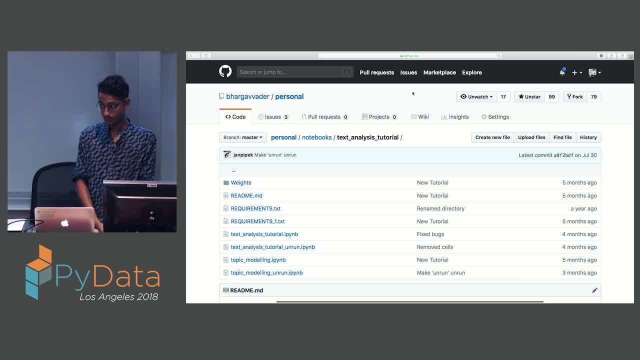 the first thing that I'm going to do is I'm going to give the days a little bit longer, and I know how to do it when I upload this video. so I'm just going to hit on my computer and I'm going to give it a few seconds and see if you would. 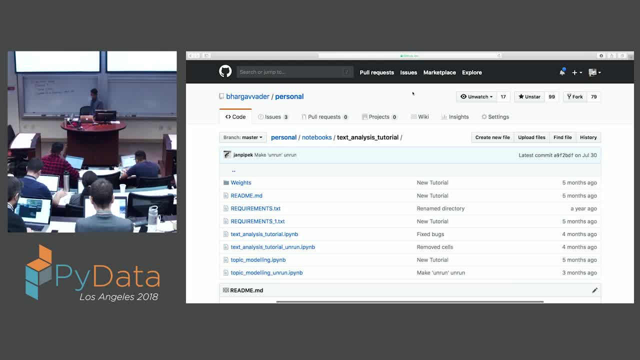 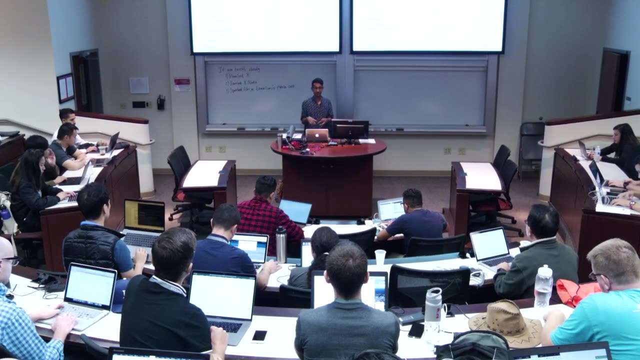 want to do it with your computer, so I'm going to give it a few seconds to see if I could do it in my computer also, just to note that, even if you cannot find this, I will be running all of these notebooks on my machine and you'll be able to see all of that and I 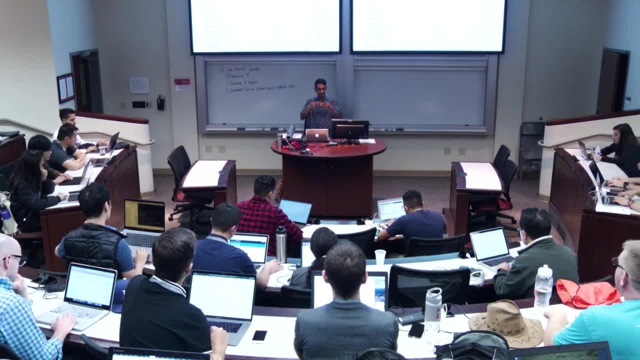 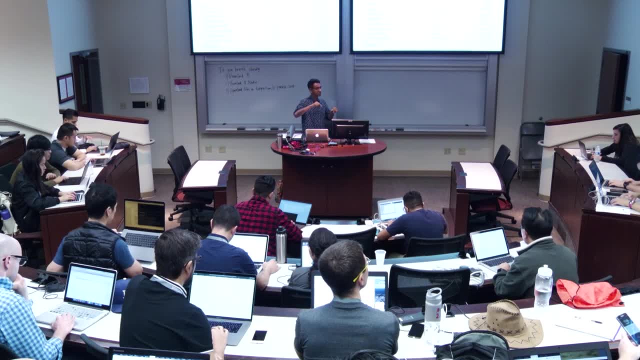 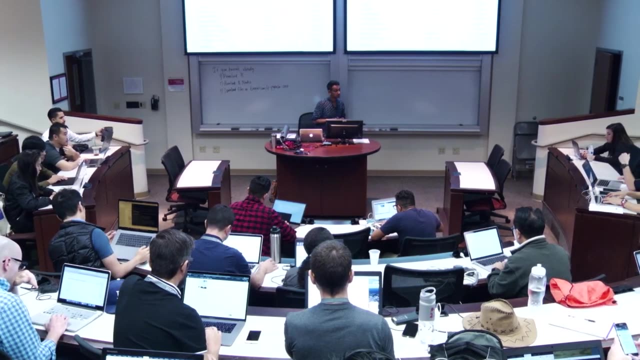 will be talking about it. it's just going to be a lot easier if you also have it in front of your computer. and I will also be talking about like I would encourage you folks to all try out different Jupiter cells if it needs to be done. but that, yeah, ok cool, I was just saying that you don't absolutely need. 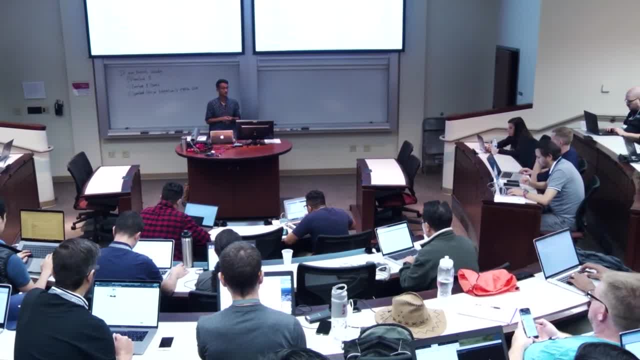 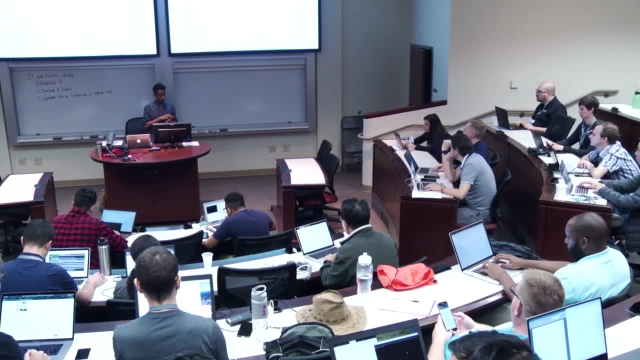 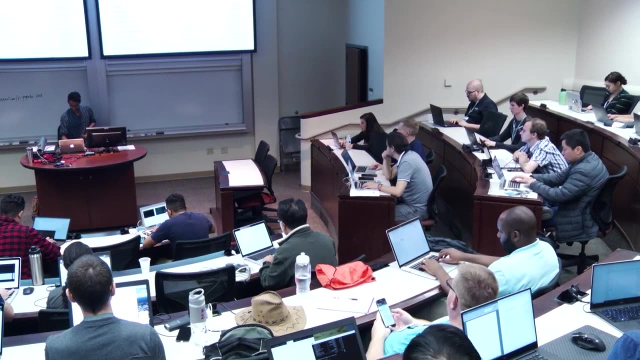 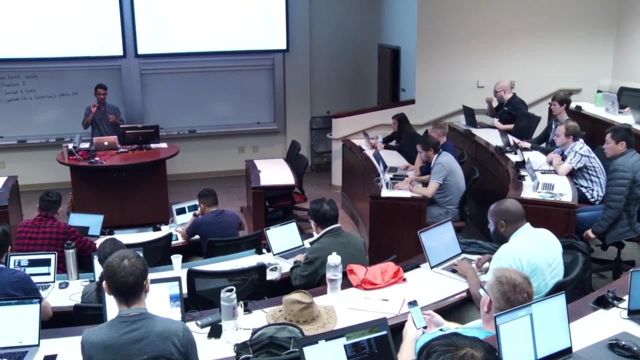 this page. it'll just be very useful. sure, so it's a Python, it's Python 3, 3.5, 3.6. but that being said, I also- I mean you can use Python 2 for this tutorial as well. well, I have. if you do, then I have a few code snippets you'd probably need to use. 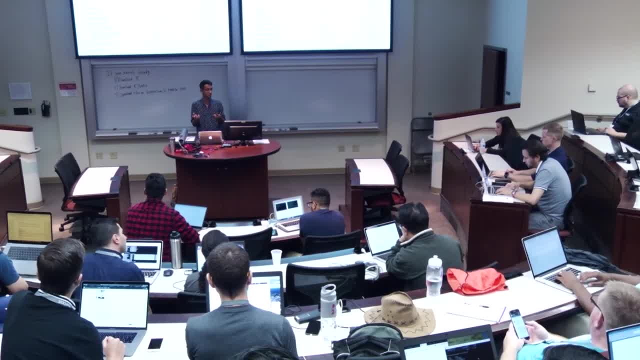 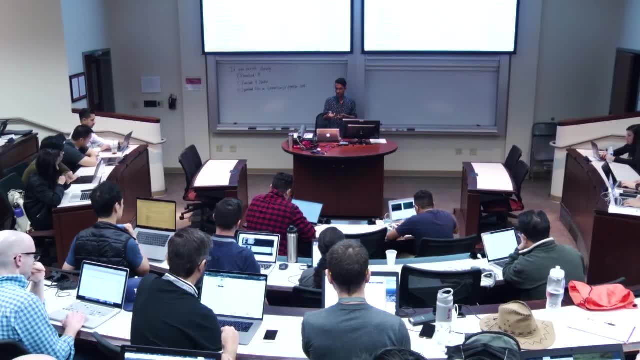 because of the Unicode and because we're dealing with textual data, so of course we need to be very clear about the Unicode part. but apart from that, you could use Python 2, Python 3. you don't even need a virtual environment. that was just what I use. or you can use piya and vanna condos- whatever you want you can. 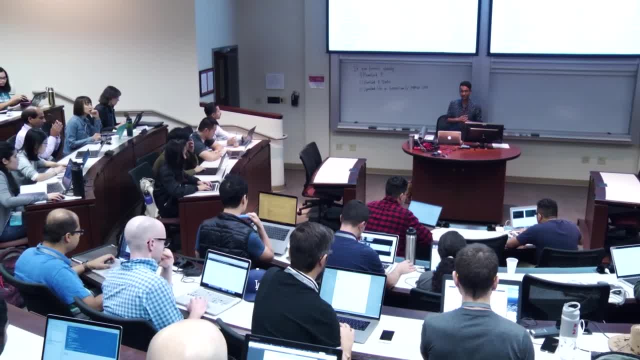 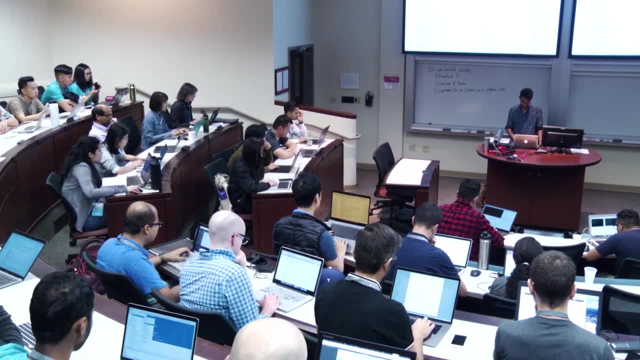 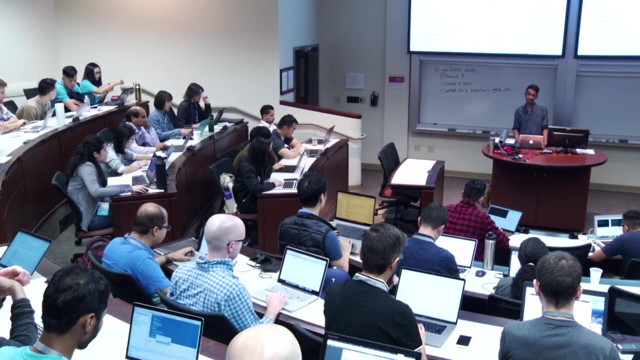 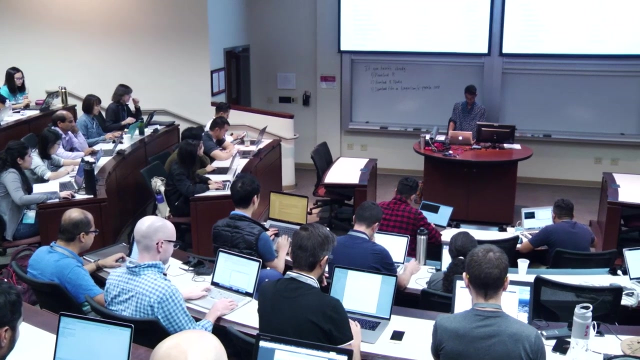 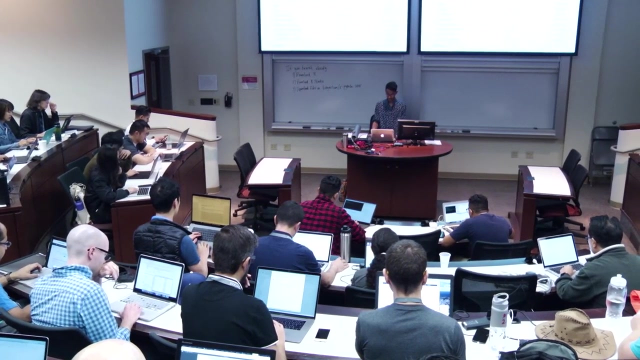 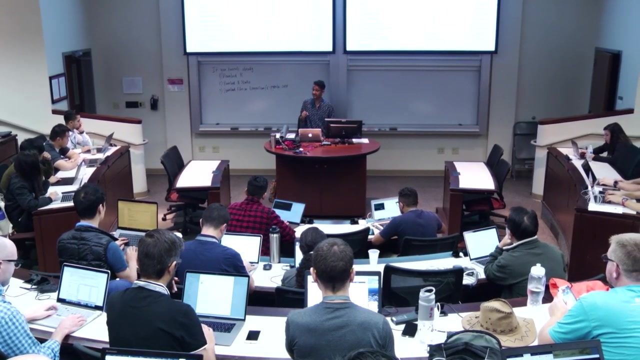 use anything, it's just mine would be on Python with Python 3 you. another note is: if you all plan to install all the requirements right now, it might take some time because there's a lot of time to do that. there's a lot of time to do that and you should. 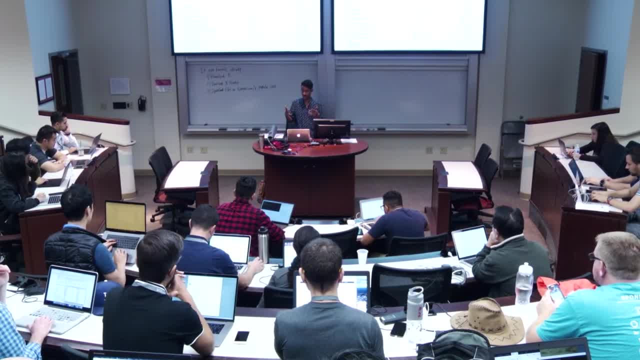 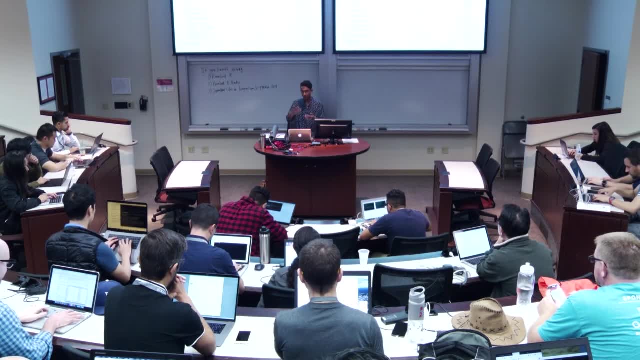 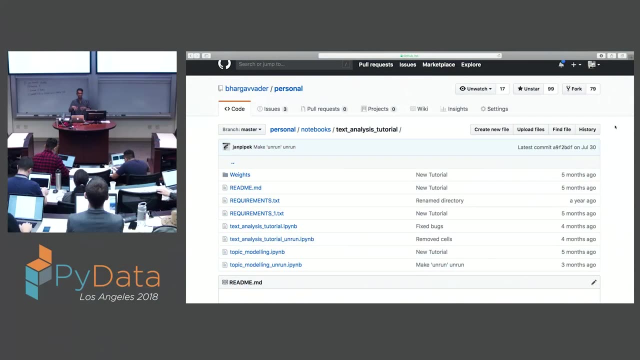 BAC has a language model which is, I think, like 45 MB or like, depending on what size. it might take some time, In which case, I mean, you could probably have it running on in the background, the installation. but again I would like to make it clear: it's not absolutely necessary for you to all get. 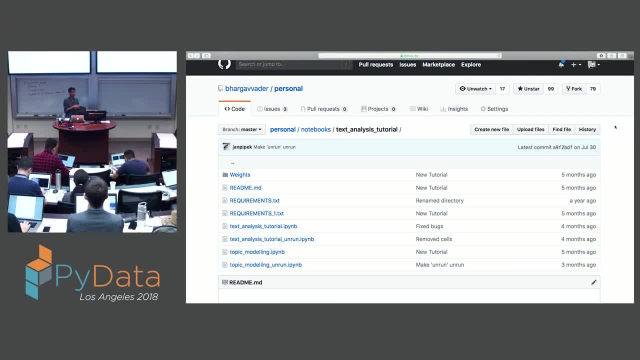 something out of this tutorial, though it would be very, very nice if it's installed so that, when you have time to go through this on your own, you can. So the spaCy language model, which I will talk about in detail, of course, but I have 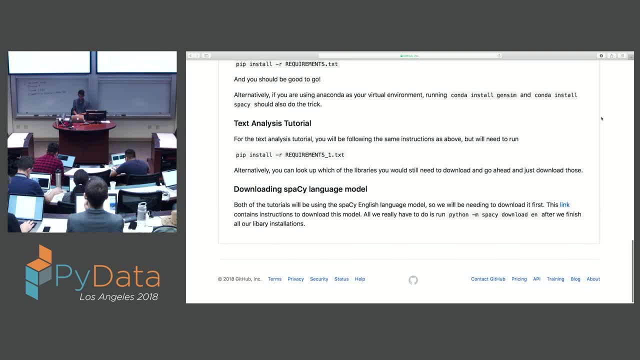 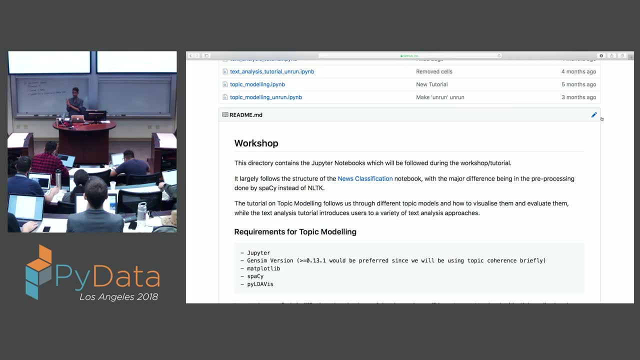 a link over there which talks about it and how to do it. And these are the Python packages. we'll be using: Jupyter for running the notebook, Gensim for topic modeling, Matplotlib for plotting, spaCy for other text analysis. 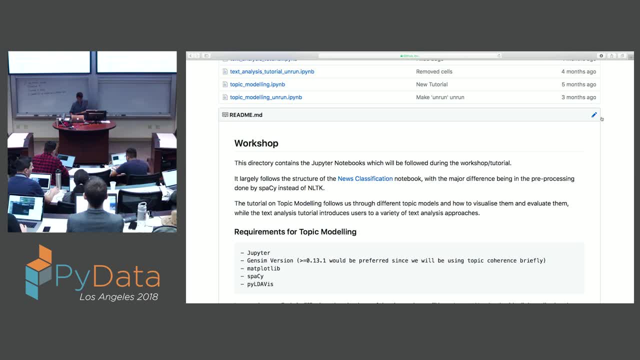 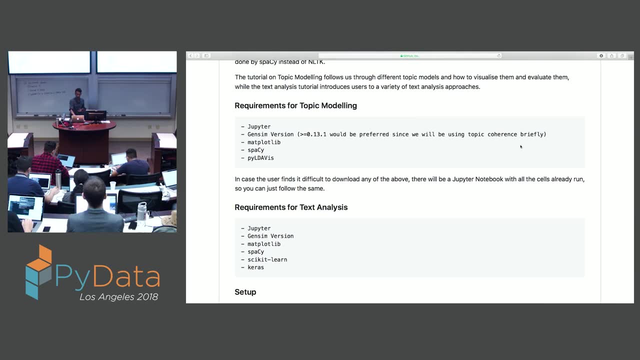 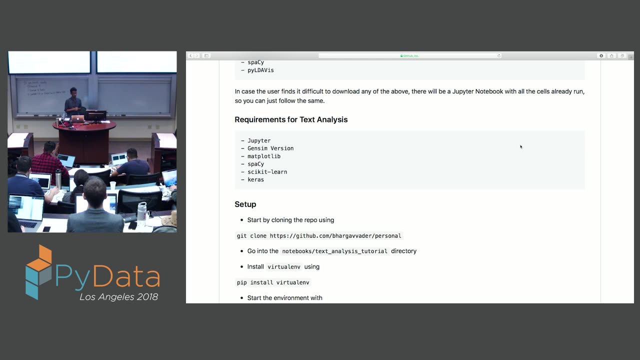 And some visualizations. Yeah, Yeah, so there's no, so I've mentioned that over here. Requirements: underscore: one is the one for text analysis, which would have Jupyter Gensim, so there are two tutorials in this. 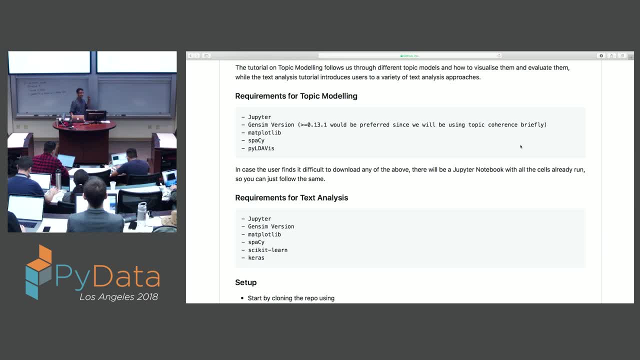 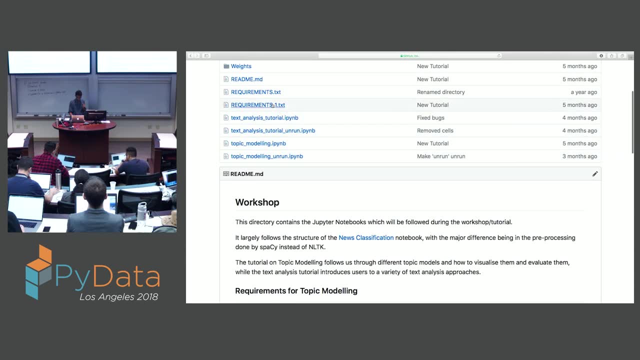 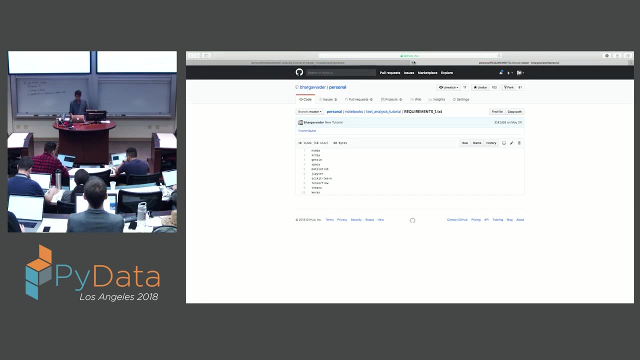 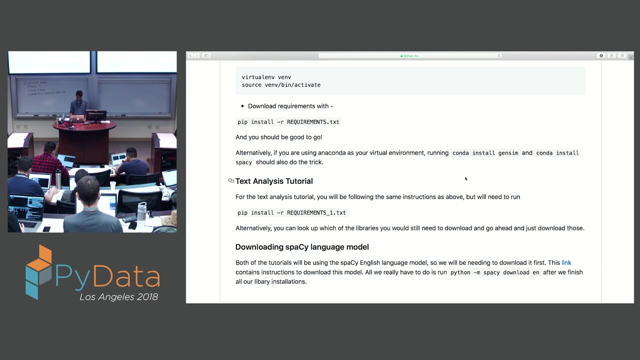 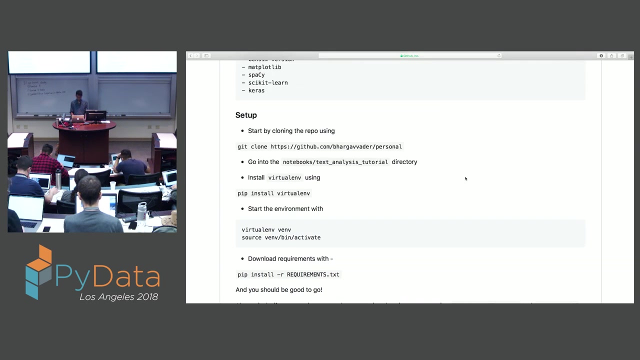 So you have topic modeling and you have text analysis. We will be doing text analysis. So I believe that The requirements underscore. one file has the ones for the tutorial. we'll be doing no problem. Cool, It's 11.10, so I'm going to start. 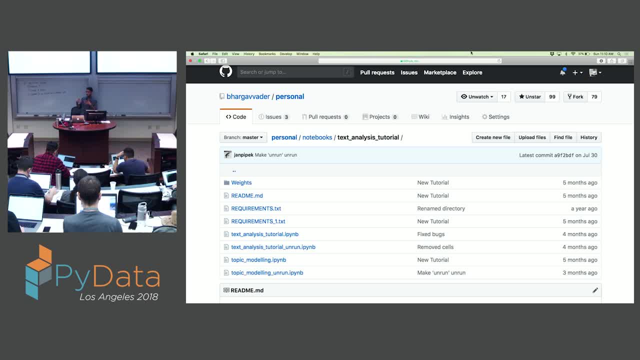 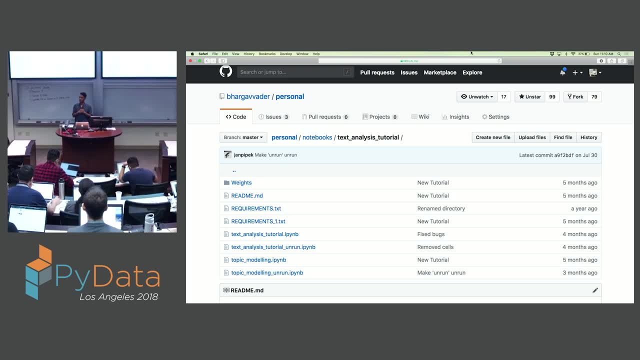 Again, just to note, because I realize there's a lot of installations and a lot of things you might want to set up. it would be very, very nice if you could all spend some time after the tutorial or during the time of the conference to actually install all the things. 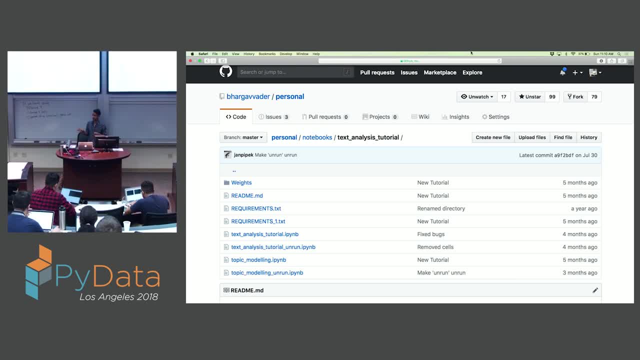 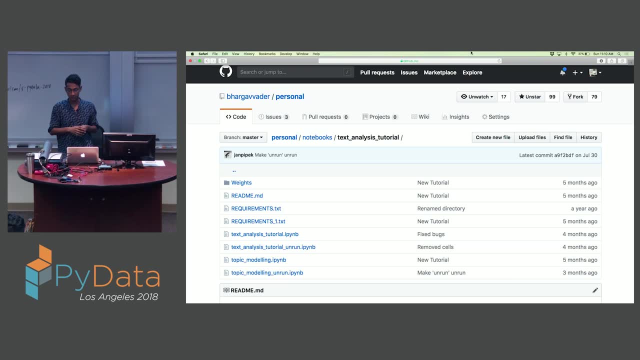 I've talked about here, because they're going to allow you to do this- on your own, of course, so that you're not just stuck to what I'm going to be talking about in the next few minutes. Cool, Thank you. Bye. 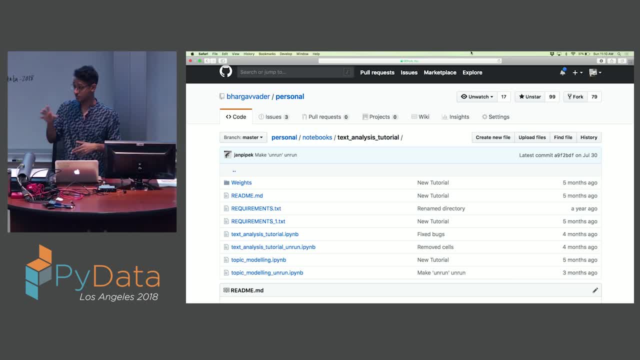 So that's just going to be really easy to get in this tutorial. but if there are problems with installations and things like that, starting right now, I will not be talking about those right away because I will be spending the rest of the time to actually talk about the. 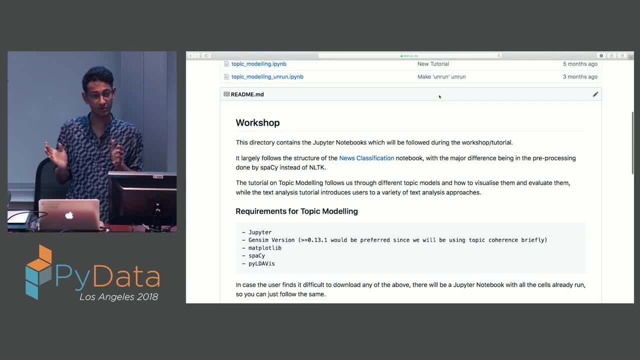 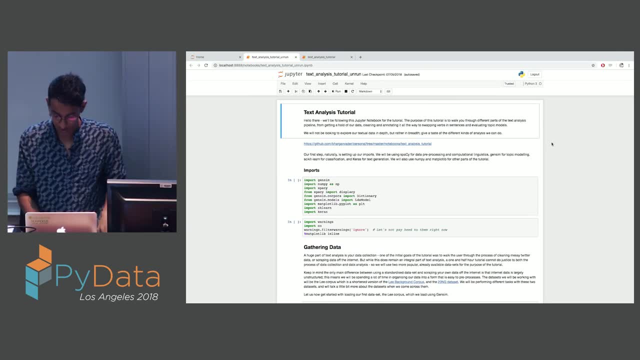 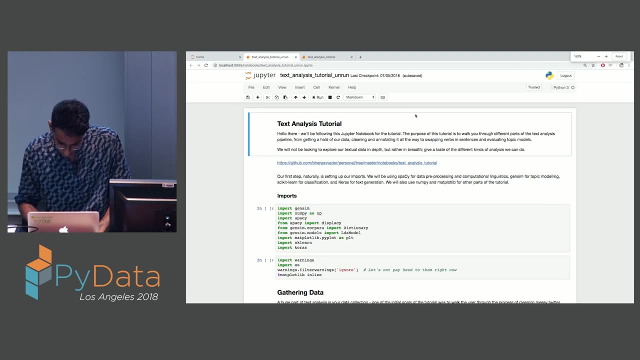 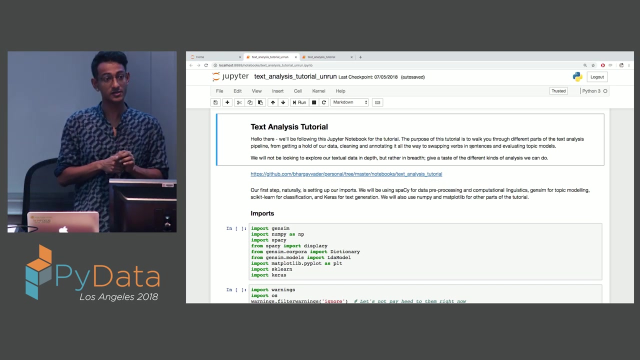 tutorial. So are there any questions before I start? Any problems, Everything OK, Awesome. So It's going to zoom in. is this okay? can everyone see this? or is the perfect level of zoom? yeah, cool, awesome. so we're going to be doing text analysis. um, text analysis is data. 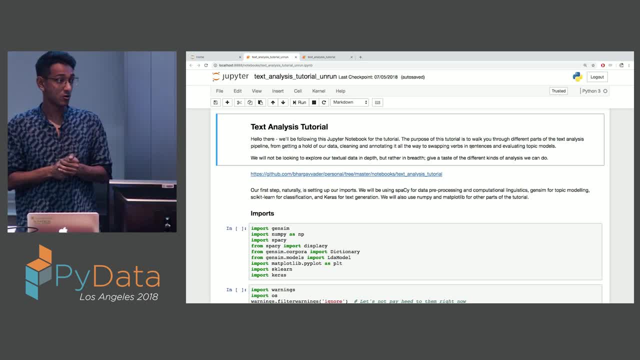 analysis where our data is text. now what I personally find where you need about text analysis is that it's very easy to actually get this data and it can also be personal and things that you care about. I find sometimes in your generic data analysis you might get kind of lost in the numbers or not very interested in. 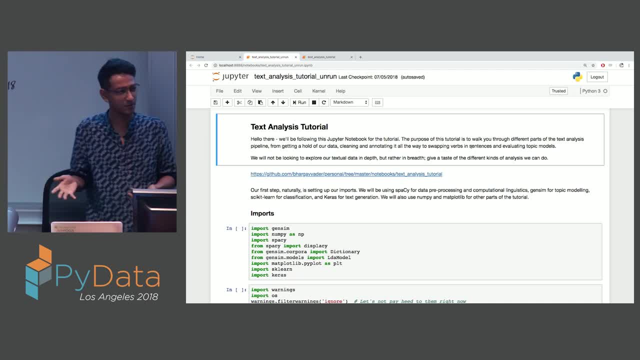 what you're trying to do like. the more common data set is, I think, the Boston housing data set for regression. it's kind of boring predicting the prices. there's the iris data set. it's again not super fun. so what for me? what I personally like about text analysis is I can use whatever text I want to. you can. 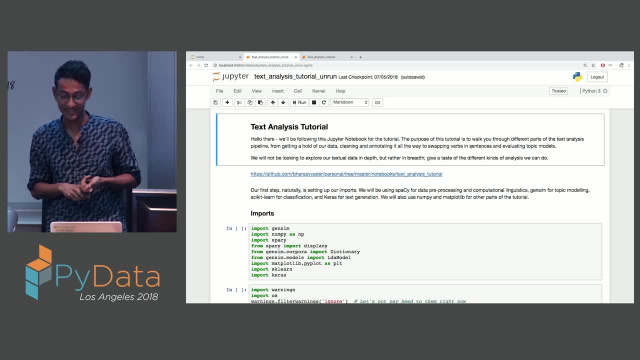 pick up tweets. you can actually. if you have legally bought PDFs, you can analyze those. you can analyze whatever kind of textual data you want. newspaper articles are a bunch of fun. I used to. I used to use the messaging WhatsApp app a lot back in Asia and Europe, so I used to actually analyze my own textual 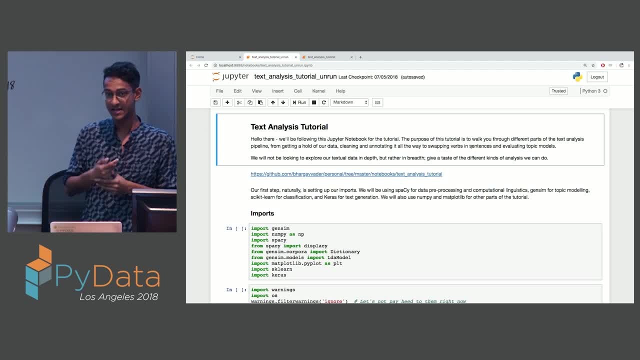 conversations which I sat with my buddies and that was also a lot of fun, and the point of me saying this is that text analysis- one of the huge parts of it, why it's interesting, is the fact that you can actually use personal data to get insights into what you're using. it's also really you also use a lot of course. 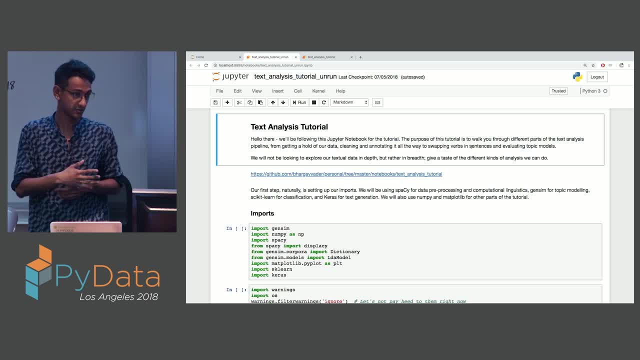 in industry by a lot of people trying to figure out like advertisements so on and so forth you can have. you have chatbots. it's also a part of text analysis. so there's a lot of generally cool stuff you can do using text analysis and text. so that's why I'll be talking about that in particular. now the idea again. like I, 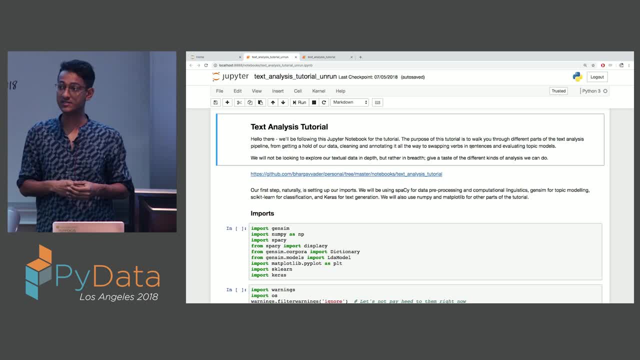 talked about before is breadth and not depth. so I will be talking about something called computational linguistics, which is basically making computers deal with linguistics. so you have things like parts of speech right, like nouns and verbs and so on. how do you write computer code to identify? 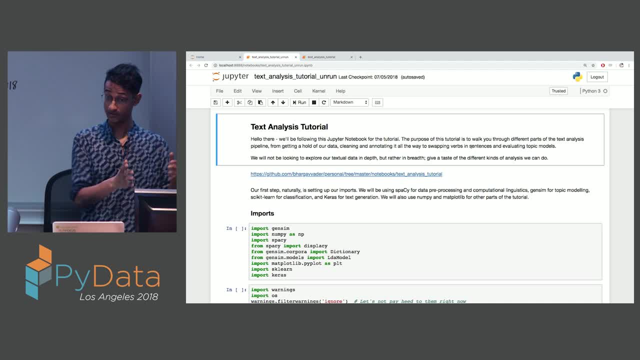 nouns and verbs in a sentence and in paragraphs and so on. that is one part of what I'll be talking about. then there's topic modeling. topic modeling is: if you have lots of large text and it's completely disorganized, how can I find underlying topics, like, if it's newspapers, how do I find like a 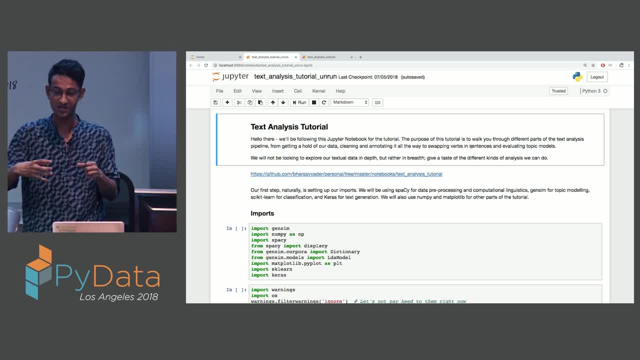 sports topic, a politics topic? how can I find this from text? how do I classify text into different categories? I've already found out for myself like spam or not spam, which everyone hears, uses email, I'd suppose so most people here would be using email, so you'd have spam and not spam. this is text classification. 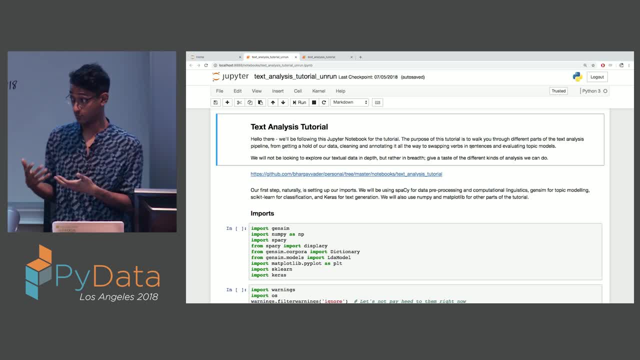 then you also have text generation, which is like what chatbots are doing, or you're kind of having a conversation or talking, so to say, with an algorithm which generates something resembling human speech. so there's a whole wide spectrum of really cool things you can do with text analysis, and we'll actually 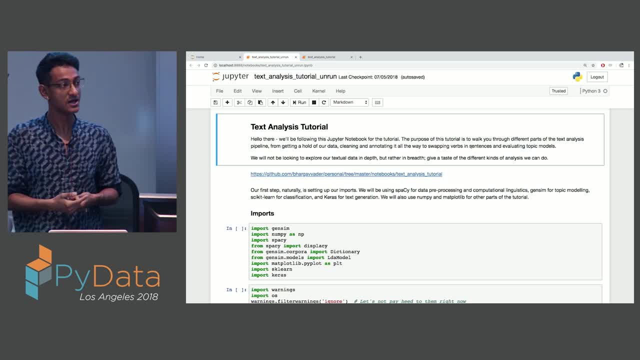 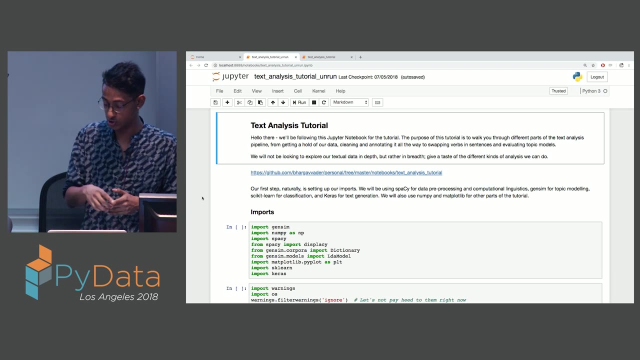 be very briefly going to do all the things I just talked about. it's gonna be kind of fast. that being said, questions are totally welcome and awesome, so please keep stopping me. if something is not clear, and well, let's get started. so what would be ideal is if everyone had this particular Jupyter notebook. 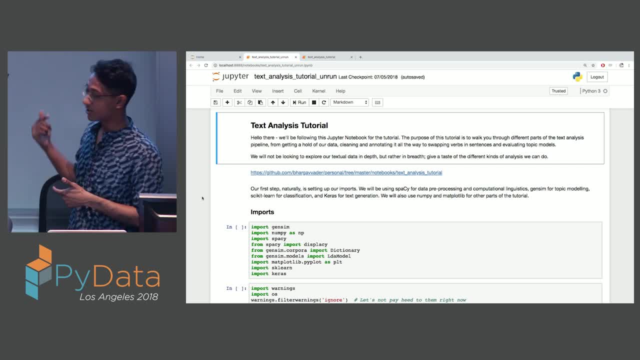 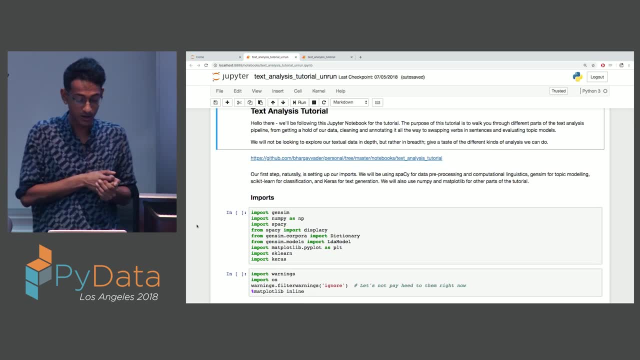 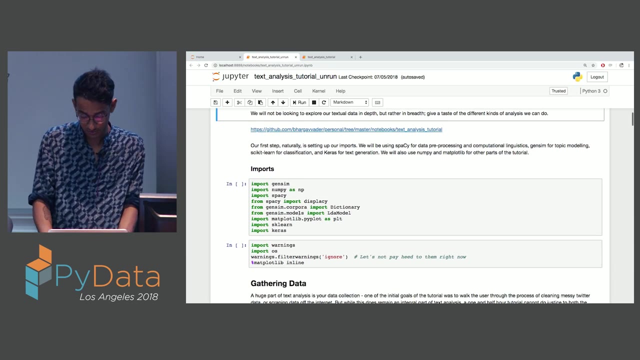 open on Jupyter, but if not, then we're just going to be watching me press, shift, enter instead of doing it yourself. briefly, so, the most. the first part about text analysis, usually, of course, finding your textual data. so that's what we're going to be starting with. I'm going to get my import set up, very briefly going. 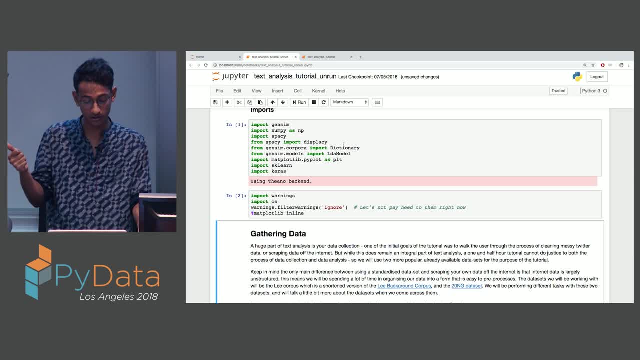 over the imports we're using or the packages we're using is what we're going to be doing first here. so your files are going to show up, and all you're going to want to do is you're going to have to come back to your Jupyter, and next to the file that you're going to be using is a folder called. 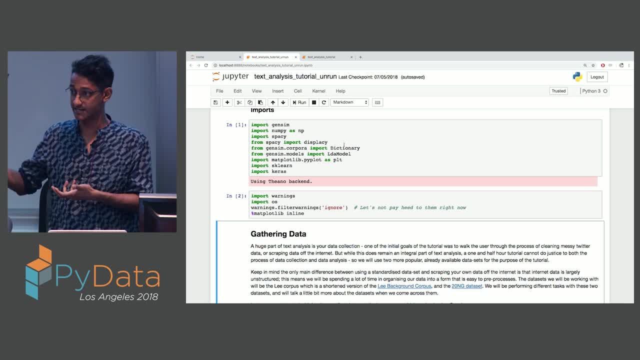 numpy. and now it's a very simple way to do this. you can just go to the folder here and just start typing, or just type in your context, and you can just go to the folder, close down and you can see that it's already done. so what you will. 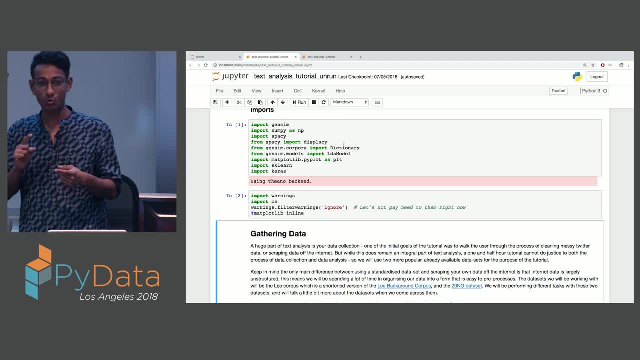 want to do next is is to make sure that we have the index, and index is ones old, and then we can go ahead and we can add it to the file which is recorded and then okay for teaching or learning NLP stuff or computational linguistics, but for 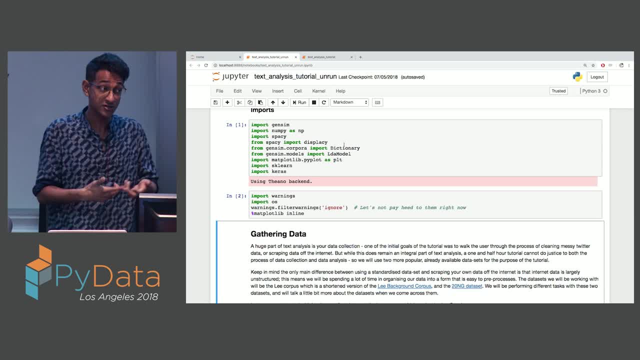 anything practical if you want to do really cool projects or even anything. you spaCy can actually be used in your- you know- production level code. so we want things to be practical, so we will be using spaCy. that being said, NLTK can be useful for learning about natural language processing. then we have matplotlib. 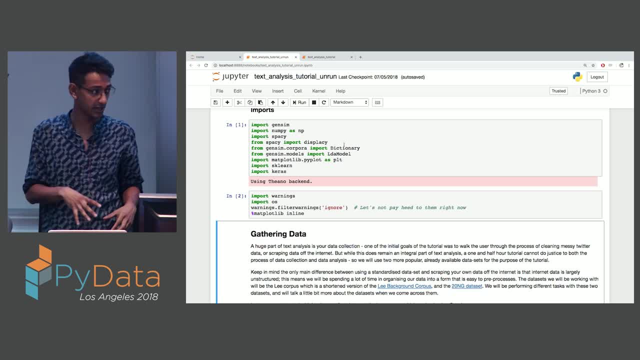 to plot stuff. scikit-learn is a machine learning library which will be using for classification, which I talked about before. this is to just briefly introduce scikit-learn in the context of textual analysis. and then we have key risk, which is a deep learning library, which is a kind of machine learning, where we're 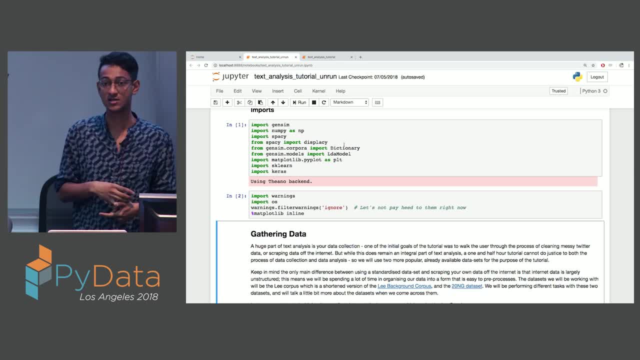 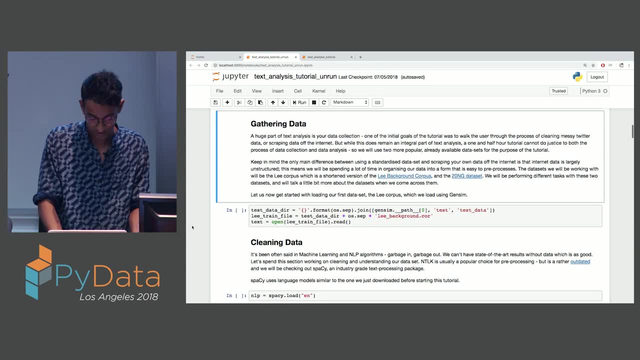 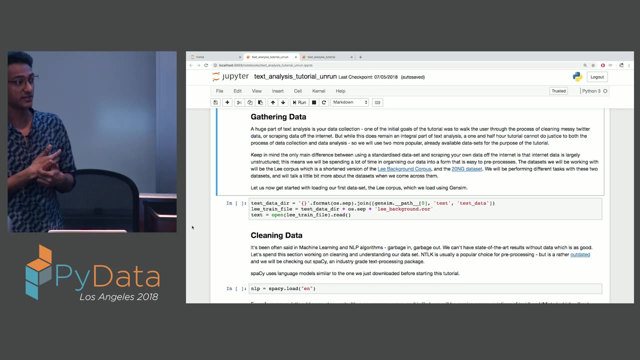 going to be dealing with neural networks and generating text. so these are the libraries we're going to be using today and I've just set up the imports and we have warnings and OS just for some other stuff. then we're going to start with gathering data now. I've talked about earlier why I like textual analysis. 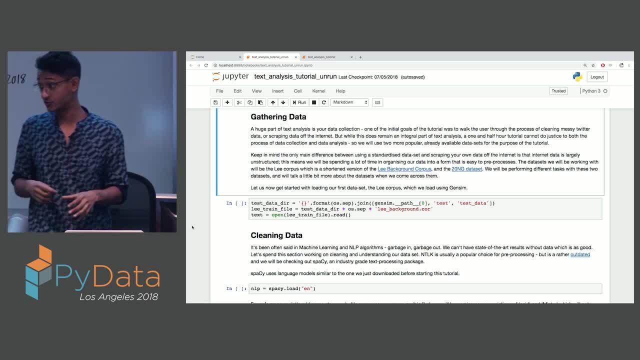 you can see that I'm using a lot of textual analysis. and I'm using a lot of analysis because I can get my data from anywhere, and when I started doing this tutorial, I started doing the whole tech, like you know, gathering data part. I wrote code to like: go on Twitter and scrape Twitter data, which is always 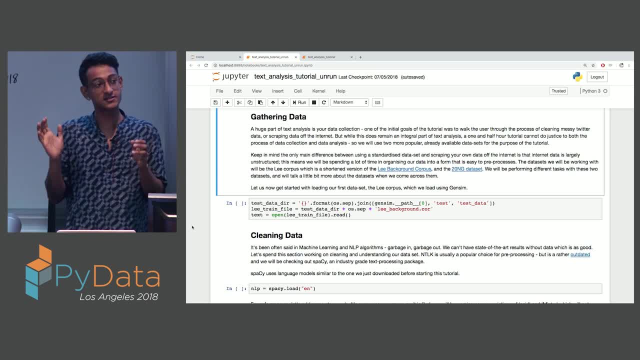 interesting because it's super relevant, right. but now the thing is that takes a lot of time and effort and ended up becoming a tutorial of its own, which I could not fit into this so well. I would love to talk about it, if any, if you want to. after this, for this tutorial, for the text, we will be using a built-in data. 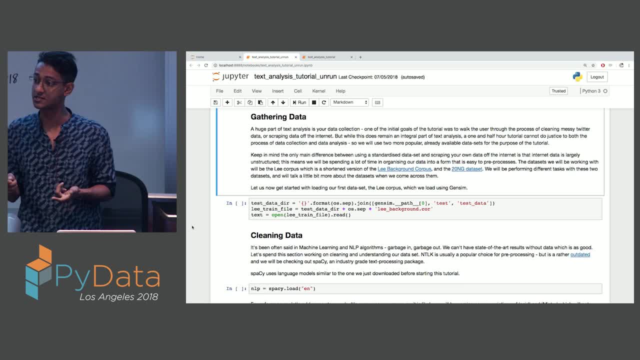 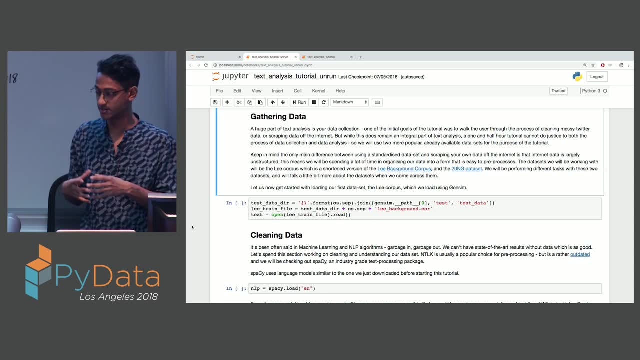 set which comes with Jensen, called the background corpus. it's basically 300 newspaper articles from an Australian newspaper broadcasting agency. so the context is Australian news early 2000, which is not super exciting but it's very easy to get. so it's what we're going to be using for the purposes of this tutorial and something called the 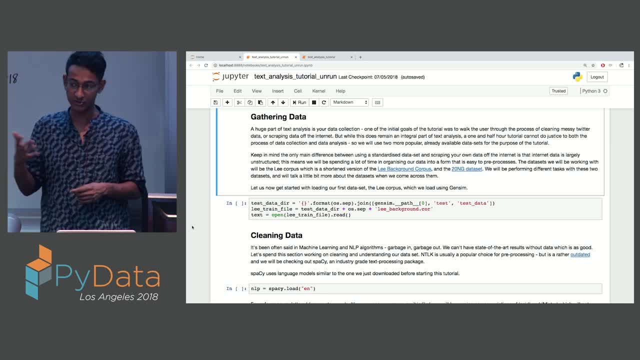 20 ng data set, which stands for 20 news groups, which is basically a massive newspaper. so the theme is newspaper articles, because it's kind of easy to understand and play with. but what would be ideal is to have some data which you know would probably of. 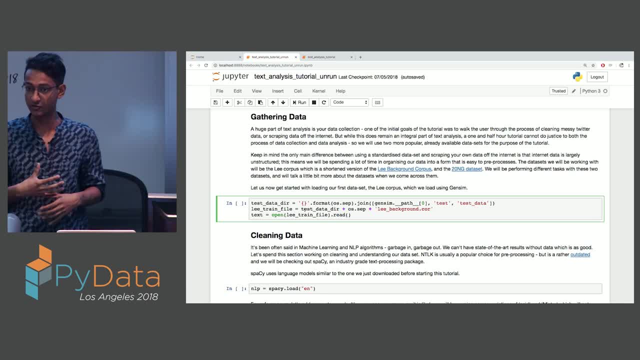 course, based on either your business model or whatever, or if it's on something personal, it's a lot more fun, for the purpose of this will be using early 2000 newspaper articles, and how we're going to be getting this data is, well, the first three lines of code over here, which is actually on the Jensen. 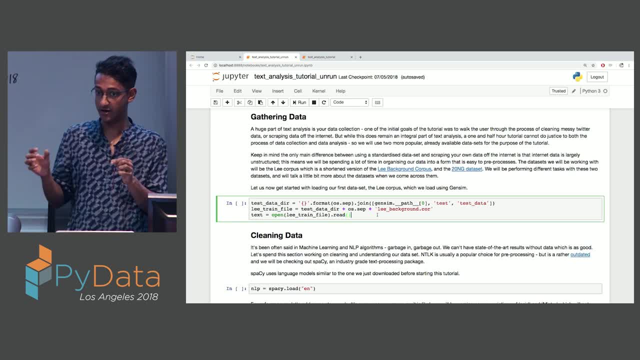 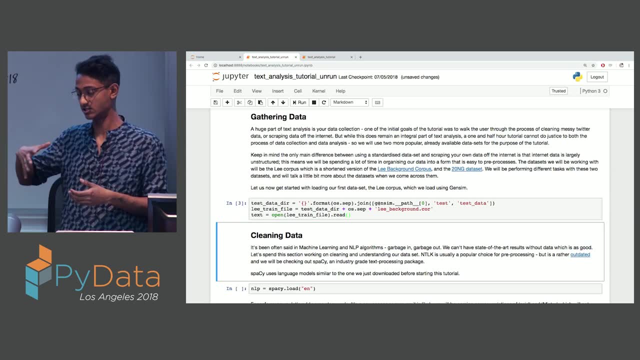 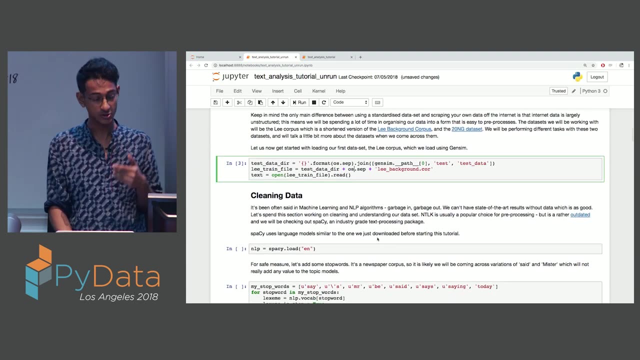 website. we're basically loading our test data from where we've installed Jensen. so what's happening over here is doing OS that's up and using the Jensen path will be basically accessing our own data set, so we're going to be using that data set, the data. so now our file, which is called text, contains all of our newspaper data. 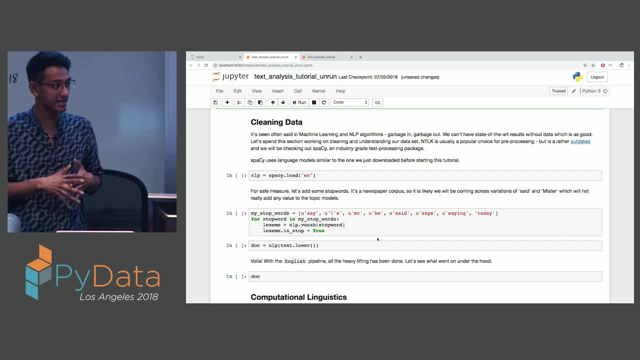 now this is a huge. I mean you like cleaning data in general is a huge, huge problem in, or no problem or thing you have to deal with in all kinds of data analysis. but in textual analysis it kind of becomes even more important because I mean you again heard this probably, or you should hear, hear about this when it 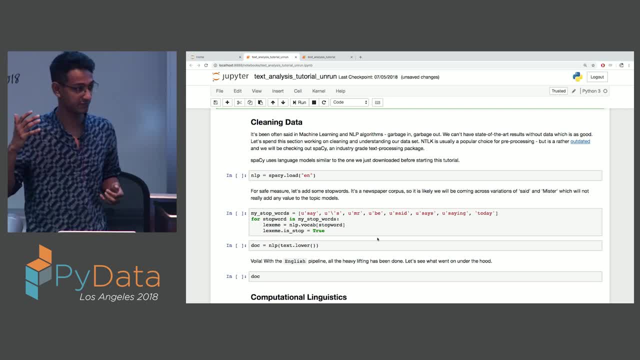 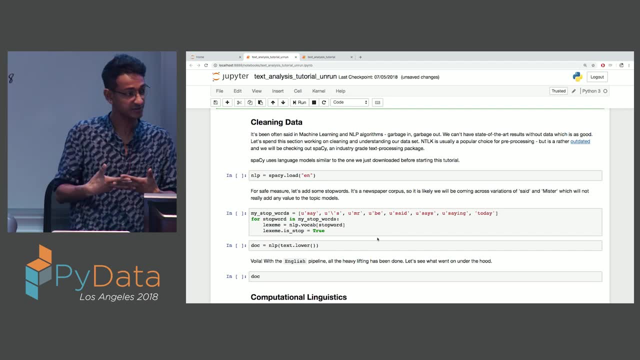 comes to data analysis. but garbage in, garbage out- if you're gonna have rubbish data, you're probably gonna get rubbish results. but again, what's important to know is that rubbish or garbage is very, very contextual. what is useful for one person might not be for the other. for example, numbers in data, in textual data. 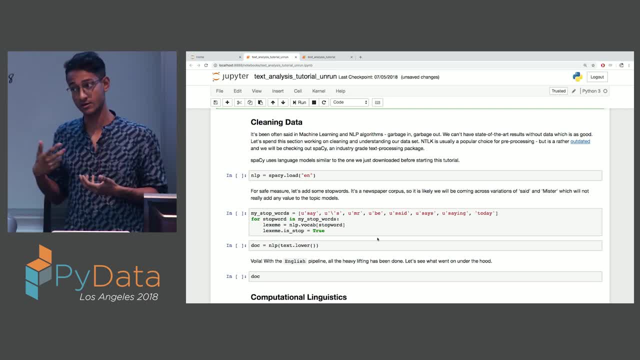 sometimes you might want to know what kind of numbers are coming up in our text. sometimes you don't, so sometimes you keep in our numbers, sometimes we don't. sometimes you want to keep in places. you don't really like verbs on Tuesdays, so that day I'm just not going to use verbs, right? so basically there's. 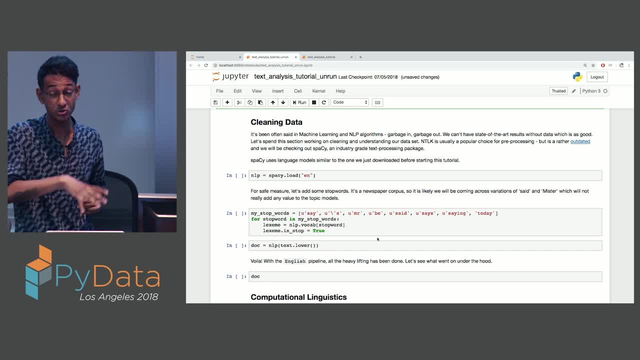 a lot of different ways you can clean your data and I'm not going to go into too much detail about that, but I'm just going to- and this is a huge part of textual analysis, and I often say that this is the most important part of the tutorial- the cleaning data part. after this, it's you. 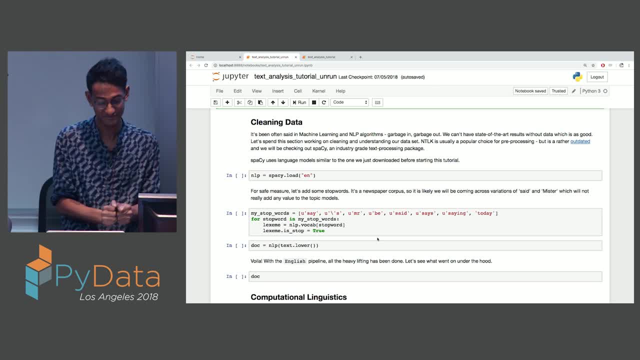 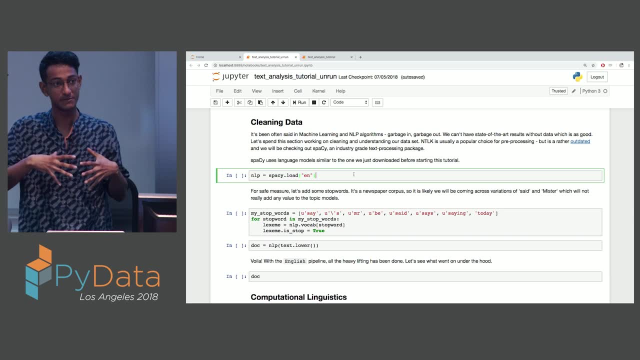 could read the code but like after this, it's not. as. this is very, very important, is my point, and we will be using spaCy to do all of this. now, the way spaCy works- and this is very important as we go on- spaCy has what you call language: 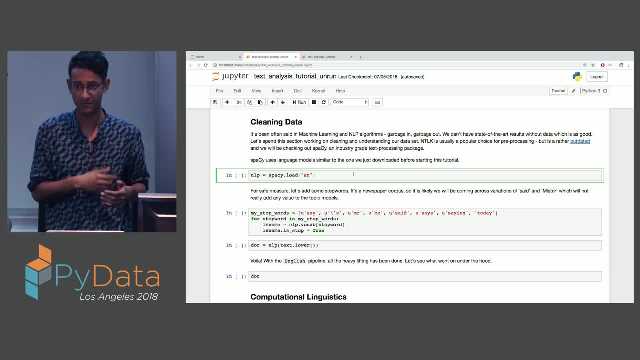 models which, based on your language. here we'll all be using English for the purposes of this tutorial, but you also have language models based on your language. here we'll all be using English for the purposes of this tutorial, but you also have Spanish, German, Italian, French as pretty well trained models available by spaCy. 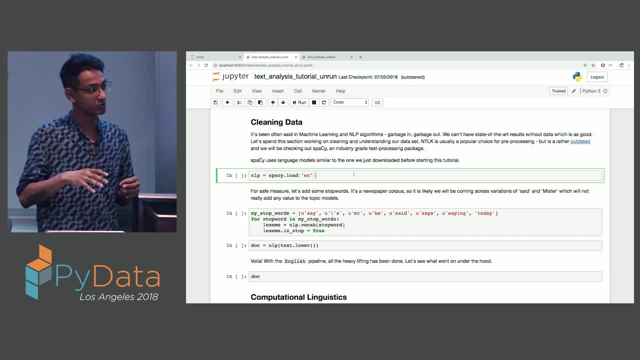 but the most popular ones are in English. now, what these language models are are statistically learned machine learning models which know what kind of words or verbs in certain contexts, which knows what kind of words or nouns, which knows what kind of words or numbers, and so on and so forth. so spaCy's language. 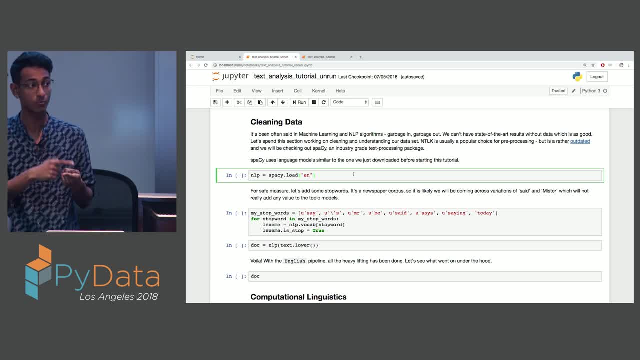 models knows what certain are stop words. stop words are certain words that you use which we believe don't have information. basically, spaCy has pre-trained models with a lot of rich linguistic information. this is very, very useful when we're cleaning our text, which are going to be seeing right now. 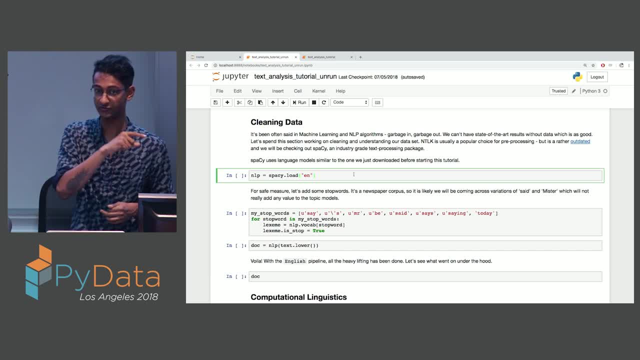 the way you load a language model after you download it, which are the instructions I've given you on the github page. after you download your language model, you would load it by with this line of code. it says: NLP is equal to spaCy dot. load en. en. here is English. for Spanish it would be es, I believe, and 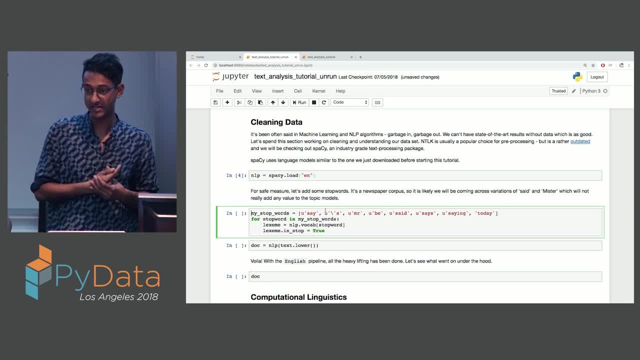 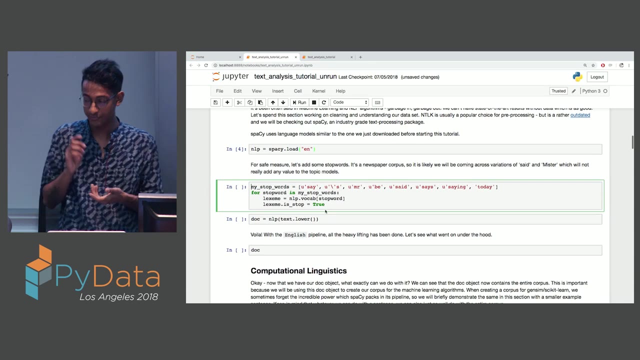 once we will. now that NLP, that variable is now our pipeline object, which basically, when we can now pass up, like pass text through this pipeline and start annotating our text and doing cool things with it. now I previously mentioned I said the word stop words, but I did not really go into it. I'm gonna 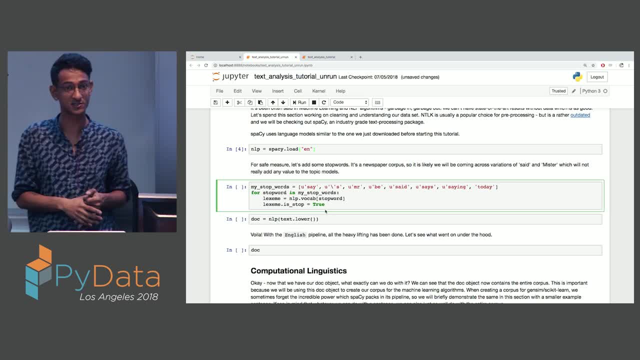 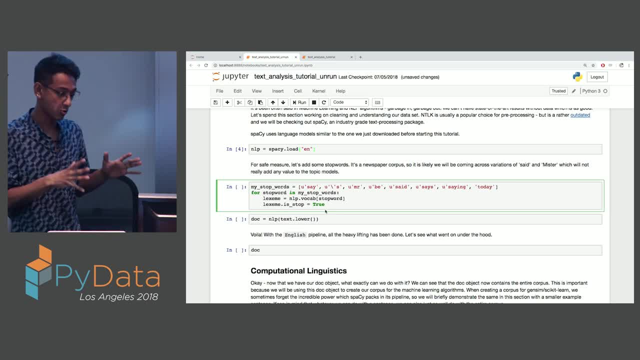 an example of this is, for example, if we want to figure out what kind of topics are coming up in newspapers, which is what we're going to be seeing in a bit as well, the word I or said or me or has the certain words don't add much. 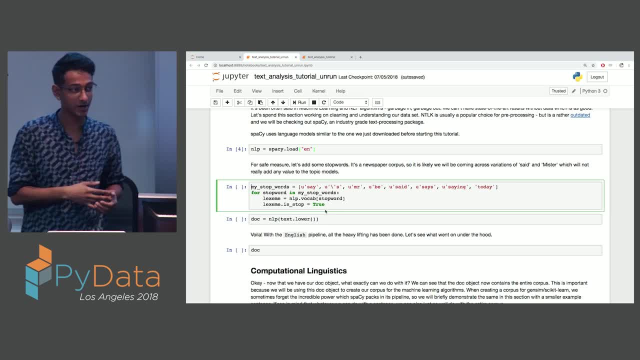 information. for example, if you want to know what the topics are, we don't want, like we don't want- a nouns topic- or you know what to do with in in general, with pronouns or something we'd rather have sports or politics, or something which has which gives us more information, so stop. 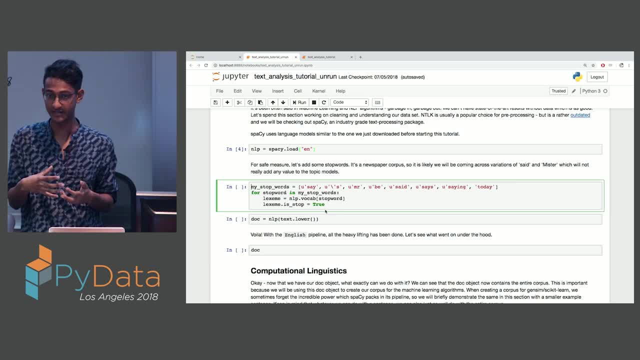 words or words which do not provide this particular information in text analysis, and we want to get rid of these words when we're generating our corpus, which we later play with. a corpus is the textual data set we will be using. so, in this context, I've already done this experiment once before and what I found 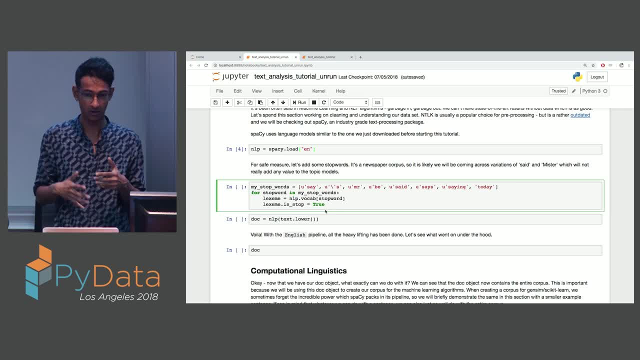 out is that the word say or saying or for the word say comes up in newspapers a lot. this is not going to be useful information in a topic if I don't know what is being talked about in between 2000 and 2001 and I just get say, said, mr, being I'm like, that's not useful. so I know this. 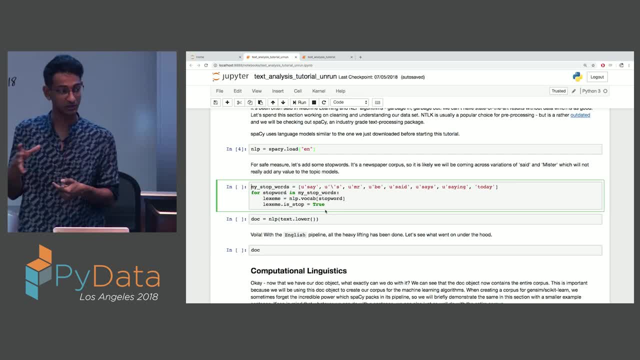 having done the experiment once, and these words are not traditionally stop words, so I'm adding these words to my stop word list in these four lines of code over here now. spacey already comes with its inbuilt a list of suggested stop words, but usually based on the context of your problem. 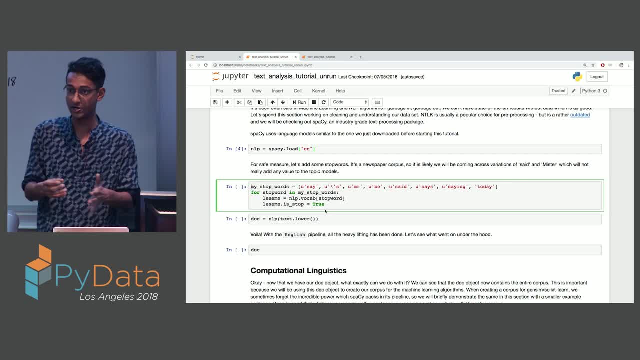 if you're dealing with biomedical data, for example, and you think one word- a protein or what I mean- probably useful, but in the context of your experiment is not useful, you would want to add that word as not useful or to my stop words list before starting. I've included that. 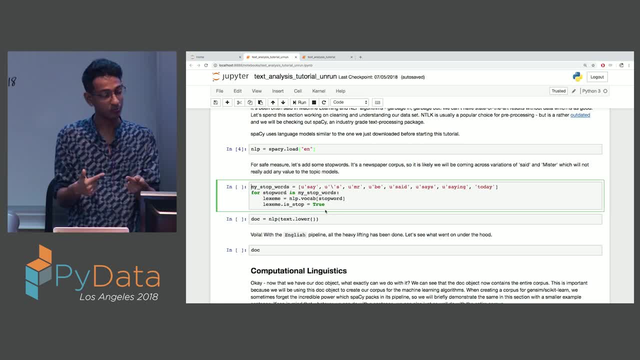 here, because later it would, just because it saves time. but normally how you figure out what's not useful is you do the whole experiment and you look at it like, oh, that's not useful. and then you come back up and then you line: you add this bit of code before you start, then you 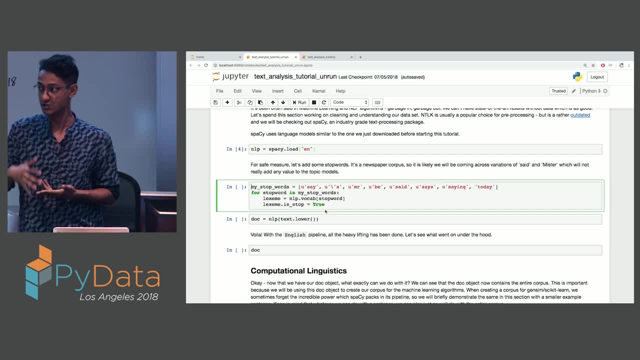 start again. but a huge part of textual analysis is this: you never get. what do you want the very first time? you kind of want to do things a whole bunch of times. I know that in the context of newspapers these are not useful words, so I do this. what is going on here is for each particular 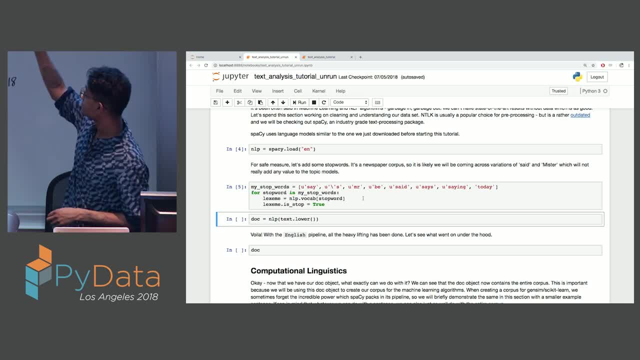 stop word in my list of stop words. I'm using the pipeline and saying the vocabulary of stop words in that pipeline. make that true. so over here, this is actually standard spacey code. this is how spacey does. uh here a lexeme is a linguistic unit and each word 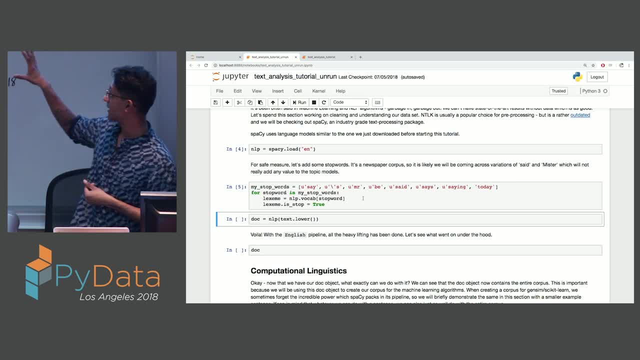 is. it's just the words which they use over here, but, as you can see, we're basically getting the lexeme which from the word and then just saying: is stop, true, yeah, it is a stop word. so this is just a small before we actually get started with um, what's going to happen? what stop words are is: 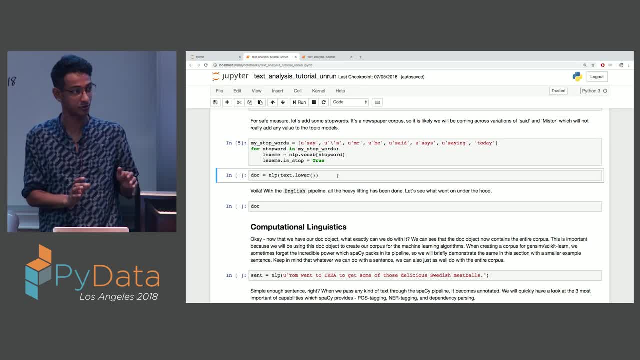 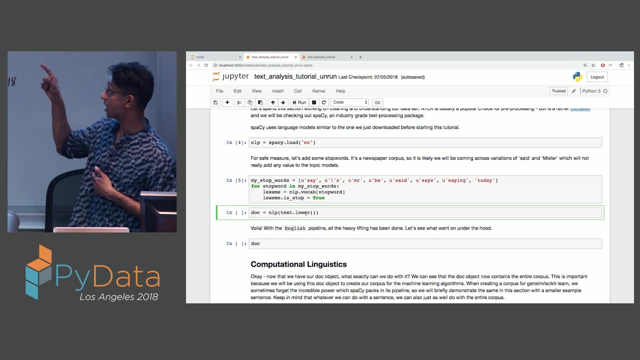 it clear what stop words are. any questions about stop words or why they're important? no, okay, cool. so now this is very important. um, our sixth line of code I'm doing, doc, is equal to nlp of text dot lower. so nlp, if you'd remember, with just two uh, Jupiter cells up is spacey dot loader contains my English. 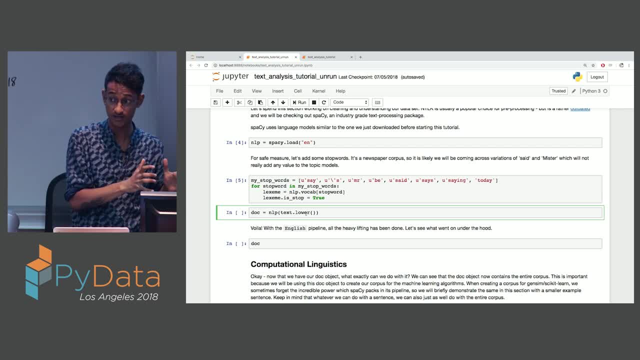 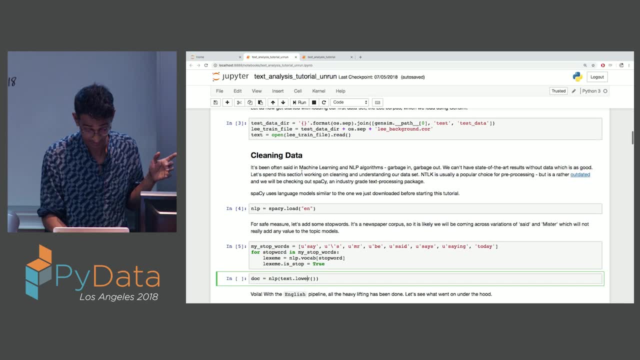 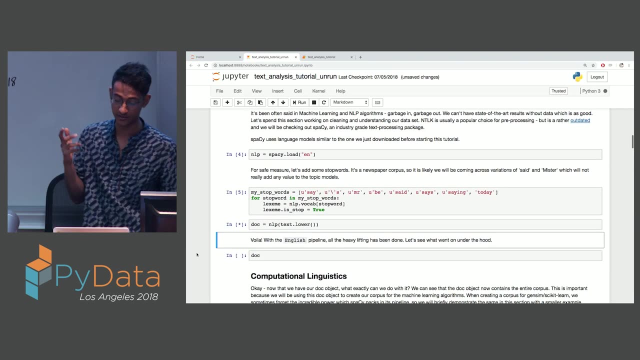 pipeline. I am now passing my document through the spacey pipeline again. what is my document? just remind you all. uh, in the context of this, it's my text which I've opened, which is the newspaper articles. so when I run this over here, which is going to take a small time but not too long, it's basically annotating. 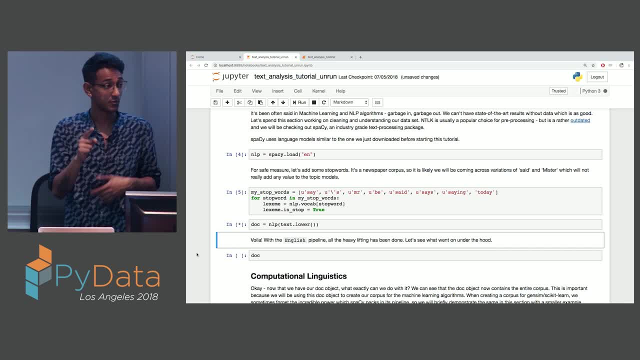 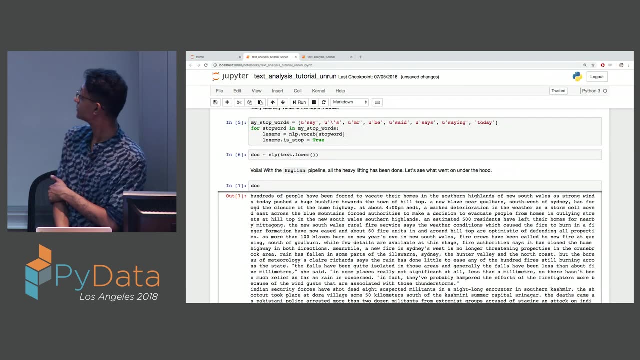 every single word in my corpus, which is all those newspaper articles. so it's going to know in all the newspaper Australian newspaper articles, the details of every single word in it which you're going to see very briefly here. so I'm going to show you what doc is so you can see it says it's: 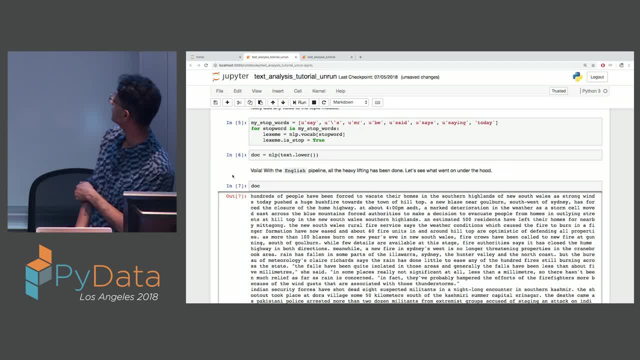 just text. it just looks like text right now, but hundreds of people have been forced to look at their homes in the southern Highlands of New South Wales. a strong wind, so it's like a fire, and they're talking about this fire in New South Wales in the. 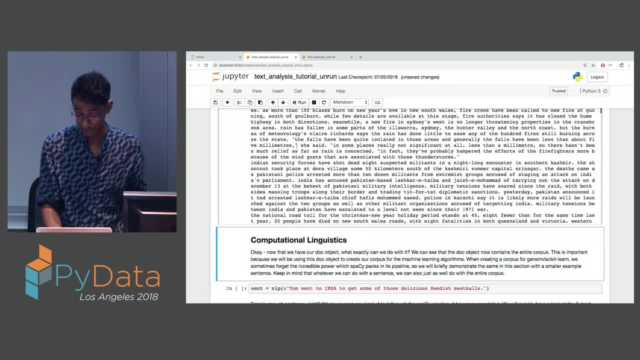 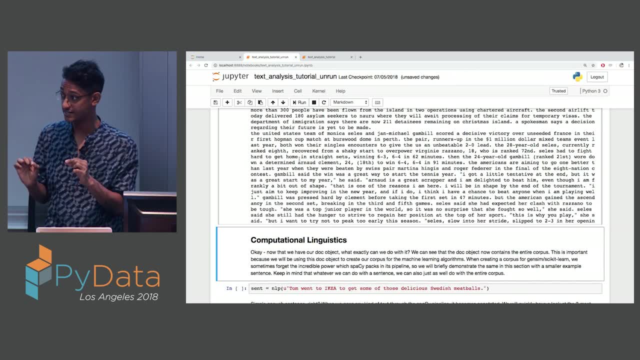 year 2000 and uh. so there's a lot of different articles and now all of these which you cannot see right now, but I'm going to show you really soon. all of this has been annotated by spacey, so now the doc object has contains information of every single words. is it a stop word, is it? 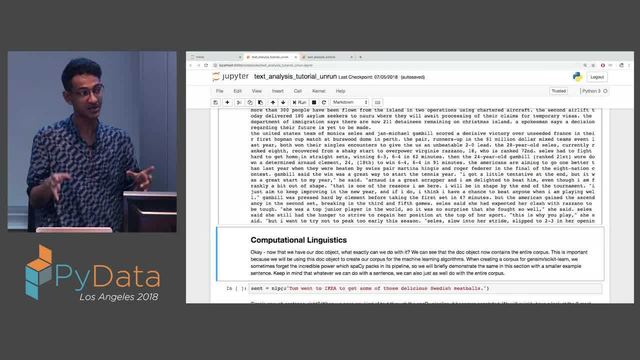 a number, what's its part of speech? a whole lot of information. this information starts becoming very useful a little later, especially when you're cleaning text. but in general it's just useful to know when you're doing any kind of textual analysis you're going to see exactly how briefly 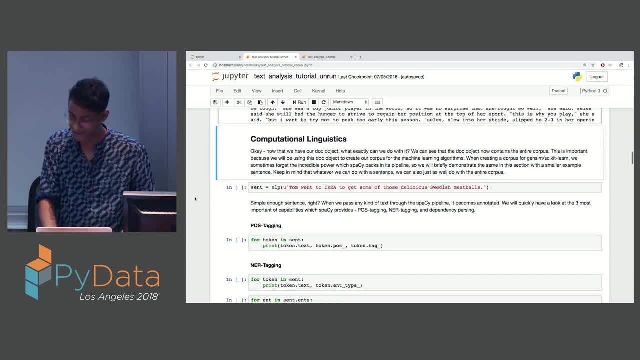 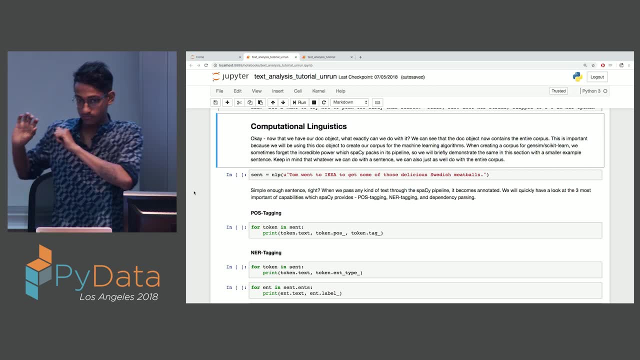 but this is what you need to know right now. again, is everyone clear what we're doing or why we're doing what we're doing? yeah, cool. so now I want all of you to remember that, but temporarily we're going to go out of context to show you what exactly computational linguistics is. so when I did that, 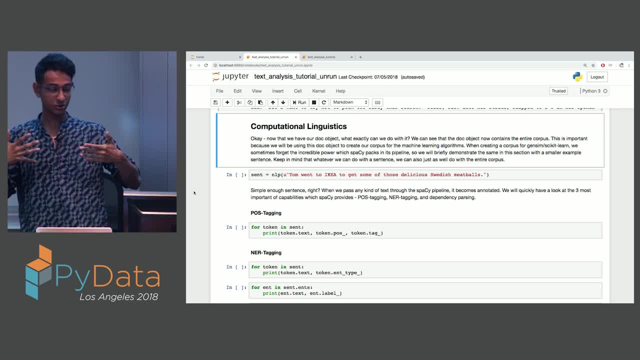 NLP of something. it annotated everything. now I don't want to show you all examples based on that massive text. I'm going to annotate one sentence and give examples based on this: uh, this particular uh subfield of text analysis is called computational linguistics, which is kind of 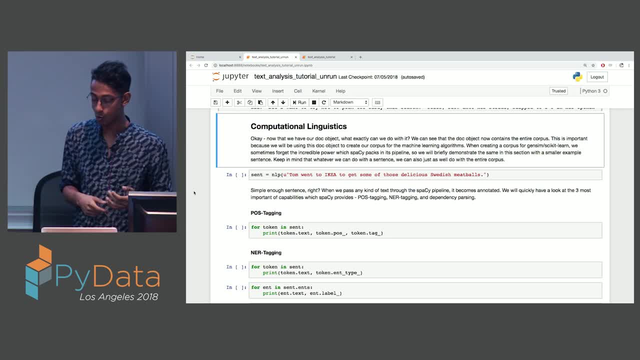 separate from natural language processing in the sense that you're dealing more with linguistics or structures of sentences and language. right, so we're not going to. we're going to now run the sentence to the same pipeline. we ran entire corpus. the sentence is: oh, it's Tom and Tarkia to. 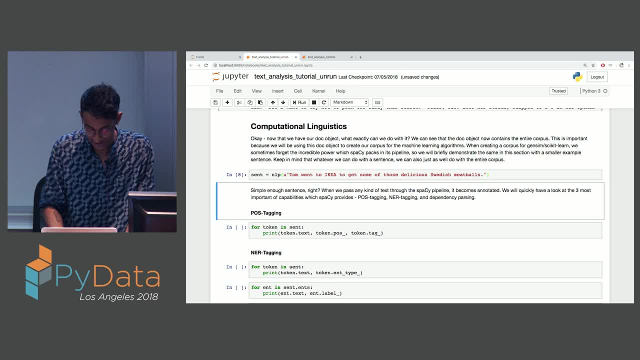 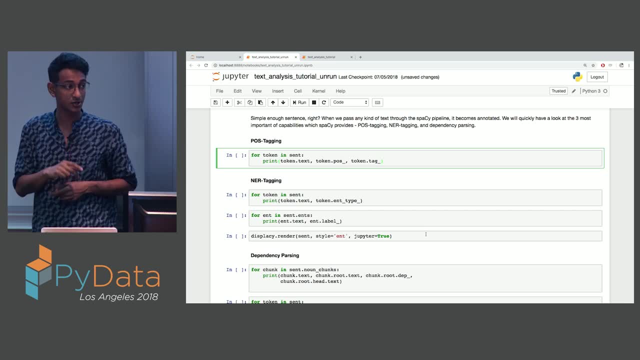 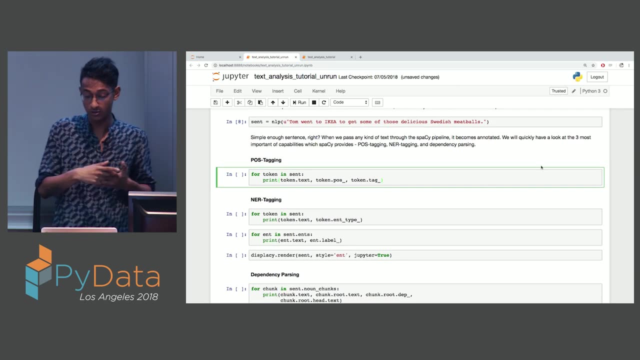 get some of those delicious Swedish meatballs. and now I'm going to go over some basic things you can do with spaCy. so the first is part of speech tagging, or pause tagging. uh, what we're going to do is we're going to now show you what parts of speech are here. so, uh, for token, in scent uh. 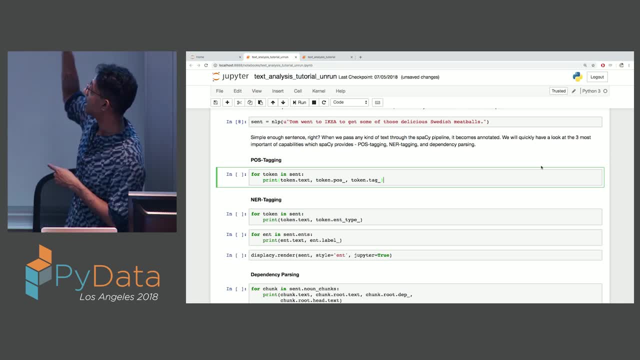 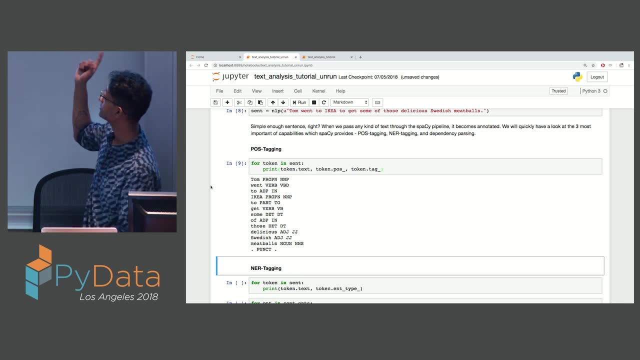 again for context. sent is basically that particular sentence after it's gone through the English language pipeline, right. so I'm running this over here and it very, very quickly. it shows me Tom is a proper noun. went as a verb to Ikea- proper noun- to get some of those delicious as an 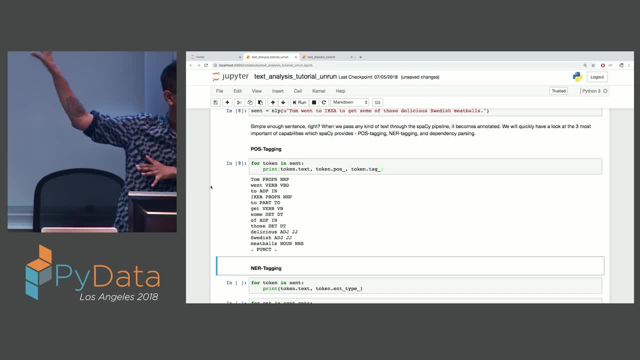 adjective, Swedish adjective. so you see what's going on here. spaCy now knows what every all the information in that sentence and gives us to you. spaCy also told you gave you all this information about that massive document before right. this is just for this particular sentence, so you can go. 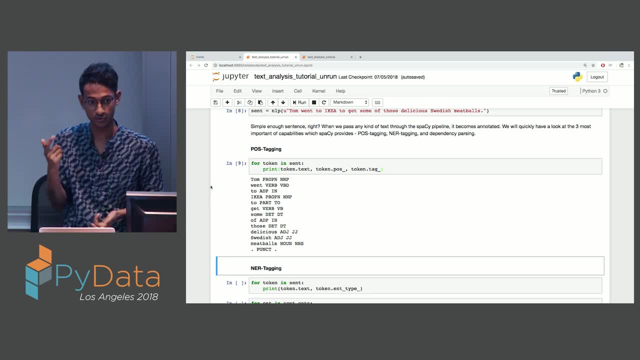 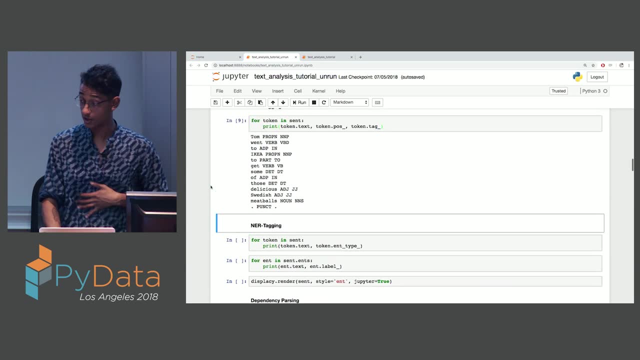 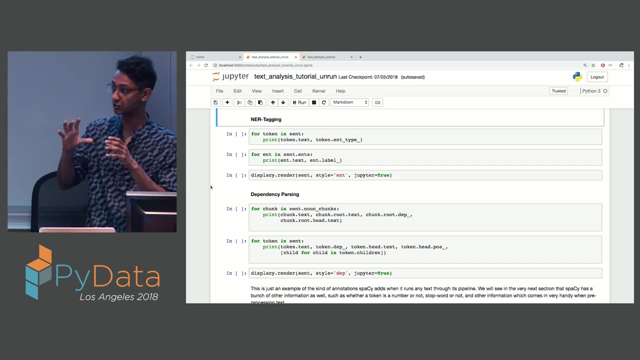 for every single token. here is a single individual linguistic unit of a sentence and gives you information. this is part of speech tagging. there's other things you can do, for example, ner tagging. ner stands for named entity recognition, which, as it suggests it, looks for specific named entities in our sentence. uh over. 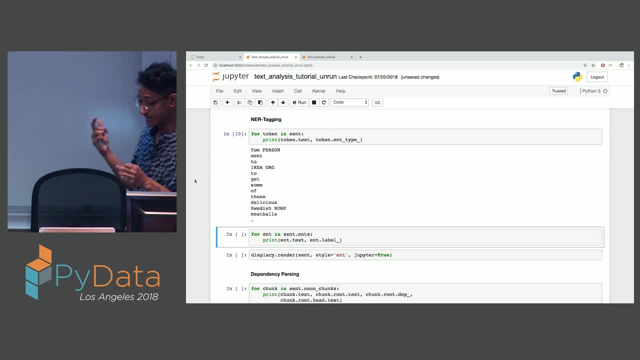 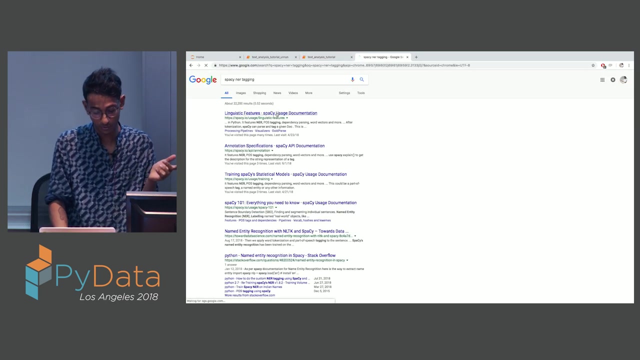 here there's only three named entities. one is Tom, who's a person, it's Ikea, which is an organization, and you have Swedish, which over here is. so, based on the context, this comes up differently. you can have political, organization, country place, so spaCy has um you have. you can go to linguistic features and look at what exactly. so over here, 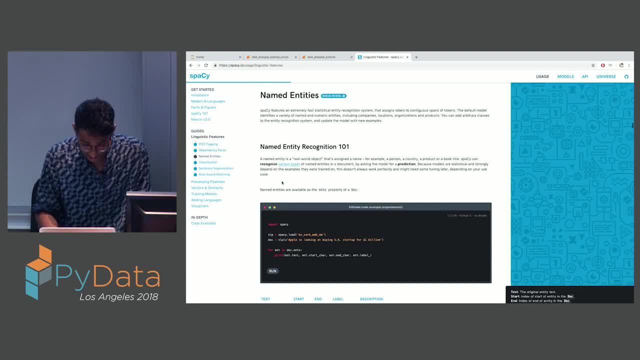 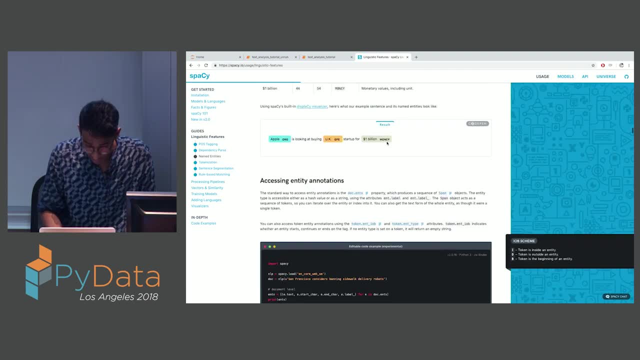 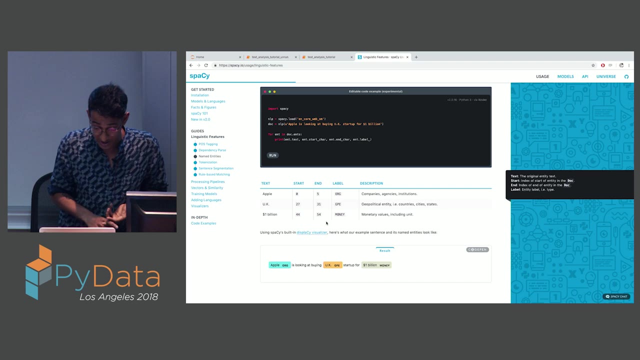 if you look at uh spaCy in terms of its named entity recognition, it has geopolitical unit, which is GPE, so you have a lot of different kinds of um labels, like organizations, uh. then you have money as well. you have a lot of different things you can do with named entities, uh. I would recommend searching it up based on. 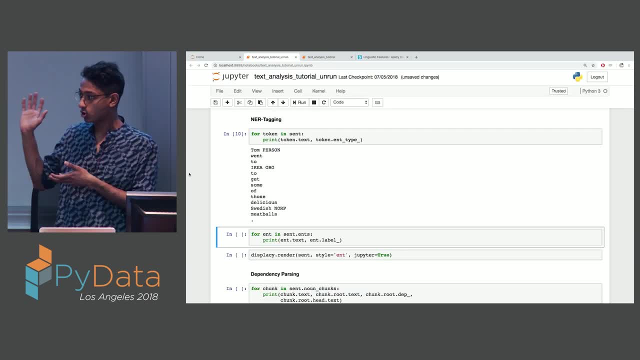 what kind of named entity you would like to look for, but the common ones are person, time place and so on. uh, you can also here. I went over every token in sentence and I printed the entity for every token. some of them don't even have them like went into. so if you want to skip all of that, 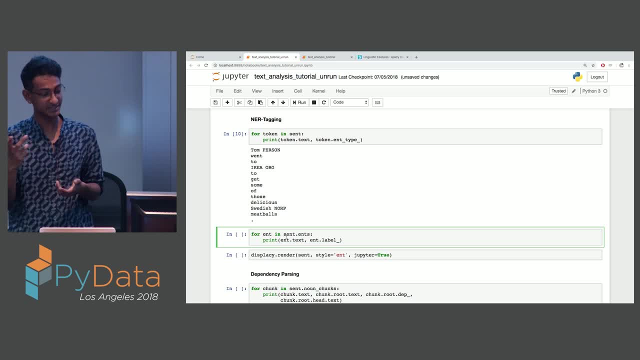 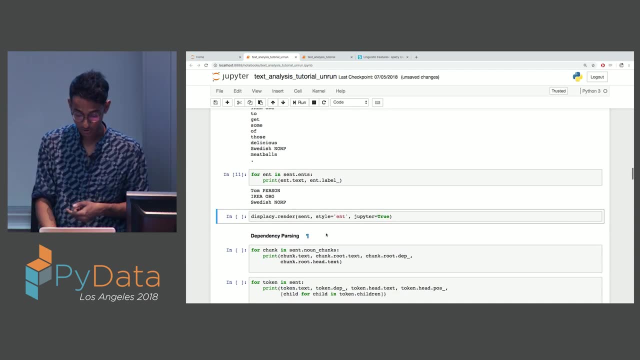 and just go through entities you can do for end here, and this entity in sentence dot, and, and you can look up the only the three entities which are here. you can also have it. spaCy has this really neat plug-in called display C which allows you to like visualize this in a pretty way. so over here. 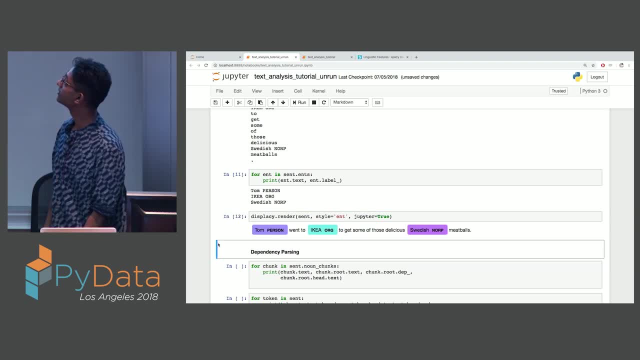 you just have this neat little purple thing over it. so, as you can see, spaCy does a lot of cool stuff. part of speech. tagging is usually very useful in general text and I'll talk about that in a little bit analysis. finding out entities like this- also pretty useful based on your problem. 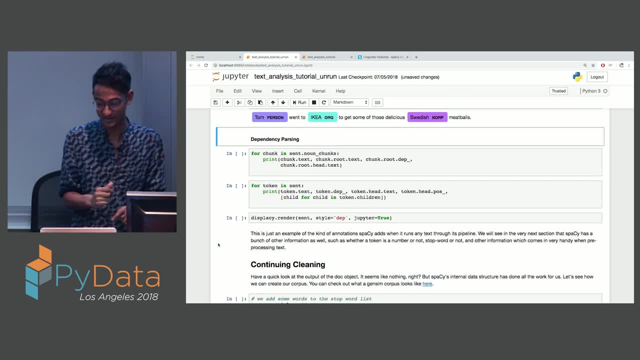 um, and again I'd like to make it clear, like spaCy did this for that massive document too, right, not just for the sentence. um, now I'm going to show you what dependency parsing is, which is the idea that, uh, in in a sentence, things are linked to each other in a certain way, like Tom went to Swedish, so 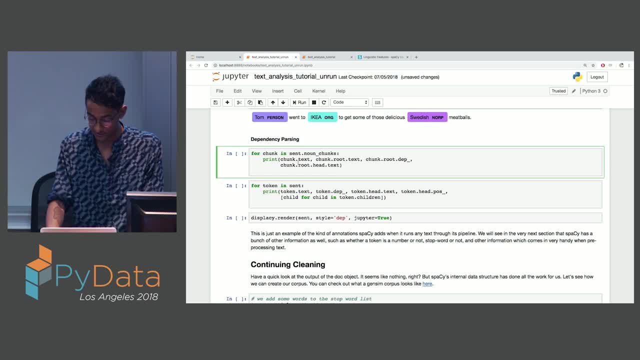 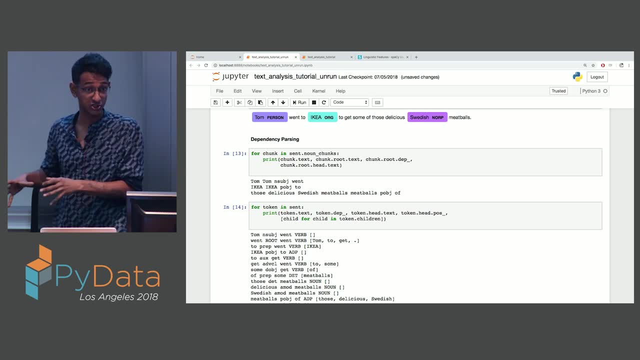 it's like Tom went is the verb, so things going on right. so to find out these dependencies. I'm not going to get into the details of what these dependencies mean, because that's honestly a lecture on its own, like dependency parsing, and parsing of textual data is a massive subfield of research. I just want to let you all. 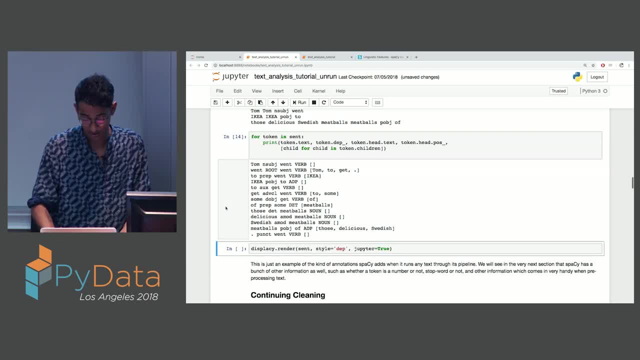 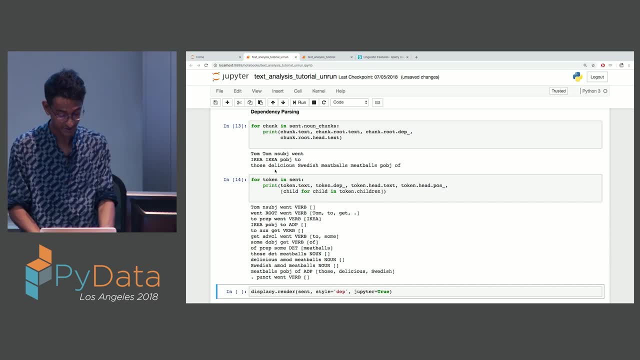 know this exists and spaCy does this for you. uh, an easy. so this basically shows you the structure again. if you're more interested in dependency parsing, I would recommend searching up how spaCy does it. but to give you an idea of the kind of information, it's basically this, so it's like here: 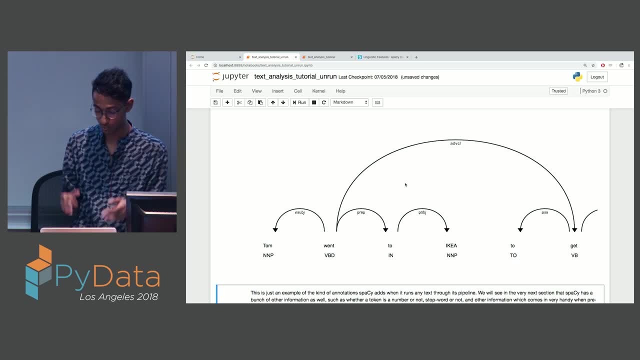 the root of those sentences, normally the verb for spaCy. so you have went being. it links. you know, Tom, and so you can see that this is what spaCy does. it gives preposition, then subject, object. it basically tells you how a sentence sentence is structured right. you can get all this kind of information using display C and. 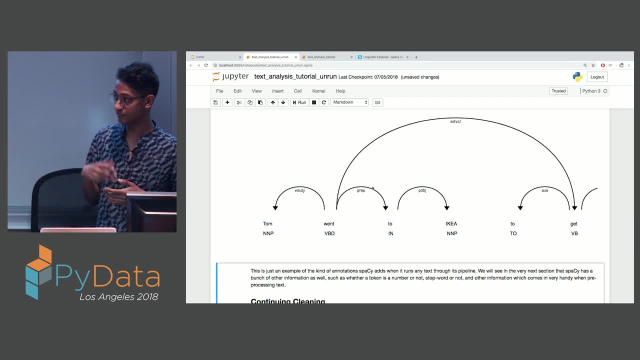 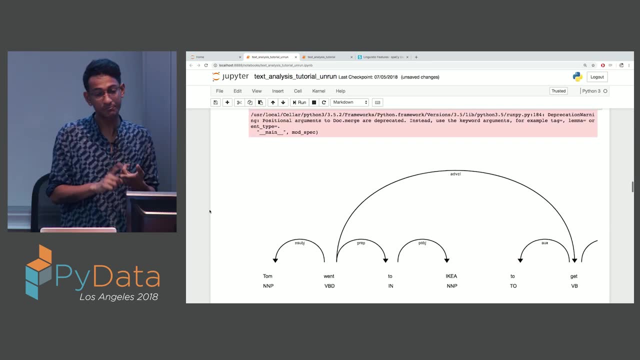 spaCy um. and this is done sentence by sentence, for every single sentence, which is why that took a little bit of time before when we were analyzing our doc. so any art post tagging, any art tagging and dependency parsing tend to be three of the most important computational 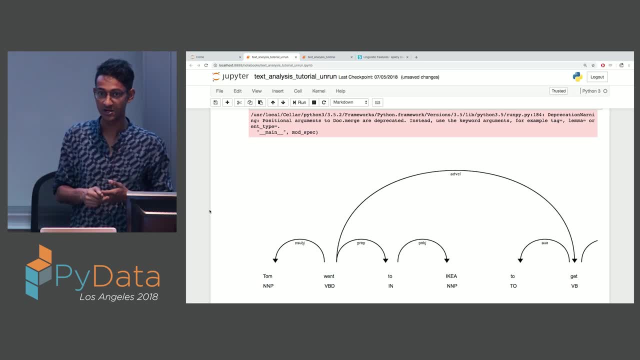 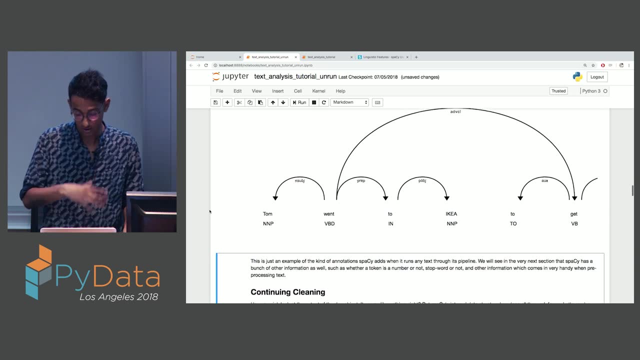 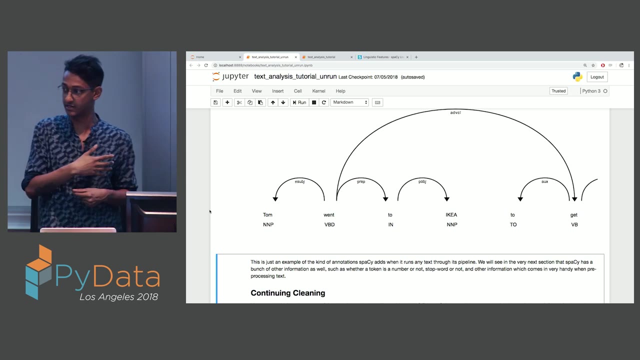 linguistic ideas which are normally talked about or discussed. so is everyone here clear with what these three are, more or less? yeah, awesome, so you can. I would really recommend getting into you also have this for Spanish, uh, French, German as well. and spaCy is open source, of course, and is always. 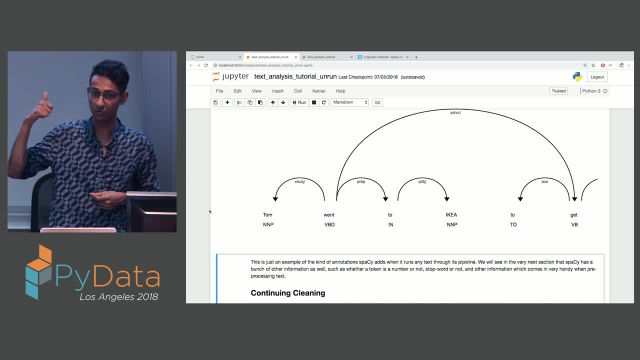 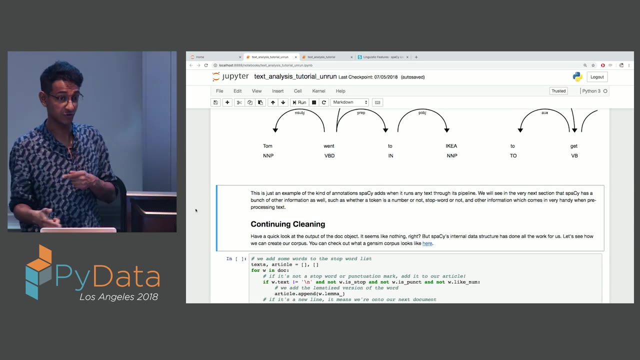 updating its models, uh, to make them better. they're all neural networks under the hood. by the way, for those who are interested, it's a, it's a deep learning Network which is trained to find out, uh, what exactly you would tag something on, as you can also train your own taggers. so if you want to, 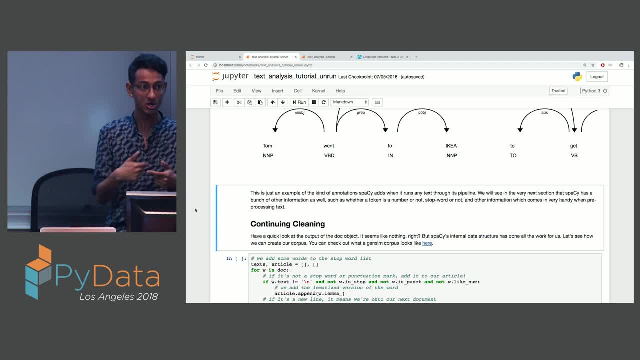 have like your own particular label or you know part of speech or whatever you can per. you can train spaCy's models with your own data, so there's a lot of really cool things you can do over here in the computational linguistics part of spaCy. 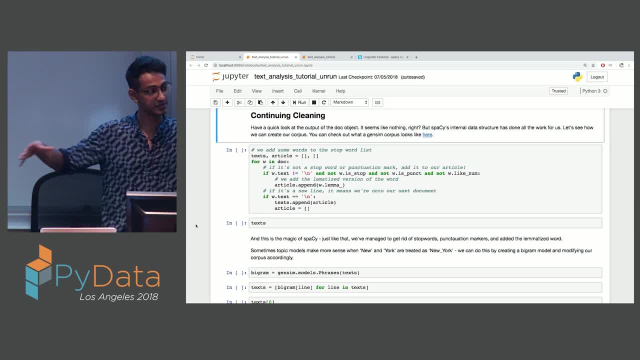 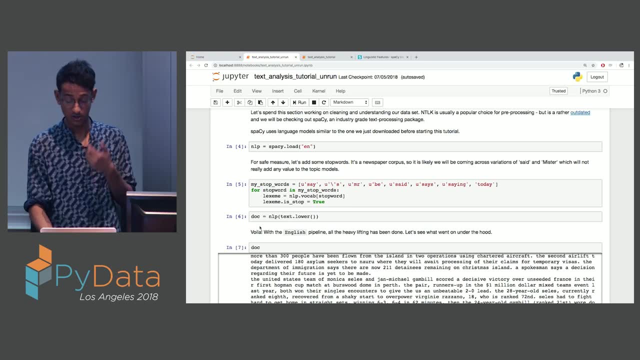 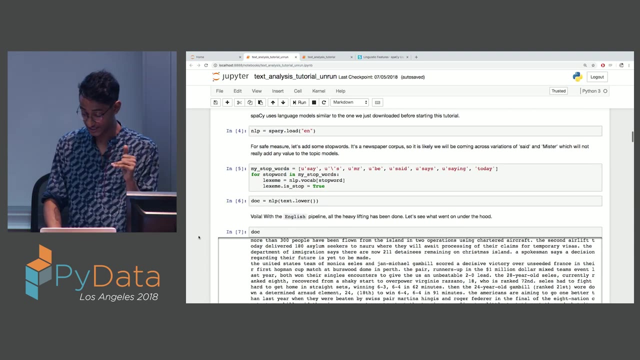 now we're gonna. so that was a small detour just to let you all know what spaCy can do. if you remember, the last thing which we had done before we took our detour is this doc? uh object which basically has all the uh Australian newspaper articles right. so now let's go back to cleaning. 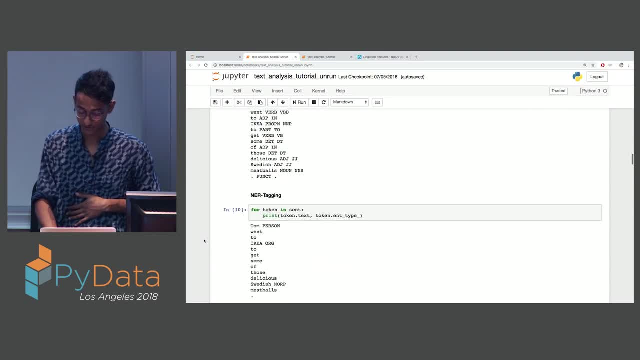 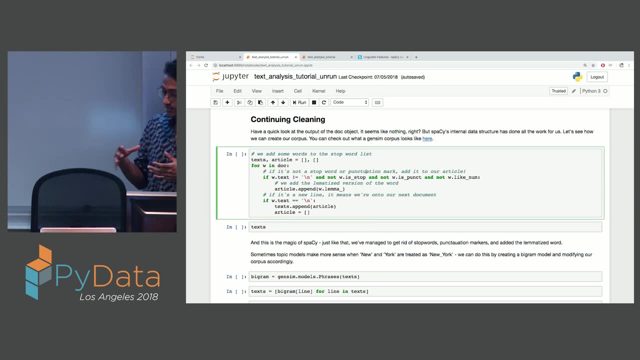 this because there's still some kind of information which might not be useful to us. so now, this is very important when the in the context of um. so what we did before this was computational linguistics. now we're slowly moving out of that realm into, uh, the machine learning part of this, and in machine learning it means what's very 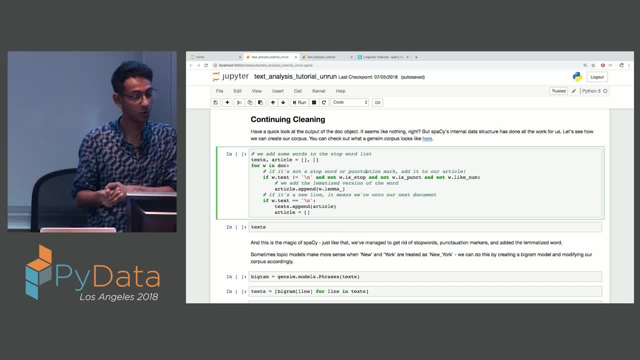 important is vectors. now, the reason why vectors are important is machines don't understand words, so we need to represent them as numbers, and numbers when there's a lot of them- and in text we have a lot of numbers because- so I'm going to take a again- a super small detour is this: 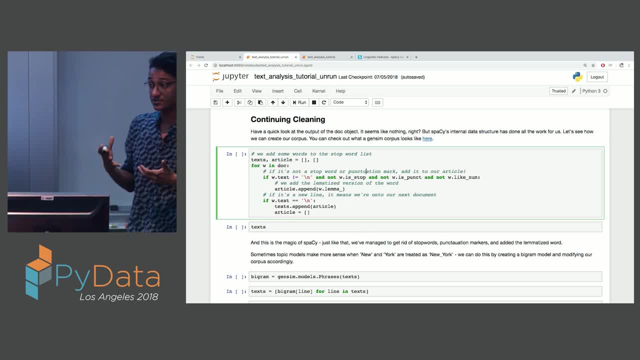 so I'm going to try and explain to you, uh, how machines understand text in terms of data structures. right, there are many ways. now let's assume that, uh, again this. these are hypothetical numbers, but they would be kind of close, maybe. uh, if you're going to look at a newspaper Corpus, I can actually just look at the. 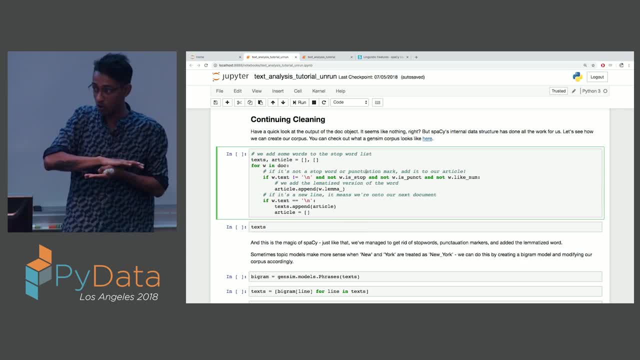 length of the dictionary in a bit, but let's talk about- let's assume that, this- all the newspaper articles which we have, the 300 newspaper articles. if you look at all the different kinds of unique words being used in them, let's just say there are 10 000 words, right? so, like all of the articles in 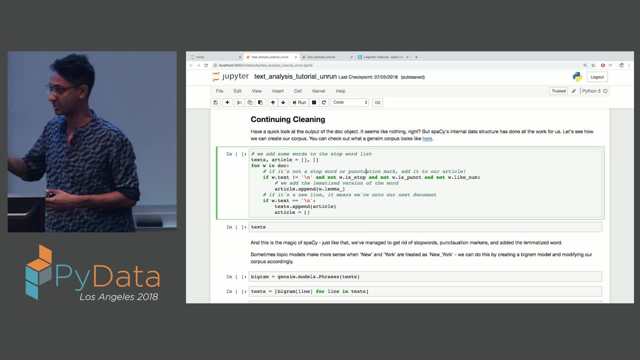 there are only made from this vocabulary of 10 000 words, but normally, of course, it's gonna be a lot more words. but in the context of every machine layer- I mean every text analysis project we do- there's always a vocabulary which is every unique word being used in your analysis. now how does a 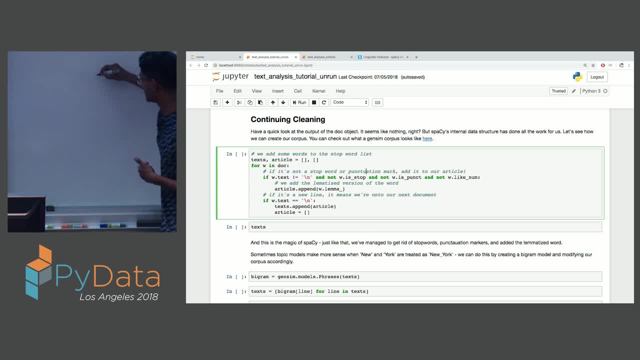 computer figure out what's in a document. it basically has this really, really massive like indexing of every single word. so if it's Tom, it would be like you know, index zero and then running up to index 10 000 in vocabulary for each word, right, and then if you have a document which 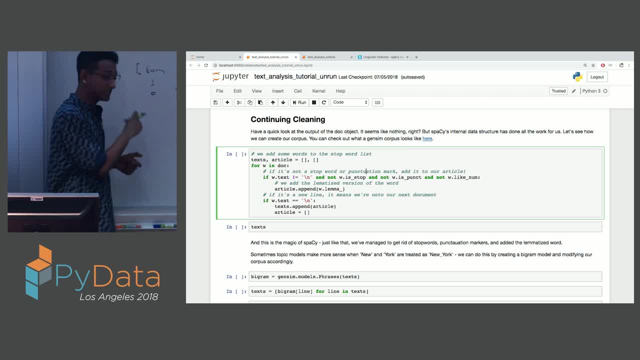 could be. even a sentence is a, it could be a document or whatever. it would basically have a zero or a one based on if that particular word exists in that document. so you'd represent a document and really each document, even if it has three words, would say nine thousand nine hundred. 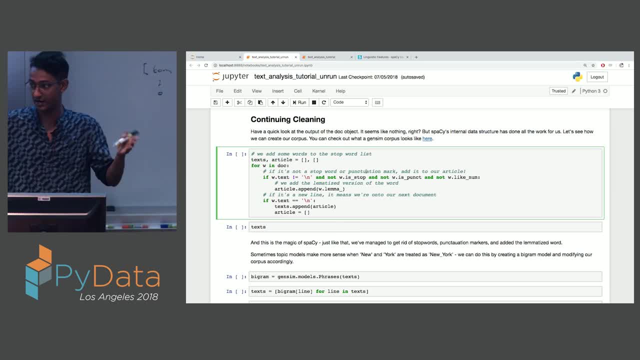 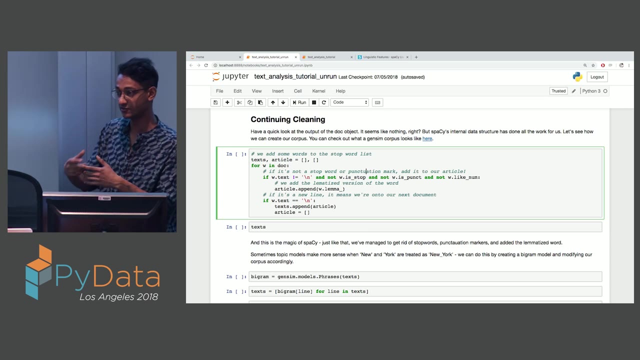 ninety seven zeros and three ones, but you're still using up all of that data, right? I mean, you're using up all that space. so this is why we have to be really careful in in the best possible way we can give information to our models, right? so I'm going to be now talking about how we create our lists, or lists- lists of 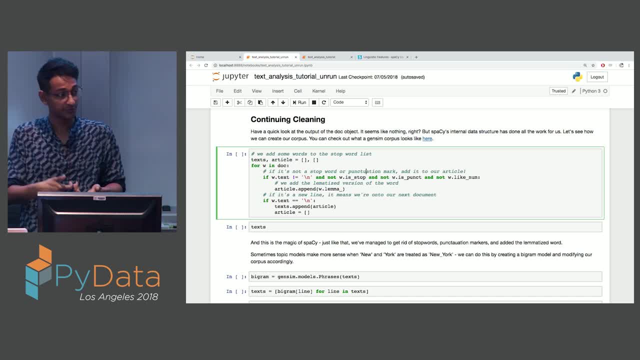 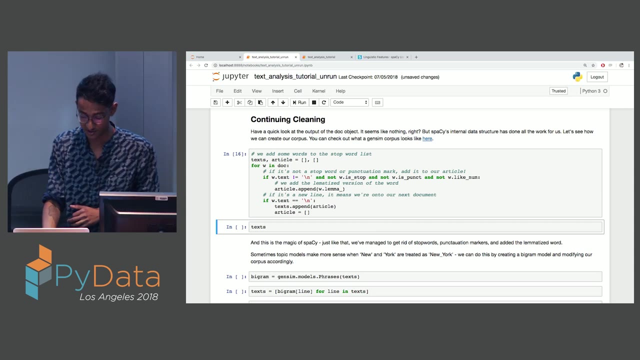 lists to demonstrate, to allow computers to actually use this textual data. now, if all this sounds a little complicated, it'll become a lot more clear once I run these. uh, I'm going to first just run this. oh, this is a super important uh cell, by the way. cell number: 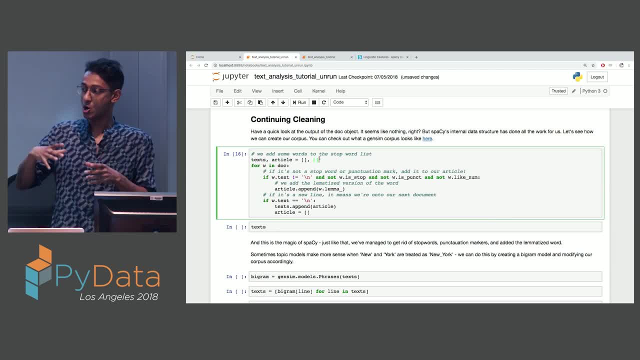 16 is very, very important because it's going to tell you how you're going to create your data structure, which is going to be your input for most machine learning algorithms. so this is the part. let's go through this really slowly. so first I create uh, two uh lists. one is called text, someone is called 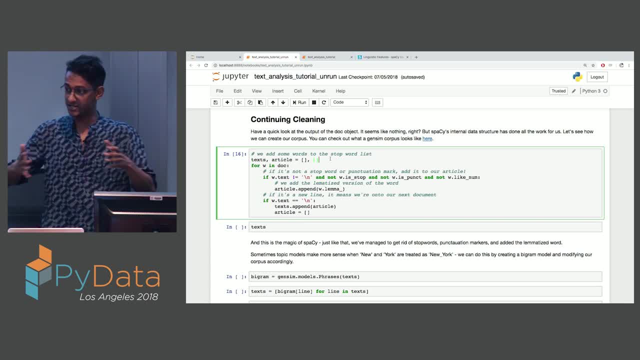 article, uh, text is basically going to be our entire data set or all our texts. an article is going to be each individual article. so for W in doc. uh, doc, again, I would like to remind you, was that massive document and W is every single word or token. so for W in doc if the text or if the contents of that word is not a new. 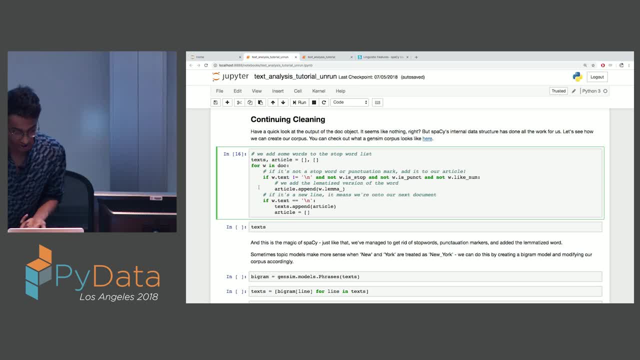 line is not a stop word, is not punctuation and is not a number. I'd like that particular word to be appended to my article. is that clear? that's basically this over here here what I'm hot. so the reason I'm doing this is because when I want to create, for example, which 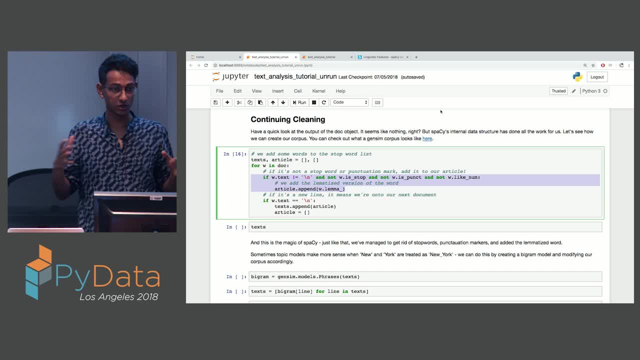 I'm going to show you in a small bit uh topic models or any kind of large statistical models. I don't want stop words. I know that I don't want a new line, because a new line in my data set represents a new article, so I want to keep it to one article, one article, if it's not a stop word. 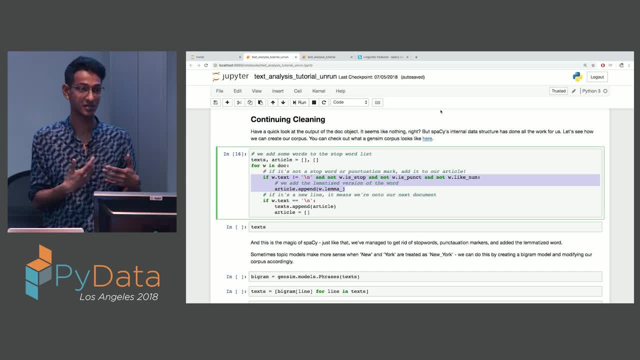 if it's not punctuation, like a full stop or a comma, is not going to give me a lot of information about this particular topic, right, uh? and if it's not a number, because in my context I don't want numbers- you all could totally keep numbers if you'd like. 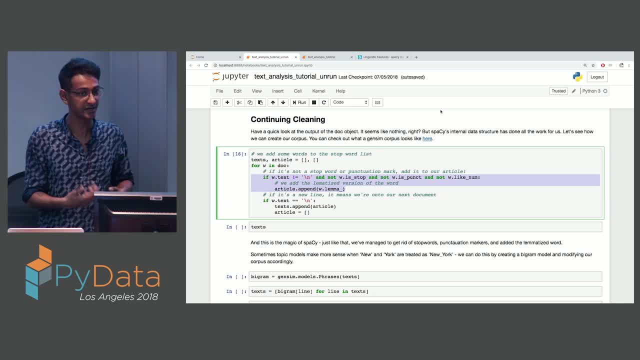 if I have, and you could add more rules. if you're trying to create a database of only- like I talked about before, like only verbs, you could search for verbs and only put in verbs. so what spacey does is spacey now allows you to have is punked like number or not, and, for example, if you want to, 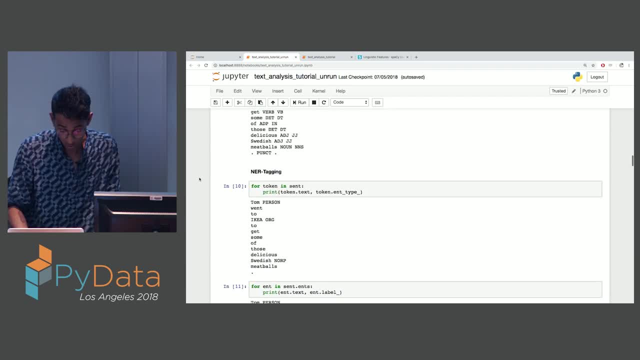 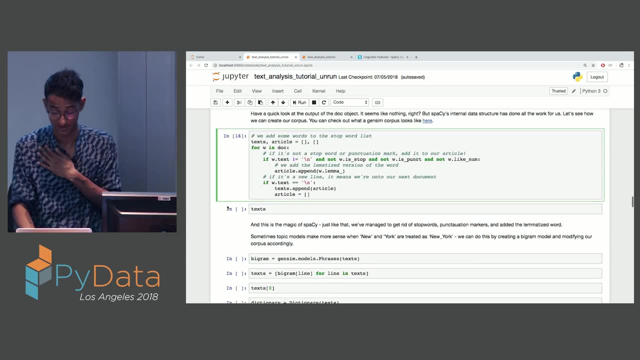 do find out what a verb is. I've talked about this briefly earlier- where it's token dot, POS, underscore, where you would have verb or part, so you can choose what you want to keep in your corpus. I've decided to keep everything which is not a stop. 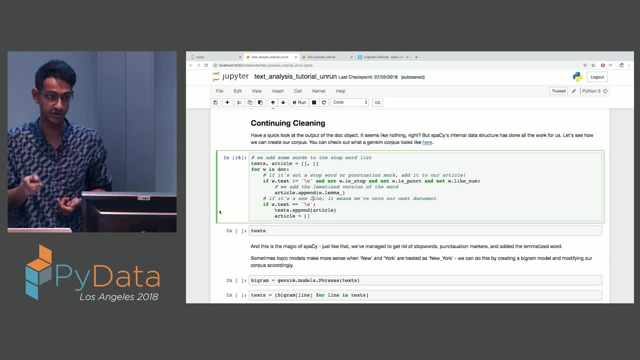 word, everything which is not a number, everything which is not punctuation or a new line as part of my corpus. and then after that, I've said: every time I do see a new line, I want to add that particular article to my text, right? so that's what's going on over here. to be clear, what now are things look like? 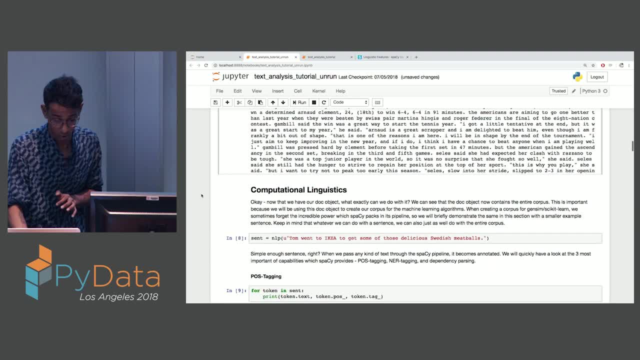 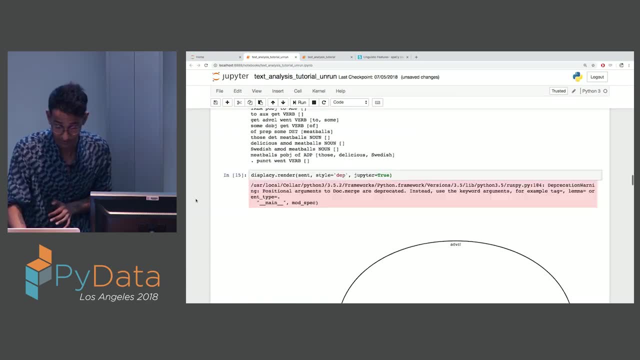 this is very important. what I've done is I've gone from this over here right, which is hundreds of people have been forced to locate their homes, blah, blah, blah, to over this where, instead of hundreds of people have been forced to locate, it's just 100 people forced. 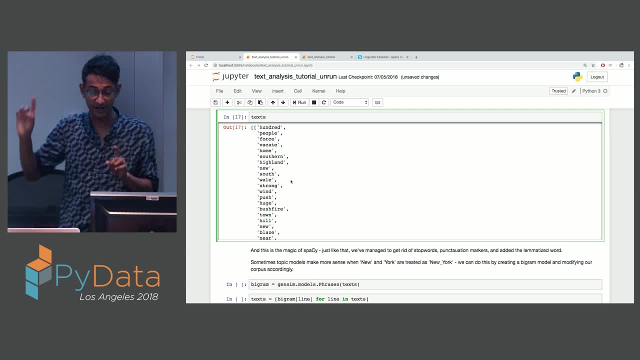 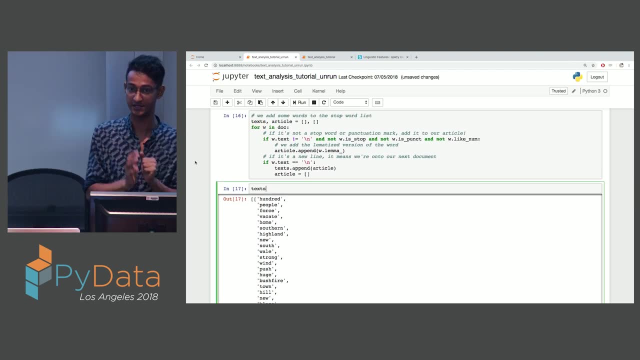 to locate home. can you see what's happening over here like? this is very important. cells 16 and 17 are very important because they talk about what cleaning textual data is. so remember what we've done before this. all the cells about this. you remember what I had, which is just like massive documents which have been annotated, and I've gone from that. 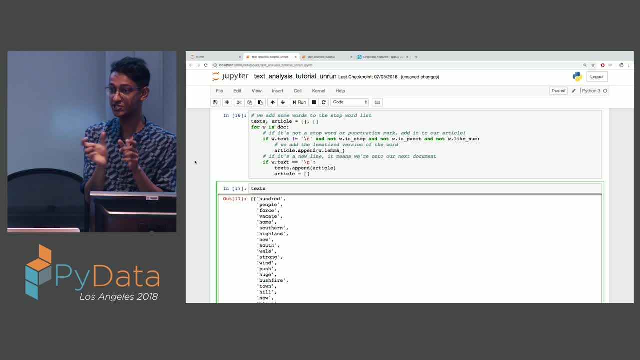 to this list of lists, where each sub, like each list within this list, is an article and each list contains all the words which I think are useful. so over here I got rid of like hundreds of hundreds of people. you're seriously seeing what's going on here, right? this is a very 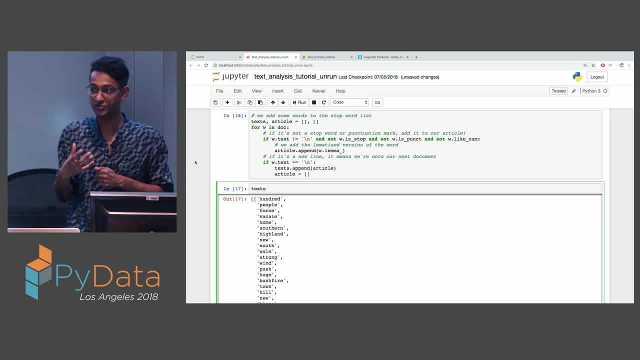 important part of text analysis and is how computers are going to get anything meaningful out of what you say. so is this like a ten thousand percent clear with everyone here? no hands up. cool, I'm going on because this is very important and the and the rest of the talk sort of builds on this, so it's. 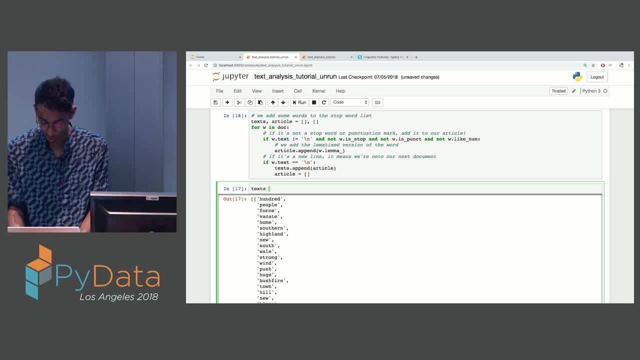 important that this is clear. so, just to make things even more clear, this would be only our first document, this would be only the 101st document and, if you'd want what is like, I don't even know if there's the seventh word in this document. which is important to us is custody must. 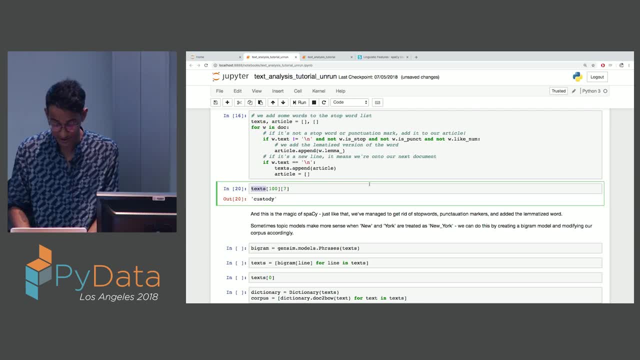 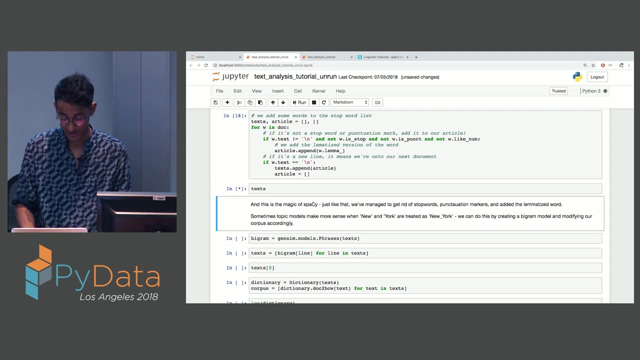 be someone's, so yeah. so this is to give you an idea of the kind of structure we have. what is the size of this data? sorry about that. so it's 299, which is 300. so this is just to give you an idea of the data set we are creating. right now. we're going to move on and I'm 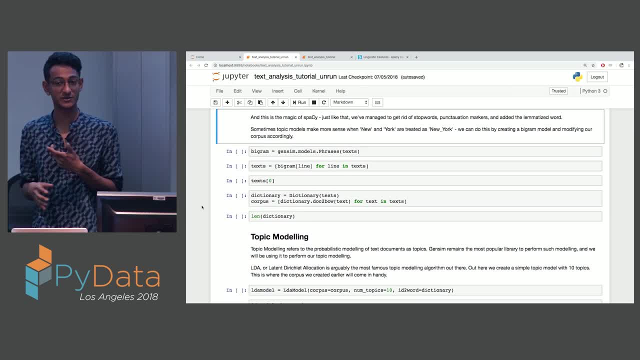 going to give you a little bit more information about the fancy kind of things we can do when we're cleaning up our documents. so we're going to introduce a topic called bigrams. bigrams or I mean n-grams. I'm going to be specifically talking about bigrams. n-grams are basically, you might. 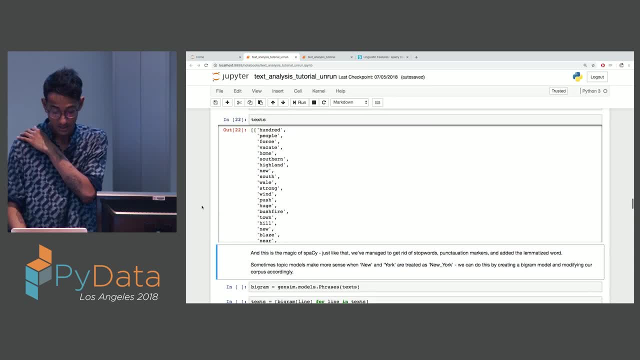 have noticed over earlier on when I looked at text right. just to give you an example like this is a really quick example. you can see New South Whale- right, these are three different words in my previous document. but a New South Wales, I believe, is a territory in southern Australia. and so now 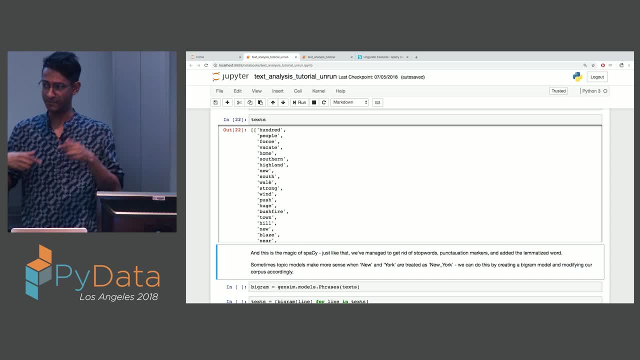 what's gonna? what's gonna happen over here is New South Wales is three separate words, but in our text analysis it kind of would make more sense if we were to look at it from a different perspective, because we would want to look at it from a different perspective. so in the Las Vegas region, 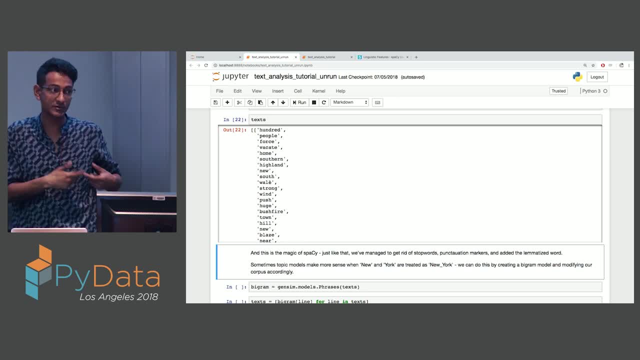 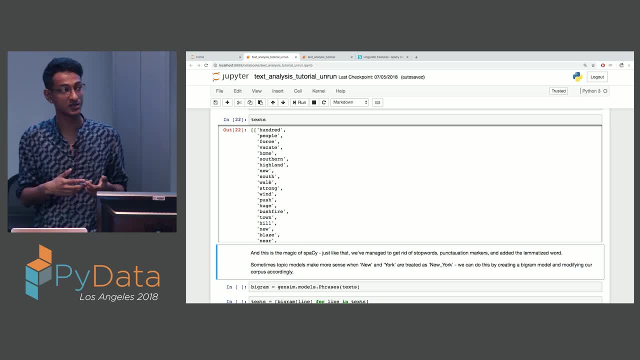 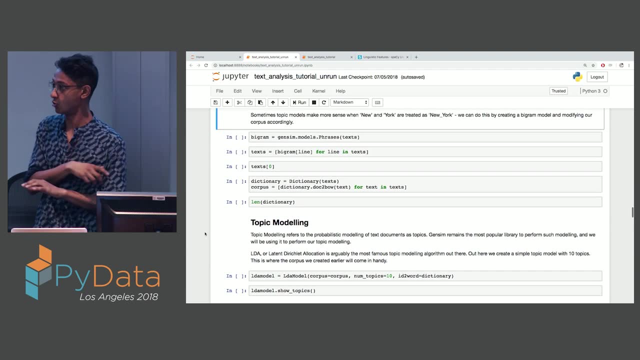 word right, because it means the same thing. if we see new york coming up again and again and again, we know it. we know that we'd want to rather deal with New York instead of new and York, and the same for Los Angeles and basically any place where two words appear around each other, so often they make 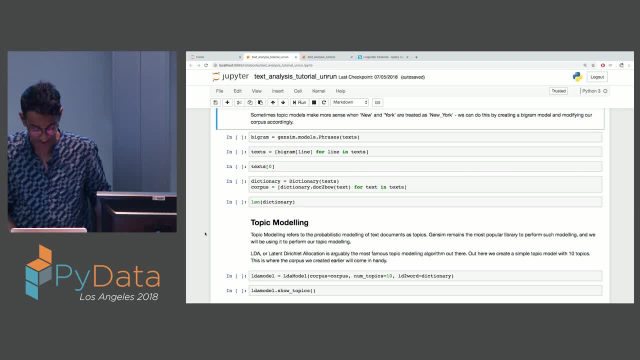 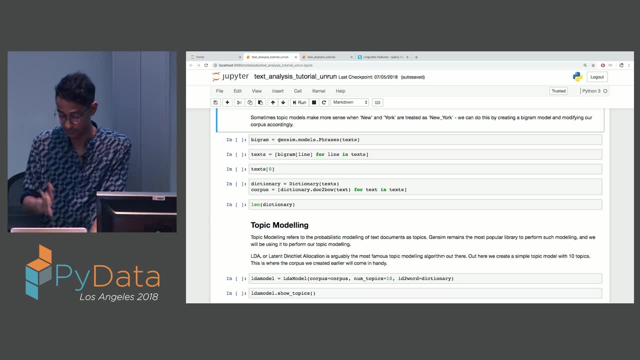 on your own. by the way, I'm these packages just makes things faster, right? so bigrams in the context of Jensen, which is the first machine learning package you'll be using, we're going to be loading it using Jensen dot models or phrases and texts, so we are basically passing all our text through this model. 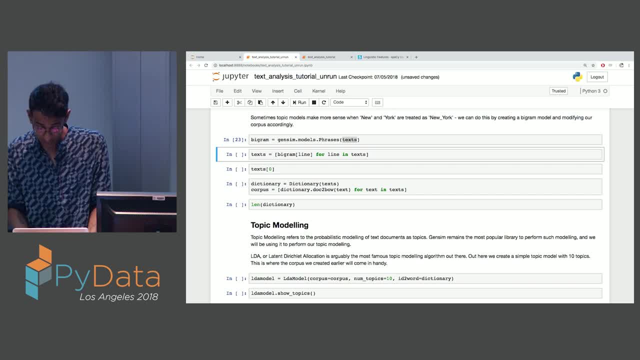 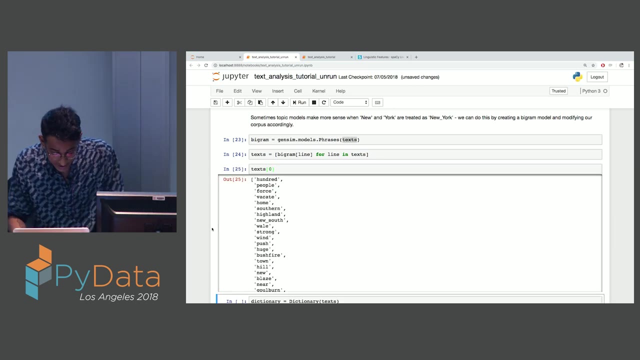 and I'm creating a bigram model. I'm gonna now do the bigram part. it's basically apply my bigram on line for every line in texts, right? so I'm. this is how I'm creating my text with bigrams. let's see what it looks like. you can see. 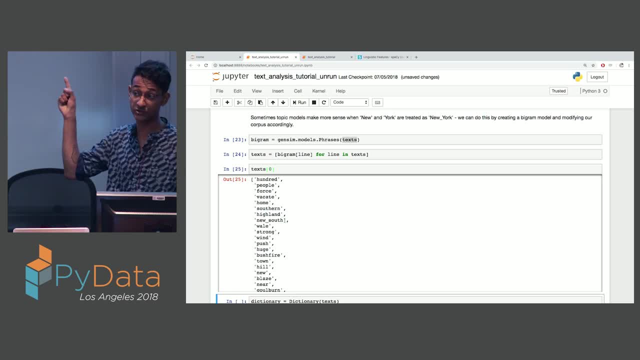 over here in New South has now has an underscore over there. it's new underscore South. so this is what happened in that one line. every instance of New South Wales or it goes to that particular corpus. for the context of that corpus, do certain words appear around each other? if they do, let's make it one word of. 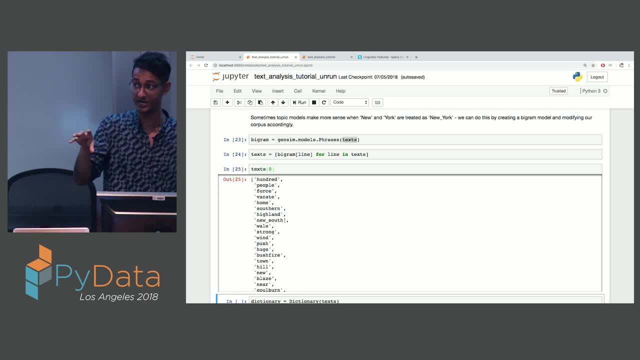 course, this doesn't mean that every time there's a new, the next word gets appended right. it only means for this particular context it gets appended. okay, so it you have different results based on what you're going to be doing. rural fire and fire burn also got picked up over here, by the way. so there is a level. 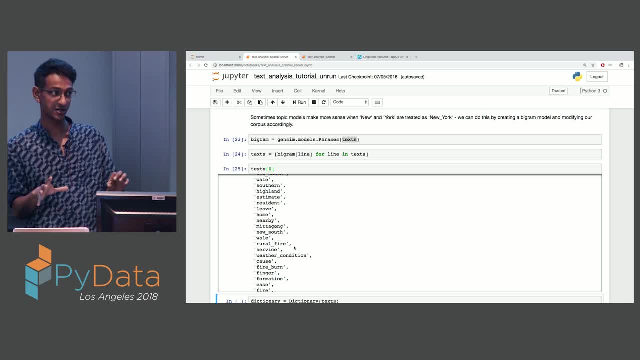 of how much you want to be able to do this. if you want to make sure it's not picking up every word or what extent of it, you'd have to go into the phrases module and play with the parameters, which I'm going to leave all as an. 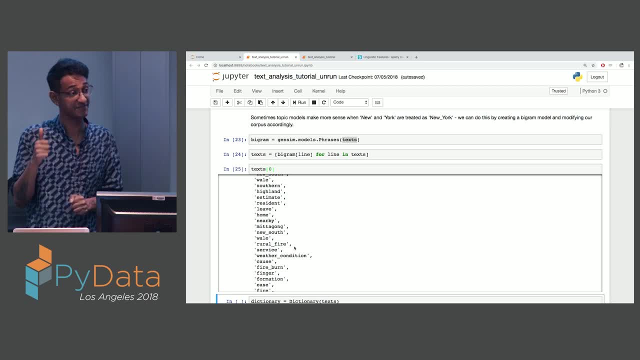 exercise, because you don't have the time to do that, but based on your context, this can be very, very useful. also, rural fire and urban fire of the different things could also be useful. if these words are coming up together a lot, maybe they do mean something. so this is to introduce: 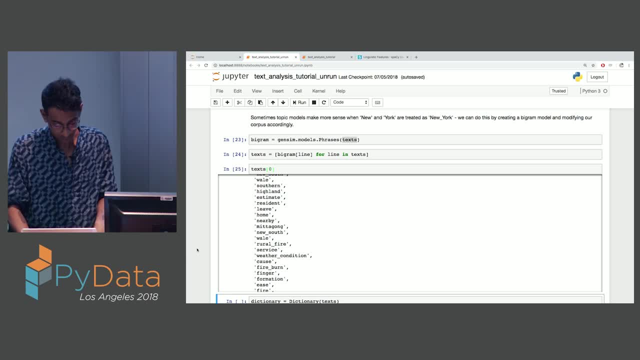 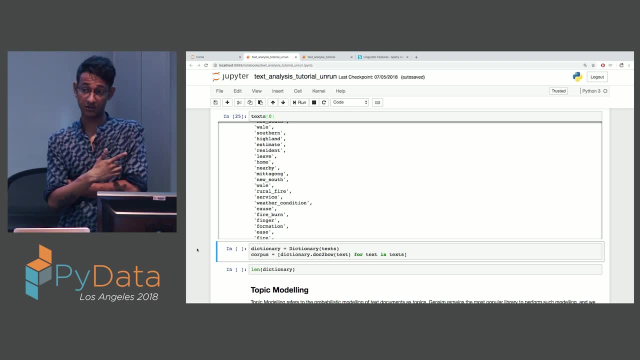 the idea of bi grams in text analysis. sure, oh, yeah, totally. so, like the, the question was: would it be, would it be worth doing a named entity recognition and then running a bigram to make sure only catching name identities? yeah, totally, that would be a good way to do. 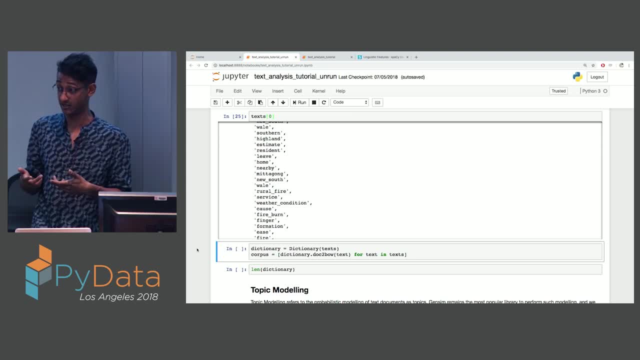 it so that you're making sure that things like rural fire not accidentally picked up on. that is something we can learn about. if you want to do it for the, So you could maybe run a bigram by. you could tag things as places and then make sure a bigram only does those places and go on and do it. 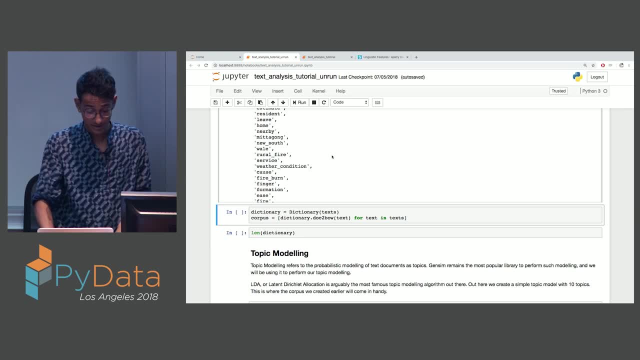 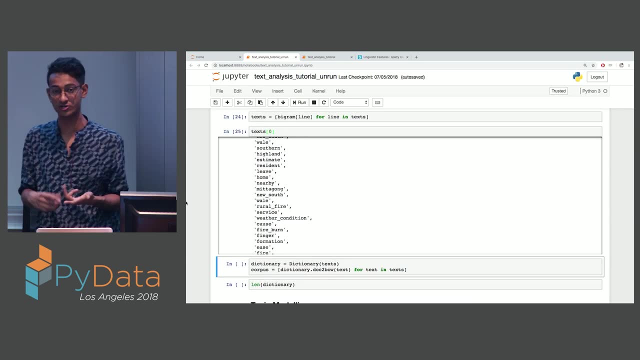 So that is definitely a way you can go about doing things Now we still have to remember that in the end, even though we now have our data set in a more cleaned up, organized way, with no stop words and some cool things put together, 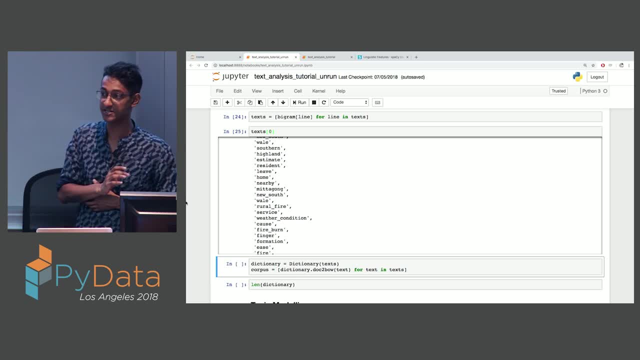 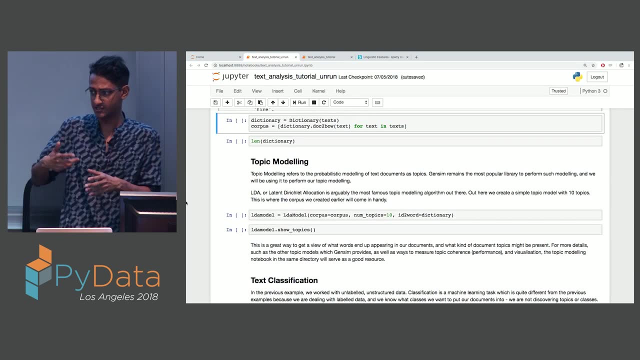 it's still words, right, And computers don't get words. So what we're going to be doing right now is converting words to numbers, And we're going to be using doing a dictionary to do this. Now, a dictionary is a Python object dictionary. 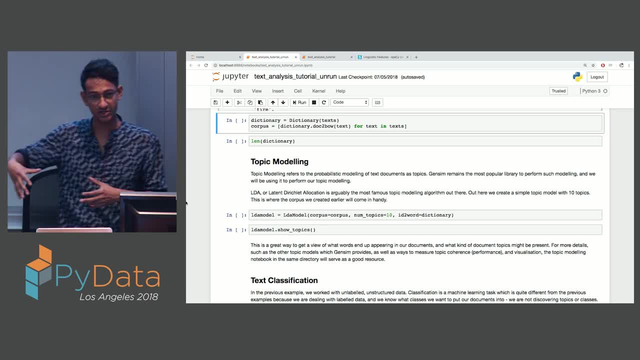 But in this particular context it's a Gensim Python object called dictionary, which basically sets it up easier for you to do things, But the idea remains the same: Every word gets an ID right. So we're going to be creating this dictionary using a dictionary over here. 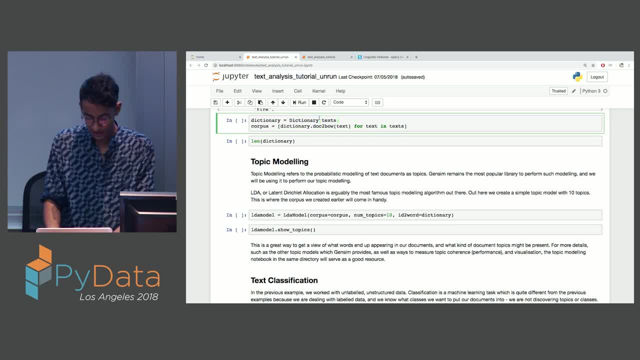 is a Gensim module, So dictionary is equal to dictionary of text. So you're creating your dictionary from texts And you're creating your corpus In text analysis talk corpus basically means your data set. It's just another word for textual data. 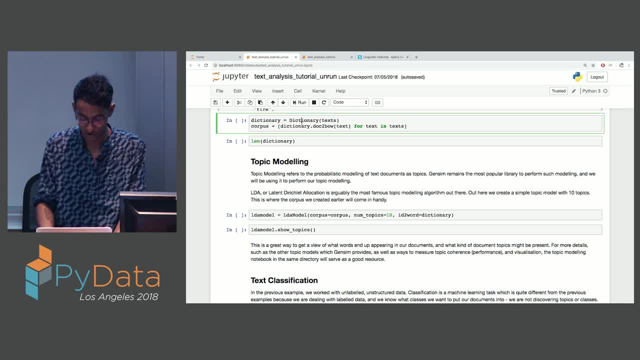 You just call it corpus. in the context of any kind of textual analysis, Or even in the context of research, if you have like a corpus of historical Renaissance data, the word is corpus. This word comes up a lot in things you might be searching up later. 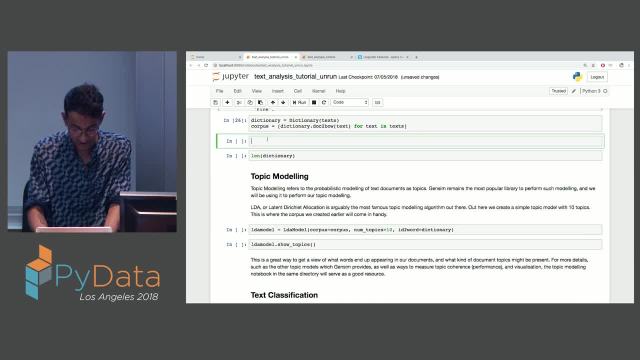 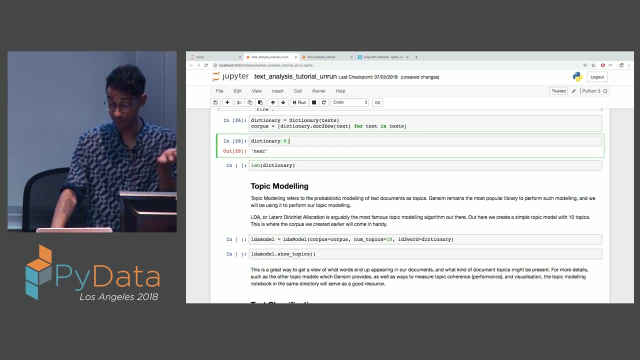 So I'm going to run this And I'm going to briefly show you what dictionary is. So it's a Gensim object, But you also, basically, the index for zero is near, and so on and so forth. So you have, based on the word, you have a different ID. 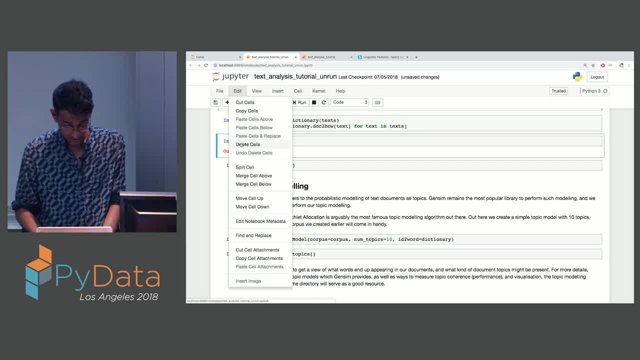 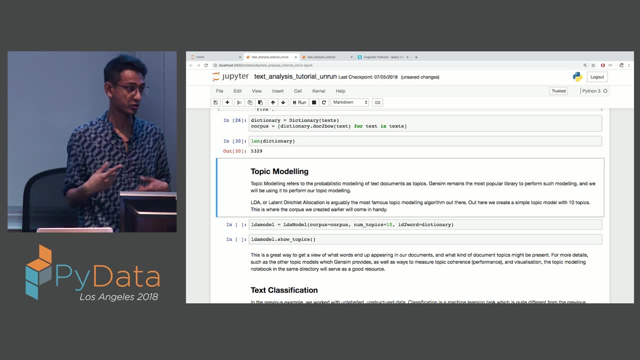 And that's what dictionary is. And now what we're going to be doing is: let's check out the length of our dictionary. So there's 5,329 unique words being used. This is after we got rid of our stop words and a whole bunch of stuff. 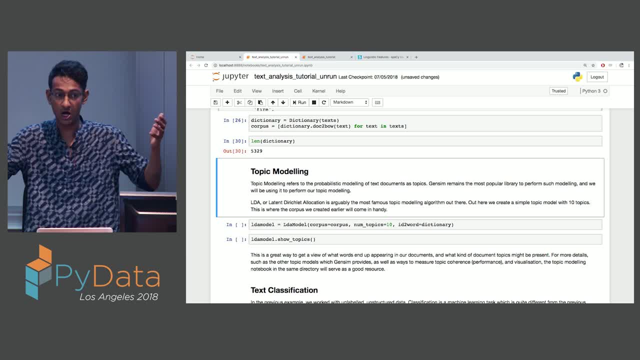 And after we combined words together and everything. So you probably have a lot more before you before you do the cleaning which we did together, I'm sorry. so the dictionary is: there's a. there's a, just a key. 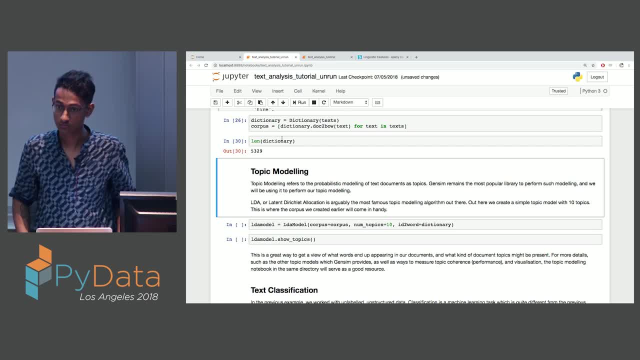 And then it's key to a word that has appeared in the corpus. Sure, Okay, So the dictionary was generated from the corpus, not like a larger list of words. No, no, no, no. Yeah, I should have made that clear. 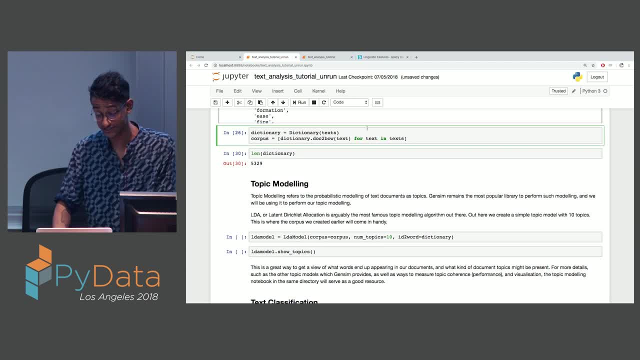 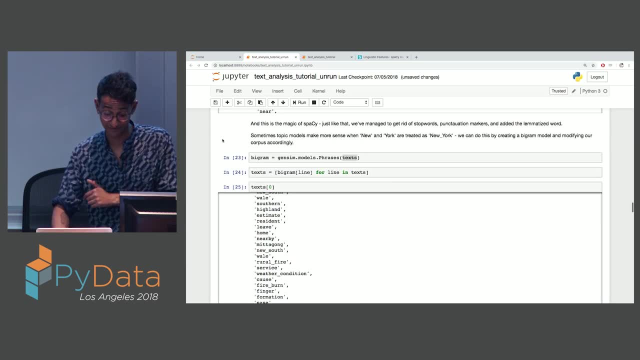 So just to be absolutely clear with that, that's why we did: dictionary is equal to dictionary of texts here, right? And text, if you remember, is just this massive, massive list over here which is all my newspaper articles, right. 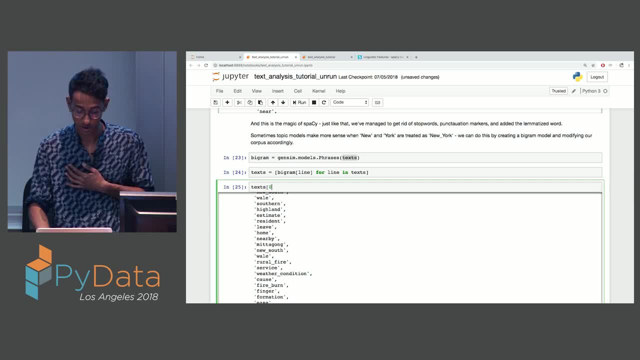 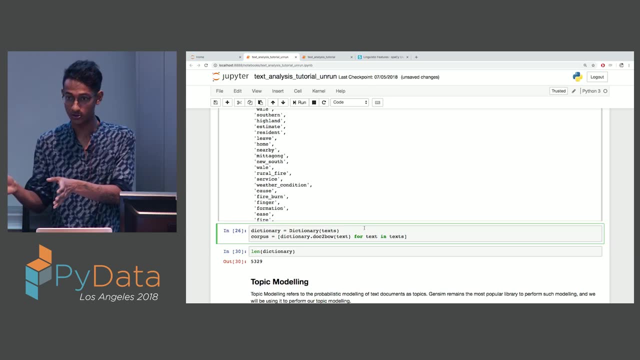 Is that clear? So texts are all my newspaper articles And dictionary of texts is basically the dictionary of all the the newspaper articles, which is all the unique words used there. But this is after we did the cleaning, right? So no stop words. 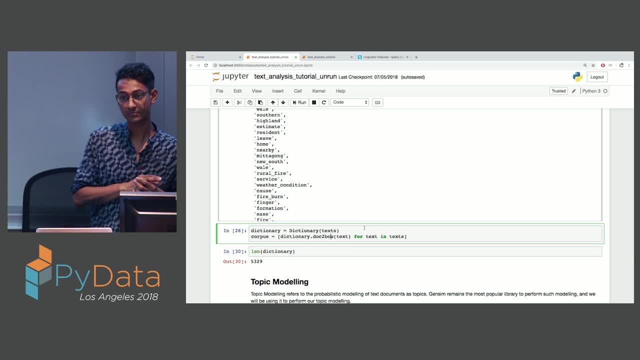 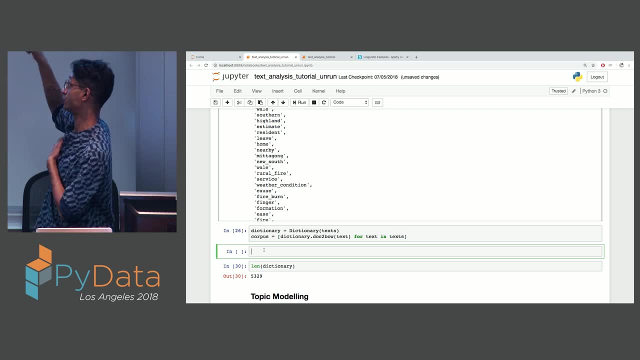 I'm going to show you right now. So corpus, what you detect. the code says corpus is dictionary dot doc to bow. Now I should probably explain that. before that, I'm going to tell you what bow is. Bow is bag of words. 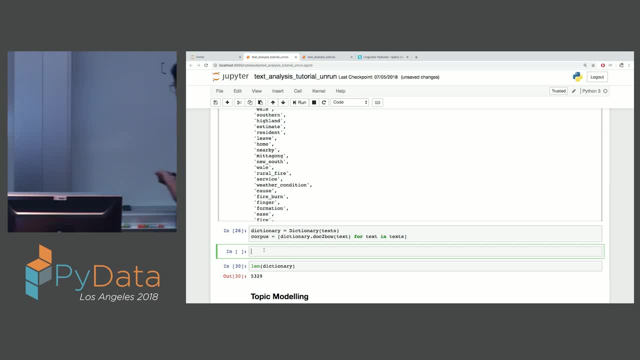 So what's been happening over here? before? if you had a document like any kind of document, it would just be zero or one based on the word being there or not being there. But again, that takes up a lot of space. What if, instead, we can do? it's probably going to be easier if I just run the code- basically a corpus of zero. 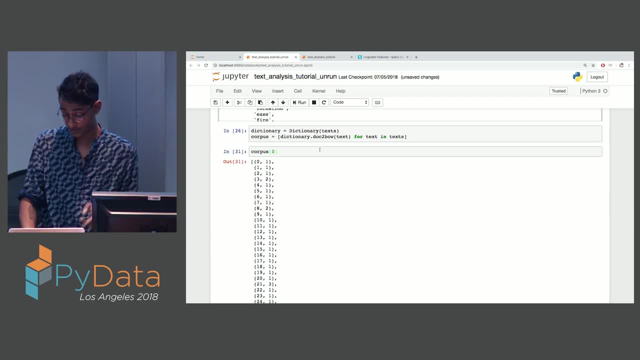 this is what text has become, has become this: zero comma one, one comma one, two comma con. What does this mean now? This basically means that the zeroth word appeared once, the first word appeared once and the third word appeared twice, and the twenty-first word appeared three times. 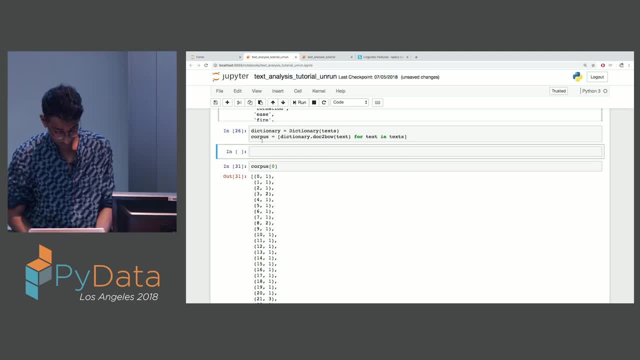 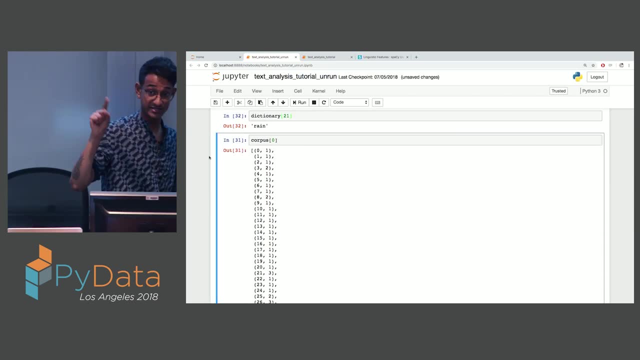 Can you see what's going on? So the twenty-first word is yes. The twenty-first word in the dictionary is rain. So in that particular document the word rain has appeared thrice. Now the reason we're doing this is because otherwise we would have this whole massive 10,000 word array. 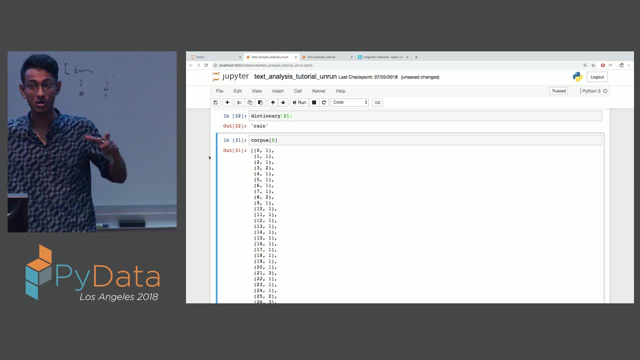 with every single, is it there or not? and we still like. so we want to compress that. So it's called a bag of words, because each of these zero, each of the indexes is like a bag and we're like counting words. 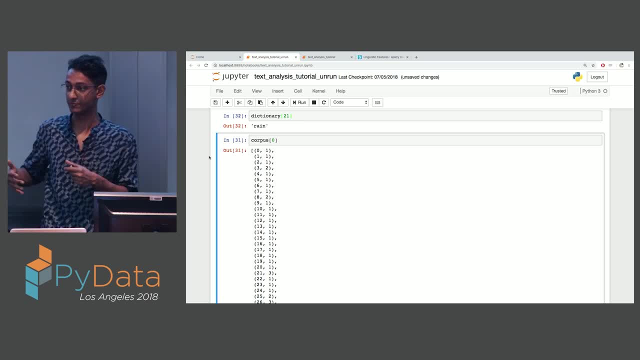 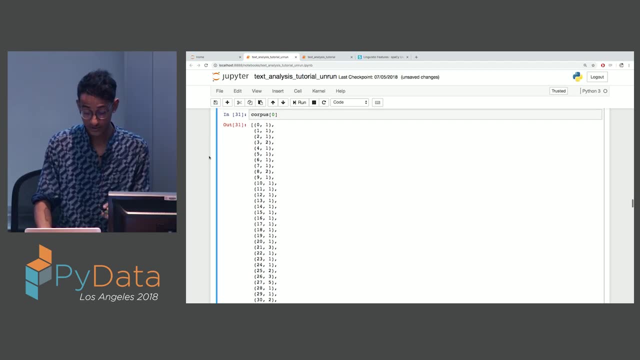 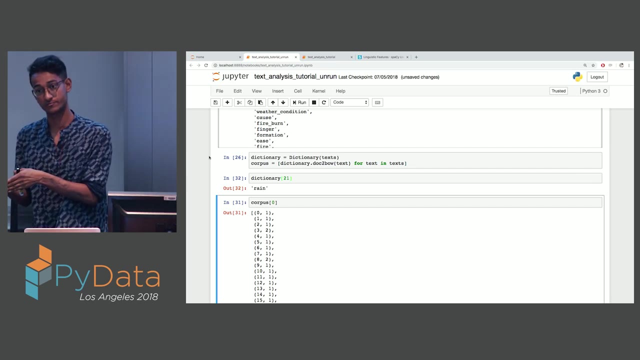 So that's what's going on over here. This is just an easier way for the computer to deal with a sparse data, a sparse vector. So that is what corpus and what is the code for that? Dictionarydoc2bao. So document two bag of words of text for each text in text. 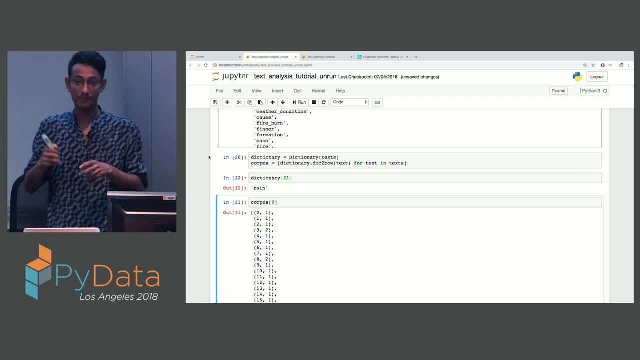 So again, I'd like to: you could actually build this dictionary yourself by. you know, it's not super fancy Python code right like just iterate through all your documents. It's just a kind of a pain to do it. Gensim is specifically for text analysis and does it for you. 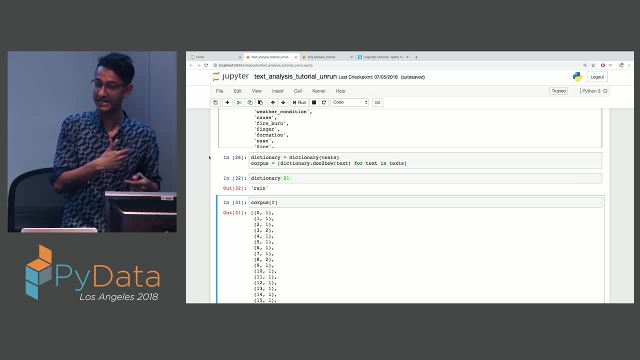 To be clear, scikit-learn also does it spacey Like any kind of Python text analysis library is going to have these words. So that's what corpus is. Library is going to have these functions in it. But I'm kind of breaking it down so you can also do the code yourself. 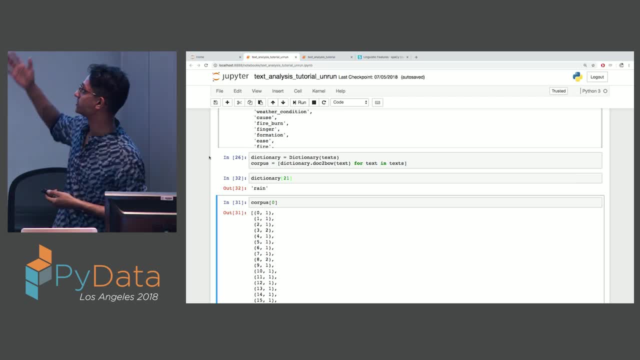 But it's optimized, it's fast, it's easy. And dictionarydoc2bag of words for text. So is that clear what we went to from where, Like we had this raw text to cleaned raw text, to list of lists of raw texts. 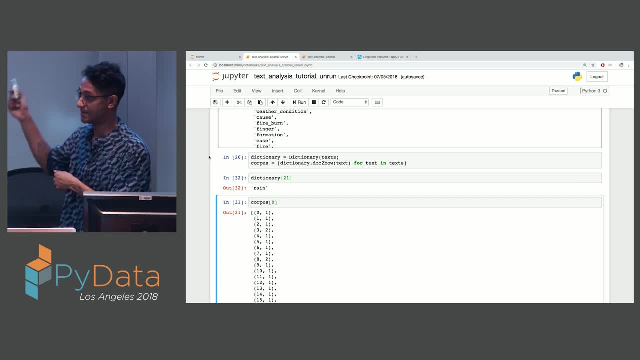 to bigram of raw text and now to a bag of words of raw text, And because this is kind of our final form of cleaning for our analysis, I'm going to call it corpus, because that's just what we normally call in this particular field. 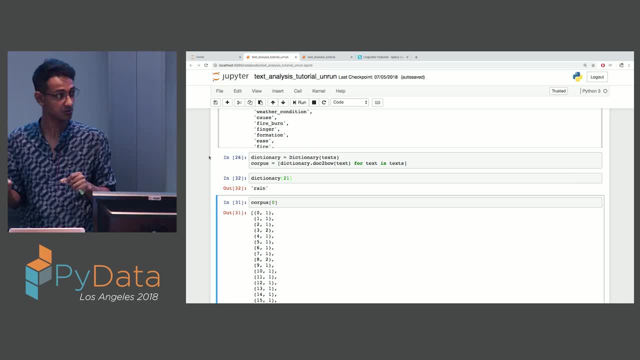 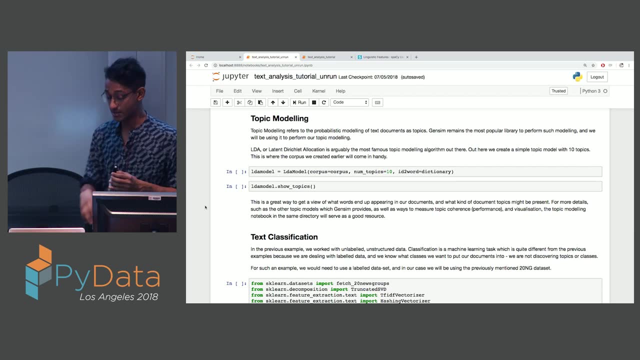 So is everyone up to speed over here at this point? Awesome, Okay, so now we're going to start with. so until now we, so it's 1147, which means it's been 47 minutes, 37 minutes more or less. 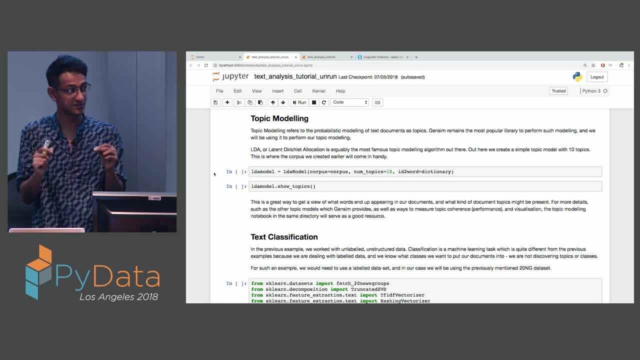 of only cleaning text. The reason I've spent so much time is because it's extremely, extremely important. You cannot, even if you know all of these things, all of these fancy machine learning methods, after this. it's pointless. You're not going to get anything interesting or useful. 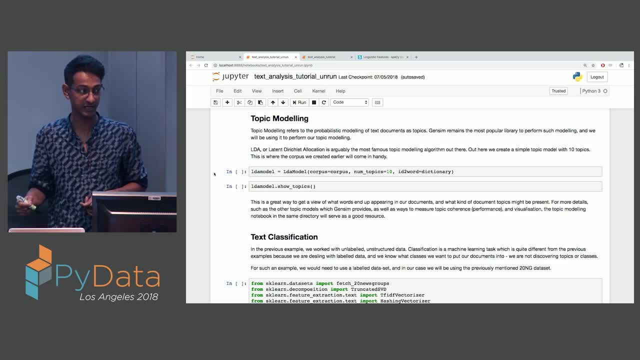 if you're not going to be very, very diligent with your text cleaning. So it's important to know what you can possibly do, why you're doing what you can possibly do, and have any sort of idea. This is not the only. these are not the only things you can do. 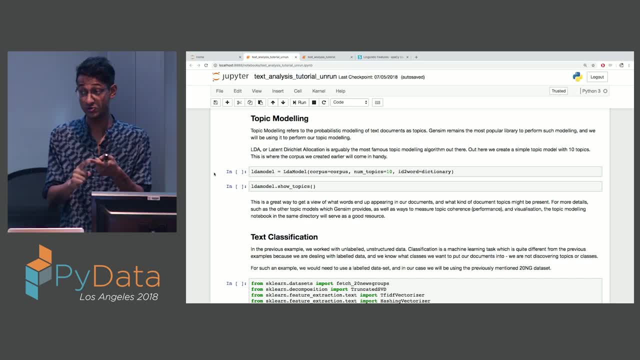 There's a lot. people get into more detail and you can get. for example, you can get rid of words which are not frequent, Like if a certain word is turning up once in one document. you're like, oh, why do I even need that word? 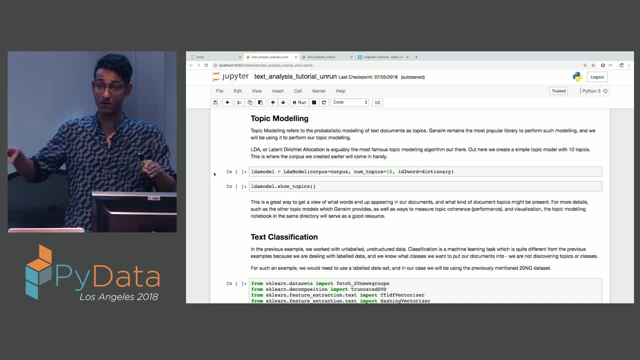 So you get rid of that And you can keep 5 or 10 or whatever number you want as your minimum frequency cutoff. You can keep a maximum if the same words are appearing in literally every document. is it information, so to say? 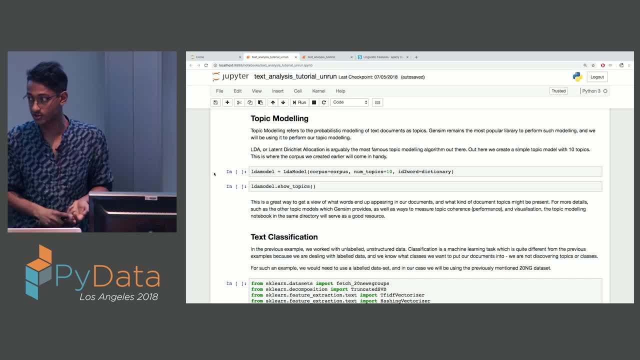 So you can get rid of the most frequent words, the least frequent words. You can do all of these things. These are also things done in text cleaning. I'm not doing them because it's not necessary, but you can totally do it. 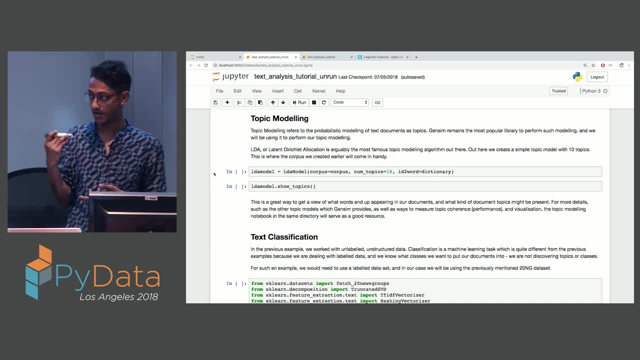 There's a lot of ways to go about doing this. This is my way of going about doing this particular way. You get different kinds of results, but it's heavily contextual, Based on your business problem or whatever personal project you're working on. 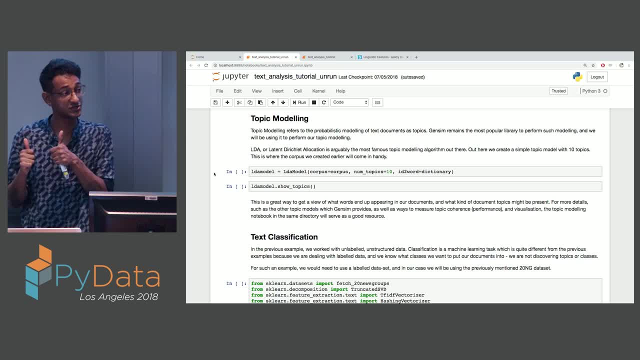 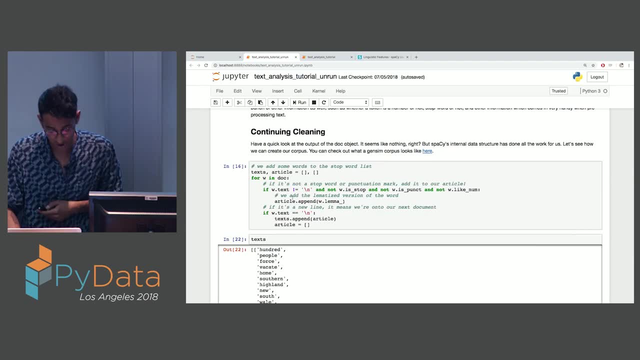 you'll be having a different cleaning process. These are the kind of stuff which everyone does. I have one thing to mention which I actually forgot to talk about Over here. this is the super important one- number 16,, which Sal was talking about. 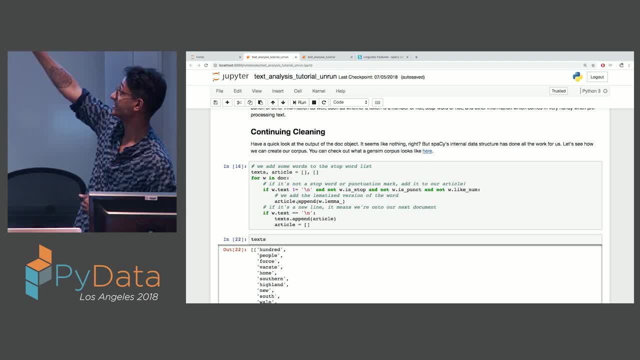 I said, articleappend is equal to wlemma Right. wlemma is not text. I've written on top. we add the lemmatized version of the word as a comment over here. I forgot to talk about what lemmatization is. 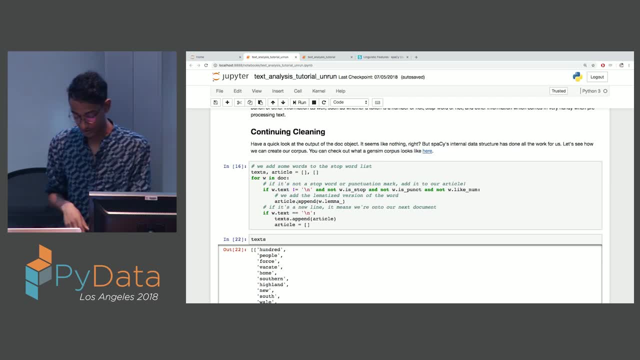 It's a very important part of text analysis. Basically, the word saying said and say, for example, all of them have the root word say, Writing, wrote, write. all of these are the same root word. If this word appears in different because of the function of the kind of word, it is. 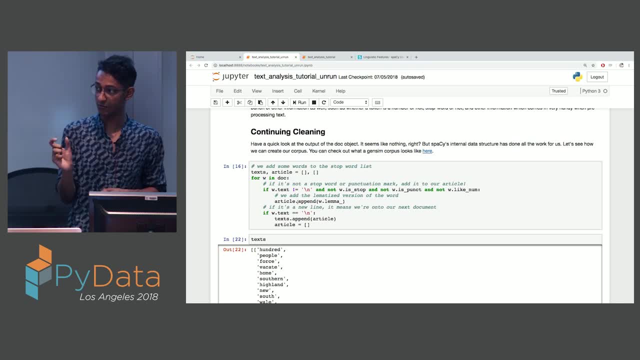 it appears in different forms in my text. it all means the same thing. If I want to capture that original root word, that's called a lemma. This form of getting the root word is called lemmatization. For some words, the word itself is the lemma. 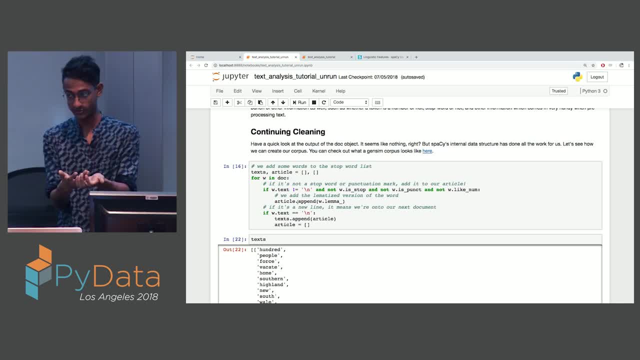 For any other words, saying will become say, and say is also say, but both of these represent the same word. It's called lemmatization. I would recommend you could do a really quick Google for lemmatization if you want to read about it. 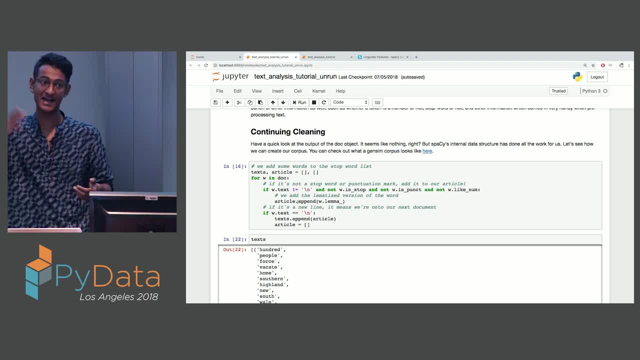 There's another concept called stemming, where you just kind of hack off the last part of the word but then it looks kind of ugly. It's not very pretty, so I prefer to use lemmatization, But you could also use stemming. 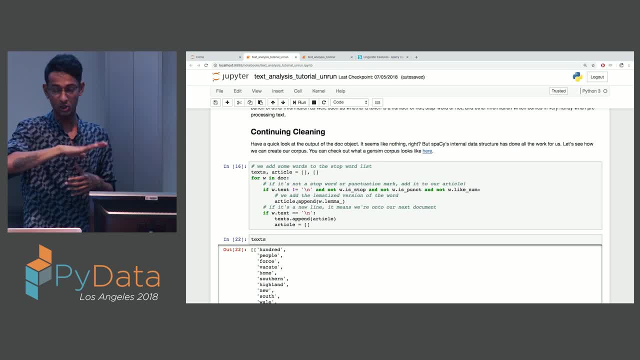 Stemming and lemmatization are two ways in which we basically, if there are a lot of words which could mean the same thing but are just different forms of the word, we want to just use that base form. That process is called lemmatization. 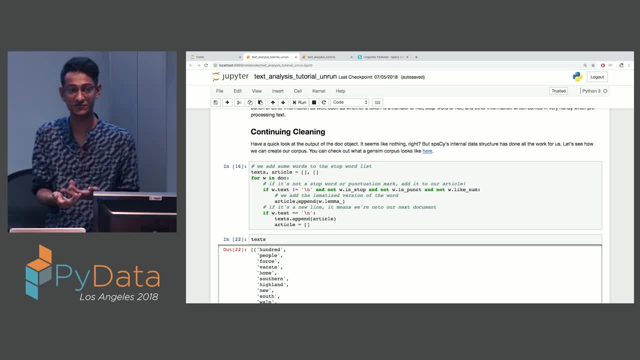 I've also only added the lemmatized forms of the words. This gives better results, Though, that being said, you could also not do this. It's really up to you, But this is a very important part which I missed out on. 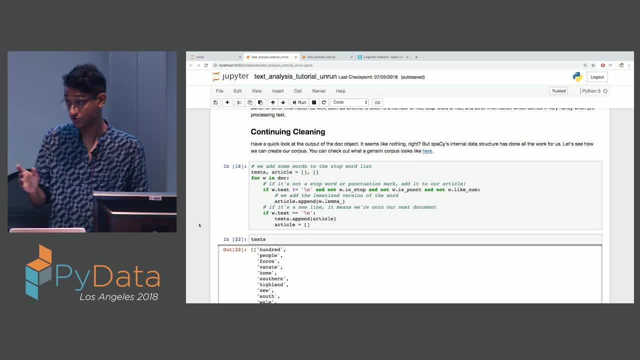 So it's the lemma and lemmatization which also spaCy's got, like when it did its whole document analysis, it did lemma as well. spaCy are not paying me, by the way, I really just like them. So we're going to start with topic modeling now. 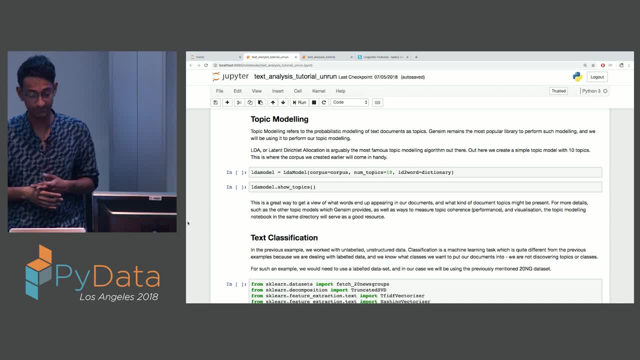 which is the first machine learning part of this tutorial, right? So I briefly talked about topic modeling before. very briefly, I said that if I have a newspaper corpus, which you happen to have, this is in a context of Australian Southern whatever. 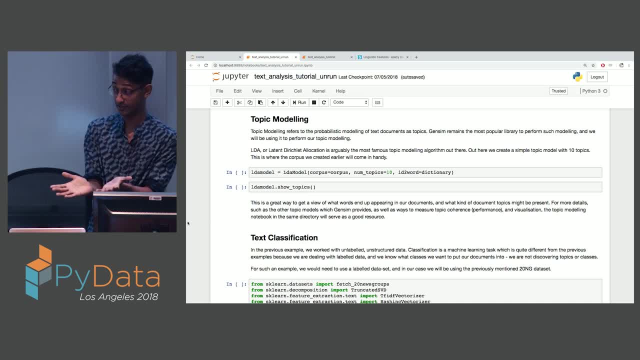 but let's just say very broadly: if I have a lot of textual data and I want to classify this and I have no information whatsoever, a topic model is a really nice way to get a cursory glance at my documents, For example, if I feed in 10,000 newspaper articles, 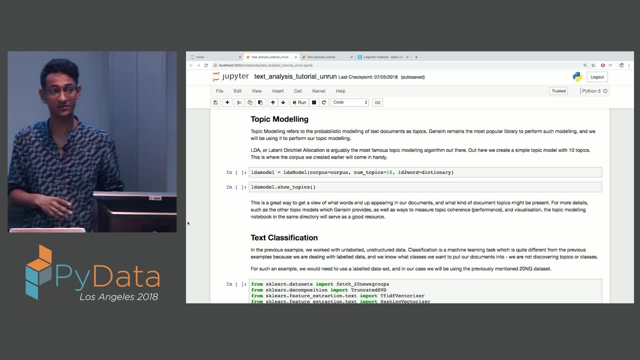 I can end up and I say four topics or three topics or something like that. I can end up getting three topics which would be sports, which would have football, soccer, basketball, baseball, so on, and maybe some names and politics. 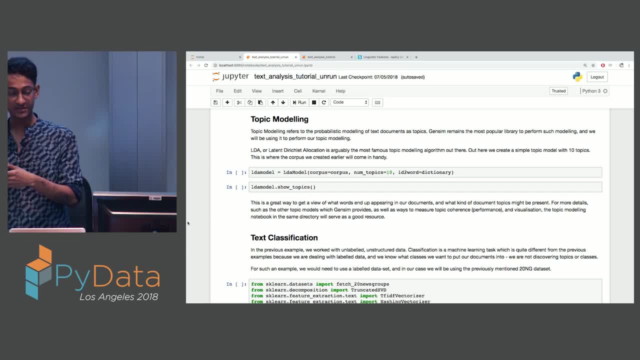 and you'd have certain names associated with politics and weather, which would be sunny, beat, so you know, or I'm from Chicago, so rain, cold, miserable. So you'd have things like this based on your newspaper articles: 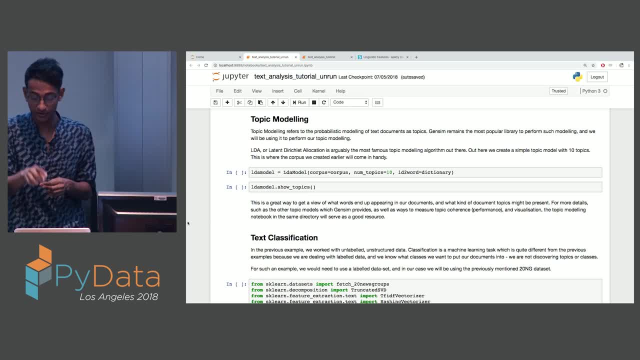 which you're actually dealing with Now we're going to find out exact. so the way it does this is. it's called latent derelict allocation is the name of the algorithm. This is the name of the most popular one. There are multiple topic modeling algorithms that you can use. 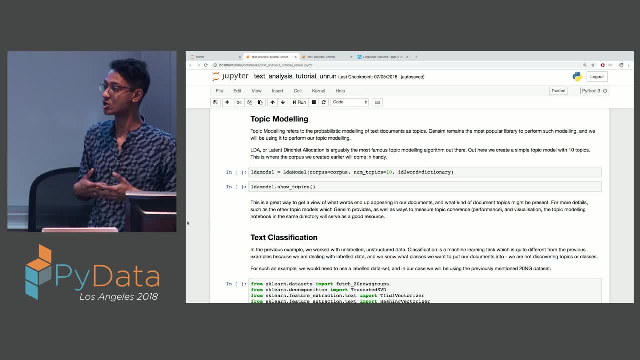 but it's called latent, derelict allocation. because latent? because these topics are not clear to us immediately. They're latent topics hidden under the text. so to say, Derelict is a kind of probabilistic distribution, which is how it does it, which is it's kind of Bayesian inference. 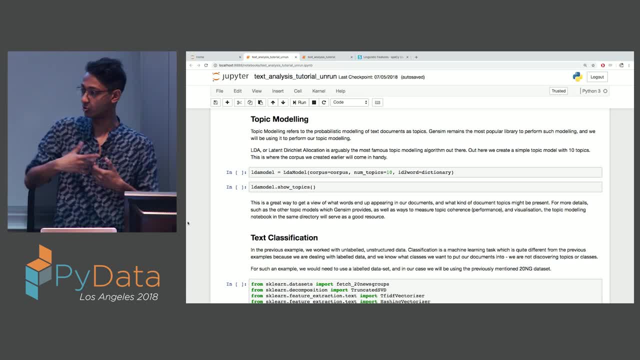 It's a statistical modeling algorithm where it looks at what kind of words appear around each other, with what probabilities, and it kind of does an analysis of trying to find topics of words and documents which come together. Topic modeling in itself is a you know. 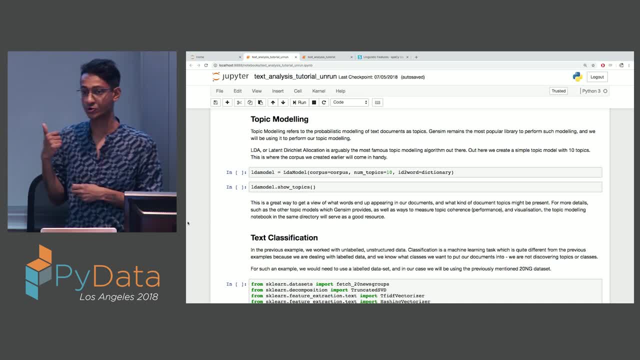 huge research field. I've done a few tutorials on topic modeling before which you can search up if you're interested, or you can just talk to me after this, But I'm going to very briefly go through what it is. Rough idea: massive, unordered, unclassified text. 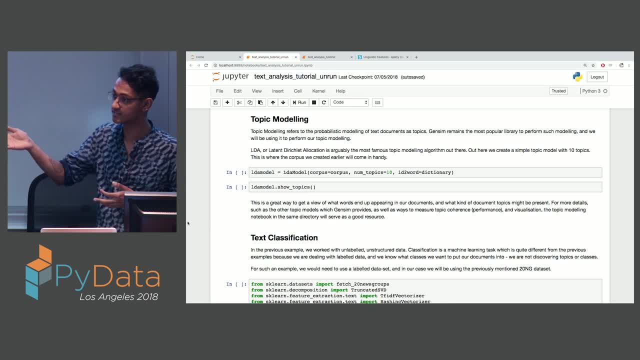 Now you have topics after which you can choose to classify or not classify, But these topic models are useful in general, right? So what am I? so I'm going to be? the import here is LDA model, which you can see over here, which is from Gensim. 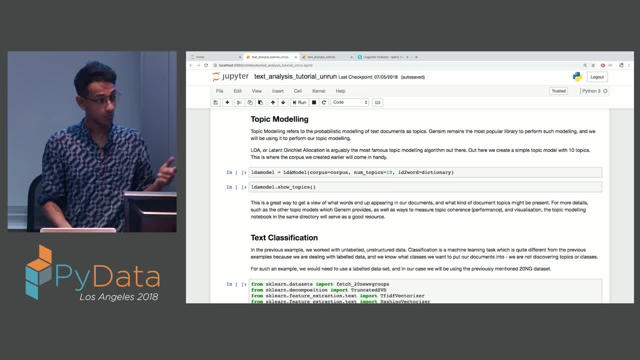 which, if you check the imports, you would find it over there. What are my inputs or the parameters over here? Corpus is the corpus we just created. Number of topics: 10, so you have to specify right the number of topics you want. this is very important. 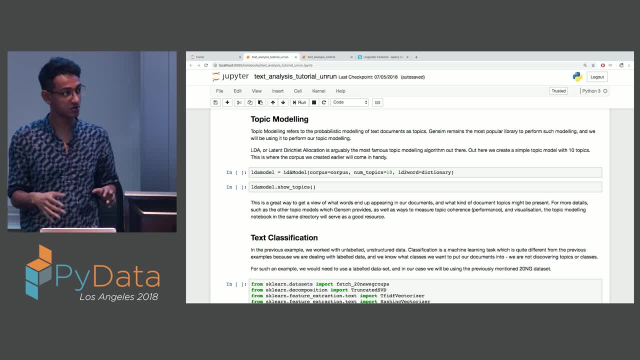 It's not going to find out the number of topics on its own. There are certain algorithms which attempt to do this, but really it's. you should have a very rough idea. Alternately, you can just run like seven. hey, this looks, this makes sense. 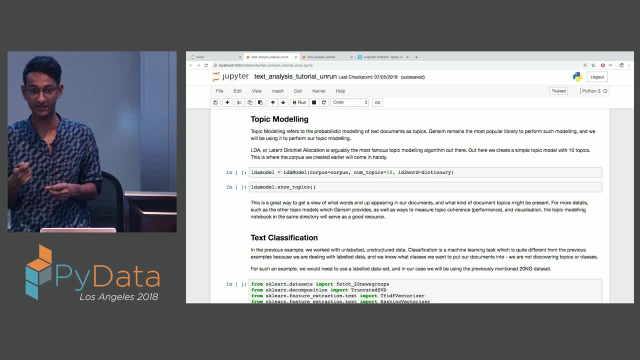 eight. this doesn't, and you can figure it out. There are more quantitative methods to find out the number of topics, but that's like a whole again field on its own. I've written tutorials about that in the same repository, which you can actually search up, since you don't have this repository. 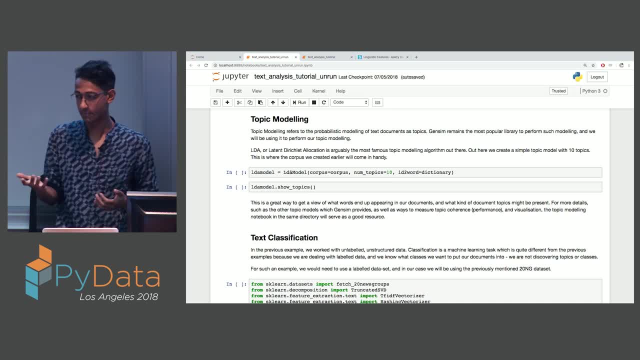 I get more into topic modeling, but the idea is you need to tell the number of topics you'd want, right? So number of topics is 10, and ID to word is dictionary. over here It basically means ID to word, which is a dictionary. 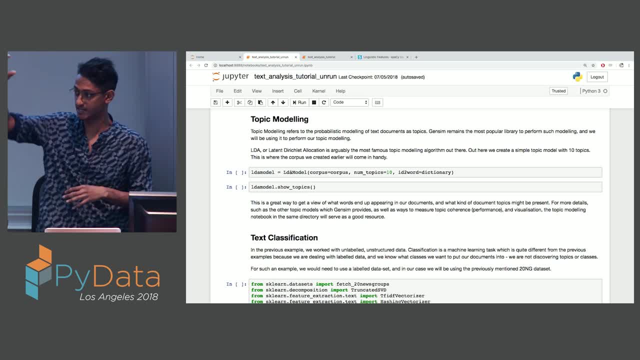 But you can put in a Gensim dictionary object. You can also put in any dictionary which has IDs and words, but the idea is zero to whatever. And the reason again is because when you print your topics it needs to have an ID to word mapping. 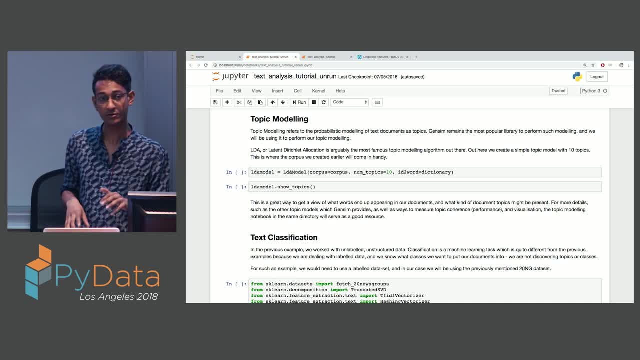 So it's just for Gensim to know what's going on, right? Any questions before that? No, Okay, cool, So I'm going to run this. It's not a super massive corpus, right? It's only 300 documents. 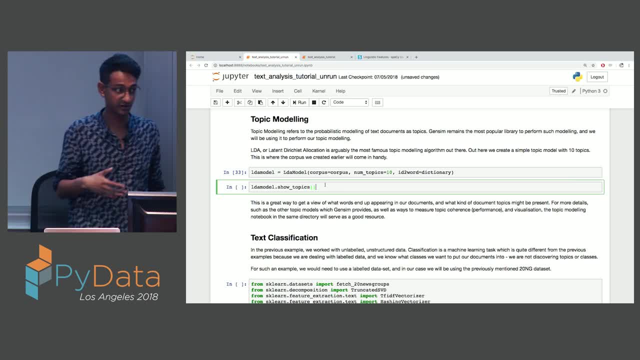 and normally that's tiny data in the context of data analysis. Normally you're dealing with thousands of documents, but for the purposes of this tutorial it's still a reasonable number. So I'd like to make it very clear: The more documents you have, 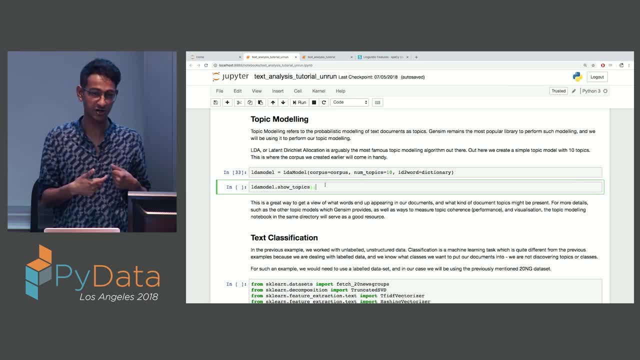 the more fleshed out your topics are going to look right. 300 documents is not enough to have really beautiful topics come up which represent some kind of complexity. But that being said, let's see what kind of topics we have. Okay, 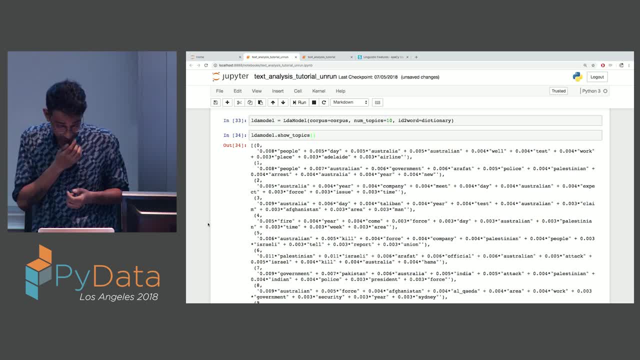 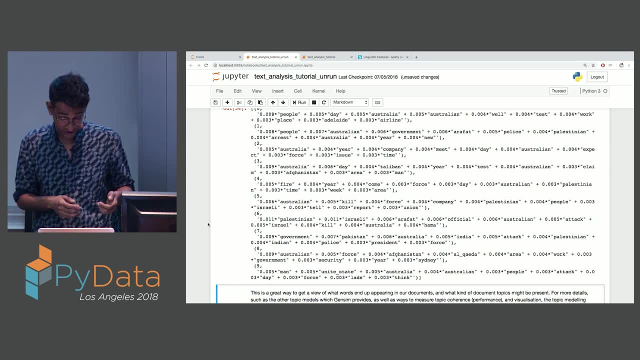 People day, Australia, Australian- Oh, this is an Australian day, maybe Adelaide airline. Then you have your company. Then you have something with the Taliban. Australian kill force company. Oh it's pretty. 2001 was not. 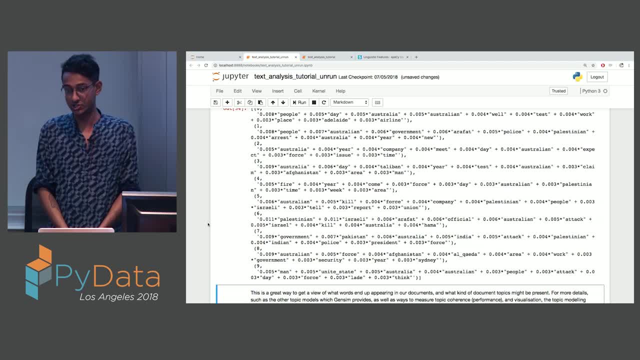 Well, yeah, So you have. These are the topics which you see. So you can see there's a kind of a theme going on. There's something: Government, Pakistan, India, attack force. So well, there's a bunch of different topics. 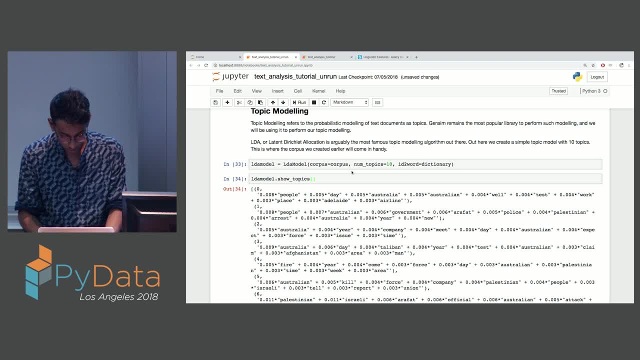 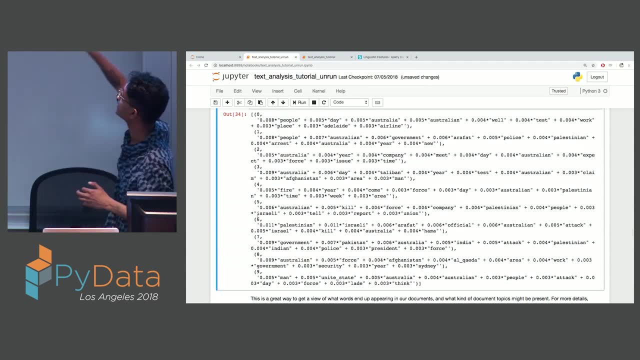 You can really fine tune. This is 10.. I could totally do like five Run this again. In the meantime you can just have a look, Tell you what this looks like. Zero is topic zero. topic one. topic two. 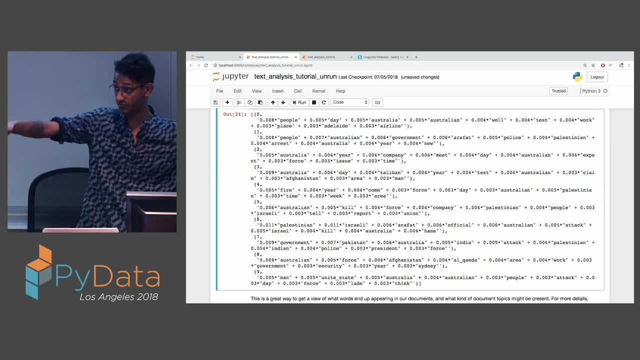 So also the topic which I have called, like the weather topic or the sports topic, it won't exist. It won't have a title. You have to give each topic a title of your own. A topic is a probabilistic distribution of words. 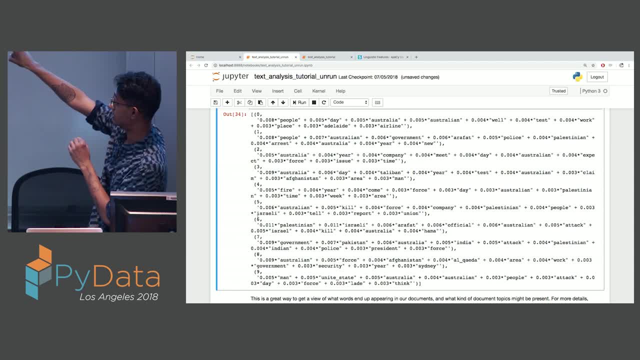 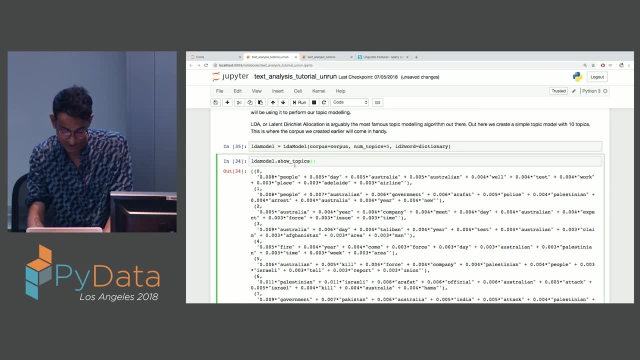 Right, So it's like these words are going to appear in this topic. with that, The odds of these words are being the topic are more. So I'm just going to show you, with five topics, what it looks like. Maybe it's a bit better. 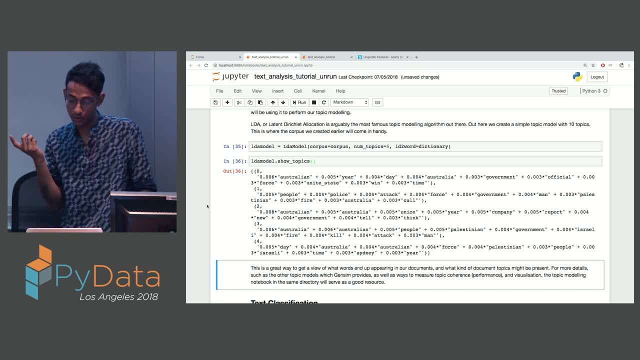 People police tech force, one in Australia. So you can see over here maybe Australia is not a very important word because it's an Australian newspaper corporation, So we don't maybe need that. You could then add that in your stop words. 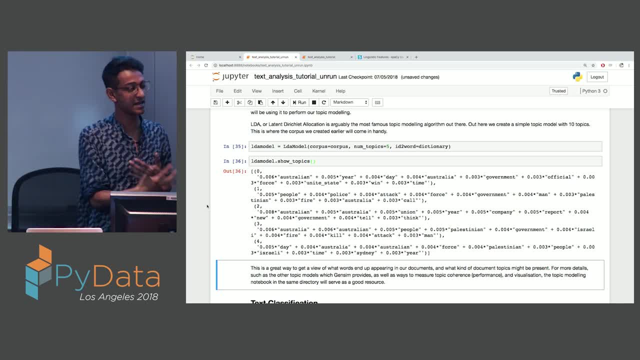 remove it and do it again and then you'd see your results Right. So you can see it's a heavily iterative process of finding out your ideal topics. Again I would. my topic modeling tutorial in the same repository goes into more details on getting better topic models. 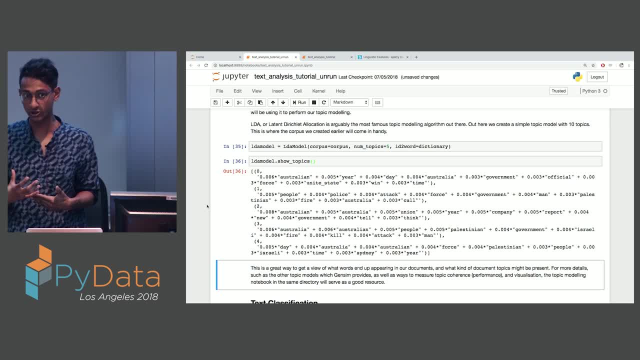 Right. This is just to give you an idea of what they look like and what you can do. Also, based on your data set, they will be. it will be varyingly useful or not useful at all. It's kind of hit and miss. 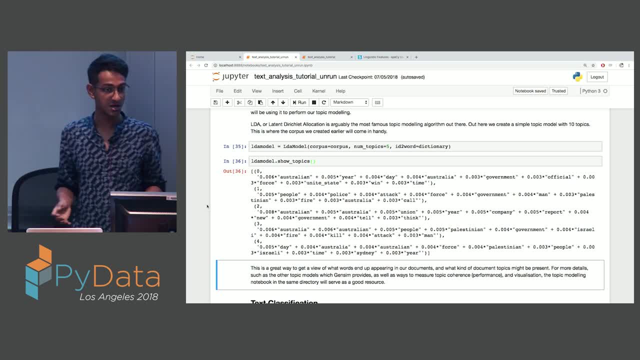 But I find it very useful in exploring large textual data sets. You could also find out the percentage of each topic in different documents. It's just a useful model of your textual data. if it's unclassified, in my opinion, Yeah. How do you decide how many topics? 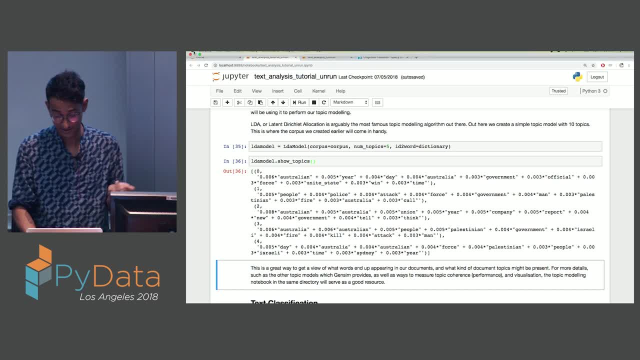 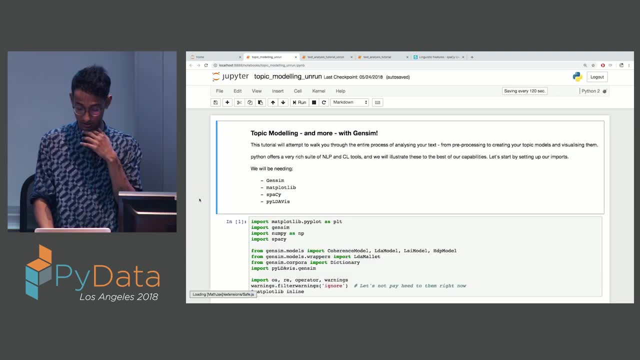 That's a very good question. Now I've actually- so I did mention about how I do have a topic modeling tutorial which I'm going to briefly open but not get into. It's called topic modeling. So over here I actually talk about how to find the number of topics. 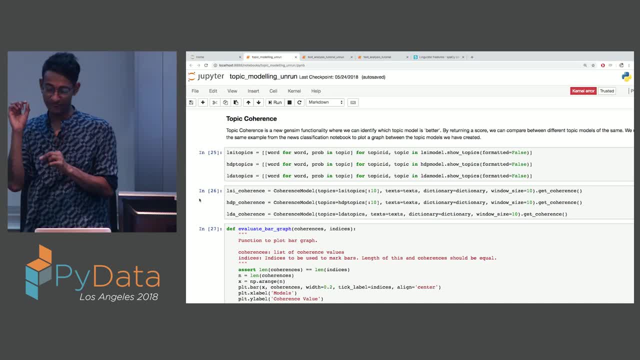 Well, one way which I'm going to very, very briefly get into, is something called topic coherence, which is a quantitative way to tell you how good or bad your topic is. So what you would do is you would run your topic model for 7,, 8,, 9,, 10, or 10,, 15,, 20,. 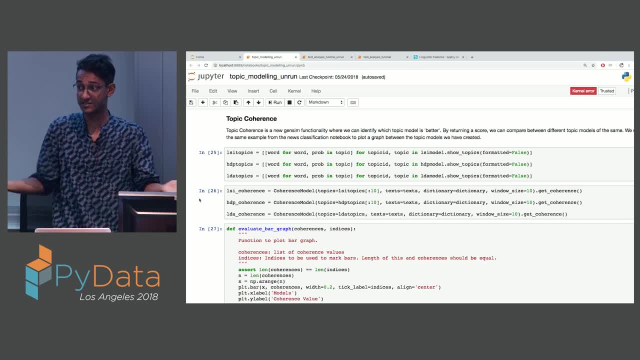 whatever you think might be the number of topics, Check out the topic coherence values for each of these topics For a number of topics, And then choose the best number. The other way is: it's a really tough question. There are different ways you can find out how good a topic model is. 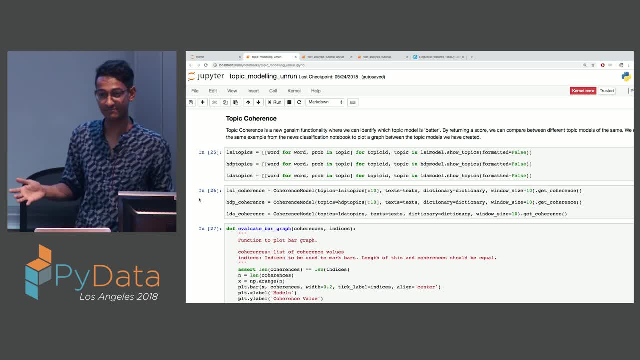 But in the end it really comes down to: hmm, this looks kind of right, you know. But that being said, there are a few quantitative ways. Topic coherence is one of these ways. There's also a bunch of pretty graphs and plots which allow you to kind of figure out, you know. 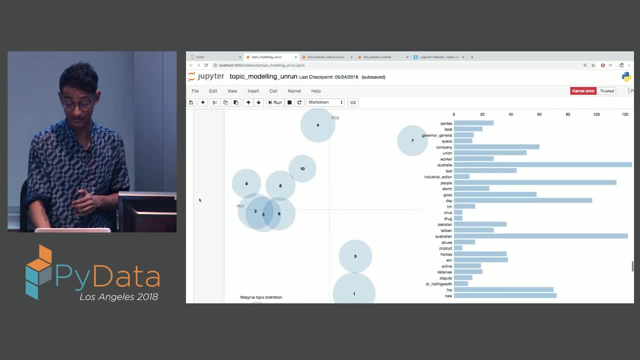 Like, for example, one way is: this is one way You can see over here. this is not in this tutorial, but a different one which you can see. You can see a lot of these. These are all topics, by the way. 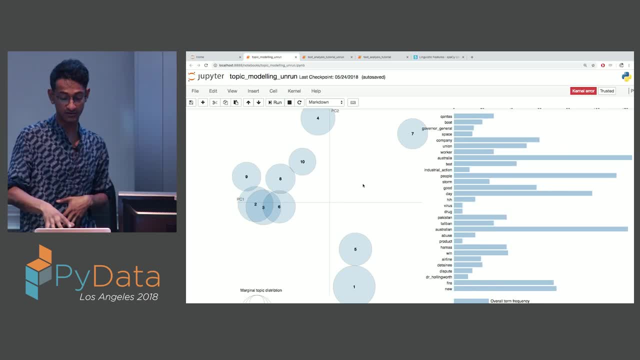 This is a visualization of topics. You can see that a lot of these topics are clustering together. So, hey, why not just have one topic instead of all of those, right? So these are ways you can try and do figure out what is optimize, your topic model, so to say. 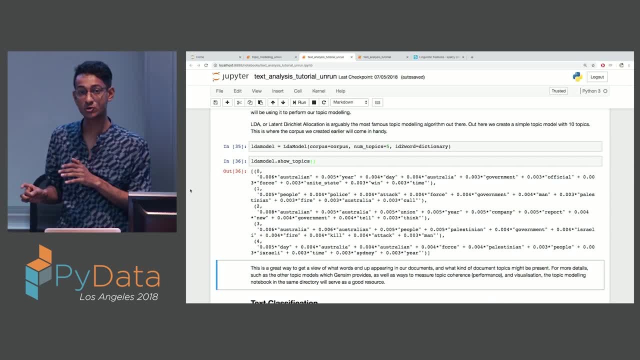 But we're not going to be getting into that. It is super interesting still, I think, just to be able to find out what kind of topics are in your text with, like no prior information. To be clear, we, there was no prior information. 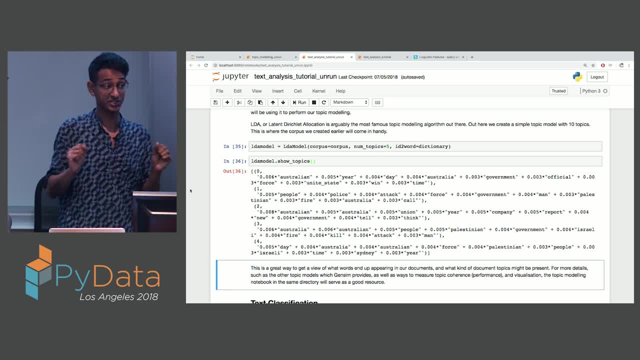 There was no classification going on over here. We gave no information, We just threw like a bunch of text and it said: this is useful information, which I think is very, very cool. So I'm a big fan of topic models and I think they're really useful and interesting. 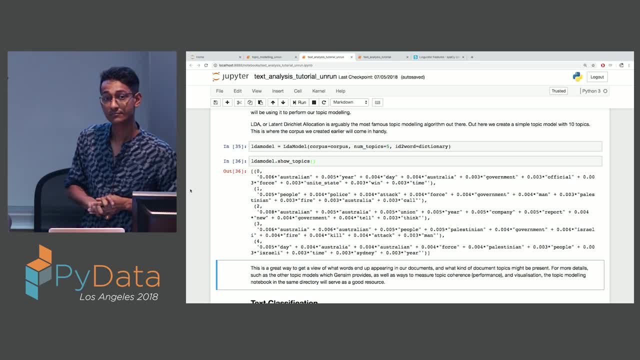 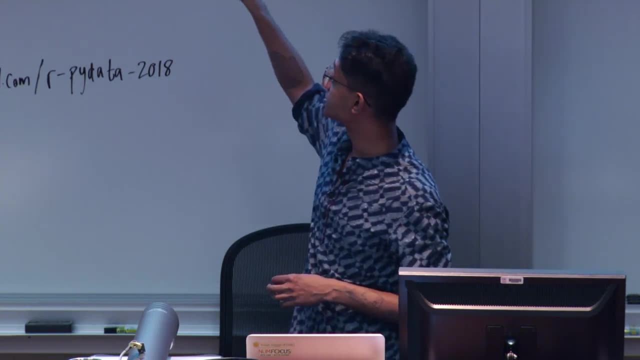 Yeah, So for the coefficient in front of the numbers like 0.005 and 0.004, is that the probability or is that a correlation of circumstance? It is the probability of that word appearing in that topic. We only show the top 10.. 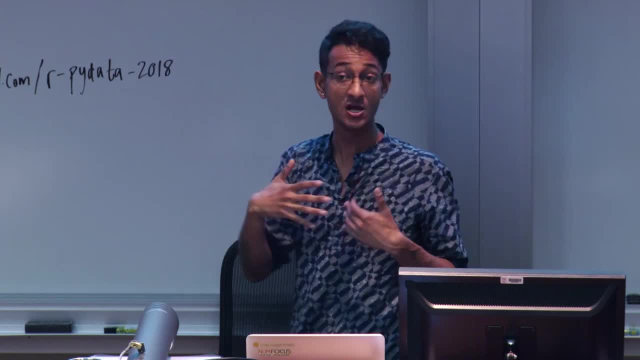 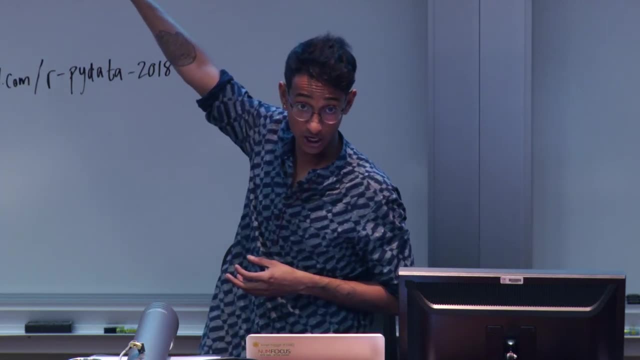 I believe it's 10.. You can choose that. by the way, Gensom allows you to choose the number of top words in a topic you want to display. In this case, it basically says: for these five topics, these are the 10 most probable words to appear in that topic. 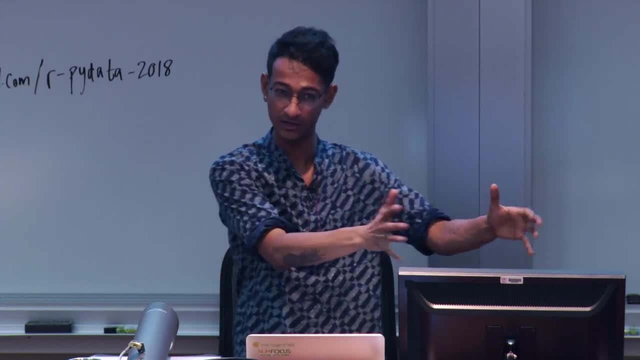 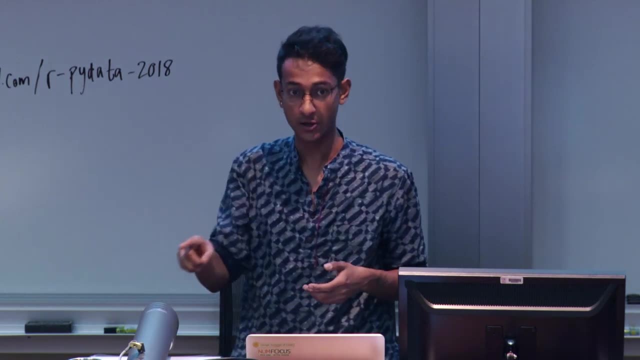 So these words tend to make, tend to aggregate over here. You see, Now, as you go on, you'd have obviously like the probability gets lower and lower and lower, And also this probability is shared between the numbers. 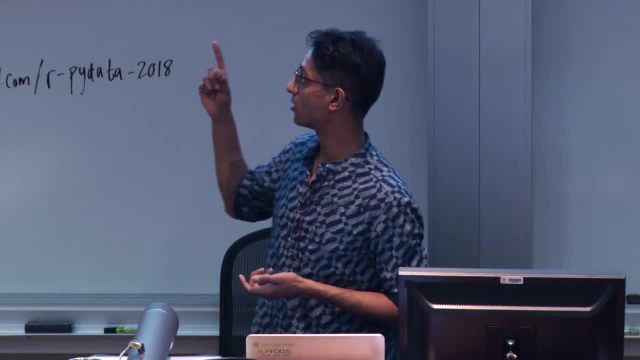 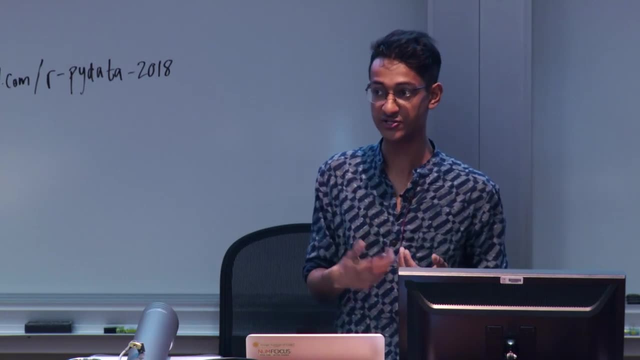 It's between 5,239 words, Right? So you may argue: oh, 0.004 is a tiny, but it's not in the context, Right? So you'd also have more interesting results, a larger data set, And Gensom is a really neat package which does a lot of different kinds of topic models. 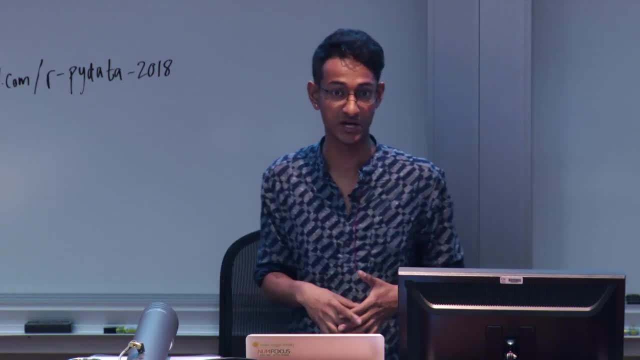 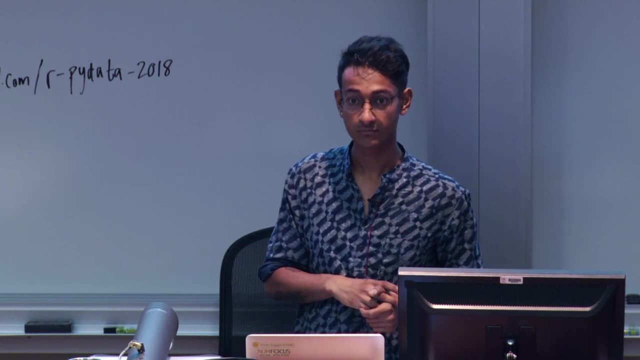 This is not the only kind. There's a lot of different kinds of topic models. by the way, Yeah, I was wondering what the same product. you ran it before, but, for example, you would see Australian, Australian, Australian nouns. 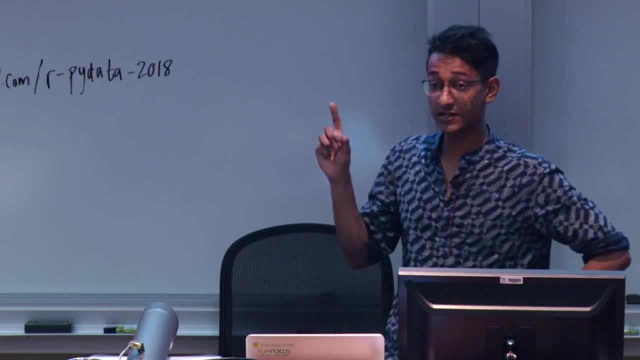 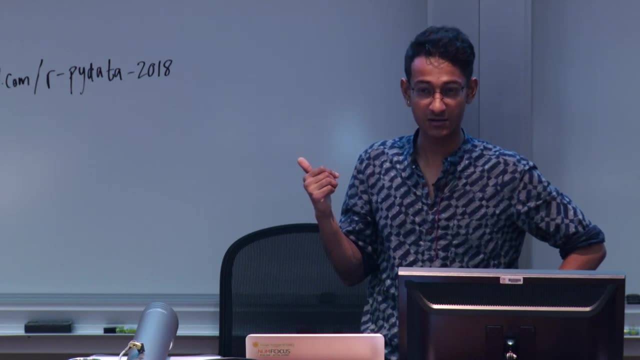 Sure, Sure. So I think in this particular case, in this kind of stemming, I think, because it's a proper noun, it's ignored. That would be my guess. Right, Yeah, That would be my guess. Normally this would be caught, though. 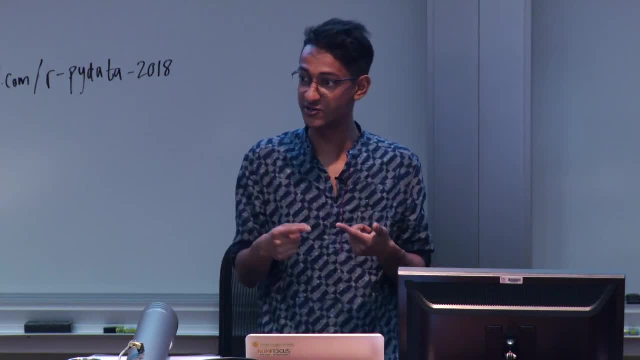 That's a good point. Again, like all of these kind of things, like every time I do like a variant of this tutorial or this tutorial, people point out that, hey, this is kind of, and that happens. 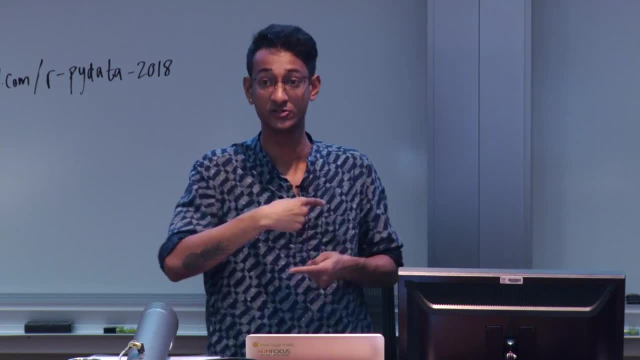 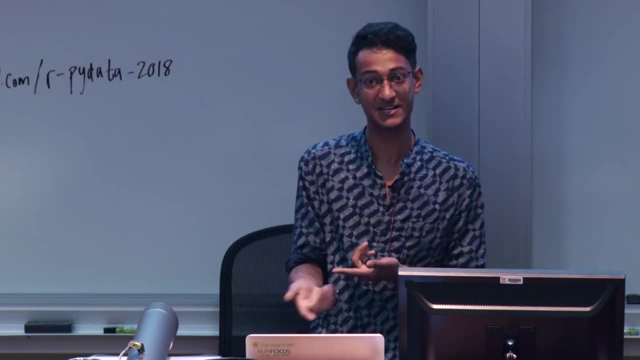 and that's awesome. That just goes to kind of prove my point that you need to do multiple iterations to get very useful results. The text cleaning part, like a lot of the text cleaning, happens after you finish the project, right, Because you're doing it the second time to get better results. 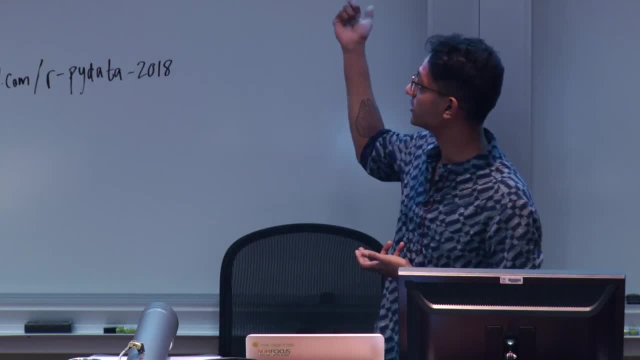 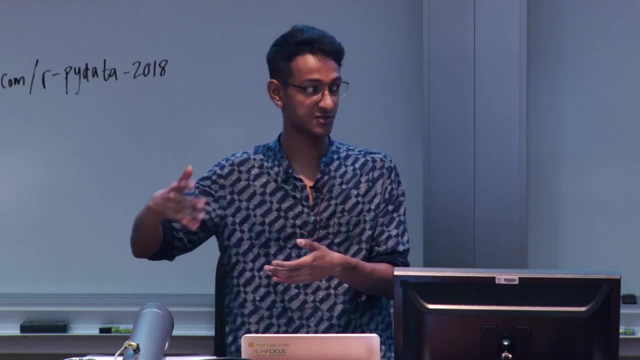 So that's something which you pointed out. Yeah, So, Australia and Australian, you'd argue that it might not be stemming or stemming. So what I would do is I would tell my spaCy model, which, on the spaCy website, you can see how you do this right. 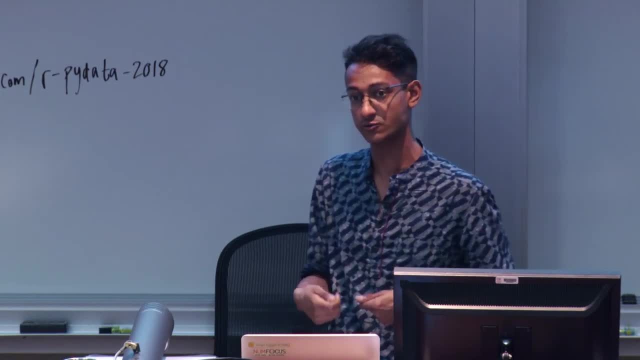 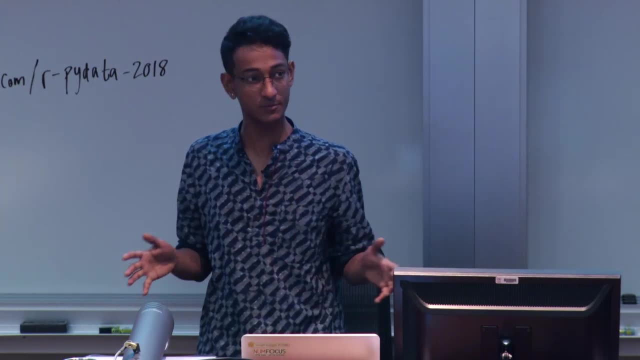 You can tell the model to make exceptions and catch these things and fine-tune your stuff. But yeah, that's a good point. So is everyone kind of clear What topic models are? Are there more questions about topic models? I wouldn't mind talking about topic models a little bit more, but you could also there's 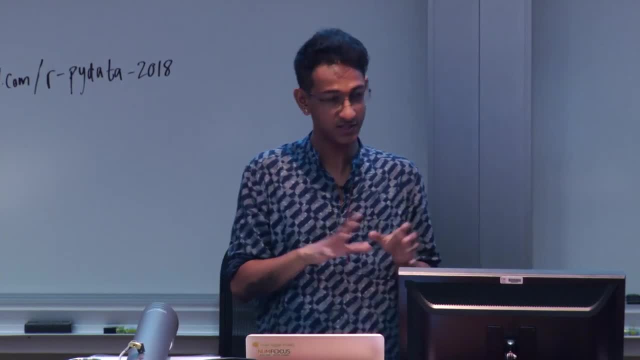 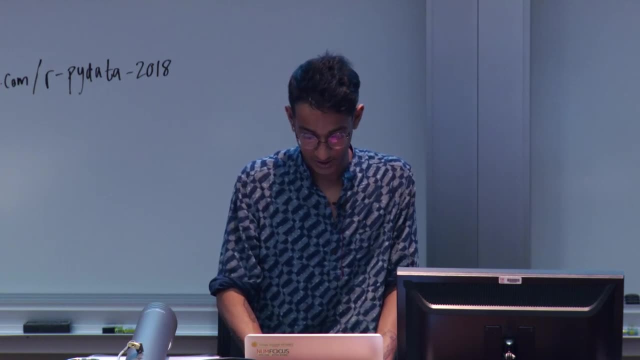 other tutorials in the same repository you can get into more details about, But that's the general idea of topic models and these are one of the things you can do with text. Now I'm going to move on to text classification. So now we're going to stop using yeah, 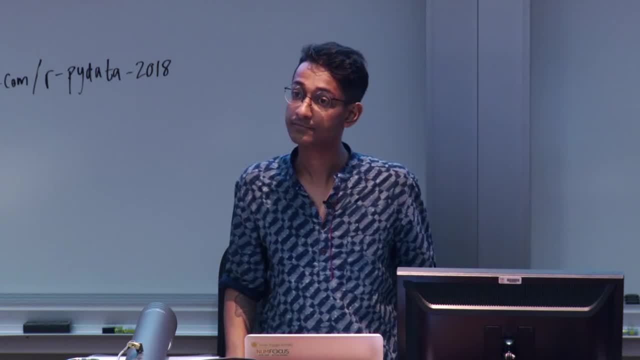 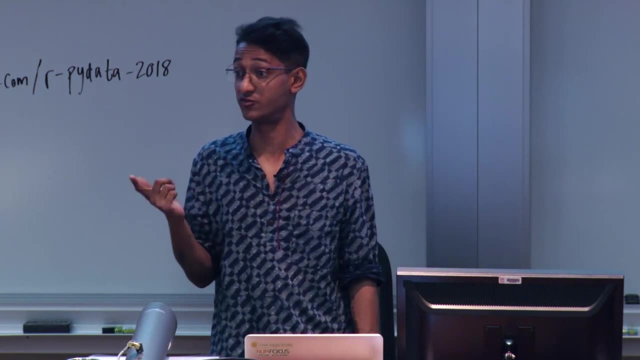 So when you're converting it to a bag of words- architecture- how are you preserving the context of the words? Oh, that's a very good question. So the question is: how are you preserving the context of the words when you're converting it into a bag of words? 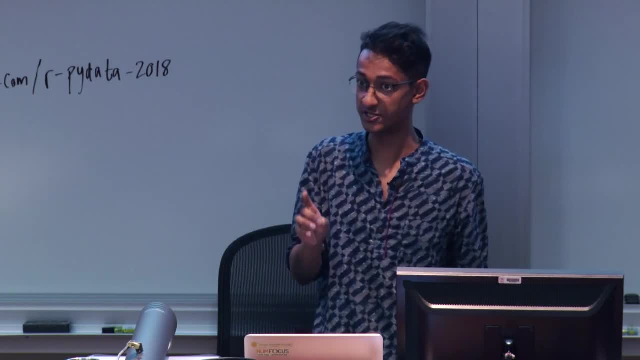 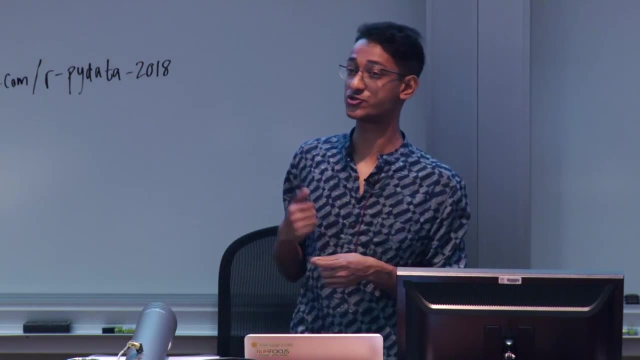 You are not. You are throwing context out the window. That's 100%. So there are, depending on what you so the thing about topic modeling right, for example, or text classification, we don't care so much so about the context of the words, as we care. 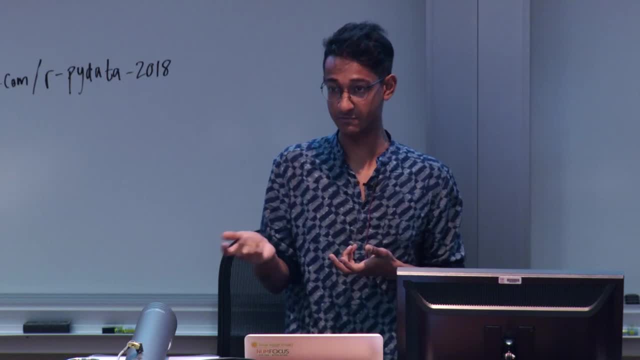 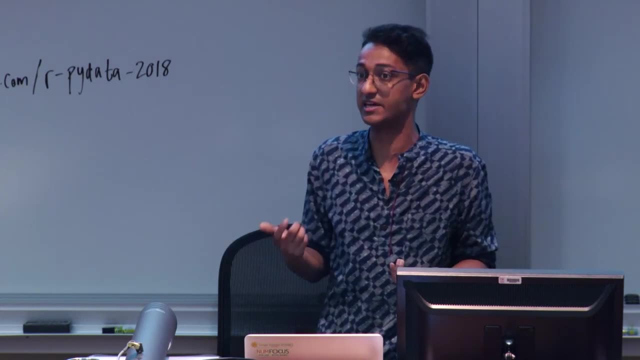 about the presence of these words, Like in spam and not spam, like a popular thing, like if you have like lottery prize winner, so on and so forth. Just the words that they exist is a big giveaway. It's not the most sophisticated way because you're certainly losing context 100%. 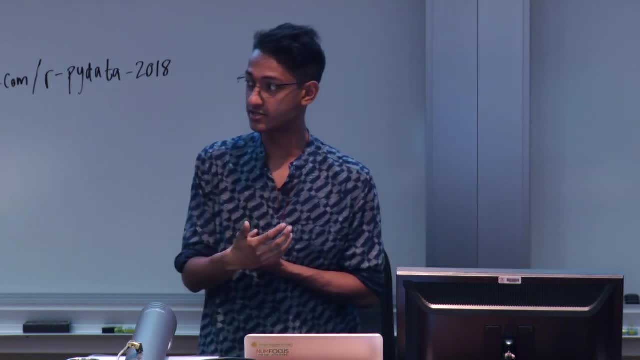 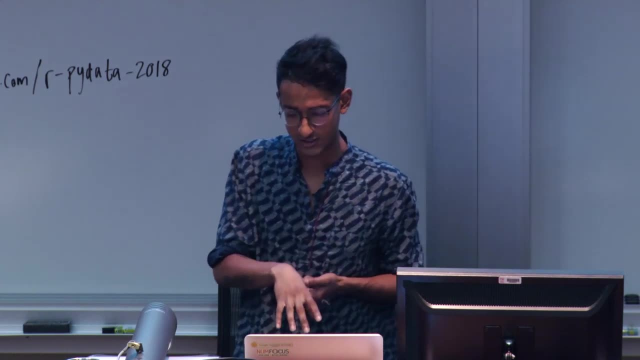 And if you want even better classification which has context, there are ways. there's something called word2vec, which is a way you preserve context, which is also really popularly used in text analysis. I might briefly talk about it later if you have the time. 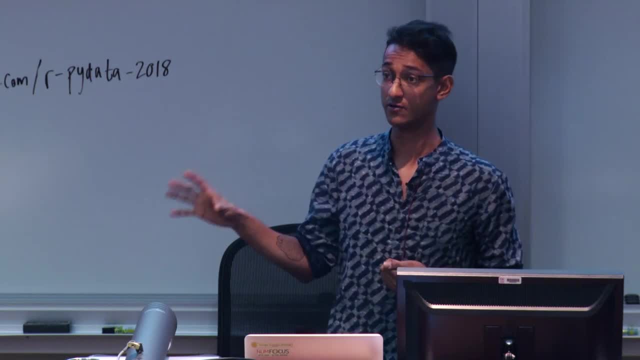 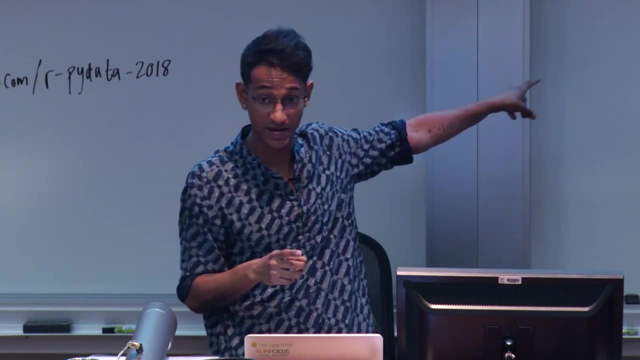 So there are methods you can use to preserve context. It really depends on the kind of project or problem you want to solve. But yeah, Bag of words, And even this original way, it only lets you know if that word exists in that document. 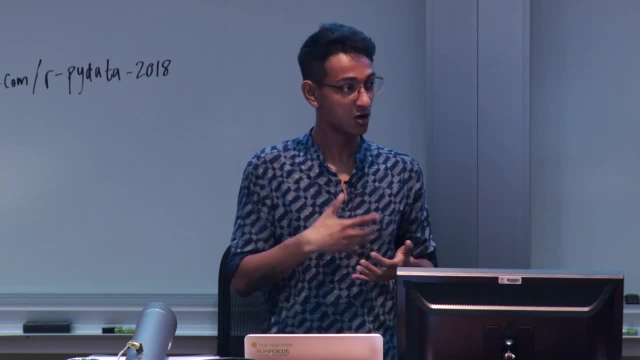 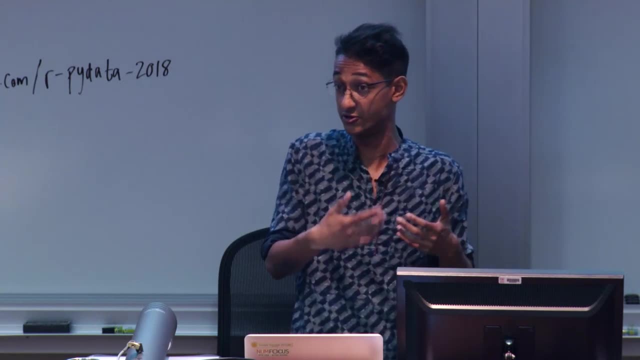 If you want to know the way sentences are structured, semantic meaning or contextual understanding. you have more interesting machine learning algorithms which allow you to do this, And I will actually be very briefly talking about them, And they are now leading the forefront of textual classification. 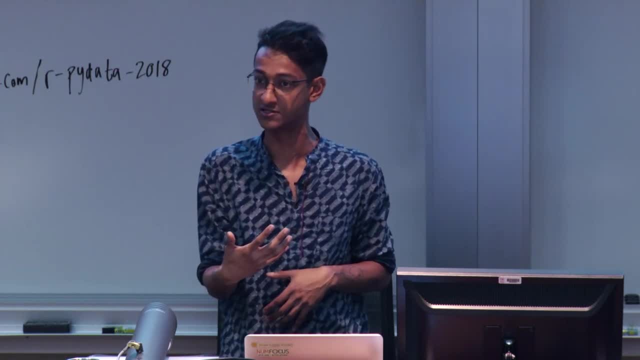 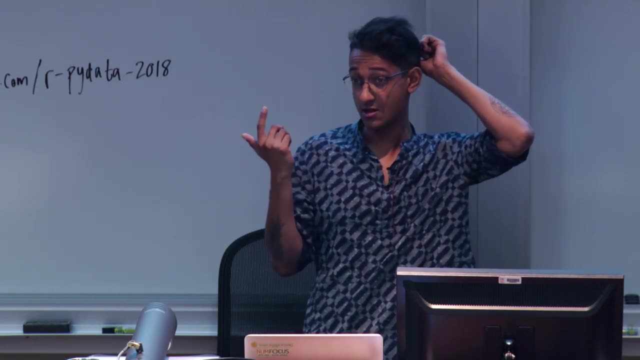 All these things are done using these context-based models which capture this, But for the longest time we didn't have context In 2013 or 2015- was when word2vec came up. I mean, people are trying to solve this context problem for a while. 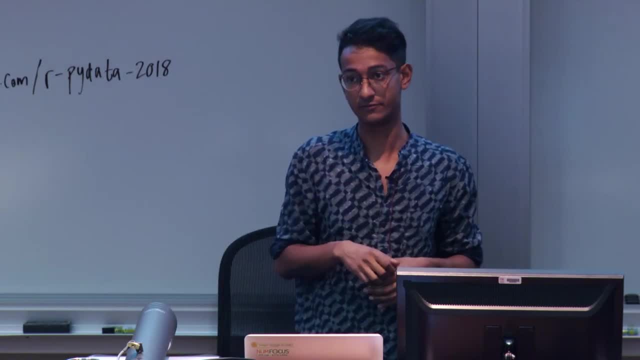 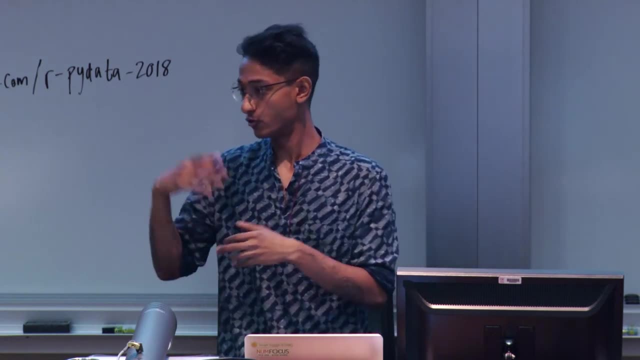 The most sophisticated way was word2vec, which is done by some folks over at Google, where they tried to capture this context which you talk about, And you can later do this as well, But for this talk, we're going to be sticking to this. 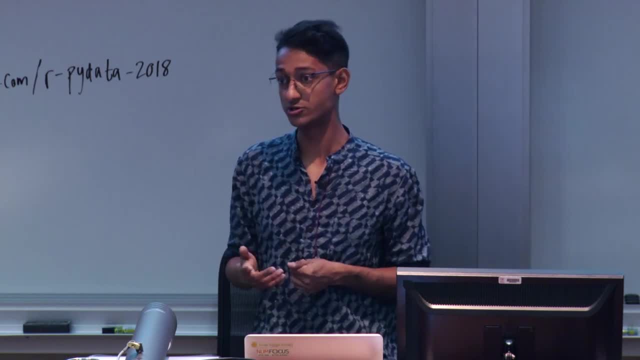 But that is a very good question And if you have more to, you should definitely read about it. Just talk to me about it after this. I would love to. Yeah, You can tell me if this has not been talked about? Yeah, 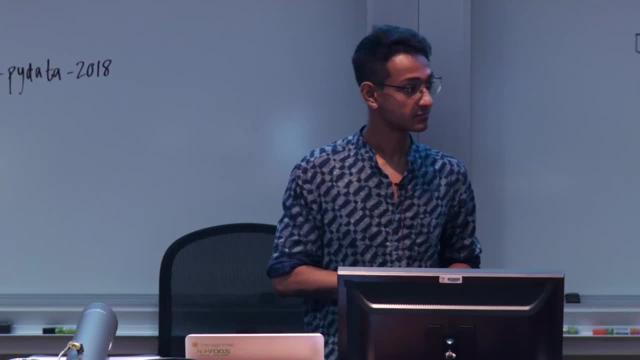 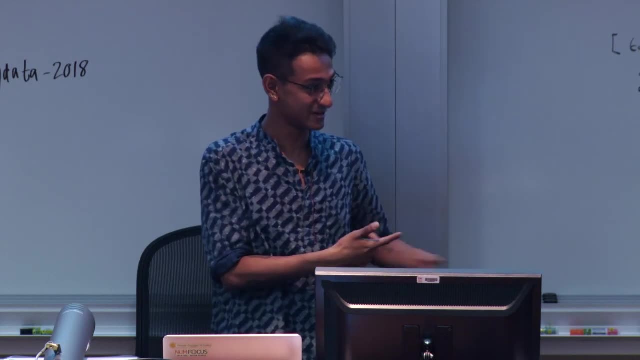 Yeah, Have you looked at LDA2vec yet? Yeah, LDA2vec is super cool. Yeah, Like last year or this year. Yeah, It's very recent. Some gen sim are trying to get that into their package as well. 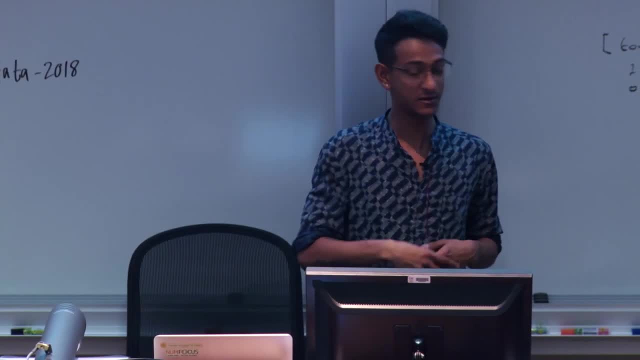 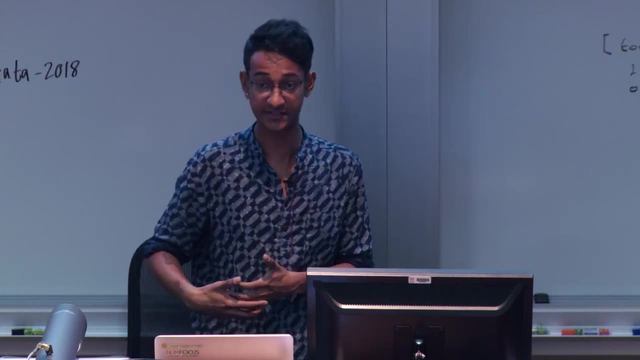 No, I totally dig LDA2vec. It's awesome, But that's so. these are other statistical learning algorithms which also use topic models as part of this context. I mean, there's a lot of things And the whole point of this tutorial is to also just kind of introduce everyone to that. 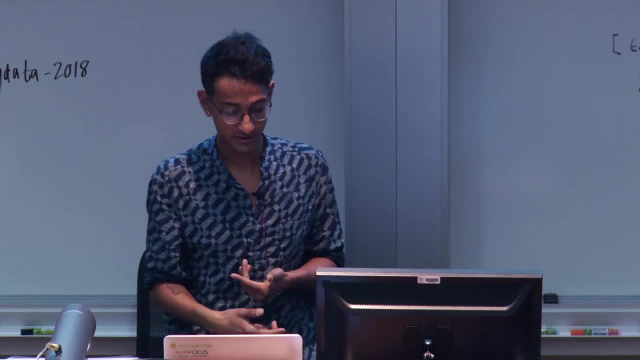 which, and then you can go into more details if you'd like. So I will talk about all of that. I will talk about all of this towards the end, but now I'm going to move on to text classification. Are there any other questions before that? 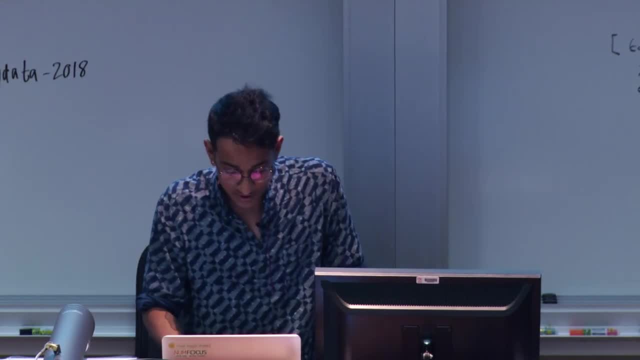 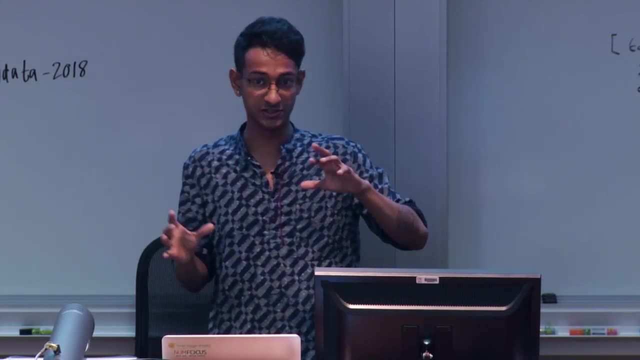 Is that it Okay? Cool. So so far we worked with unlabeled, unstructured data, right, Like we got the data dump of newspaper articles. There was no. we didn't know what it was going to be about. I mean, I knew because I saw it, but the computer had no clue about what it was going to be. 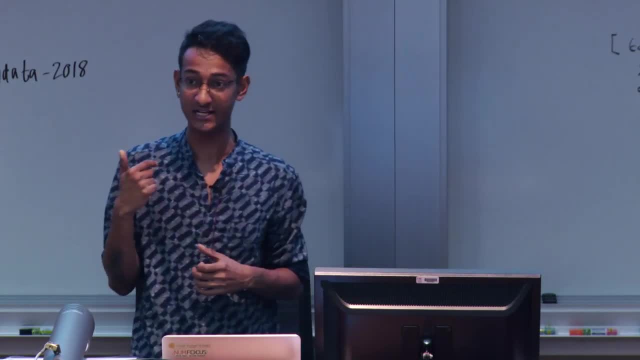 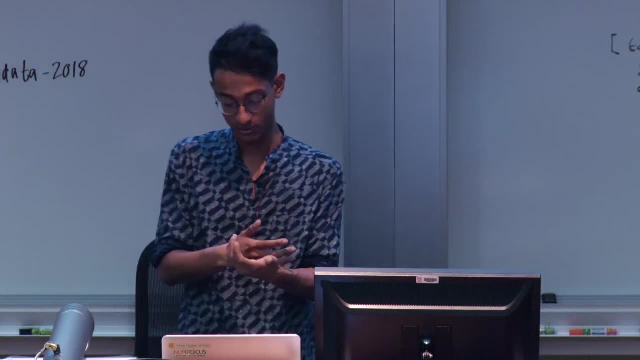 about Now we're going to be dealing with data which is already classified, When you know, for example, I mean there's an interesting project Which I was trying to work on before with a bunch of people back at my university where we're looking at if we can predict if someone has early signs of depression based on looking. 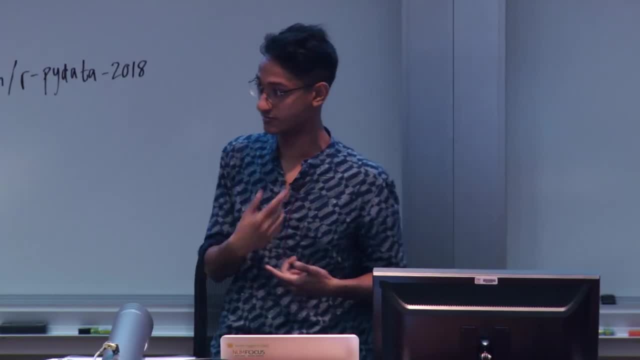 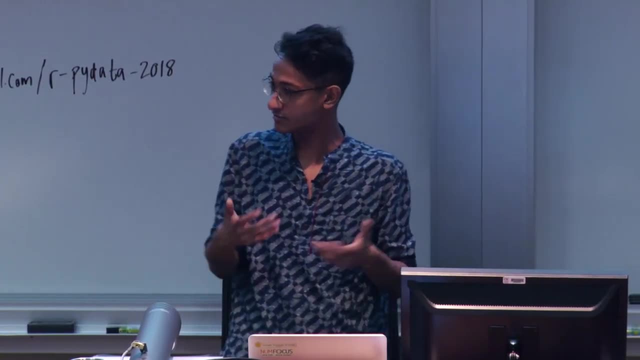 at their social media posts, And this is a particular example where text analysis is super handy, right. So I had data where I knew where certain updates or posts were like, ranked as how depressive they are, so to say, And based on that, I was supposed to tell how depressive or non-depressive other social 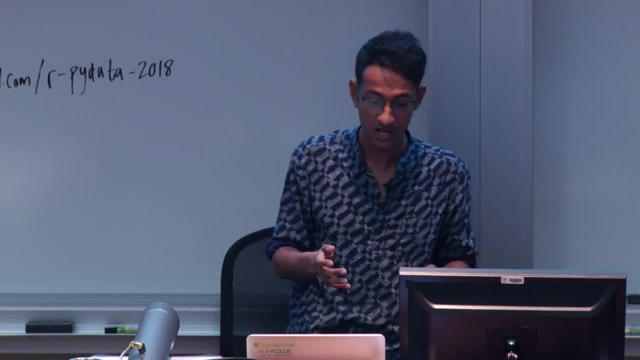 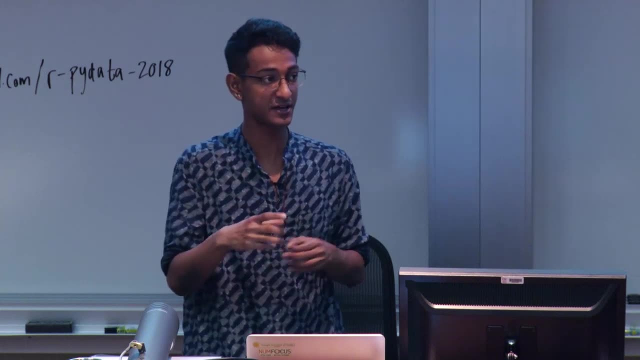 media posts. Again, this is just one context. It could be literally anything right? So in this case, we classify our data before or we annotate our data before. Annotating or classifying basically. annotating actually basically means when you're part. 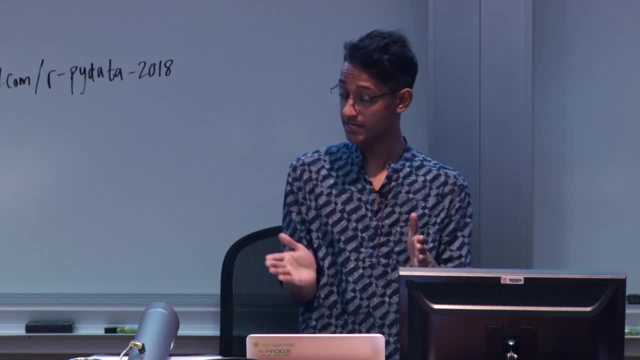 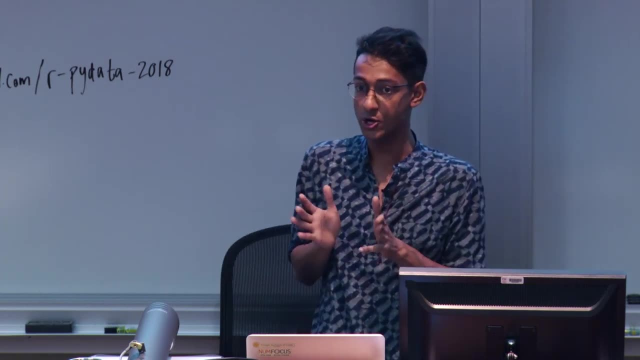 of speech. tagging is also a part of a kind of annotation. It's when you tell your data what it is before you do any kind of classification task. when you mark it, label or annotate it, the computer knows your machine learning algorithm knows what kind of data labels you're dealing with. 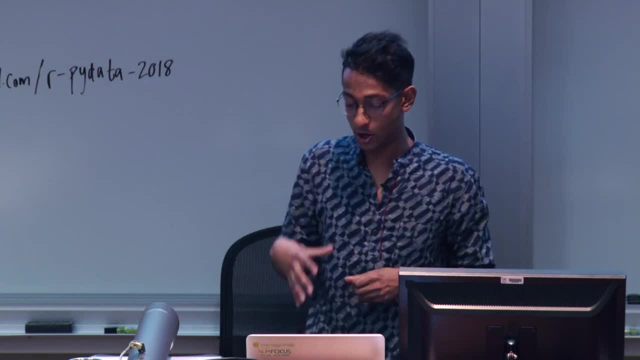 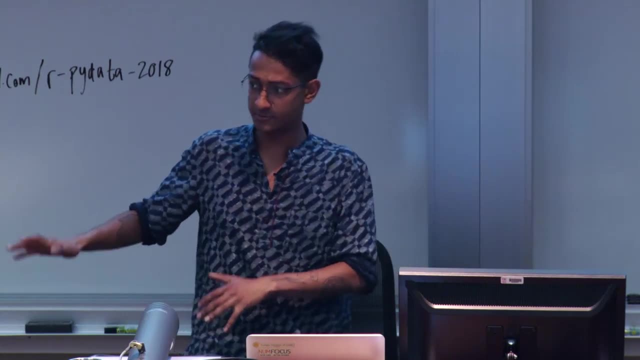 It's just also called labeling your data. So we're going to be looking at now problems where we have labels on our data And most usually, when you're lucky, you have some kind of labels. You want to get a percentage of accuracy. 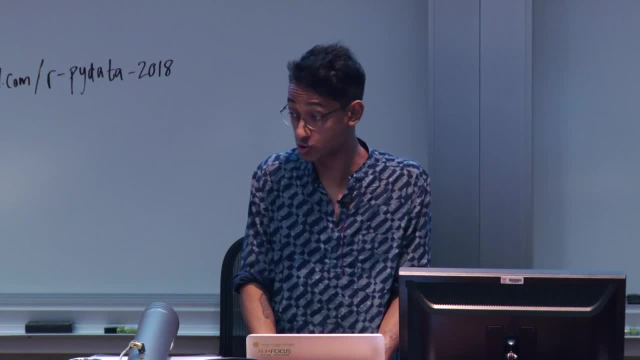 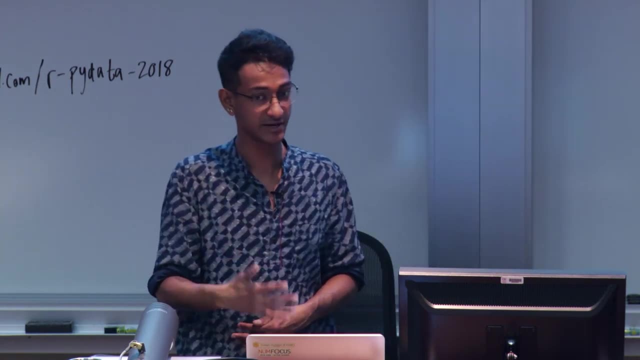 So this is called classification problems or supervised learning. Supervised because you're giving labels or annotations. What we did before was unsupervised because we didn't really apart from the number of topics, but it's still called unsupervised and this is called supervised. 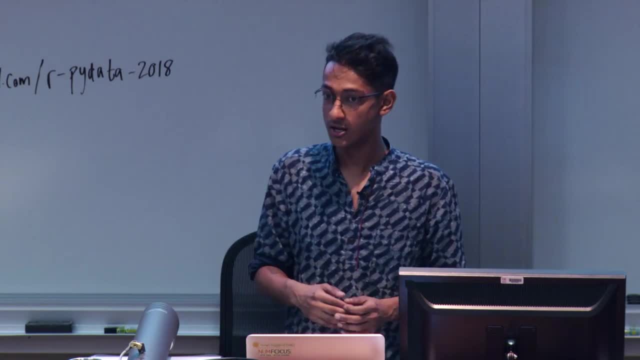 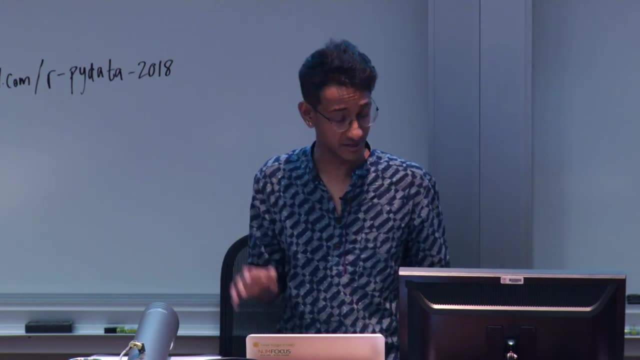 Now I'm going to be going over this part a lot faster, because it's the idea. it's just to again let you know what's available, right? If you want me to slow down, though, please let me know and I will go slow, but it's also. 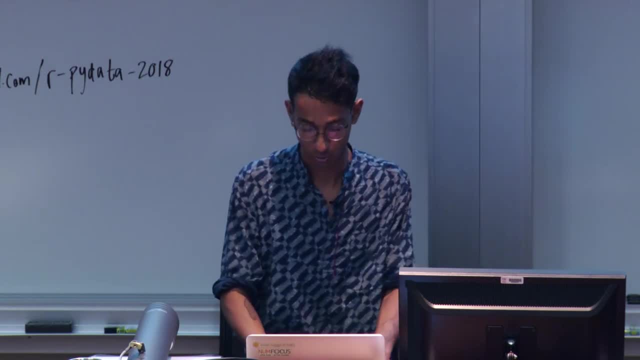 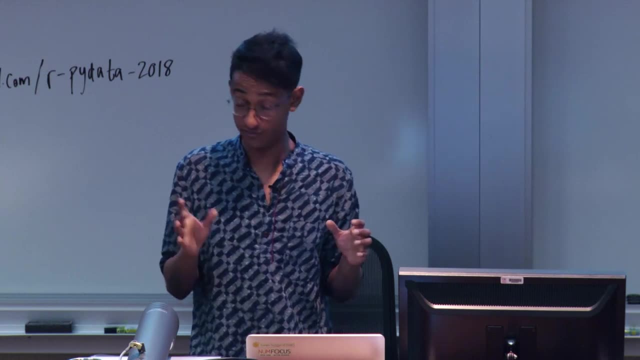 the last 25 minutes, So I'm going to kind of up the pace over here. So a bunch of imports over here. All these imports are to get our data set ready and we're going to be using scikit-learn now. 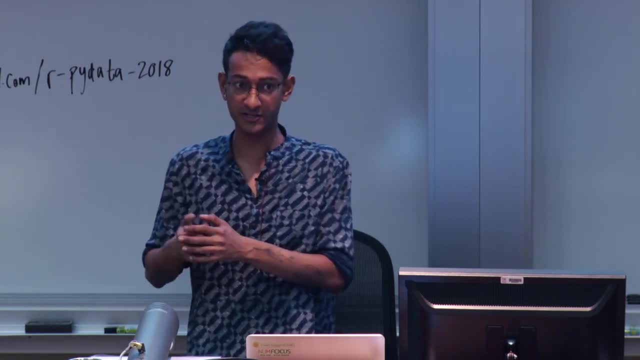 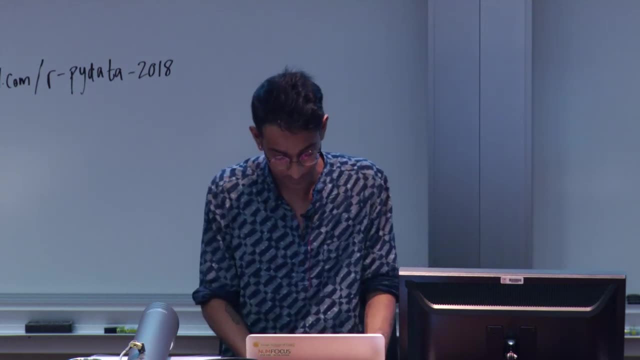 And we're going to move. I'm moving away from Gensim and going to scikit-learn, because scikit-learn is very popular in machine learning and it also has a lot of cool tech stuff, which is what I want to introduce everyone to. 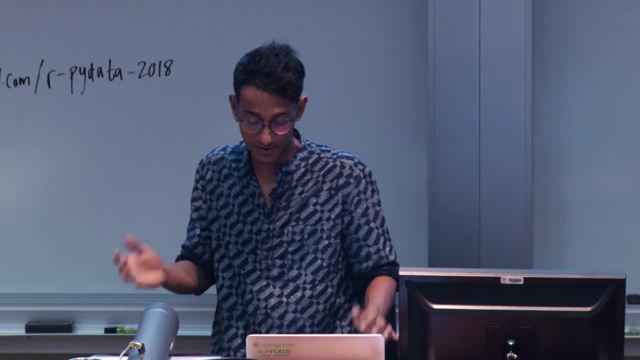 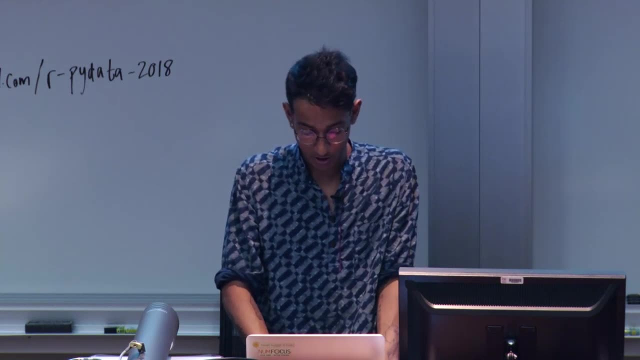 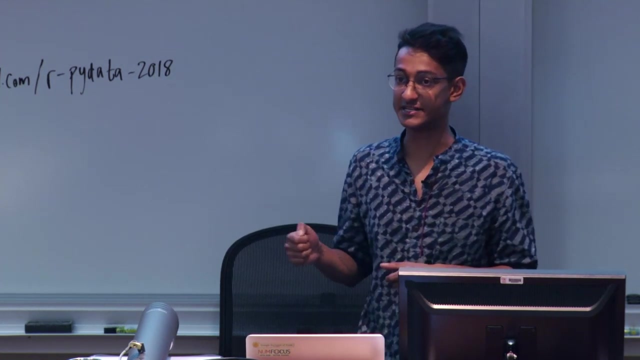 So I'm going to do some things for feature extraction, which is tf id vector, blah, blah blah. bunch of imports, Basically a lot of imports, but we need these and I will explain why. Now, what I'm going to be doing in this particular cell is data transformations and getting my 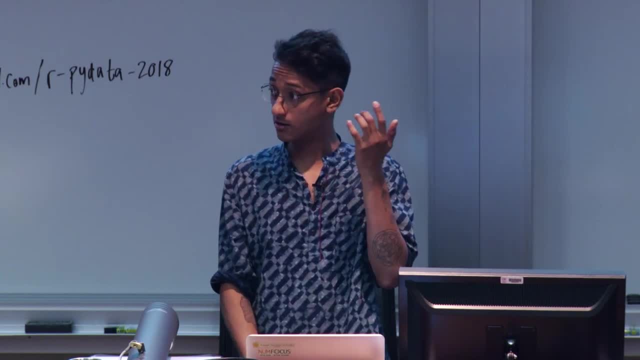 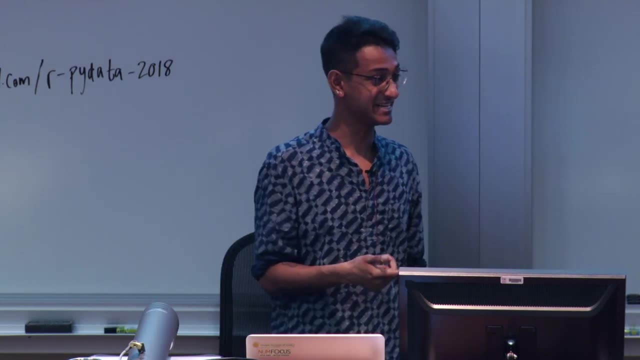 data. Now what I talked about. we're going to be also switching data sets. so we're going out of our Australian newspaper corpus, right? So now it's going to. we're going to be using something called the 20NG data set. 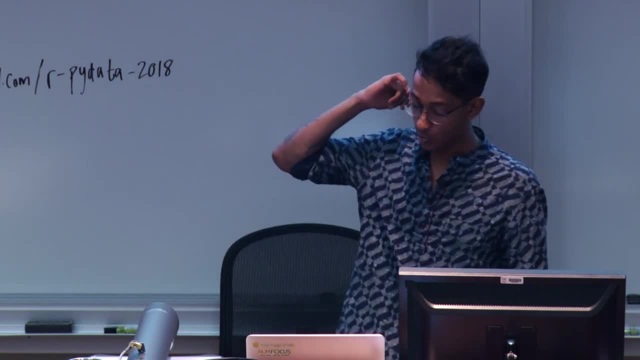 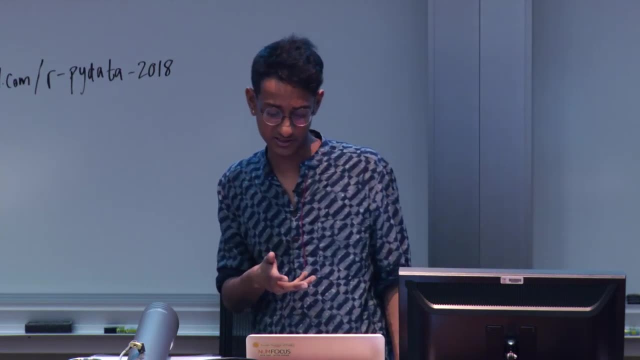 Our 20 newsgroups data set. There are 20 categories. We're only going to be using four of these 20 categories, which are? these are random, but two of them are about religion, one is on graphics, one is space. 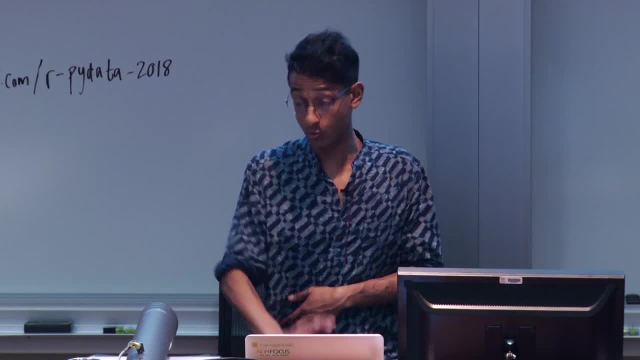 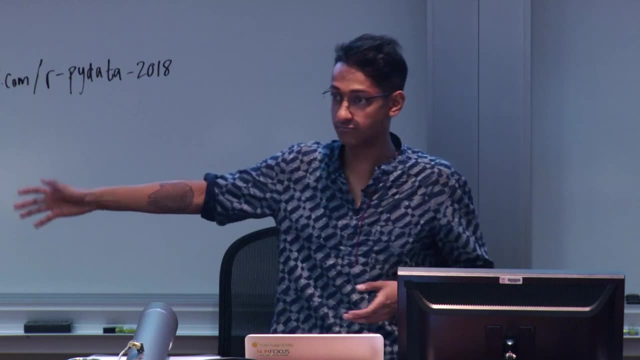 I just picked the first four, I think. So we're not going to be doing classification for all 20.. We're going to be doing four. That's again for this particular example. You would have complex tasks with 20 or even more labels. 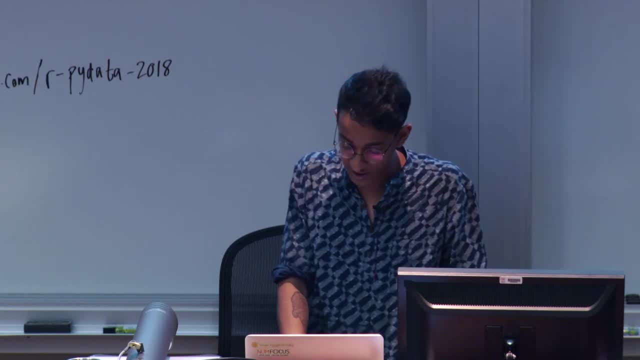 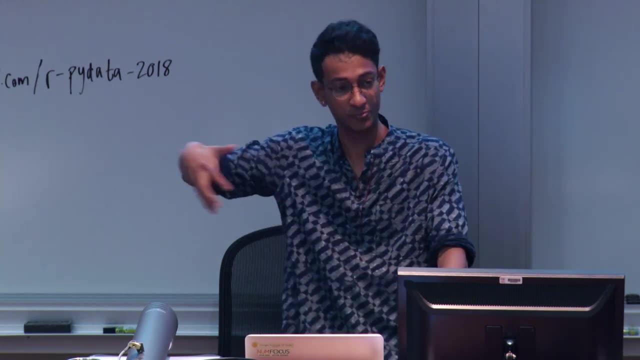 For this one, we're just using four because it's faster. So data train. So in these kind of cases You have, you are training- a model which you are then using to predict right. That's a kind of different kind of paradigm than what we dealt with before. 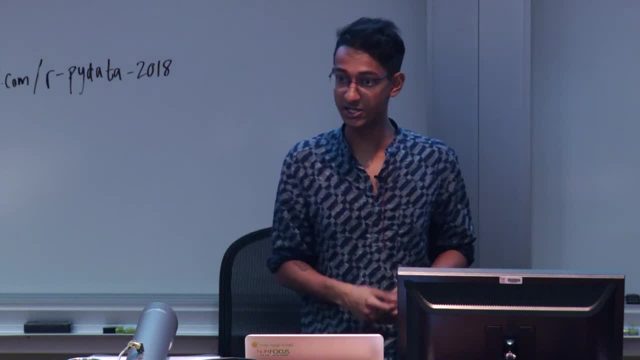 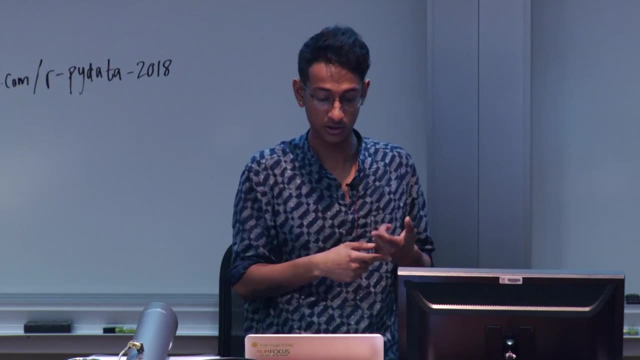 Previously we were just, you know, kind of getting information about our data. Now we're going to actually train a machine learning model based on what we saw and classify into a particular class based on that model. If any of these words are not making sense, stop me, but I will explain them in a wee bit. 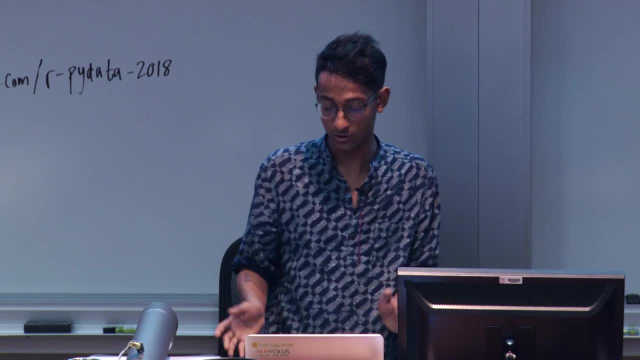 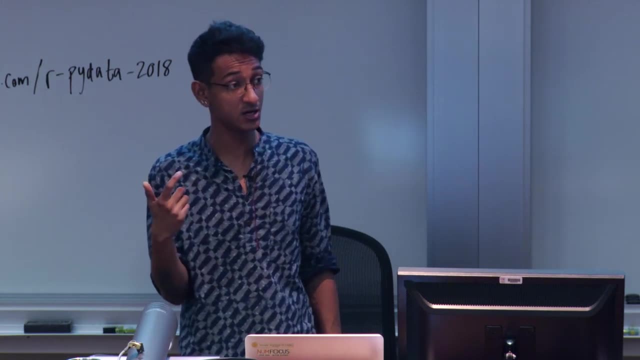 So you have data train, which is a variable. So fetch 20 news groups, Basically fetch this data, which is just a function of my scikit-learn. The subset is only train, so I'm only getting my training data. 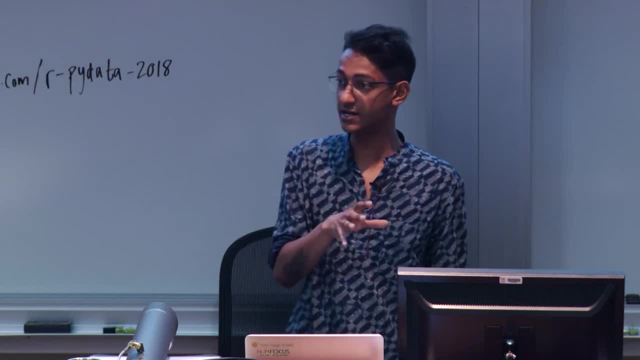 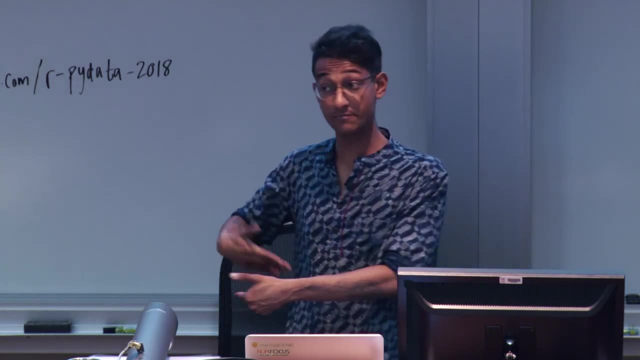 Training data is labeled data right. That's very important. Any kind of data which you're using to train a model on is like already has labels or annotations. We're going to be learning from these annotations and this data to make new predictions or new labels for unseen documents. 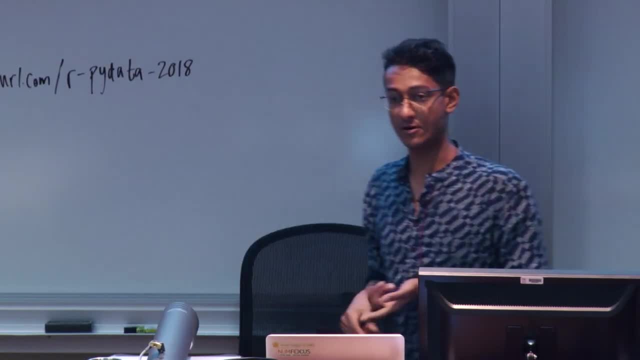 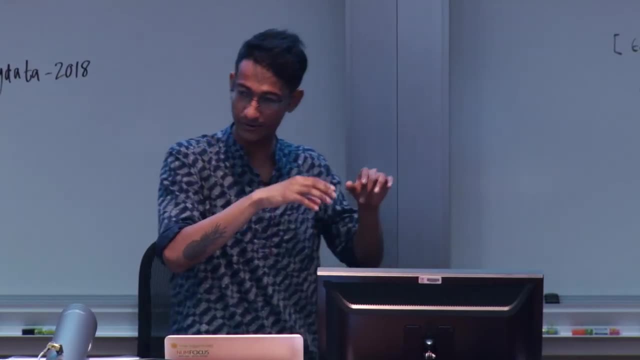 So now the other thing. So I previously talked about bag of words. right, And that's fine. That's one way to represent your textual data. Now we're going to be. That was also kind of manual, where we kind of created that using Jensen. 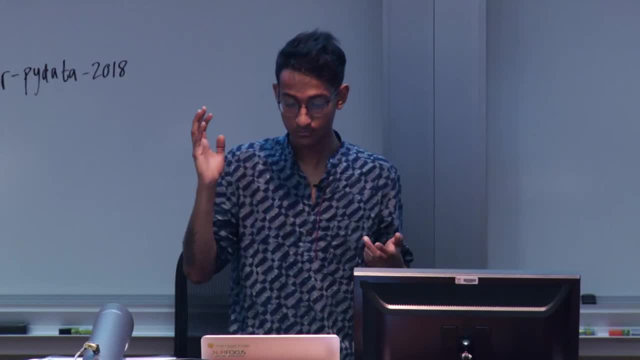 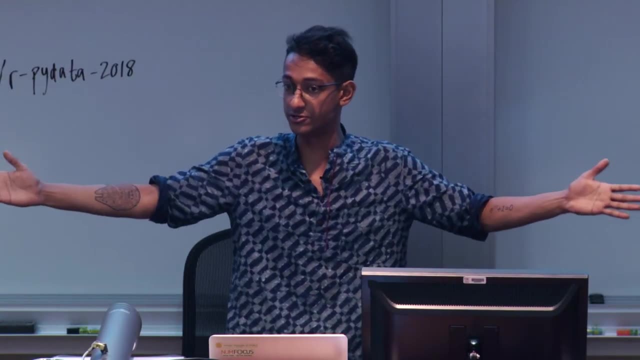 Now I'm going to show you how scikit-learn does this. So now I'm going to say I don't want bag of words, I want to make it even more sparse. I want to use five In this case five. 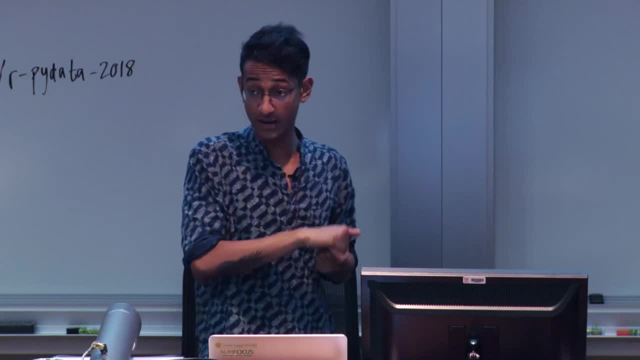 I mean, I just chose five. It could be anything right. So again we have a vocabulary. Last case was 5,300 and something. This time it would probably be around that as well. I don't want to use the entire vocabulary. 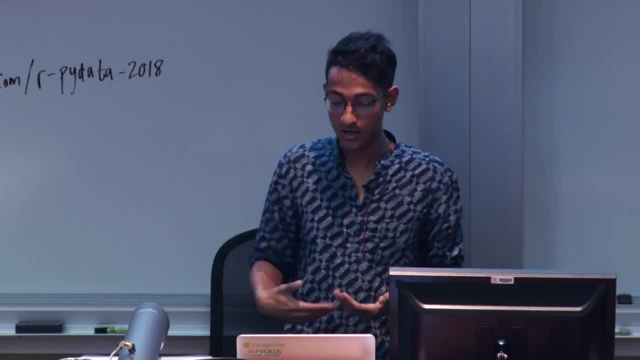 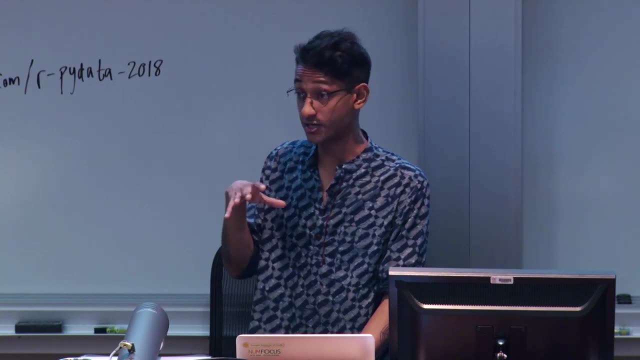 I want to train it on a smaller part of it, So I'm going to Here: the number of components is five And I am training. I'm basically transforming my data. Now, what does this mean? Previously we also did this, actually. 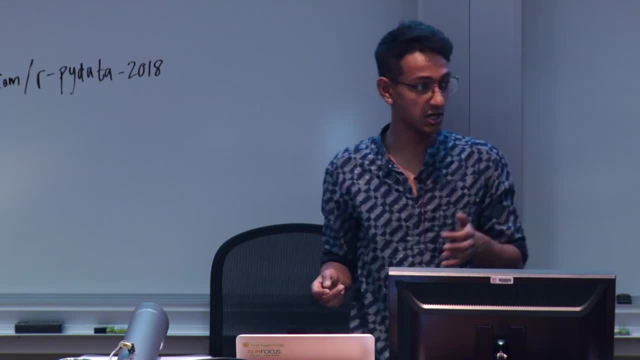 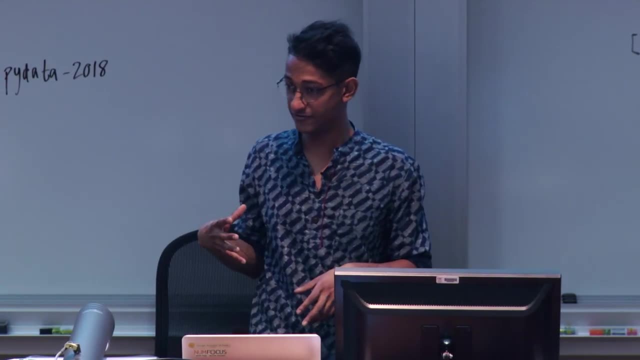 When we transformed our data from our raw textual data to our bag of words, and this part what I showed you before. Now we're going to be transforming our data into something called TF-IDF, which stands for term frequency, inverse document frequency. 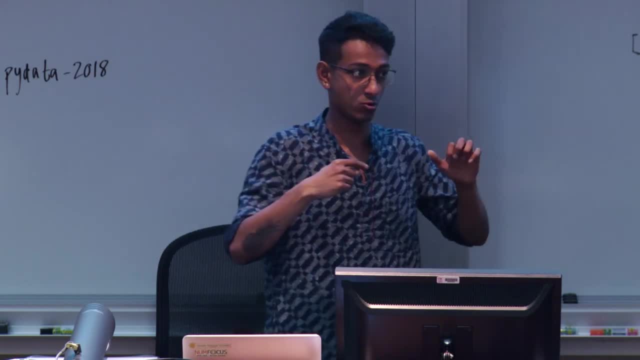 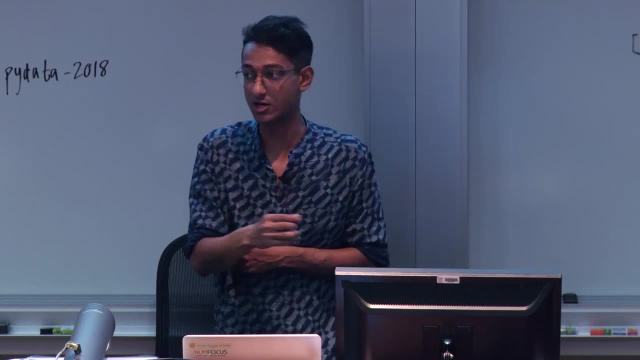 It's what it stands for. The idea is you want to get words which are appearing a whole lot of times in a lot of documents, but not in every document, So it's called inverse document. I'm not going to get into the math part of it right now. 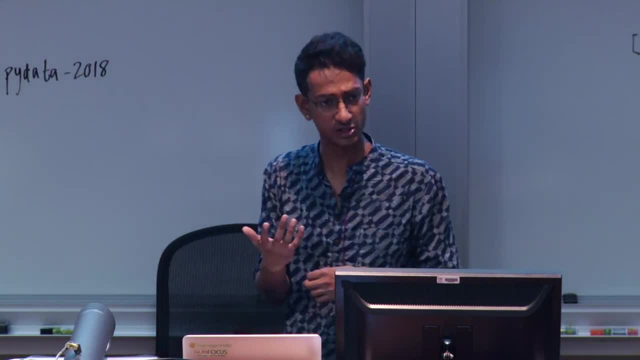 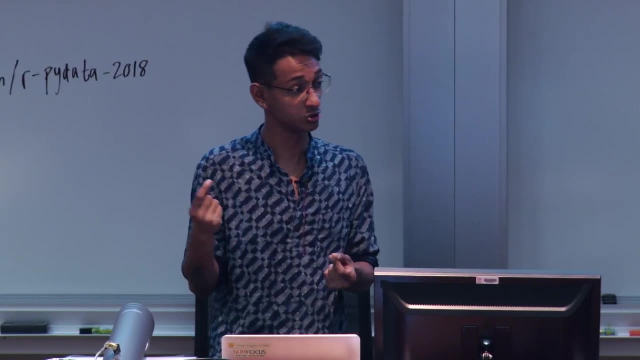 If you are interested again, you can search it up. It's really popular in text analysis terms. It's basically like a bag of words. It's a way of representing your textual data. So that's why you have TF-IDF vectorizer training on transforming. 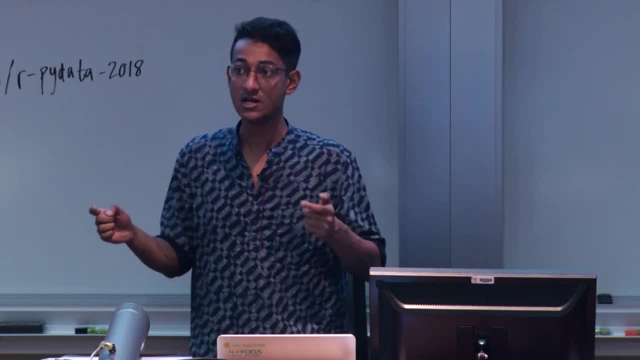 Even after I do this, there's still a lot of words in my vocabulary. So now what I want to do is I want to reduce the number of dimensions. There's a lot of ways you can reduce the number of dimensions of something. 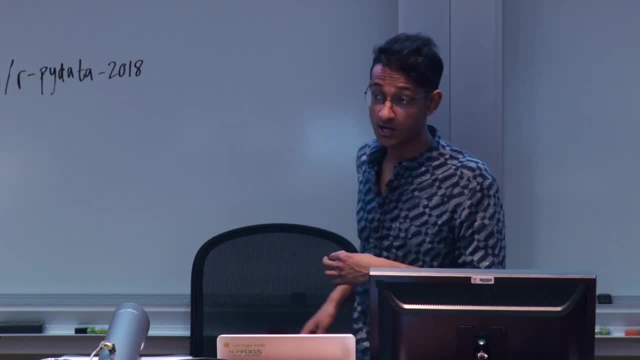 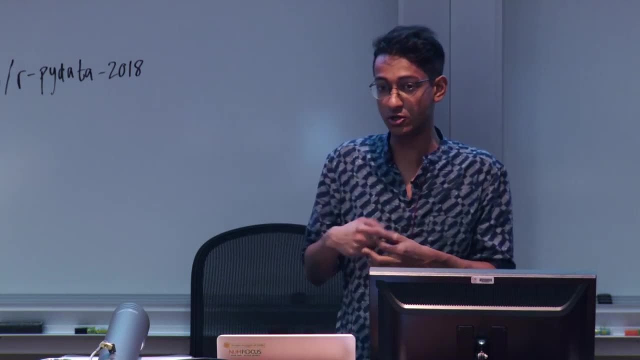 This just means 10,000 dimensions over here. I want to reduce that to 4 or 5 or something which is easier for a computer to understand. Here. that's SVD, or it's called So. SVD is basically a vector decomposition singular vector. 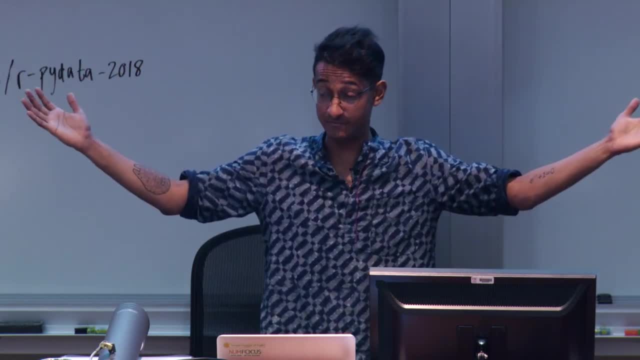 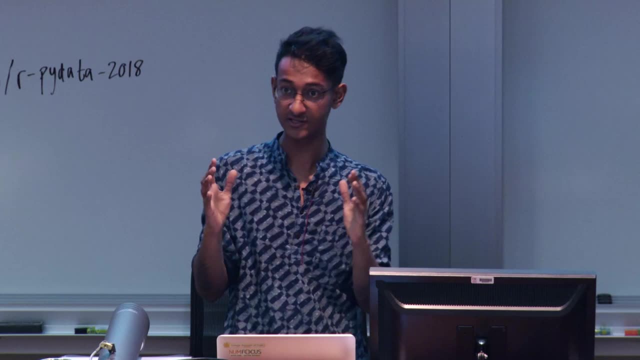 So it's a kind of decomposition, where you have a massive matrix. Now all of these, when you have a lot of documents, becomes a really massive matrix, right, When you want to reduce this to a small number of dimensions, use different kinds of machine learning or linear algebra methods to do this. 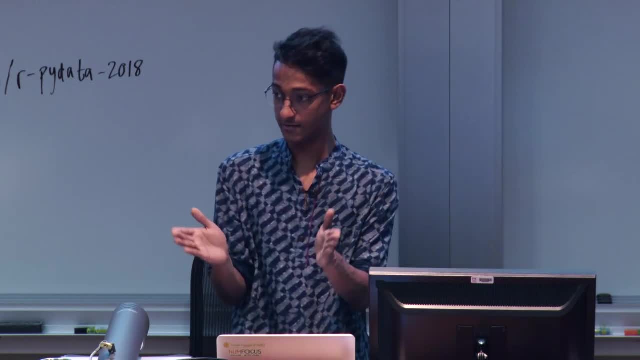 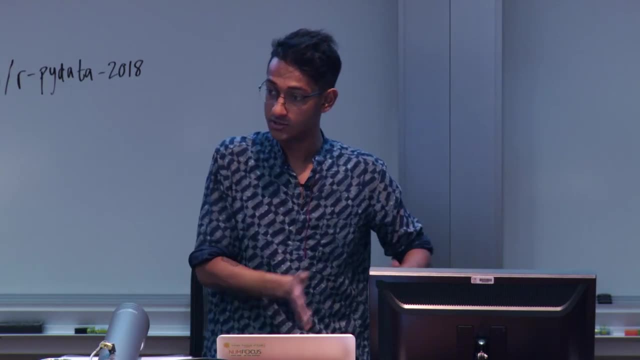 One way is SVD, So SVD. So these are Again. I just want to introduce you all to different ways in which you can normalize your data or basically make a huge vocabulary smaller. So what we're doing now is we are 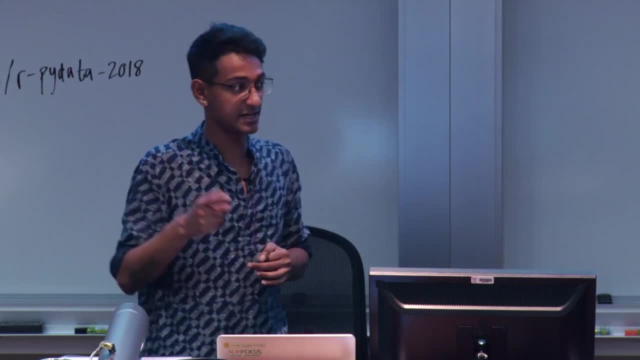 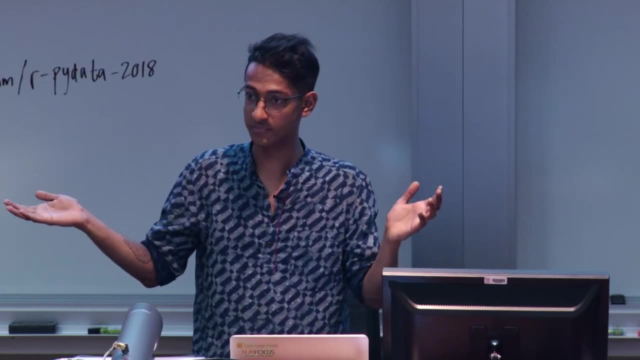 So LSA is latent semantic analysis. All of these are basically. The idea is: have a lot of words, A lot of words are going to be kind of complicated in classification, So let's lower our dimensions into something we can use better. 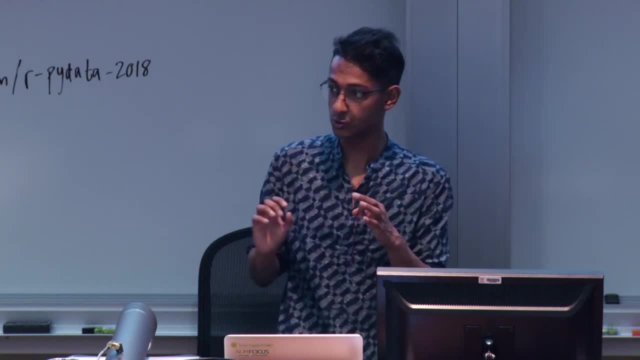 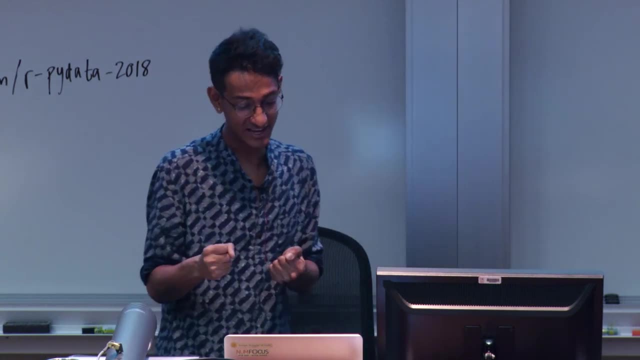 And in this case it's TF, IDF and SVD. I also want to just kind of throw a lot of words at you all so you can later go and Google it and then be like: wow, I learned all this cool stuff. 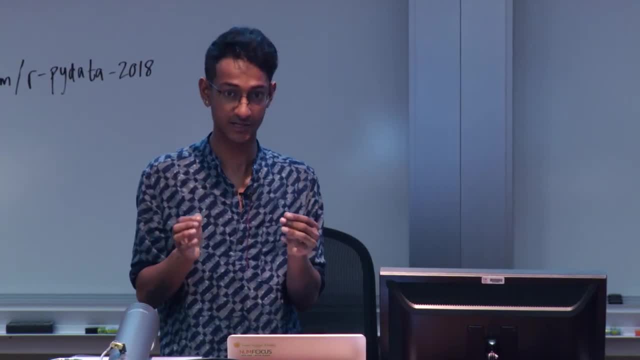 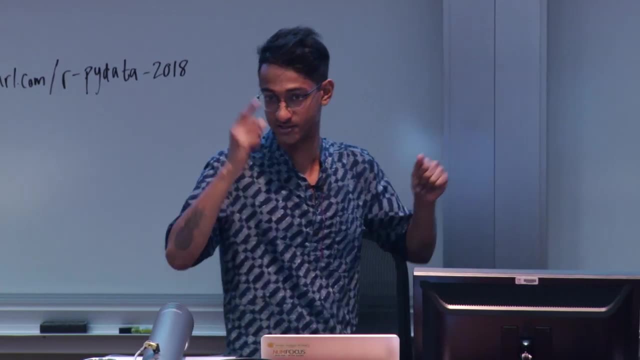 But the idea is to lower. The idea is to lower your number of dimensions. That is the core idea of this. The reason why we do it is, again like I talked about before. these are a lot of dimensions Here. dimensions is the features. 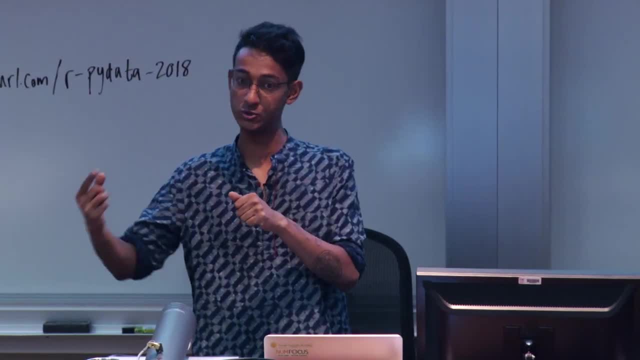 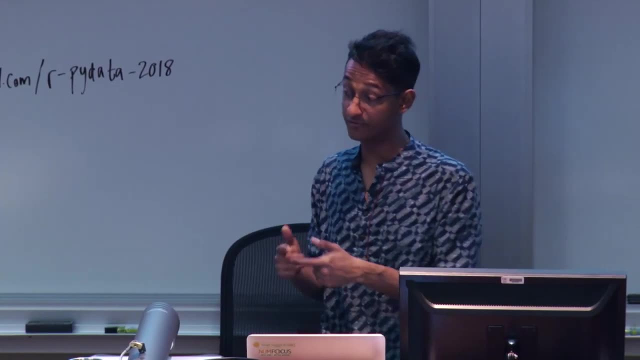 Dimensions are basically the number of things you are using to make a prediction or train a model. right Now I'm doing the same thing, but I'm doing it for my testing data. Before this, it was my training data. Remember, we have classification now, which means it's supervised. 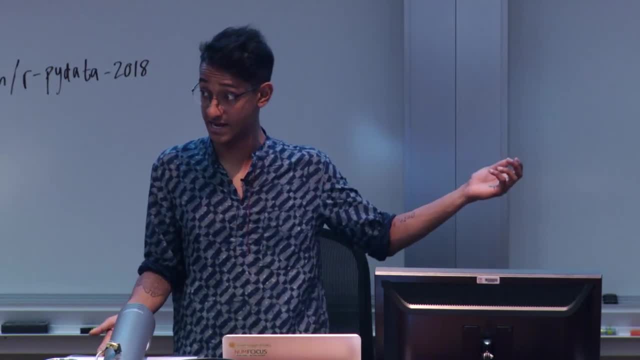 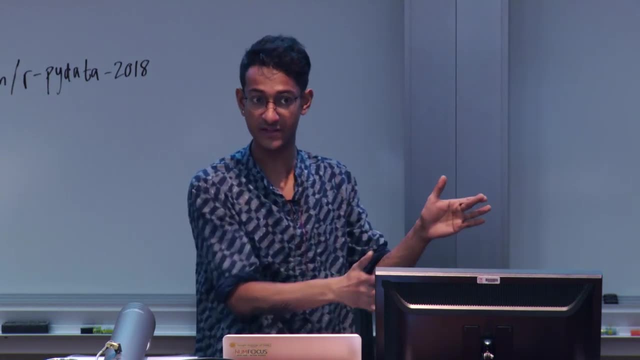 which means we have training and testing and things like this which we did not have before with topic models. So we train our, We create our model by training on certain kind of data and then we see how good this model is by testing it on test data, right. 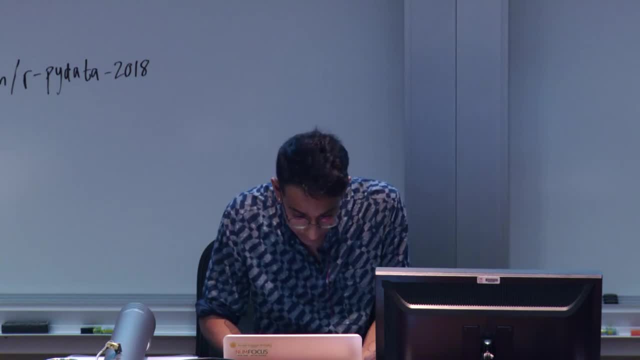 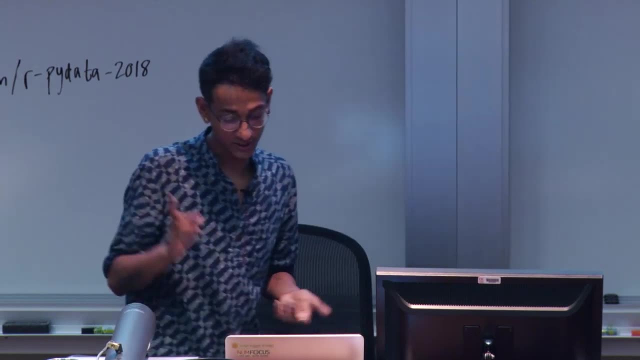 So you can see over here like: so scikit-learn offers. I'm sorry I didn't run this. I panicked there for a bit. There we go, So that happened really fast. Also, scikit-learn offers really nice tutorials. 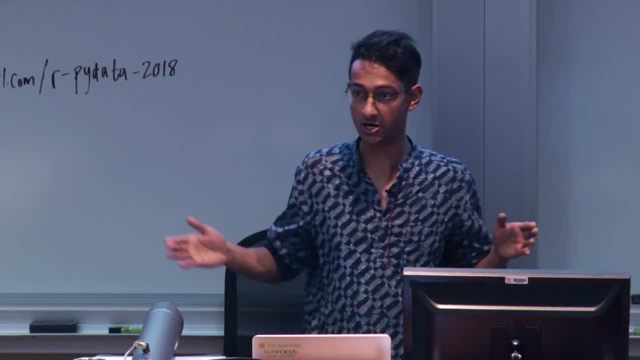 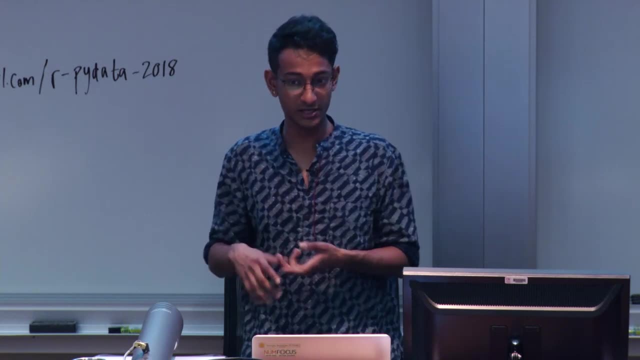 on what exactly is going on within this. It's out of the context for me to talk. It's out of the context of this drill for me to talk about how exactly the data reduction- dimension reduction- is going on. I would really recommend Googling it and finding out more about it. 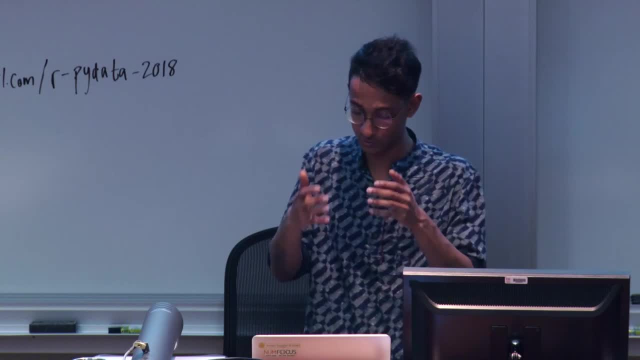 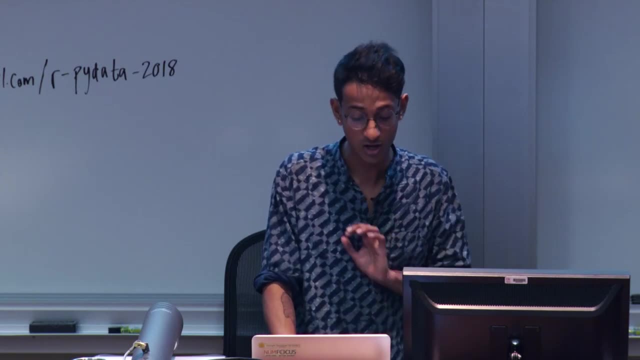 because it's a pretty important idea. But since we're sticking to text analysis, I'm going to move on. So now we created our training and testing set Again. these two cells have a lot of code. Take your time to go through it in the documentation later. 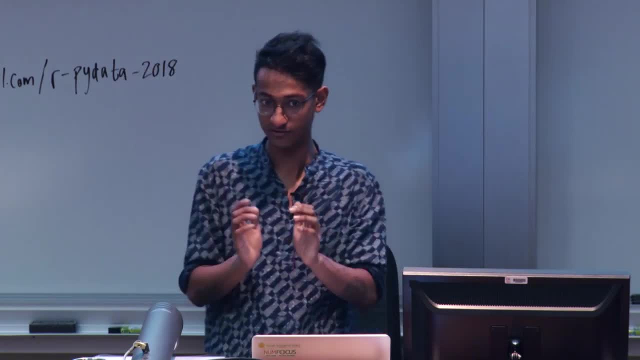 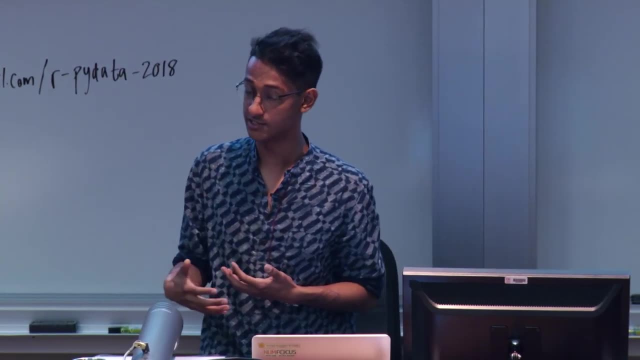 so you know what exactly is going on. What you need to know is a lot of dimensions, less dimensions. data is not ready. So what exactly are we doing? There are many different kinds of machines. There are many machine learning algorithms which we can use to classify data. 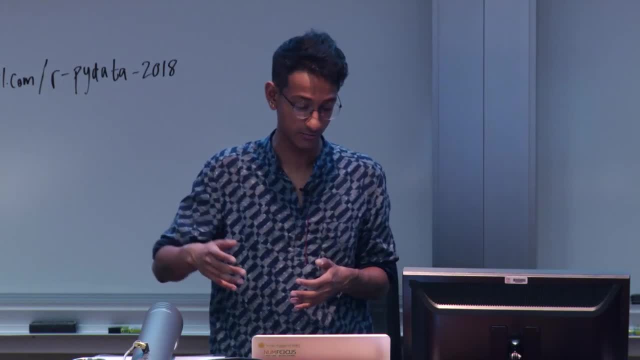 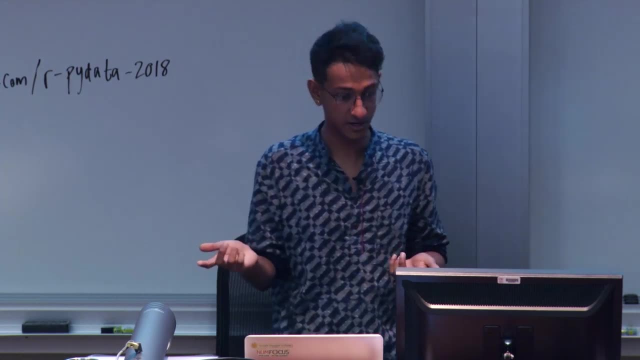 What we used before. topic models are also a suite of probabilistic or machine learning models, but that was not classification. Classification, like I said before, you know a label, you make a prediction like the spam and not spam thing. 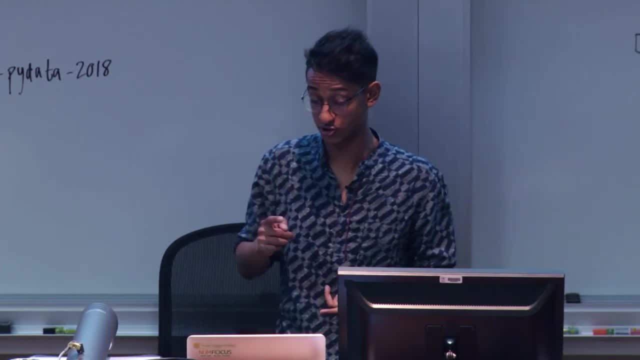 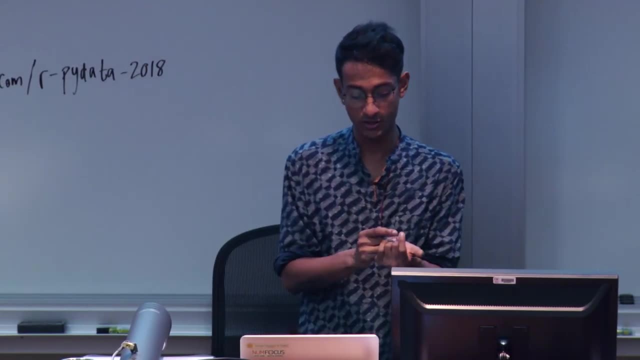 Even for spam and not spam. the earliest spam identification models were usually something called Gaussian Naive Bayes, which is basically a classification. It's a classification algorithm where it looks at: oh, these kind of words end up appearing- which have spam. 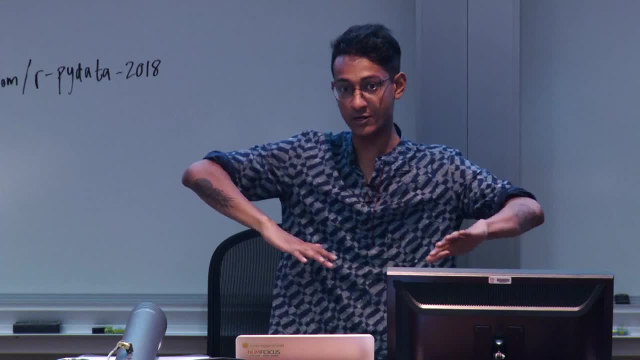 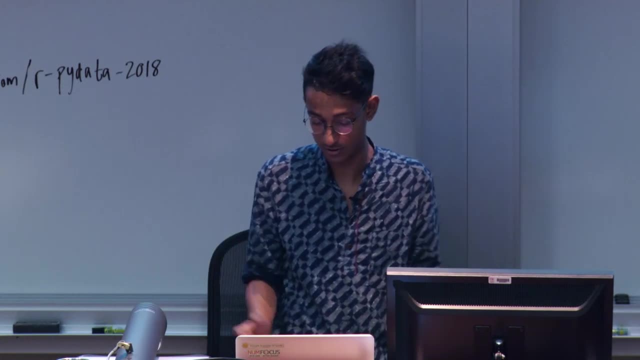 So these kind of words are probably more spammy words. So that's how it does it under the hood, right In a probabilistic manner. by looking at each word and adjusting these probabilities, We're just going to do import Gaussian NB, which makes your life a lot easier. 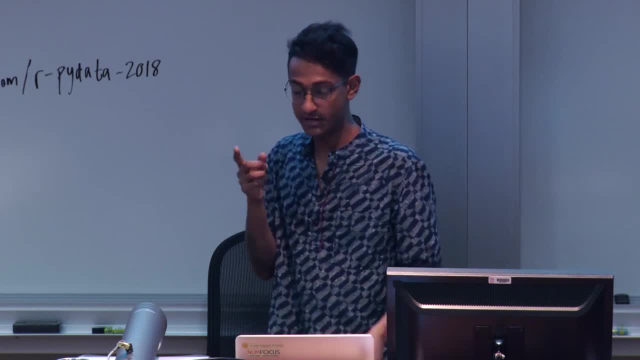 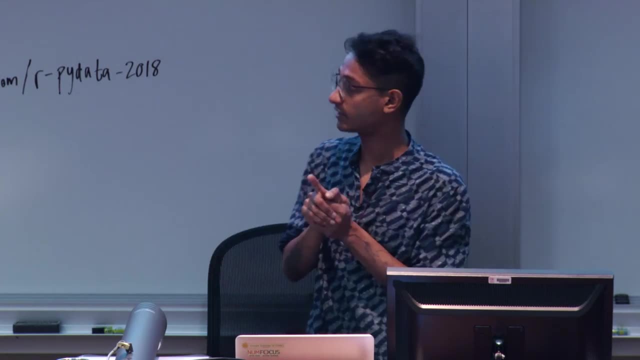 And we train these models. Now I've done: GNB is equal to Gaussian NB, which is our model. Then I've done GNBfit: predict What exactly is going on. I am fitting my model. This could also be in two lines. 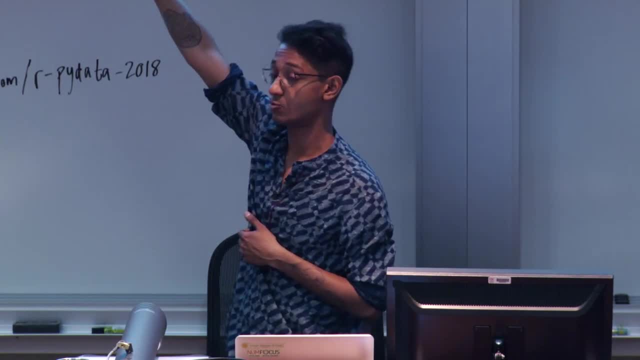 I'm just doing it in one line over here, But I'm fitting my model using my X-train and Y-train. X-train is my data, Y-train is the label for the data. I've talked about labels before. 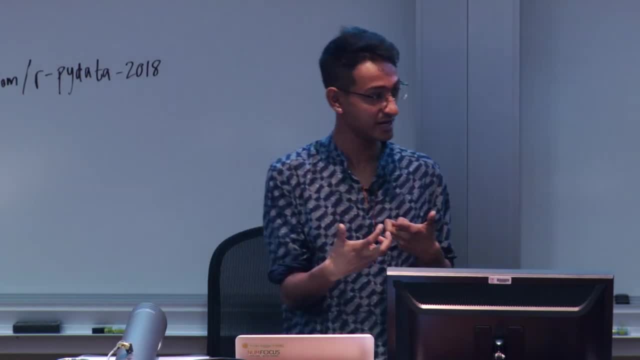 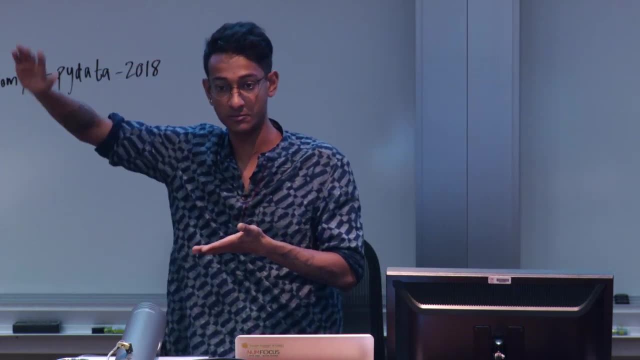 And now, once I fit my model Here, fit is training. I'm now creating my model And once I'm done training or fitting my model, it's fit because it fits it according to the probabilistic thing, And then after that it's predict. 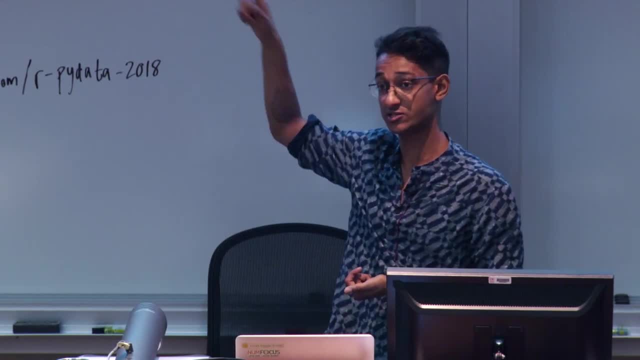 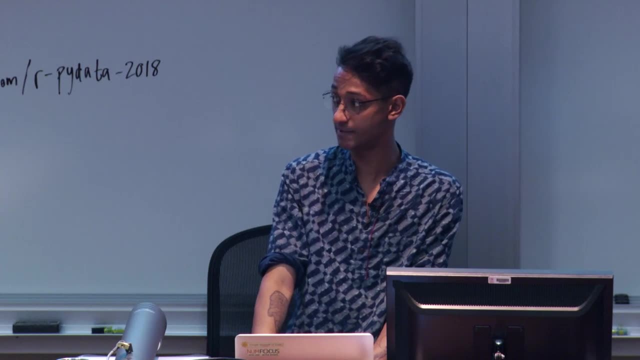 which means I'm making a prediction on X-test, which is my testing data. So Y-pred NB would be the prediction which my machine learning model has made on the test data And you can see it's a 0, 3.. 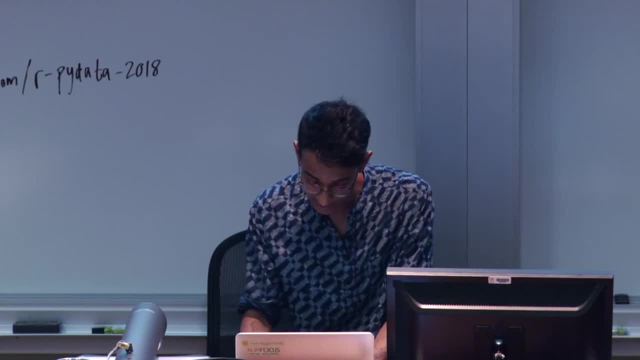 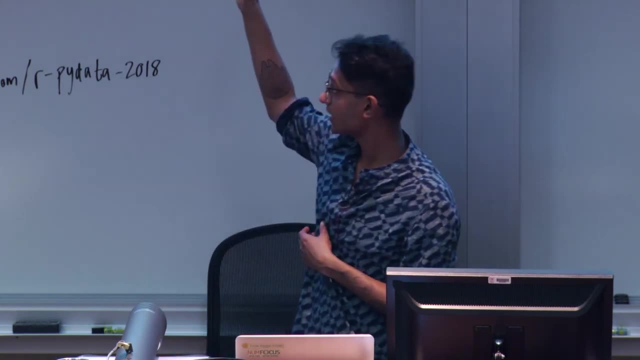 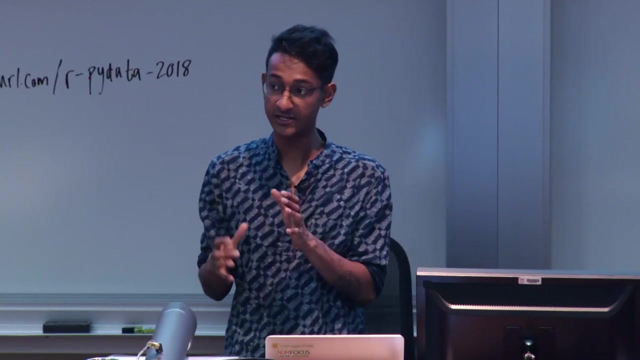 And why does it say that? It basically says: okay, let's just look at the first document. So the first document was which, in our test data, was classified into class 0. Do you see, So, based on the contents of what was our first test file, 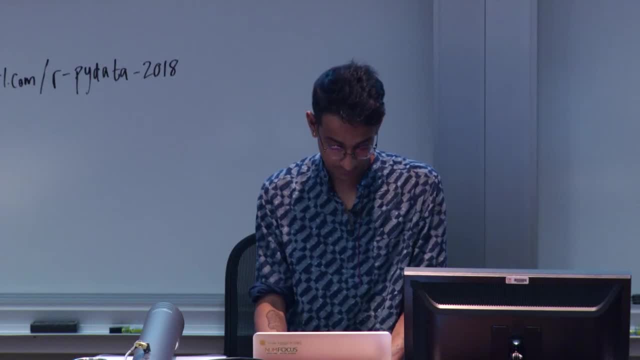 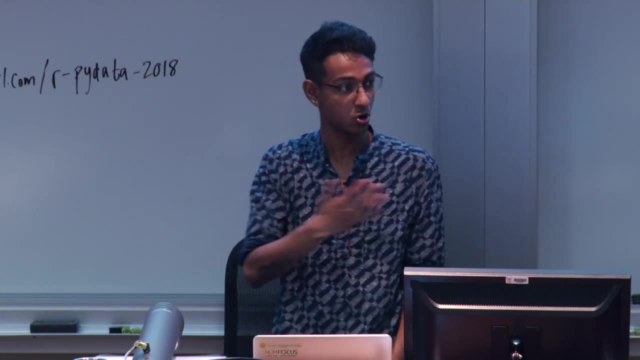 it was placed over there, And 3 is our fourth class, and the 22nd document was put in our fourth class, and so on and so forth. So now what you've done is you have X-test, which is all of your testing data. 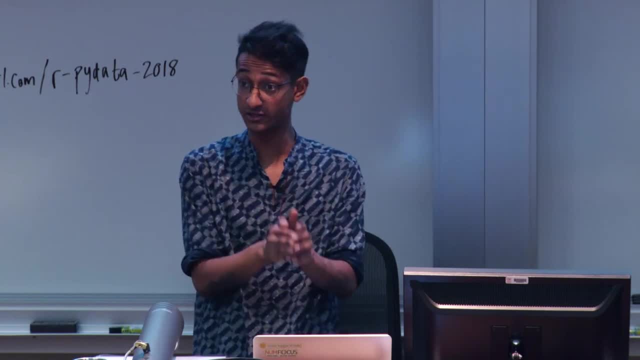 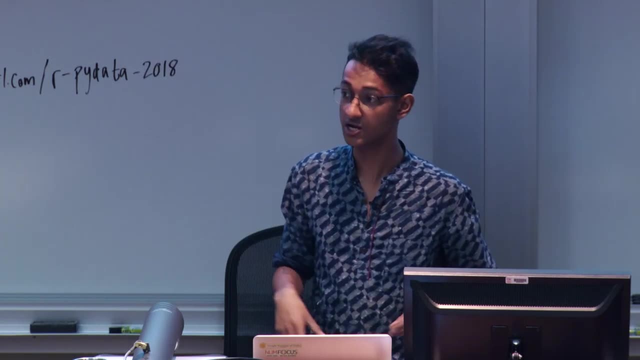 which we didn't know what class. this was right. We are now using this model to classify this test data into one of these four classes, which is what has happened over here. Classification is not limited to only text, by the way, The same methods I've used before. 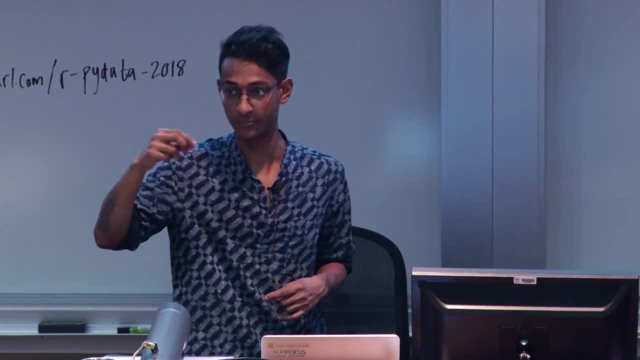 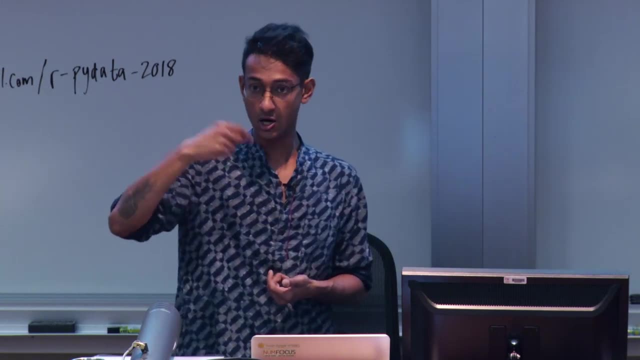 like TF-IDF is particularly for text because it's term frequency, But you also do image classification right. That's like a super common task where you have handwritten- like you're handwriting from 0 to 9, and you want to see every single handwritten- 0 to 9,. 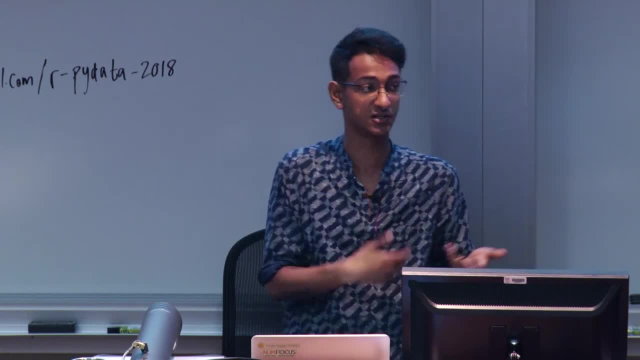 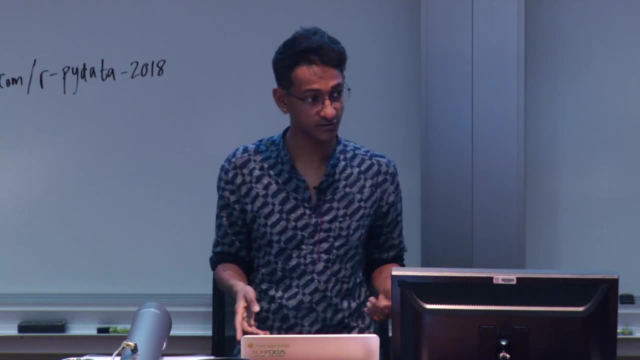 what does the computer call it? That's also classification. It's just the labels and classes are different in a different context. But classification is a generic machine learning problem In the context of text classification. what just happened was I had a document. 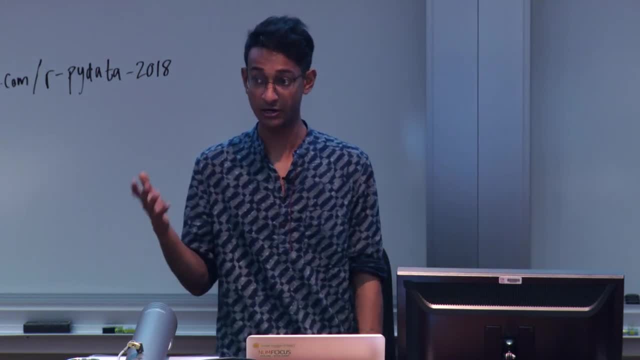 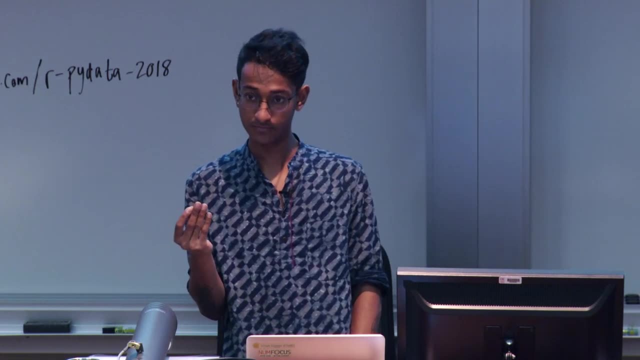 which is either about atheism, religion, graphics or space, and it was classified into one of these four based on the contents of that document, right? Everyone cool with classification, more or less. So here we use scikit-learn to do it. 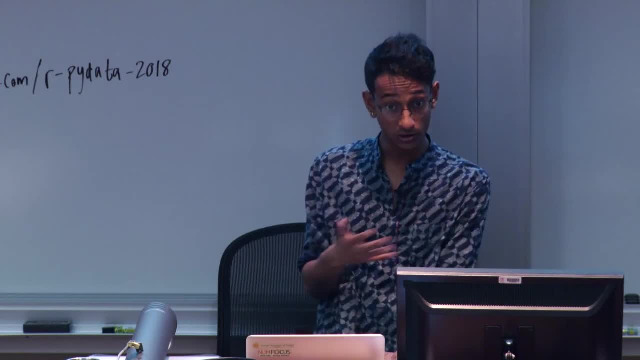 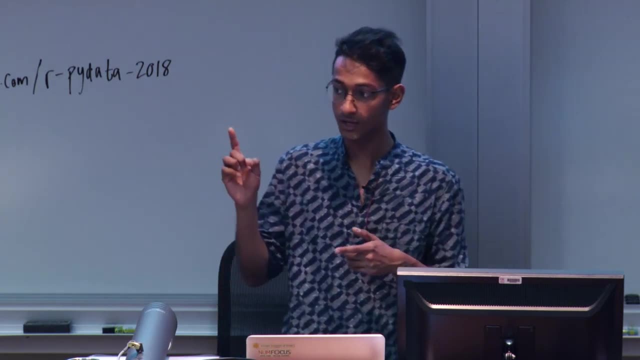 Scikit-learn has pretty much the same kind of pipeline for all classification tasks, So this kind of teaches you how to do classification for other contexts as well. But in text you'd use TF-IDF and all these things over here. So Gensim and scikit-learn are kind of different. 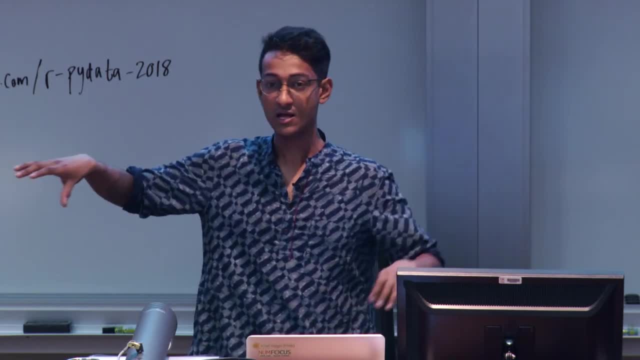 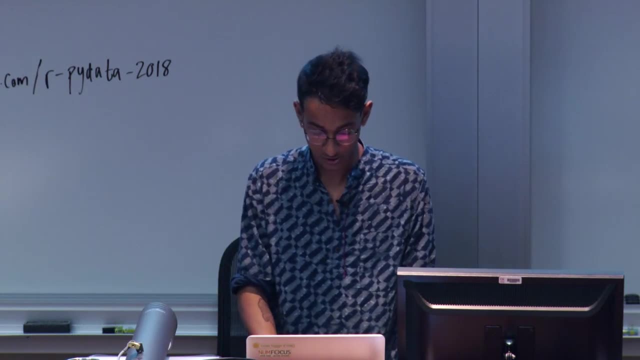 in that context of the kind of problems you want to solve and the way you want to do it. but they're both fairly easy and you can kind of use the same corpus in both places. It's pretty cool. SVC is something called support vector classifier. 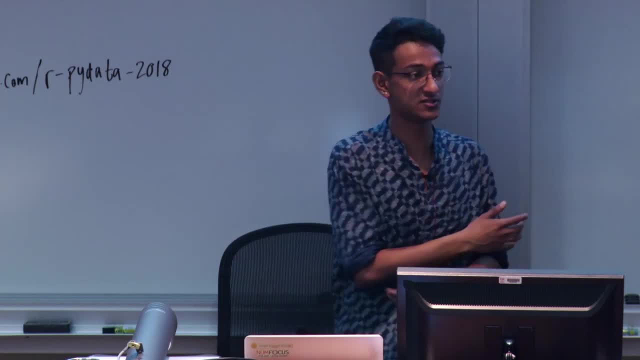 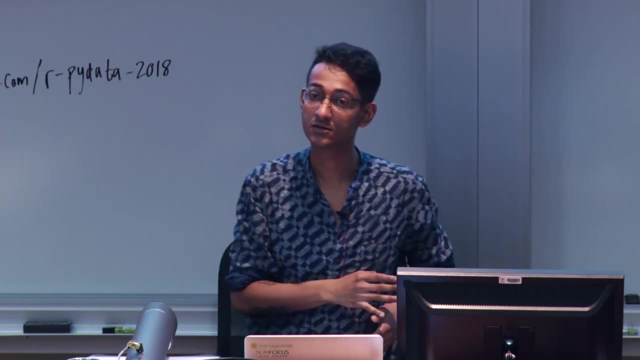 where support vector machines are another kind of machine learning algorithm where you try to create a plane. instead of classifying by a line, you use a plane instead. Yeah Yeah, In TF-IDF I can see a bunch of parameters for document frequency in the idea. 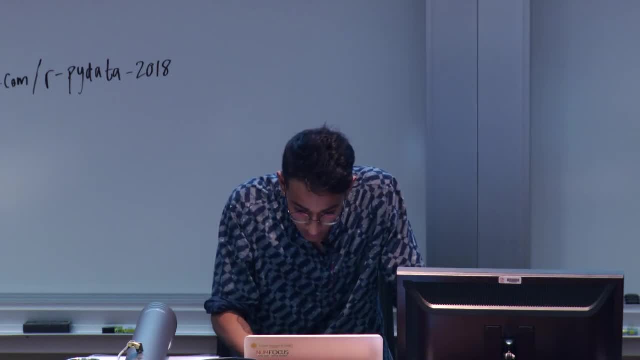 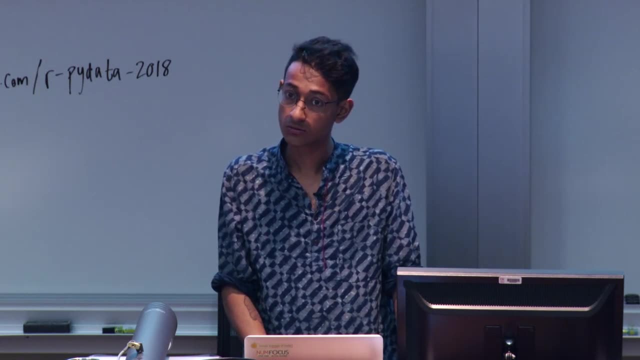 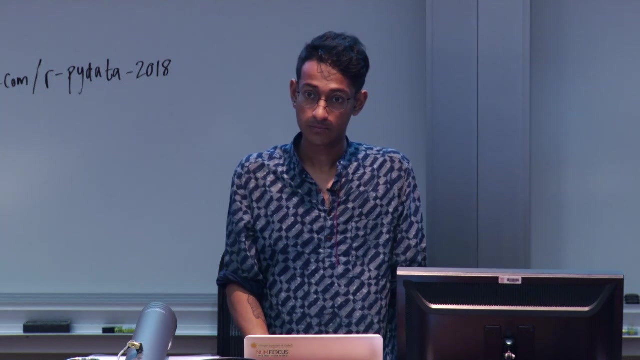 Sure, That I understand. But how does it take, considered like TF part, Because we have multiple documents? Sure, Like some frequencies are attached with each document, right, Sure? So how does it make a single vector throughout the corpus? 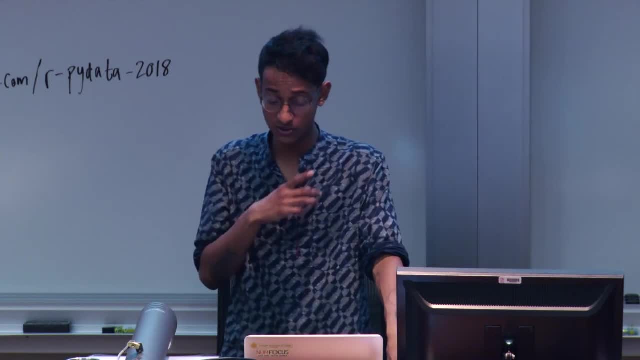 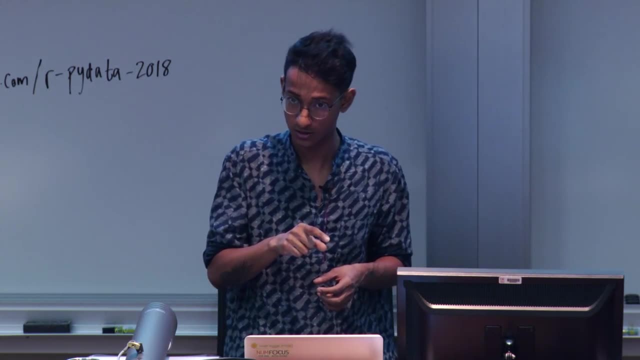 So I'd actually have to be absolutely honest. so the question is basically: how does the scikit-learn TF-IDF vectorizer find the term frequencies for all the documents Correct? So I'm not sure how scikit-learn does this under the hood. 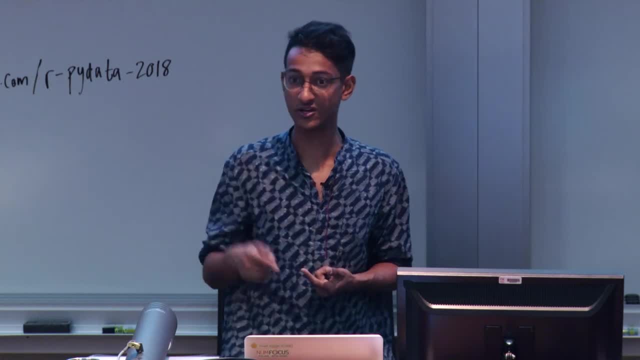 I would have to go and double check and then maybe we can like look at it later. I'm not sure, I'm not actually sure how it does it under the hood, but it does seem to do the job because this particular module right. 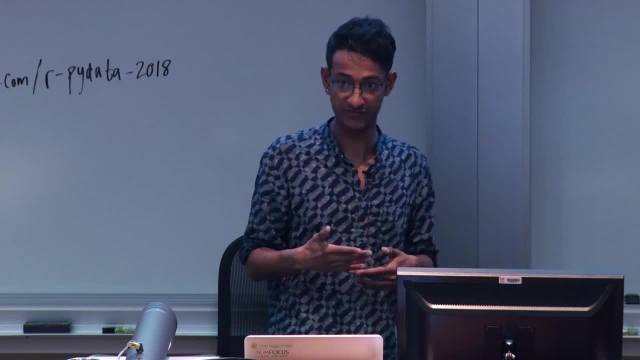 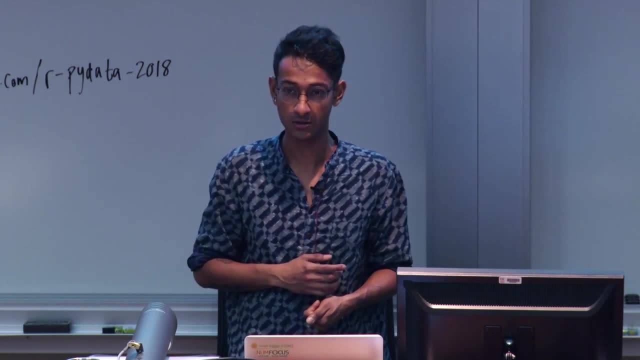 is for text analysis, like the TF-IDF part. so the way they've set it up is such that it takes care of this, But I'm not sure exactly how I'd have to look at the code or look at the parameters and see what's going on. 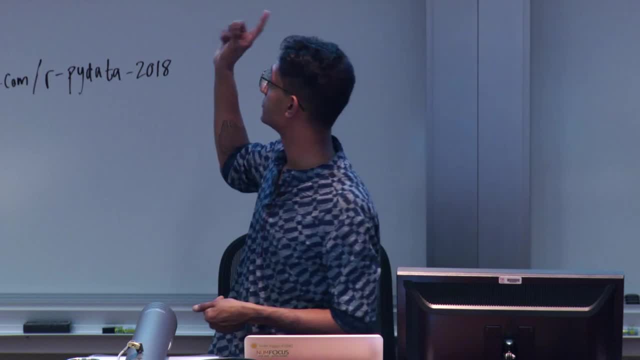 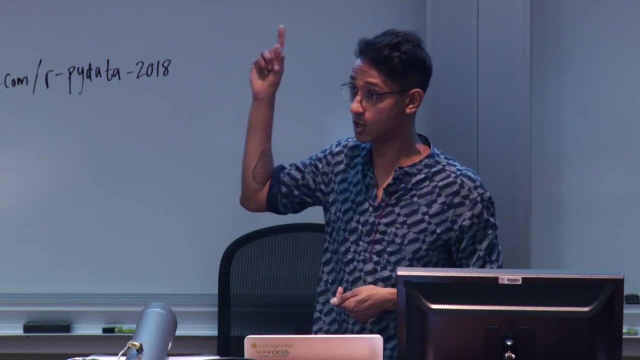 But it's a good thing you pointed out because you can also look at the other parameters which are part of that. which says stop words is English. We did the stop words bit a bit more manually before Here. scikit-learn does the stop words as part of it. 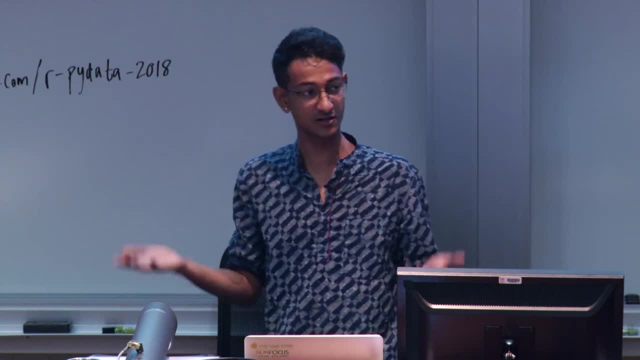 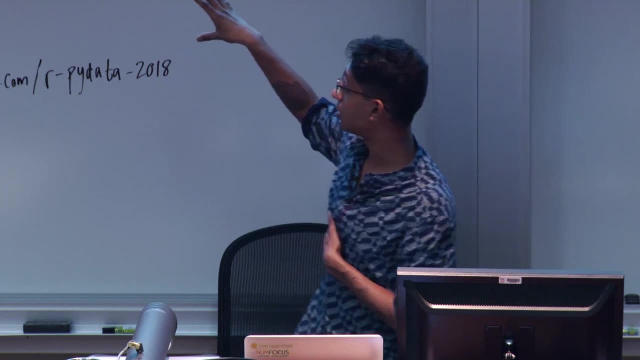 but also means you cannot play around with the stop words as much. so there's like certain levels, Use IDF true or false, then the maximum document frequency, minimum doc. So these are the standard values which I picked up off scikit-learn. 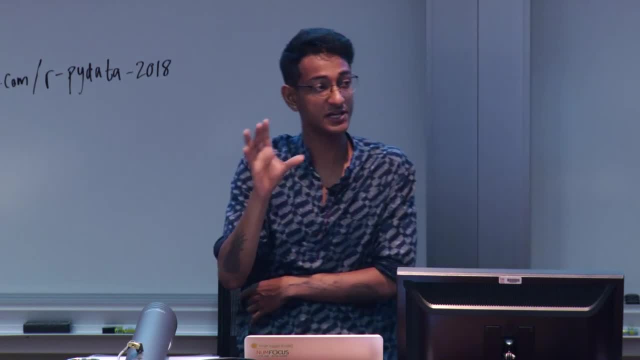 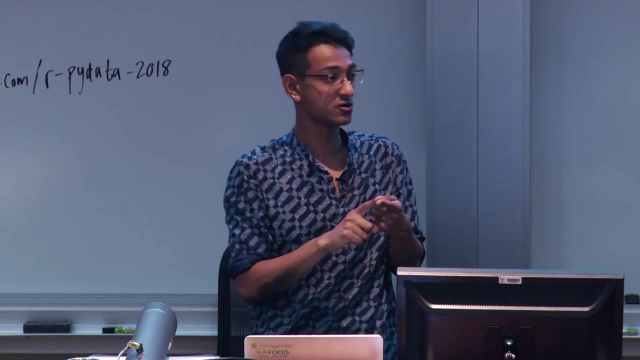 You can really play around with it. Again, to be clear: TF-IDF term frequency- inverse document frequency: different way of representing our textual documents, similar to bag of words that you used before, but a little more nuanced, And you don't have to use it. 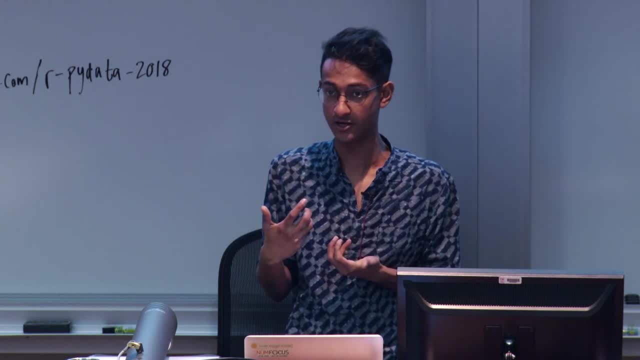 It's just useful and you can do cool things with it and represent your data better. To answer your question in particular, we'd have to go over the scikit-learn documentation and figure it out. I don't want to give a wrong answer. 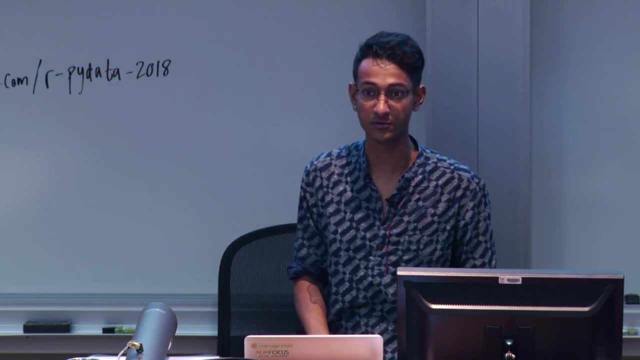 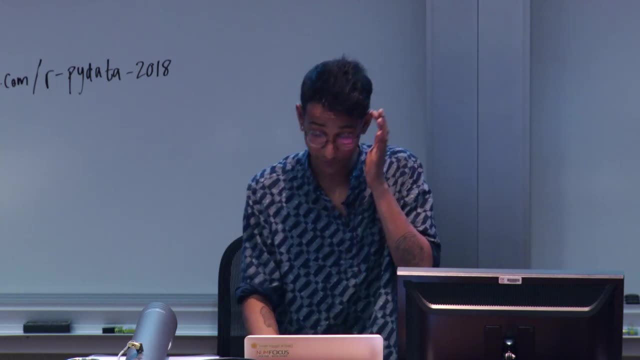 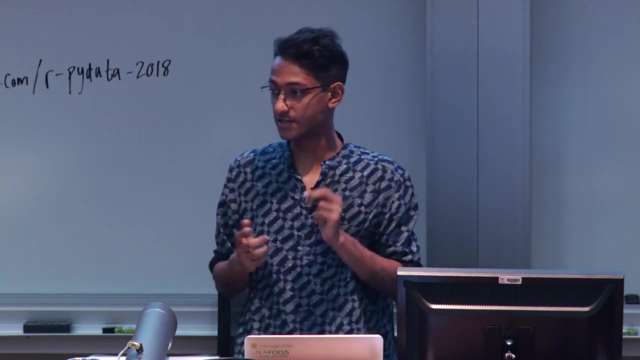 which I'm not 100% sure about, but we can definitely think about it. Cool, So we are at the last part of the tutorial. I will be going over this part a little faster because there are 12 minutes left and I want to give at least. 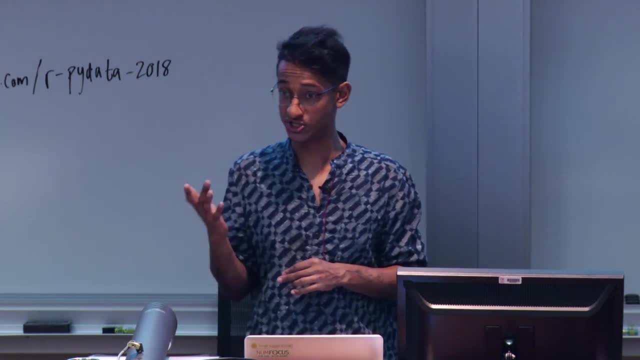 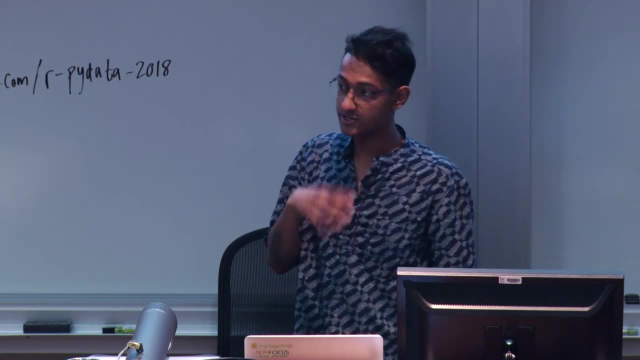 five to seven minutes for questions. If we don't have questions then I can do this in more detail. But I'm going to go really fast into this. So deep learning is a subfield of machine learning I don't think I really introduced. 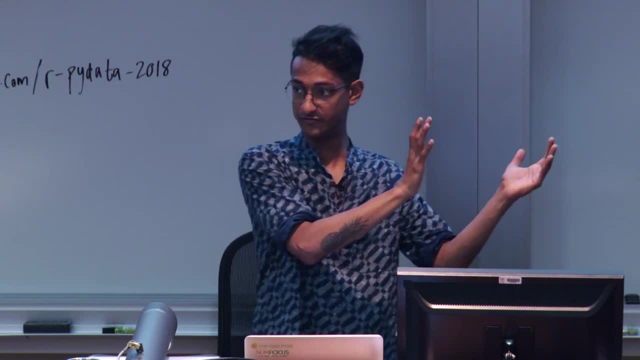 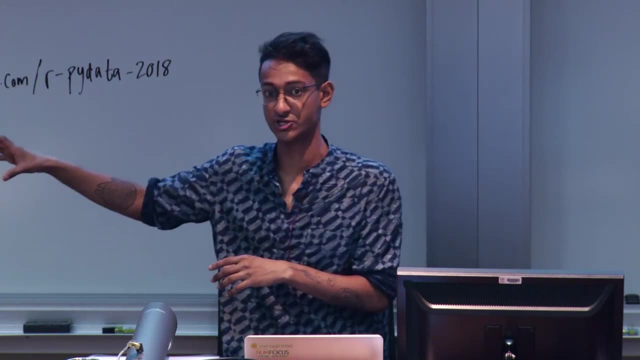 what machine learning is. Machine learning is basically a lot of data. then you put it inside a usually statistical or an iterative algorithm which learns from data and makes prediction. That is a general idea, which we've been doing before this as well, right? 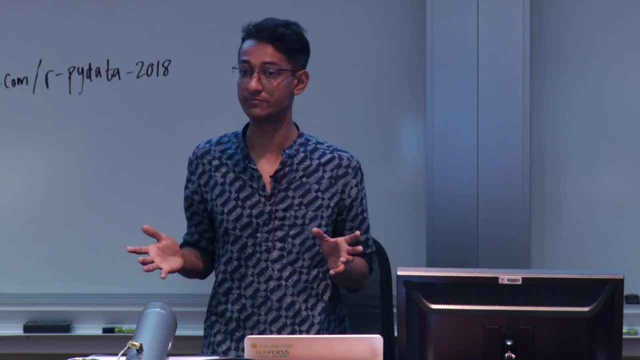 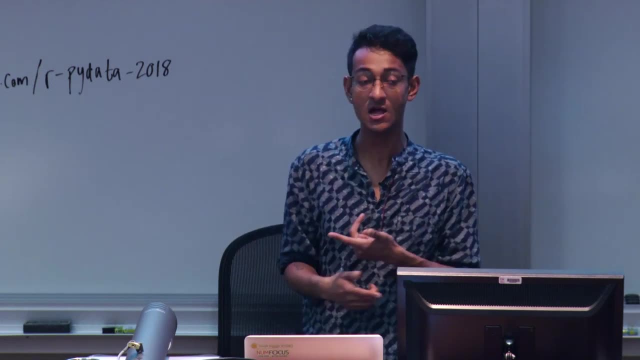 So deep learning, Deep learning is. it's called deep learning because we use something called deep neural networks. There's also something called shallow learning, by the way, when we just use, like a neural network, just one or two layers. The reason it's called deep: 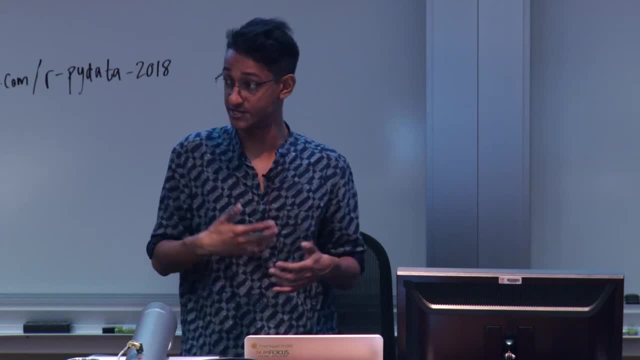 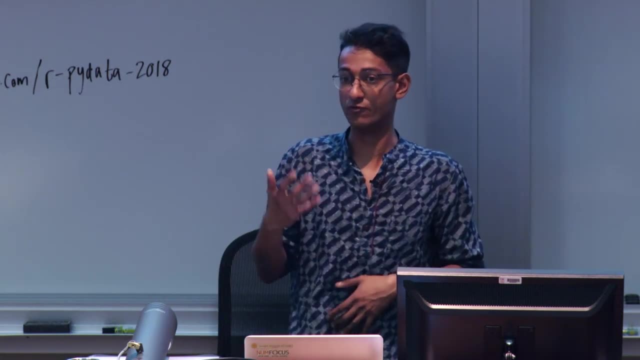 is because you use multiple layers. The more layers you have, the deeper your network is And in general, deep learning largely comes. I mean like all these kinds of neural networks which have over like an arbitrary number of networks, like eight, you would say, layers. 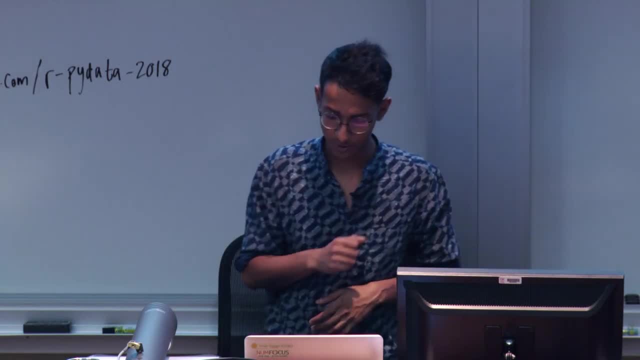 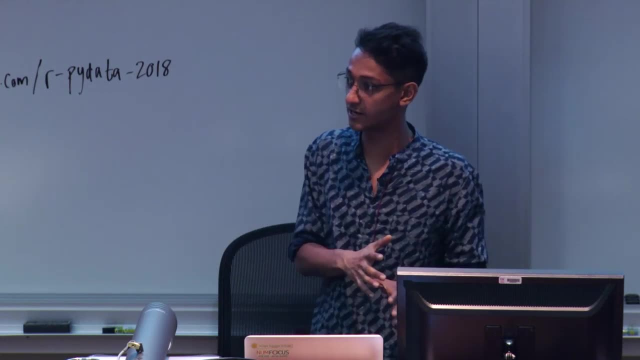 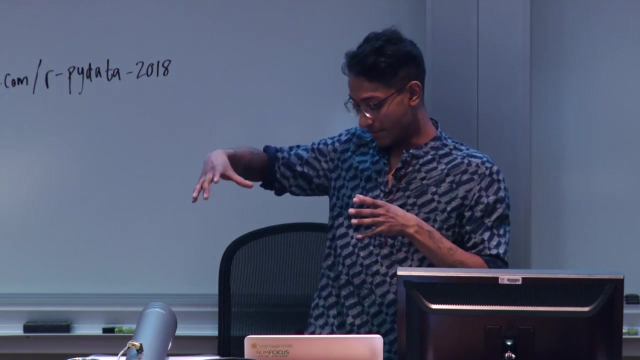 would all be deep learning networks. Pardon me. There are many kinds of deep learning networks or neural networks in general. There are a lot of different kinds of neural networks. Neural networks are kind of like they are a mathematical system or a mathematical construct. 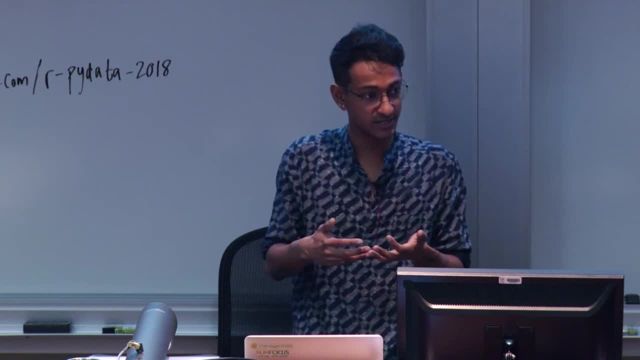 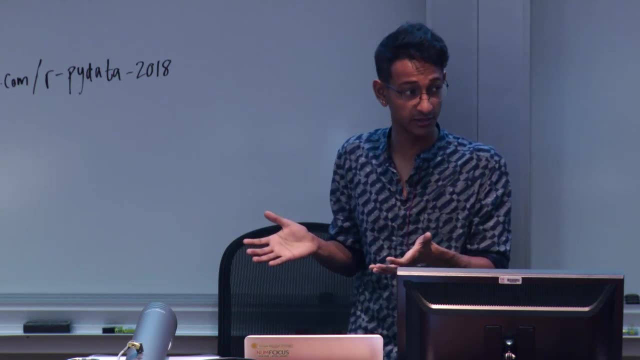 which is kind of modeled after a human brain, more or less in the way it passes information between different nodes. I will not get into details of what a neural network is because, again, that is like a huge talk of its own. What you would know is: 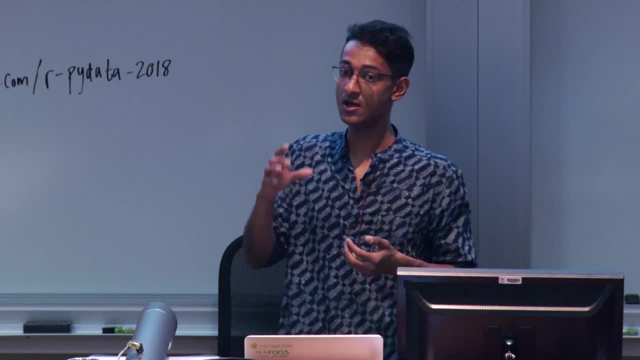 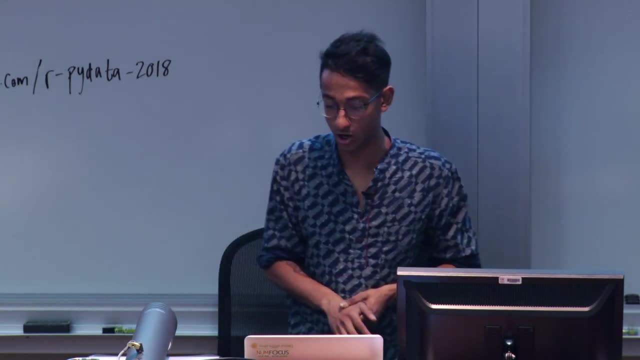 these are more powerful, computationally intensive class of machine learning algorithms which are loosely modeled on the biological brain. It's a very brief idea of what they are. There are many different kinds of neural networks. What we will be using is something called. 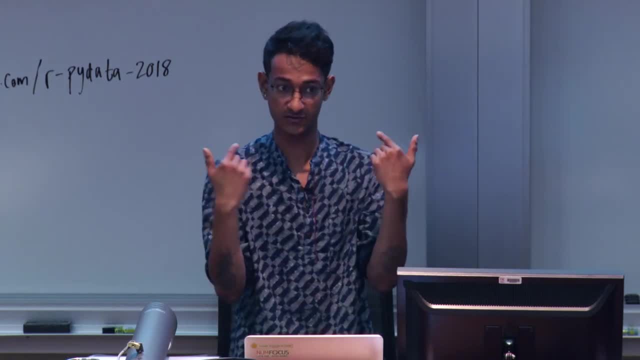 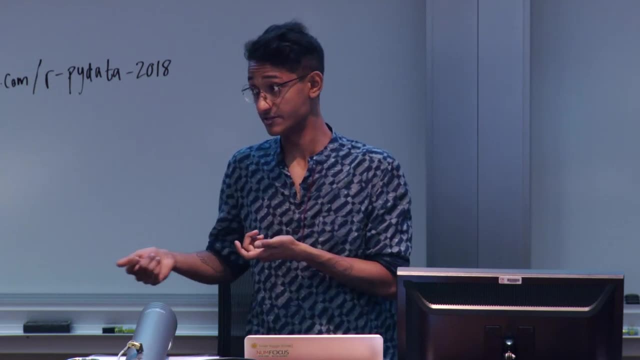 recurrent neural networks, which are kind of like stacked, in a way where the data is recurrent. In particular, we'll be using something called LSTM, which stands for long, short-term memory, which is a way, because memory is important, because you have to remember context. 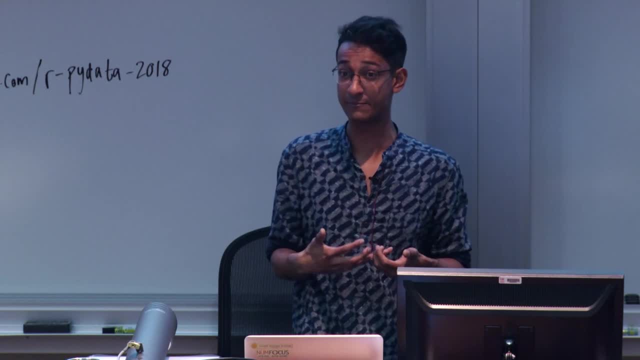 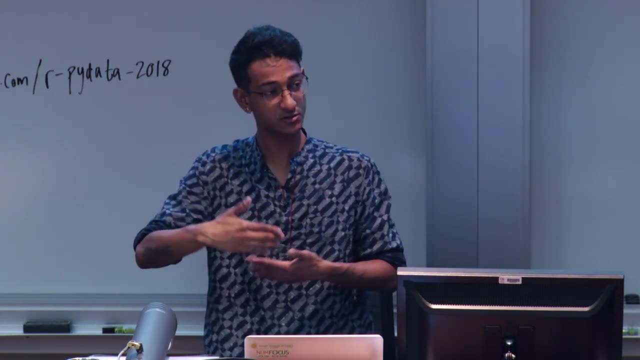 Someone asked me about context before. Neural networks are really good at capturing context. Someone also mentioned LDA2Vec, which stands for LDA2Vector or Word2Vector. These are all things I've said before. All of these are really useful. 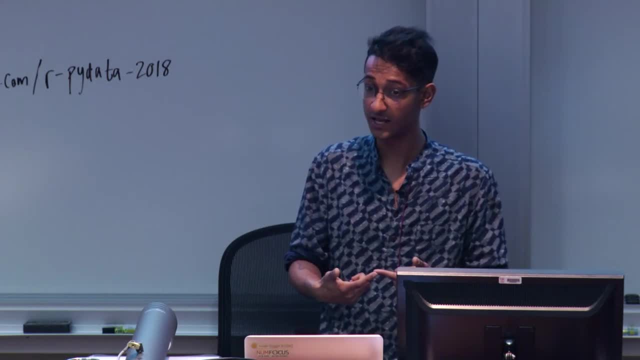 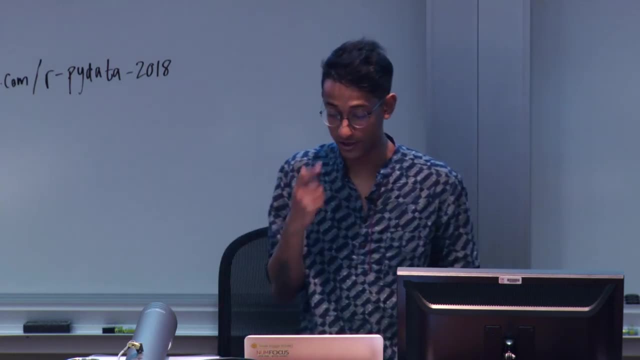 in understanding context because they have memory, So to say. in terms of how they learn these models. They're more sophisticated, more intensive and really cool actually. I've put up a lot of links over here and I would really really recommend reading these links. 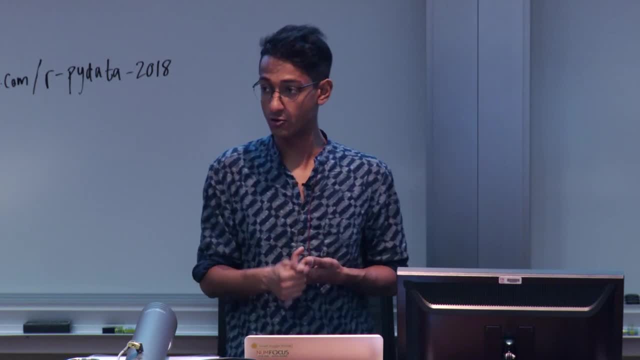 because it's an excellent blog post over there. these two links. I would also any word you don't understand in this tutorial. just Google it. There's a lot of really nice resources. or mail me or raise an issue on my repository. 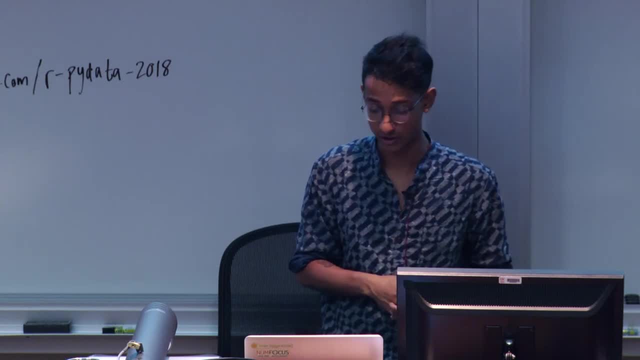 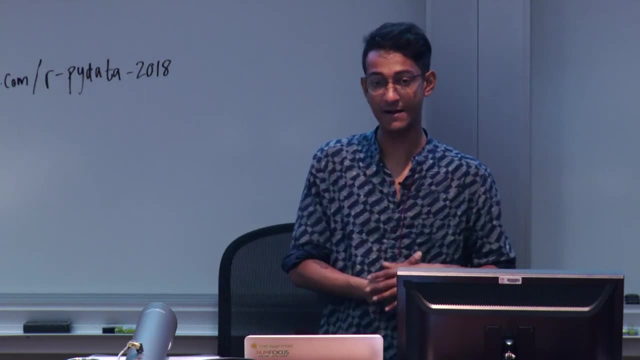 and I could direct you to some interesting reading material about these things. Now, what we're going to be using is this machine learning model to learn text. The way it happens, I'm going to kind of be a little fast about this, but the general idea is that. 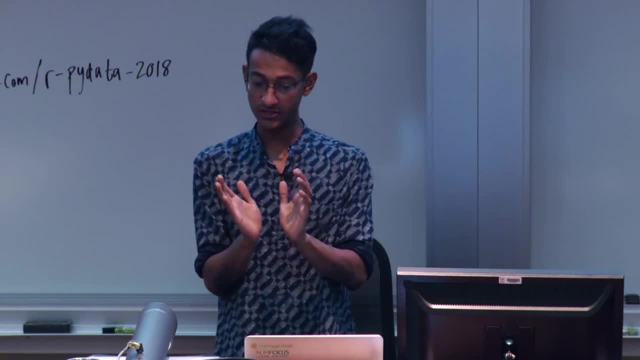 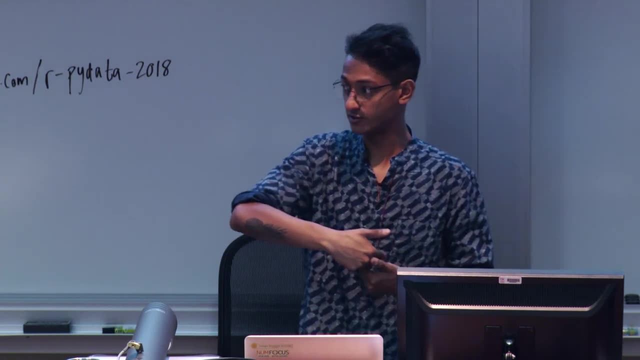 this neural network learns based on the context of one particular character. what is the most likely character on either side? Now you extend this to words and so on and so forth. So what does this mean? It means I am most likely. 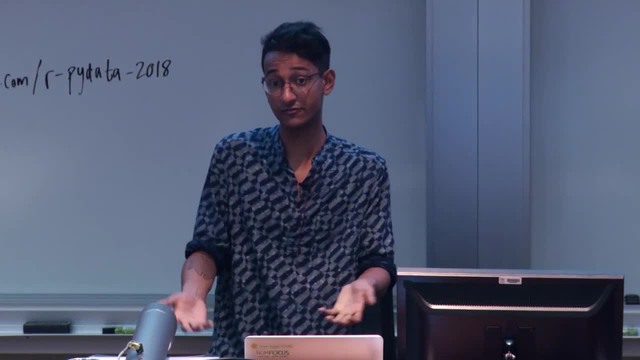 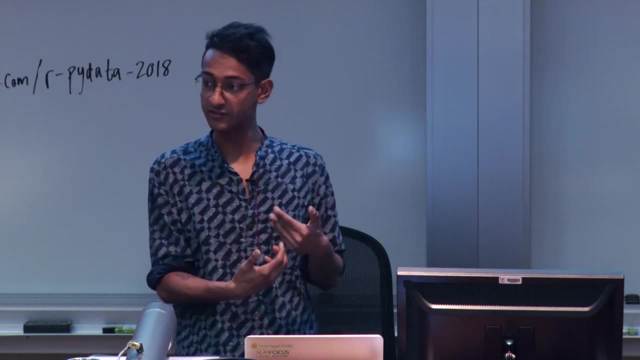 personally, I am most likely, if I'm going to be talking about myself, for example, like in this context, I would start a sentence with I right, So neural networks starts to learn these things that you start sentences with I. 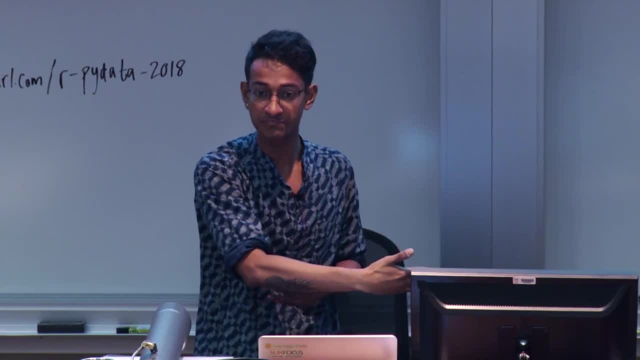 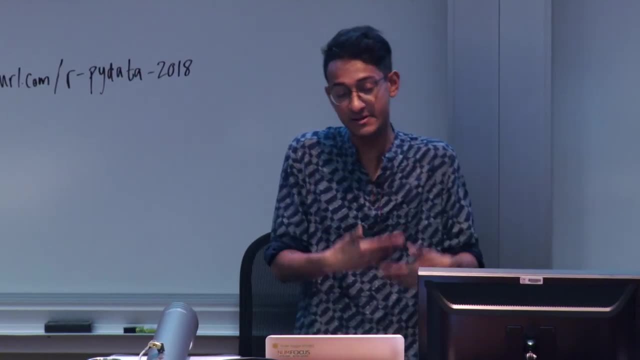 or he or she or they or whatever. It learns these things And it learns after a particular word. what is the most likely like? after deep, I'm probably going to have fried after that. I mean, it's just going to learn. 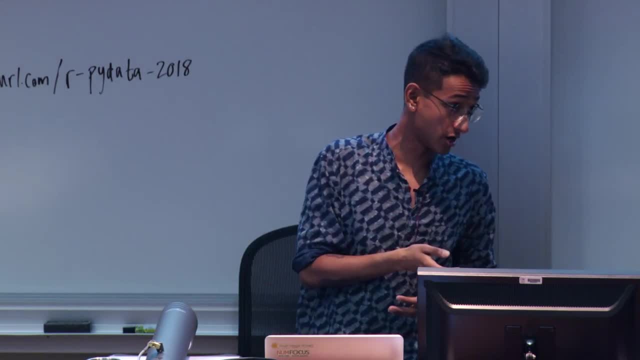 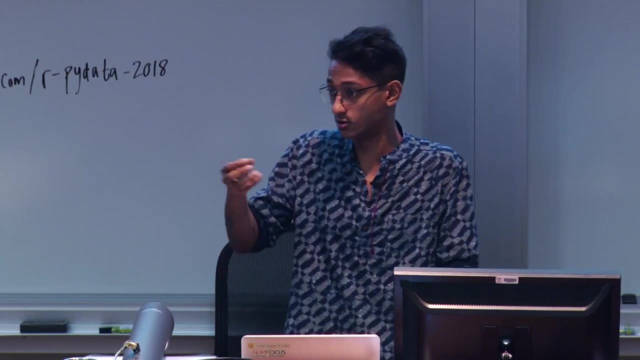 different kinds of things. based on the context, based on the data you're training it on, It could be drastically different, But what it learns is what is the most likely character or word after this particular character would I already have? That's what it's going to do. 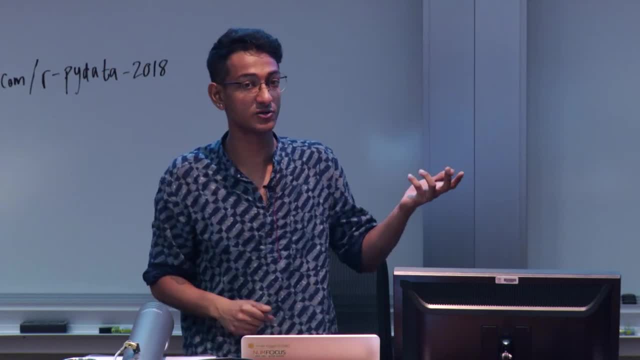 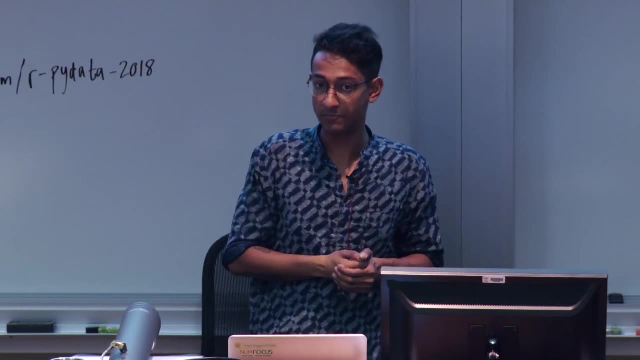 Now, how is this cool? You can pretty much teach a neural network to talk like Shakespeare If you give a whole bunch of like, not a whole, like every single play written by Shakespeare, which is also an example given in this blog post. 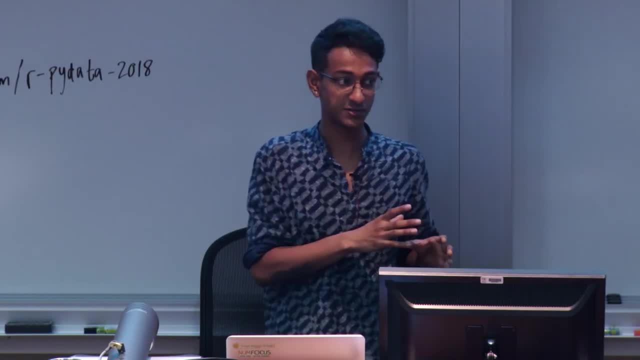 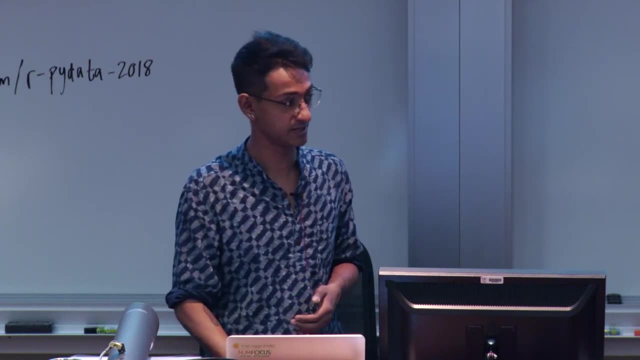 If you give every single Shakespeare play, this computer would learn that. this neural network would learn that in the context of Shakespeare plays after thou, the most likely word would be hast or whatever. So it's really cool, It learns the most likely word. 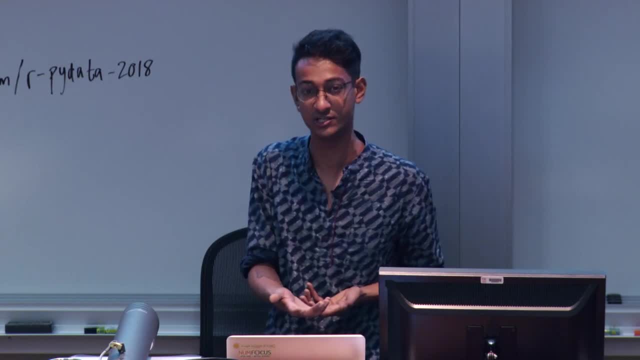 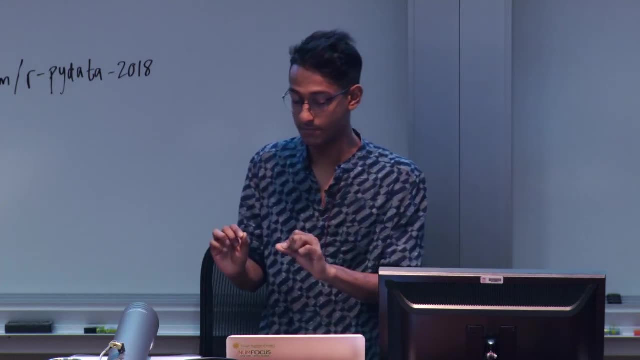 What this means is it learns English or Spanish or whatever you're teaching it. It doesn't really know what's going on, but it knows what's the most likely thing to happen. Now I've told you about this and I never have the time. 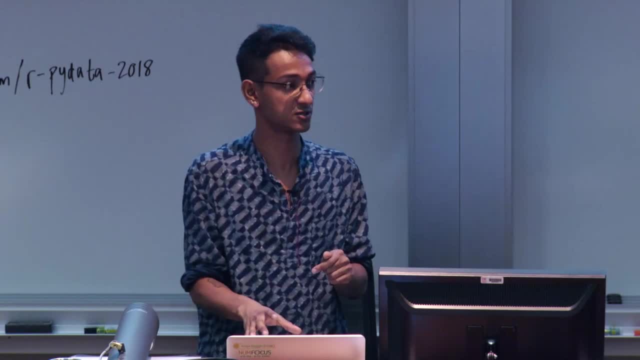 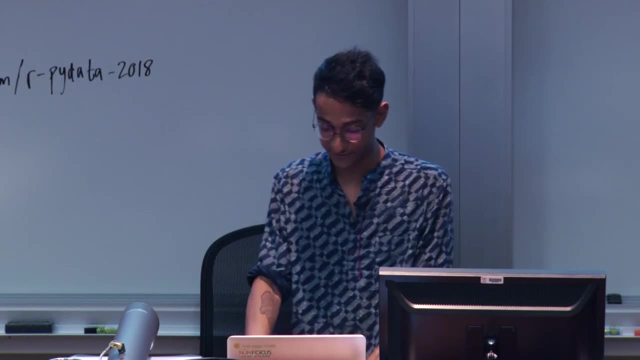 to get into the details of how to do this, but I always still have this code over here because it's useful. Let's go super, super fast. There's like five minutes left, So what's going on over here is this is just. 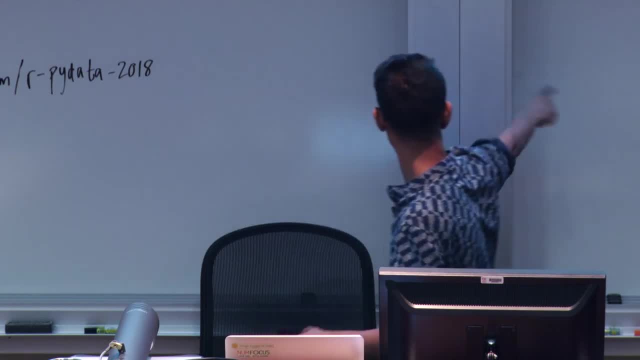 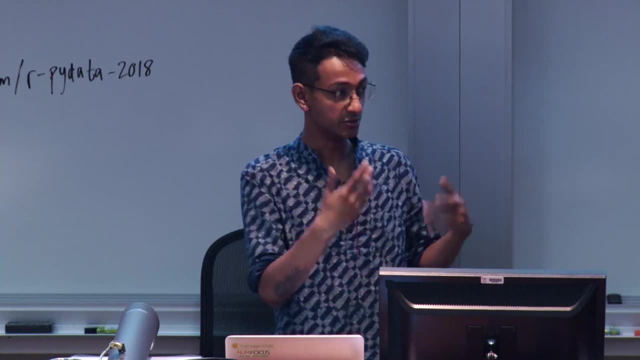 my imports. This is just remember. I talked about how data is stored. This is called one hot encoding, where you have one yes, and then all of these. This is just to show you the kind of data which neural networks take in as inputs. 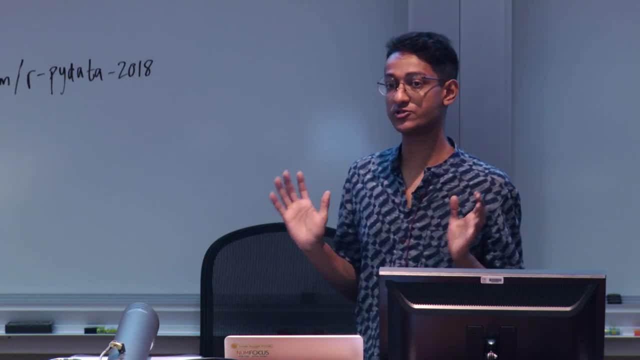 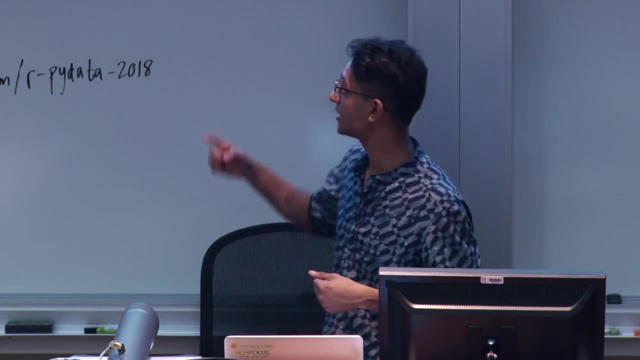 Now. so a lot of the parts of these neural networks are very complex in the way they're made right, But there are lots of tutorials to tell you how to make these neural networks, so you don't make them from scratch. This is one way. 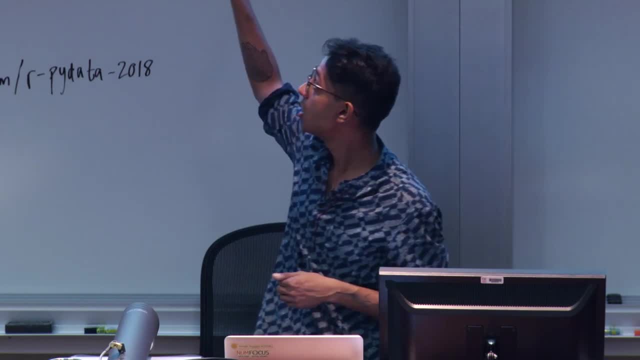 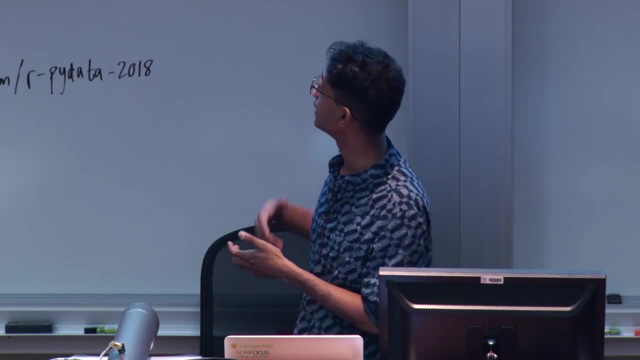 So you have like a hidden dimension. Then you have what? the drop rate, softmax, All of these are the characteristics of these neural networks. Softmax is a kind of activation. Then you have drop rate, which is at what point you stop overfitting. 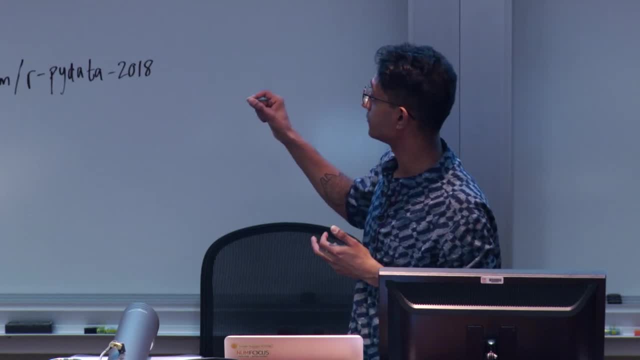 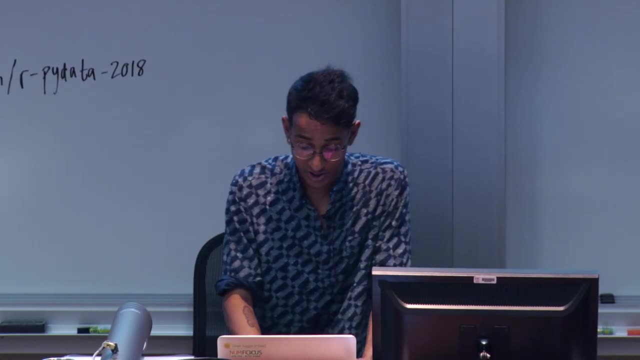 So these are a lot of things which are particular to neural networks, and this is how we're creating our model. So I'm just running these three functions. So over here you have certain characteristics of these neural networks which, again, I do not possibly. 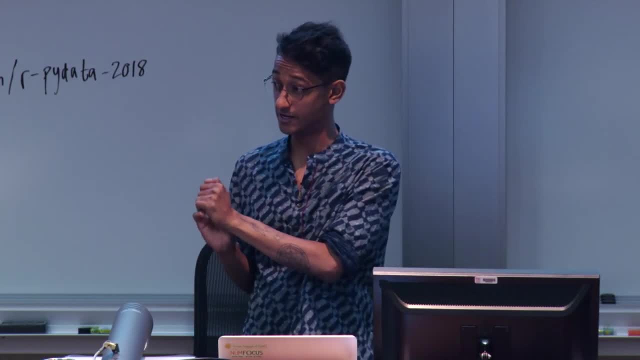 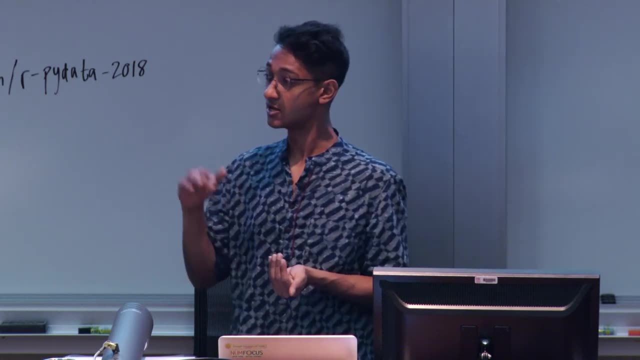 have the time to explain it to you, but I would really recommend going in and finding out what exactly they do, because, depending on how you want to keep these parameters, the way your neural network learns, things are very different. Neural networks also take a very long time. 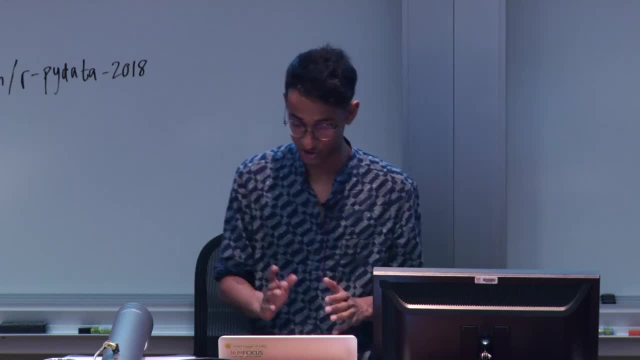 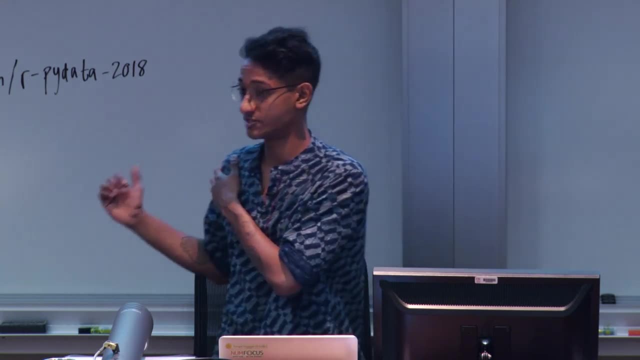 to actually train, like hours, days to train, depending on how big it is right. So all this code over here will take you. you don't need to really pay too much attention to it right now. This is for you all to try out. 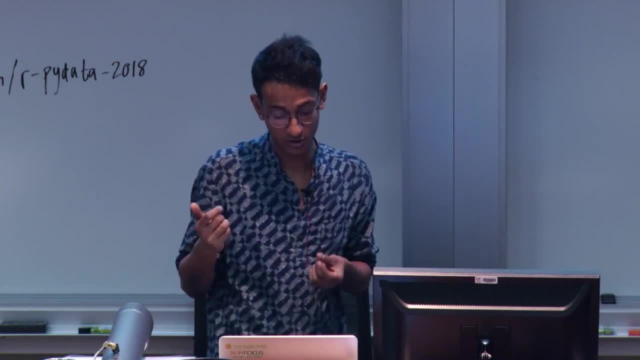 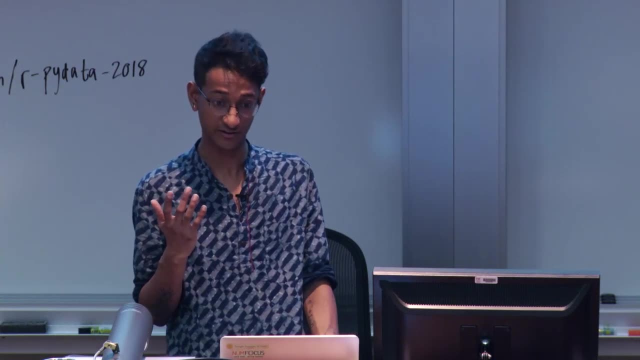 when you're home or wherever. So this is what we're going to be doing: to get our models. This is how we train it, and now what we're going. what I told you before is: I generate text right, So this is. 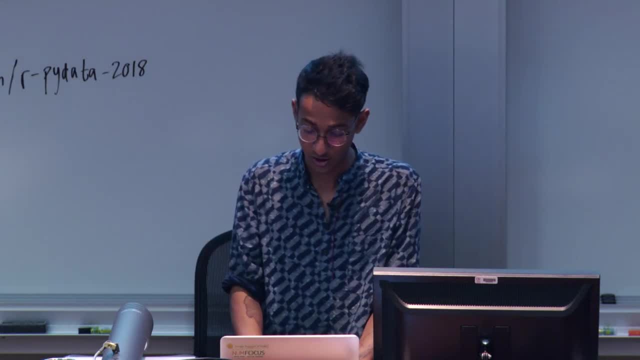 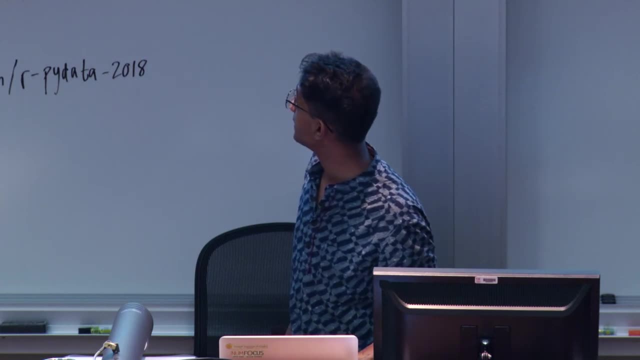 now our model. the code, the functions are done for training the model. This is how I'm going to generate my model. It's basically really really fast, right? I start with a random seed and then after that I basically say: 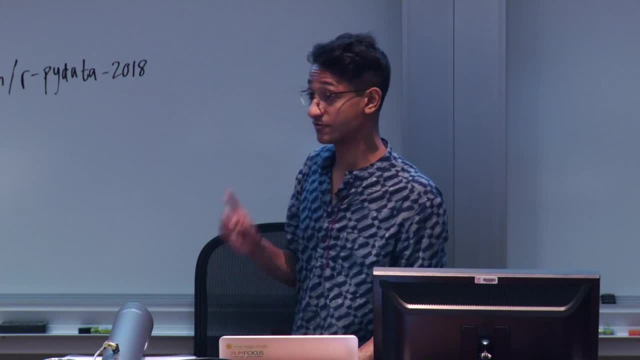 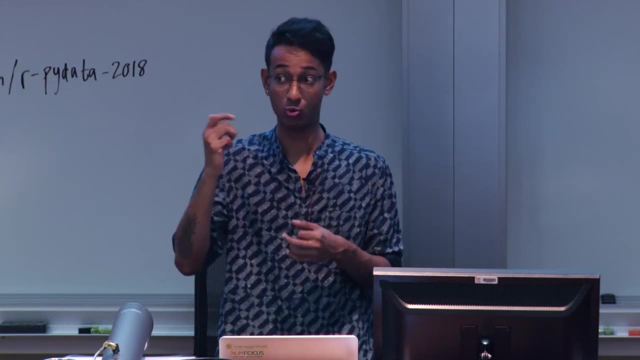 based on the current word. I make a prediction of the based on the current character. not even this is a character level learning model. There's also a word-based learning model. right, This has actually learned words on its own, not just. 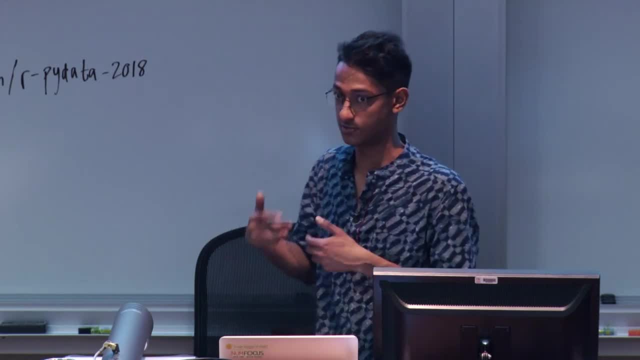 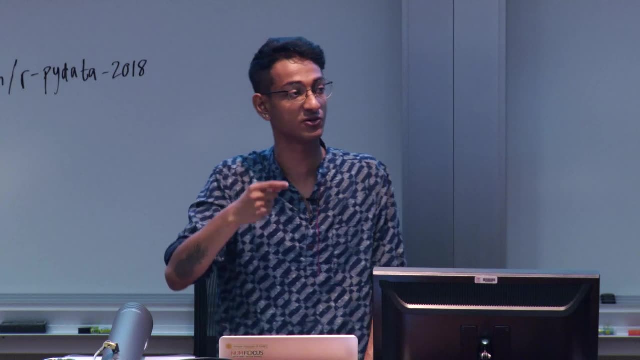 it's learned how to make words, Not just what comes afterwards. It's a pretty complex model, So what's going happening over here is based on the previous word. I'm going to make a based on the previous character. I'm going to make a prediction. 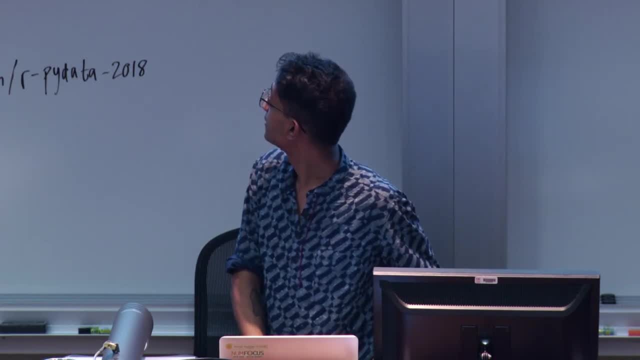 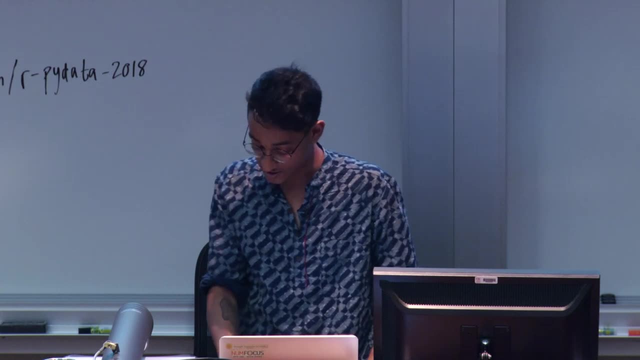 of what the next character is, and it does that, and I'm going to be using the lead background corpus. I had this Game of Thrones corpus, just cool, but it was totally legal, So I'm going to. actually, you never saw that, So I'm going to go back. 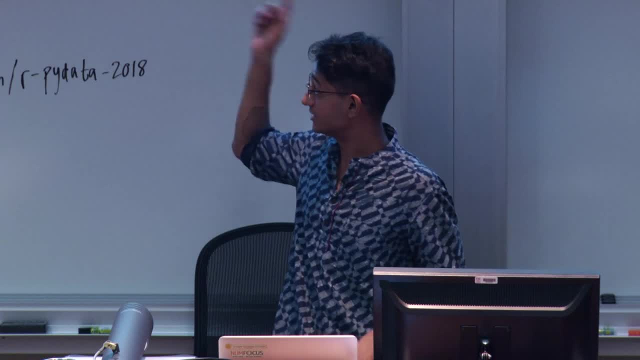 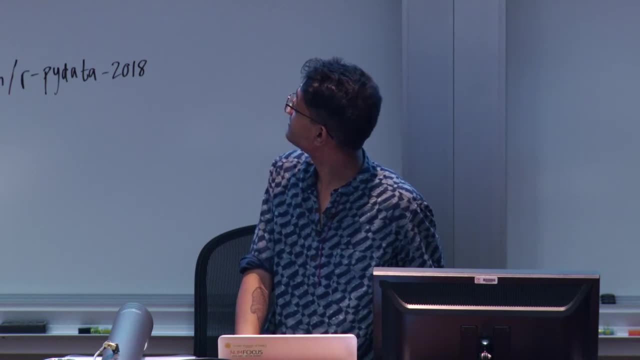 and use the, the lead newspaper corpus which we were talking about before, and these are all my unique things and characters and mapping and bam bam running a lot of code. But basically the point is, what's happened over here is I've used all of that. 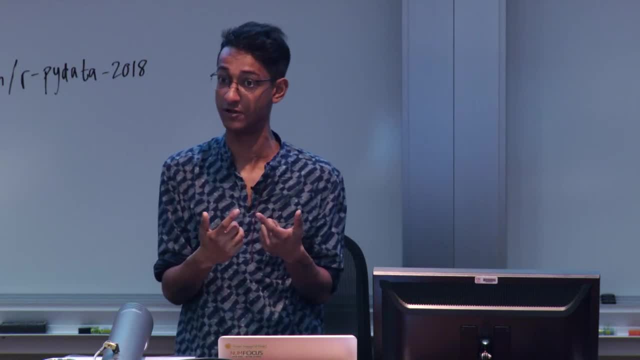 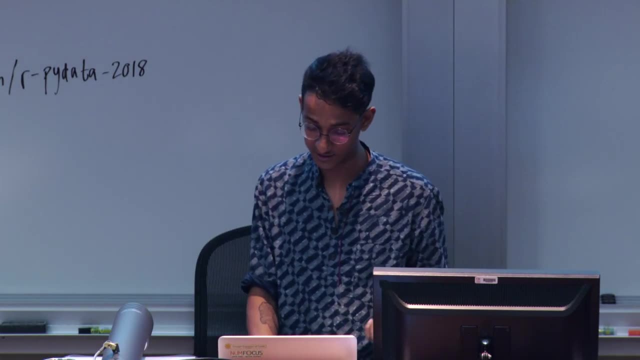 newspaper article corpus to kind of teach this model of what exactly did newspaper articles look like in the, and it's going to do that Now. it's going to take some time to load, because it takes some, but I want to very, very briefly show you. 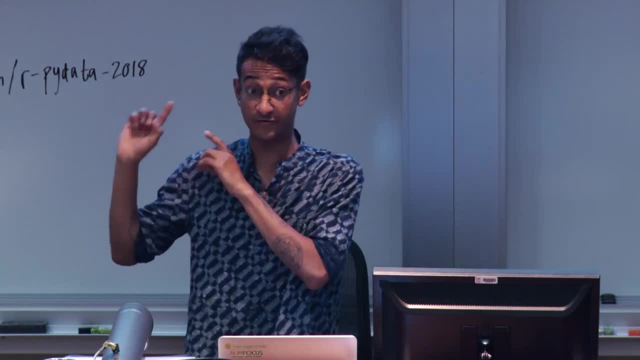 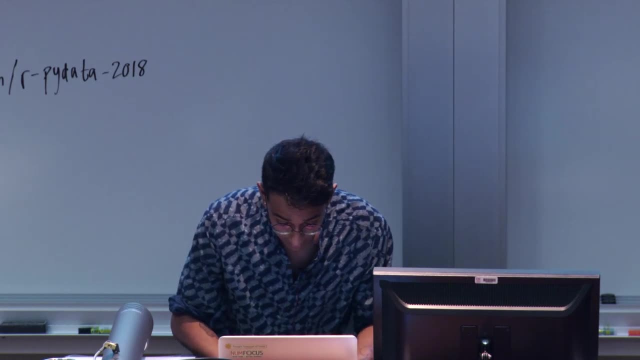 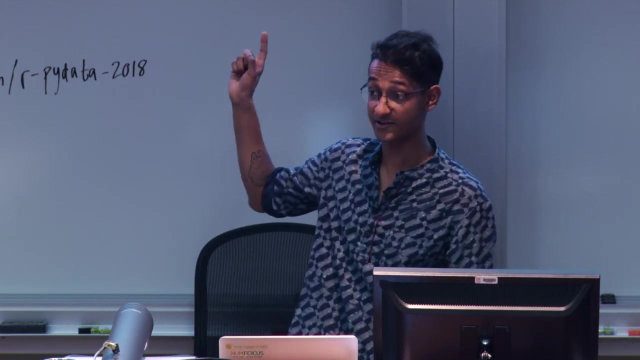 some of like. what I've done is. what you've seen is the actual code of how to do this yourself in this blog post, which I've linked to this over here. over here, this is Shakespeare written by a neural network. This is not a human being. 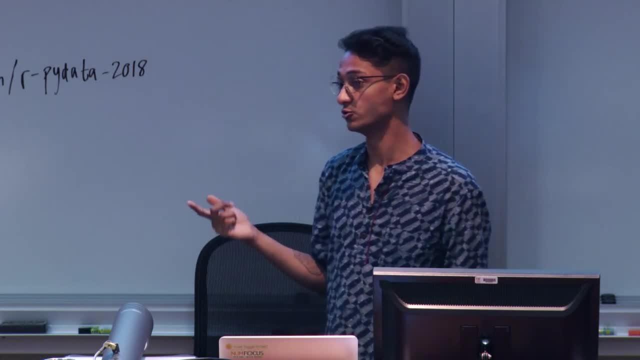 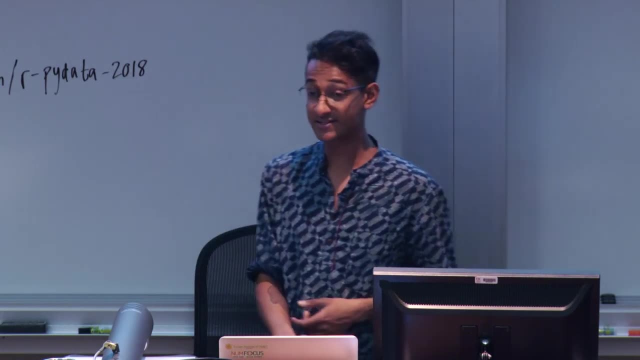 This is a neural network which has done this. I would have loved to show you Shakespeare data myself, but it takes a lot of time to train these models. This is an example from the blog post which I've linked to. It has- actually it has- learned how to write code. 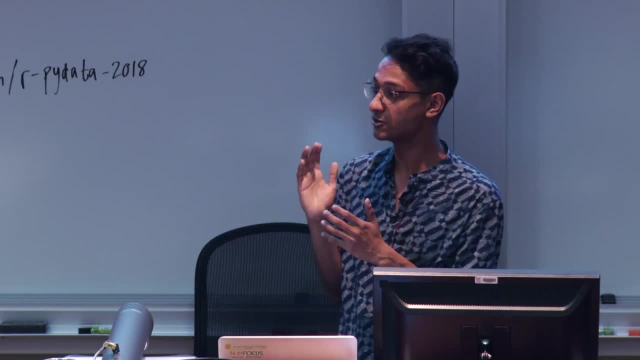 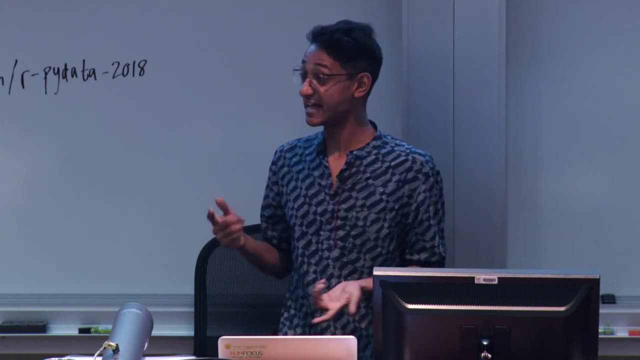 It can do latex, It's. it's pretty nuts. You can do a lot of very cool things. I'm not sure about how useful it is- I'm not always 100% sure, but it's still. it's still very interesting. 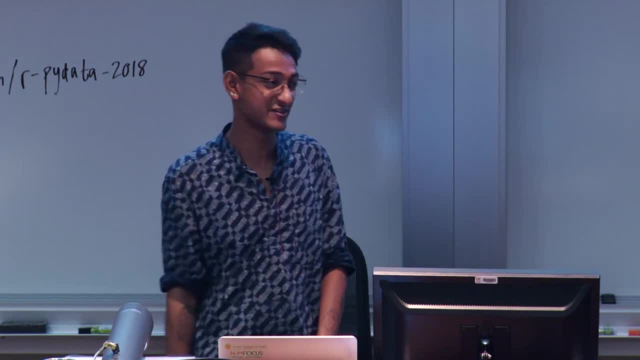 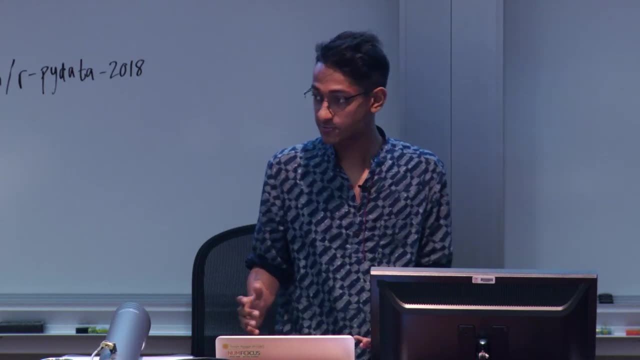 and it could possibly have some business. I'm a researcher so I can just do things for fun and not really care about how it's useful in the real world. but this is one of the cool things you can also do, So that's pretty much. 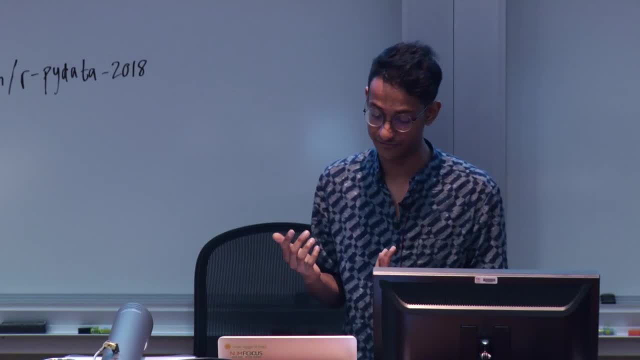 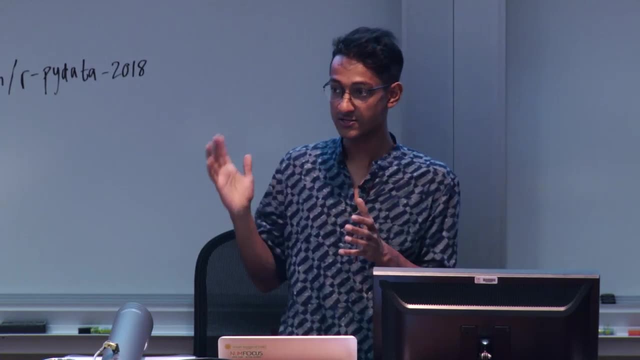 what the tutorial is. I'm sorry for running through the last bit of it- I usually end up always doing that- but I want to include this in the tutorial. You can have the code and look at it in more detail. So this is everything.